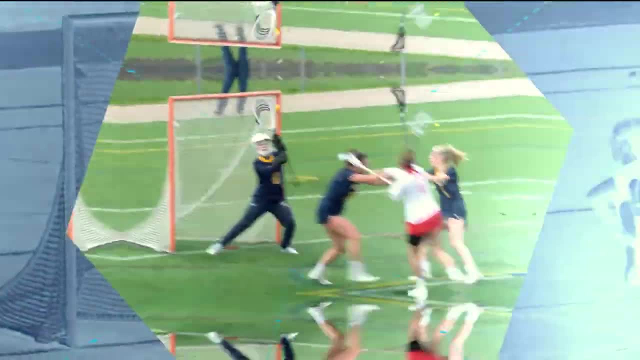 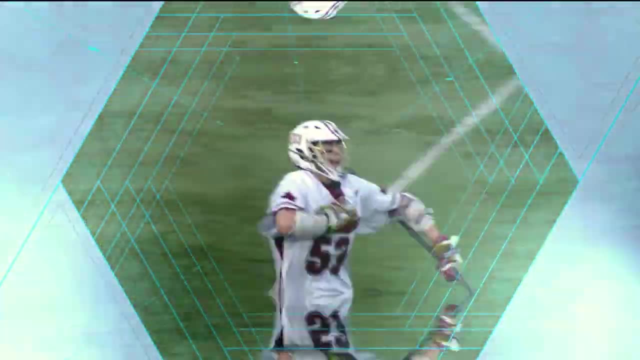 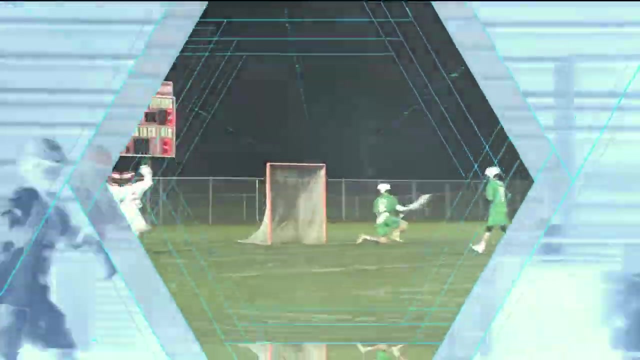 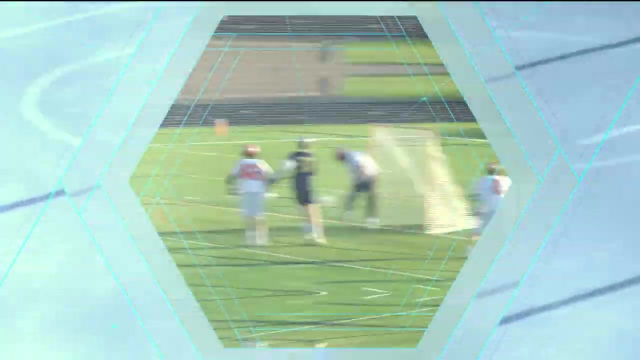 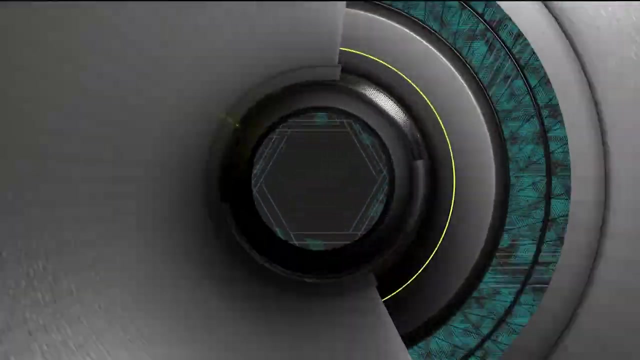 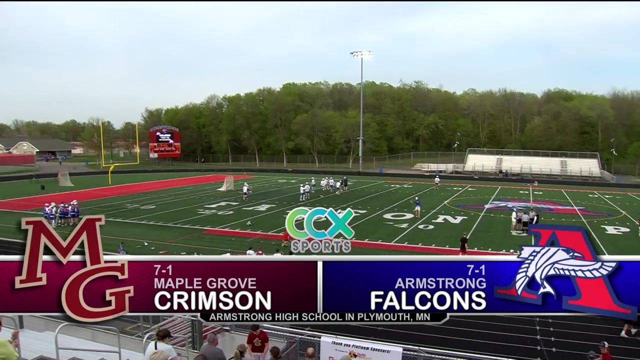 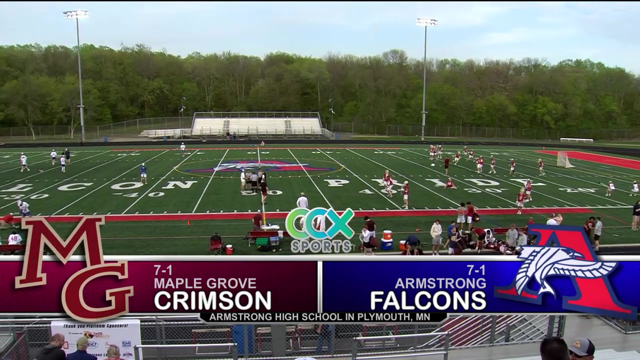 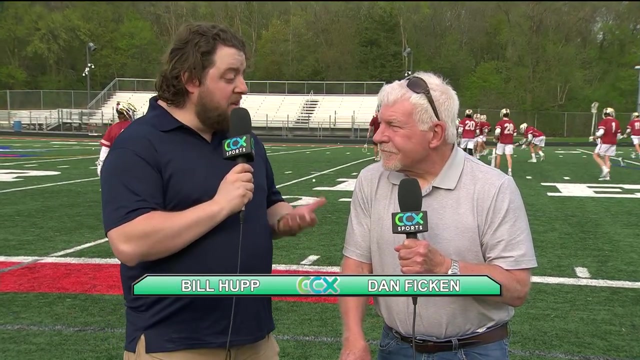 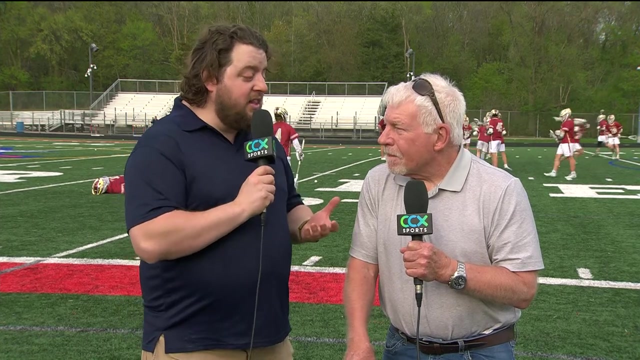 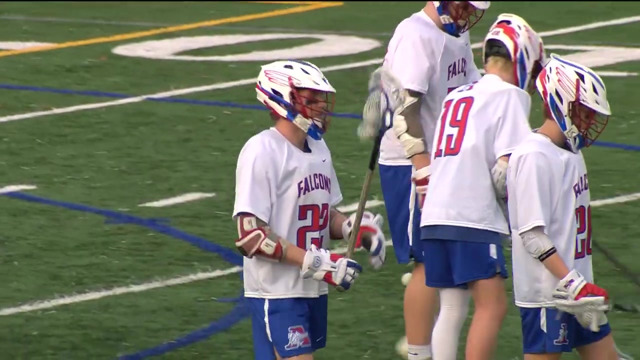 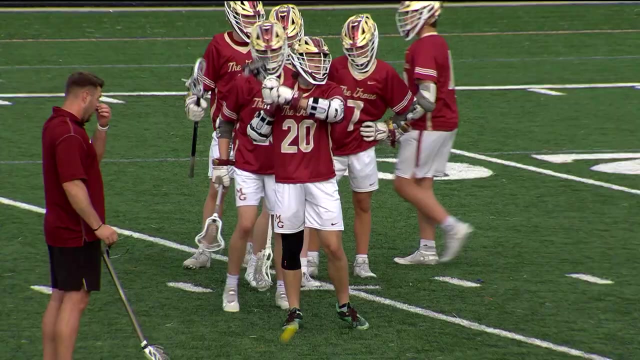 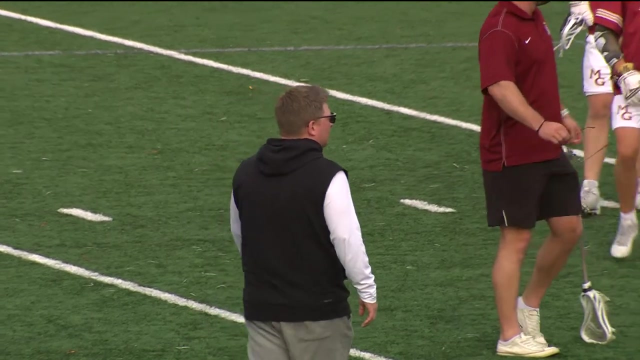 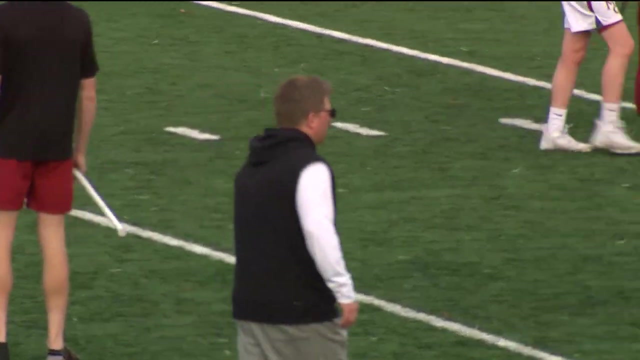 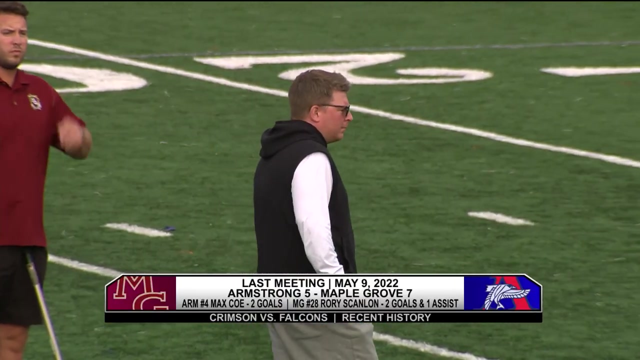 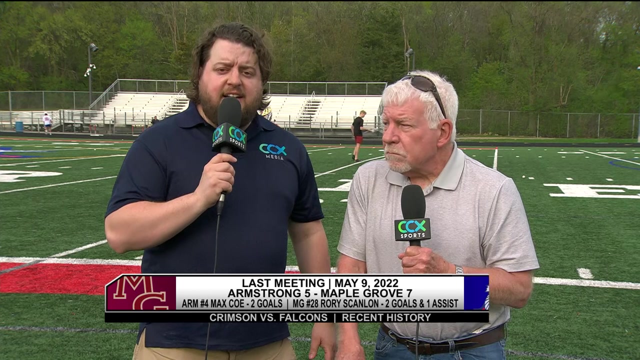 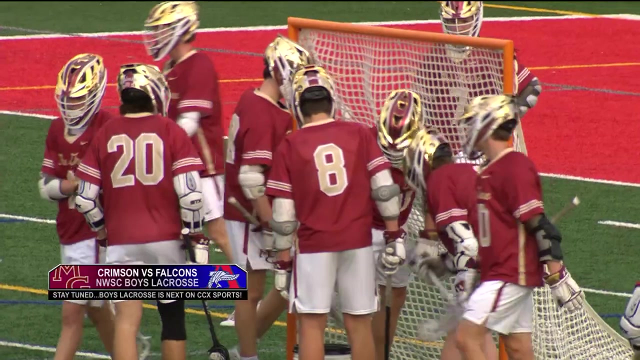 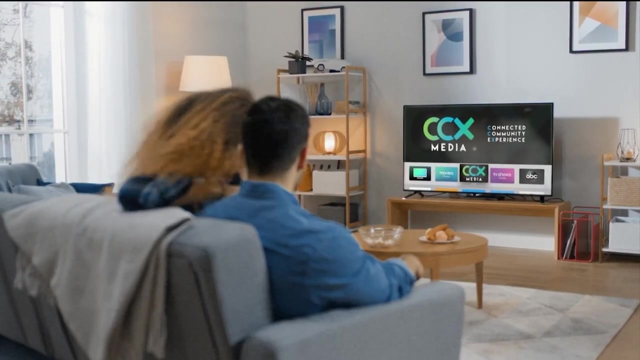 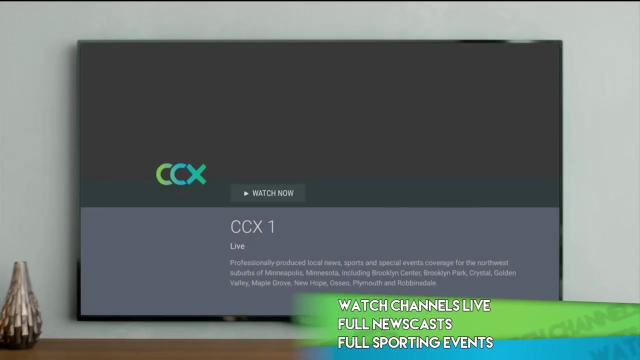 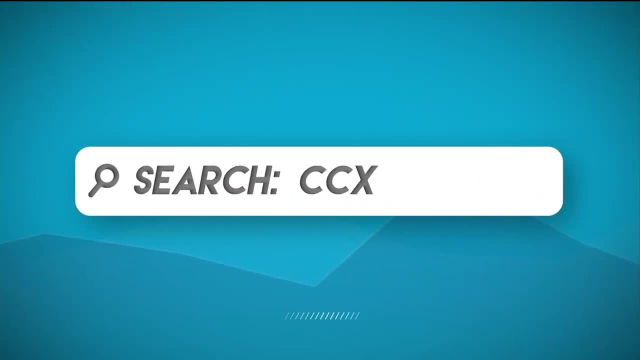 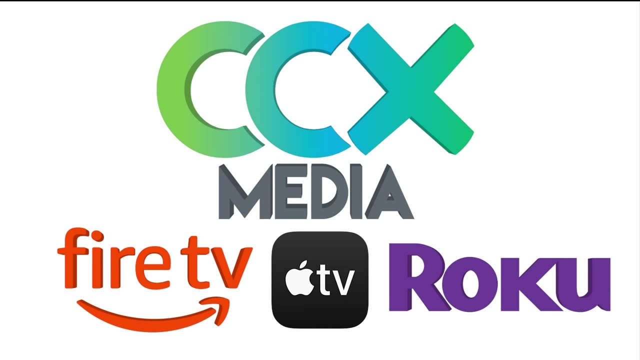 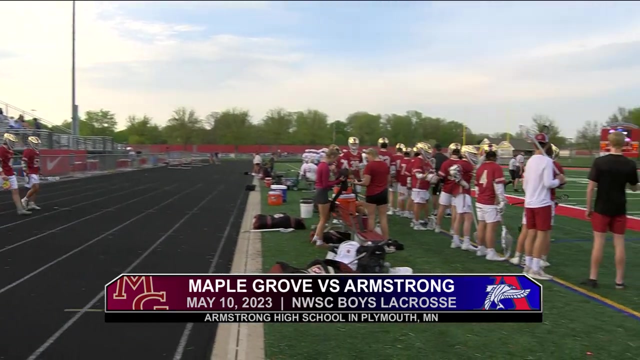 To find us, go to the store, search CCX and download our free app. Then sit back and enjoy all of your favorite local content: The CCX Media app available on Amazon, Fire TV, Apple TV and Roku. Back here at the Falcon's Nest at Armstrong High School. 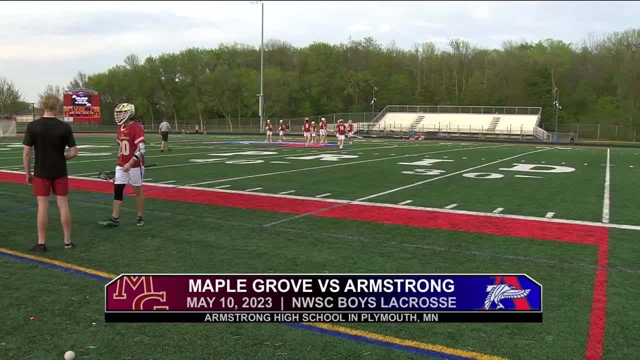 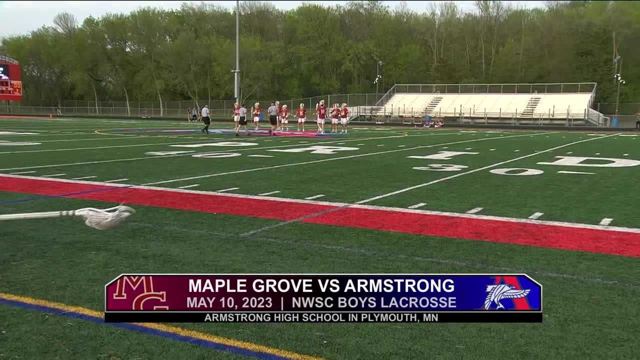 in Plymouth for a fifth-ranked. Maple Grove versus Robbinsdale-Armstrong clash The two top teams in the Northwest Suburban Conference. two of the four undefeated teams in Section 5.. As you take a look at the Northwest Suburban Conference standings, 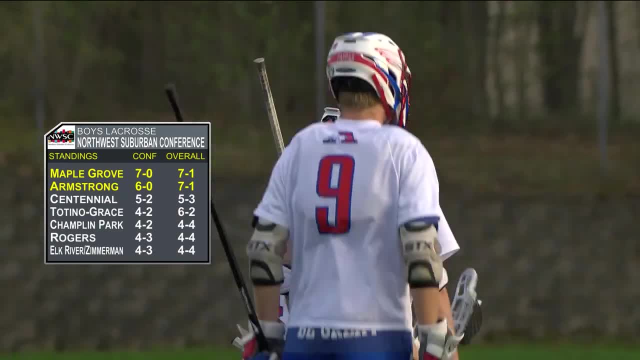 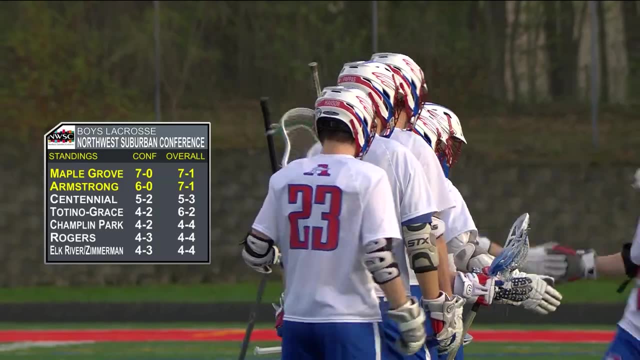 and right there. Armstrong has won just one less game than Maple Grove, but both teams sporting impressive 7-1 records. And, as I bring in my broadcast partner, Dan Fickin, Dan, this sets up to be a really important game. 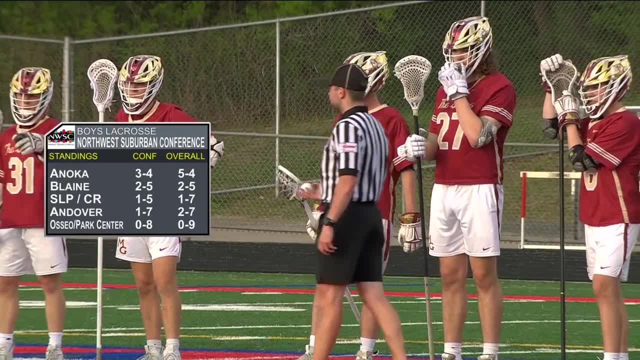 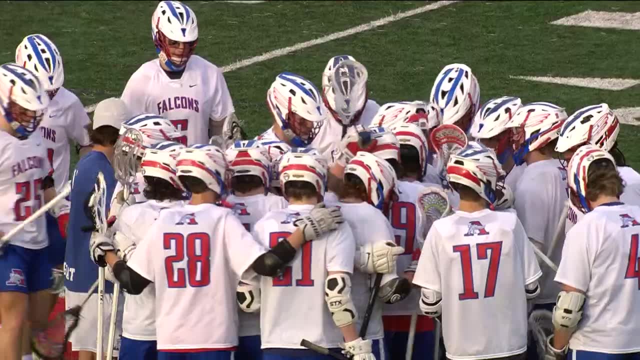 And a really good battle between two teams that are very familiar with each other. Well, you're talking to both coaches and also some of the players and stuff. It's like they haven't played a game like this all year. I mean, this is something new for them, both of them. 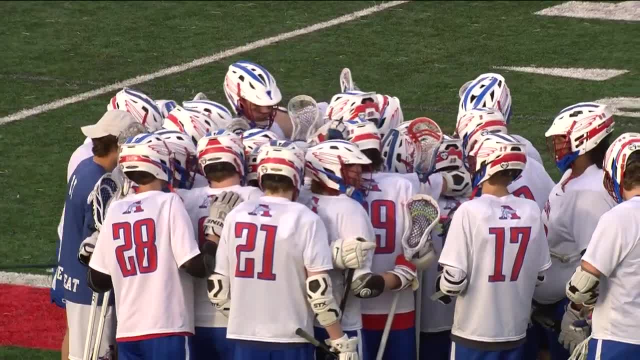 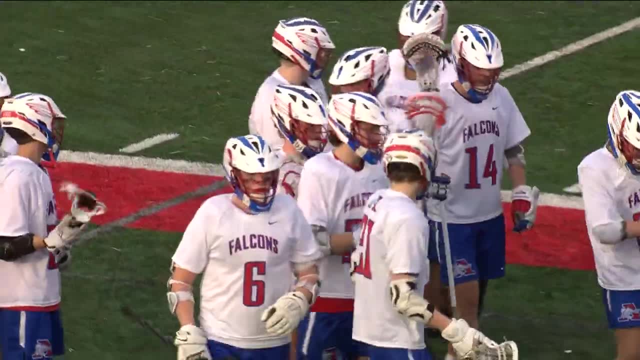 And they're wondering how they're going to stand up to it, And we'll see who pulls out when it gets tough. They're both very good, move the ball extremely well. We're going to see a lot of offense tonight. Yep, it certainly seems that way. 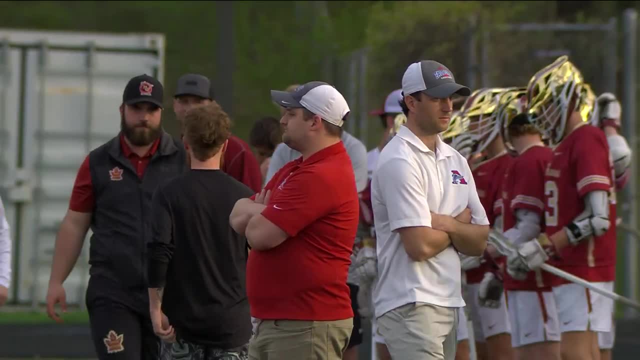 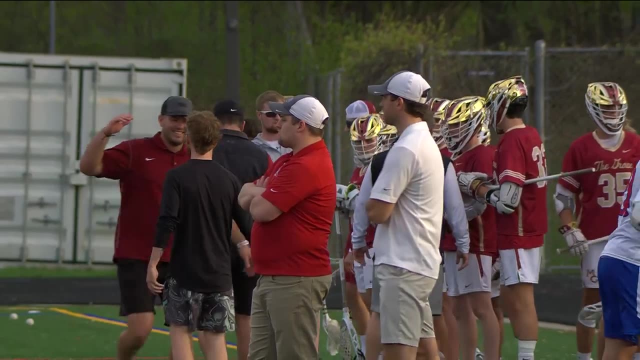 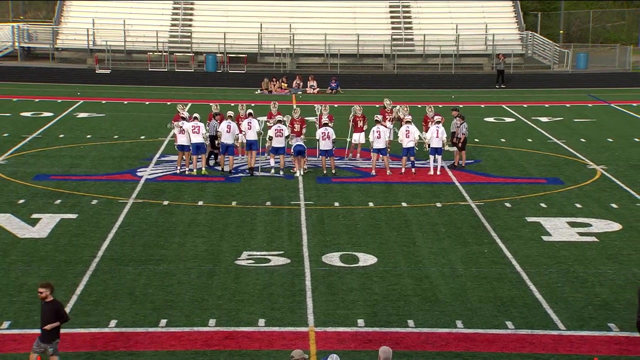 Maple Grove, averaging 12.88 goals per game. As you take a look at their coaching staff, led by first-year head coach Kyle Fickin, who came over from Rogers after eight seasons in charge of the Royals, And, on the other side, Ian Murphy, in his third season as head coach of the Falcons, 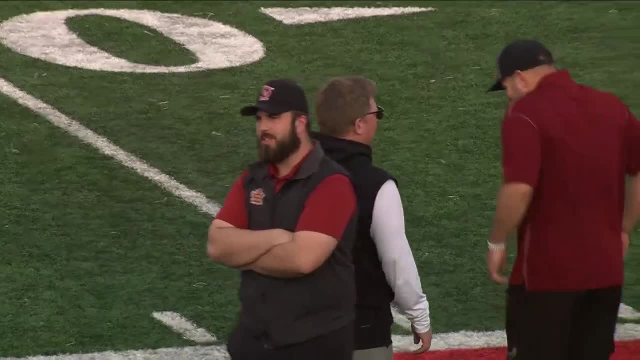 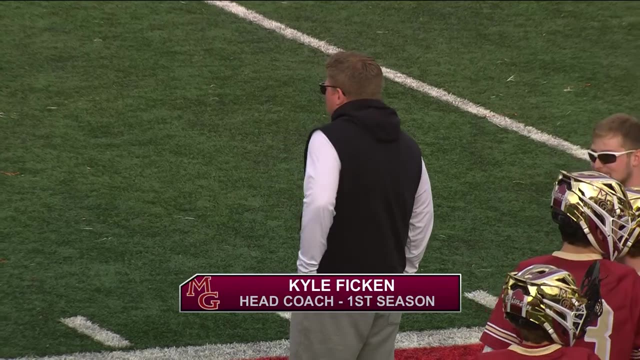 but all ninth season overall with the program as the two teams, As you take a look at Kyle Fickin And yes, in case you're wondering, Yes, The son of Dan Fickin in our broadcast booth, Dale Farniak and Xavier. 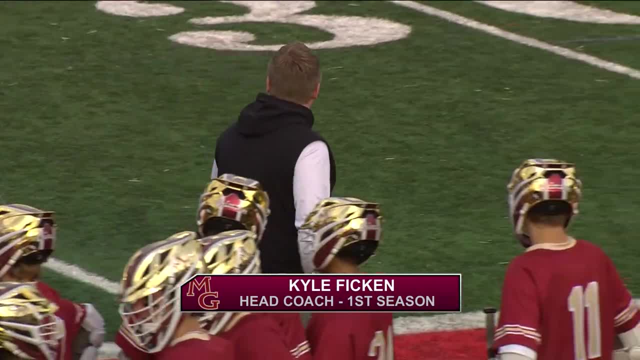 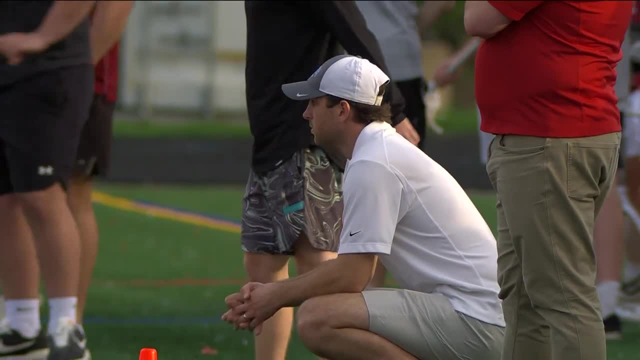 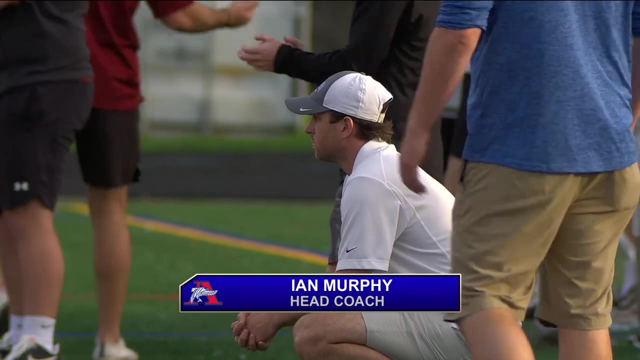 Xavier Wells touch gloves and go to their respective ends as Maple Grove in those sweet chrome helmets, the new maroon and gold uniforms As you take a look at Ian Murphy And both teams talked about the need for controlling, Both coaches talked about the need for controlling emotions in this game. 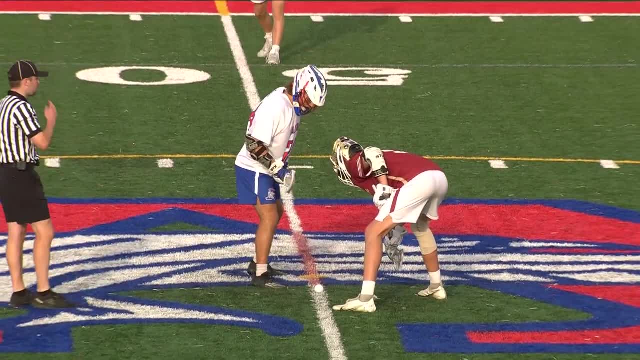 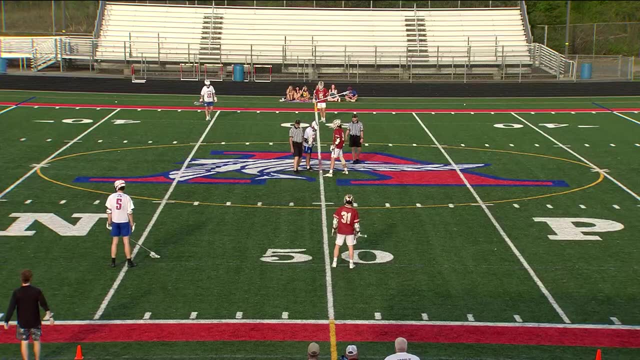 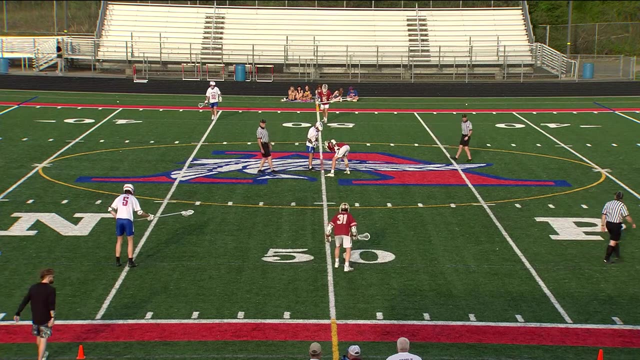 So we'll see how that goes for each team, as it'll be Tristan Mack and Shea House doing Battle right at the A. to start things off, House is 46.4% on the season and Tristan Mack 45% face-off. Yeah, but overall the Falcons have done very well. 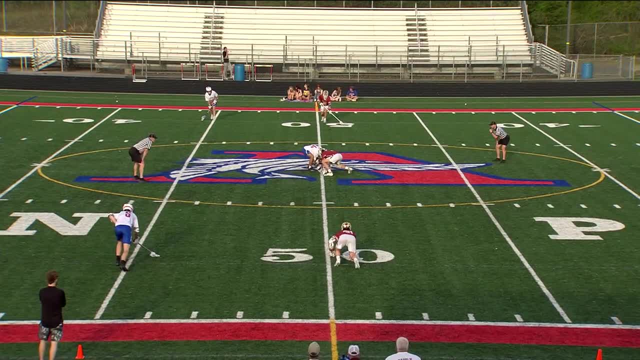 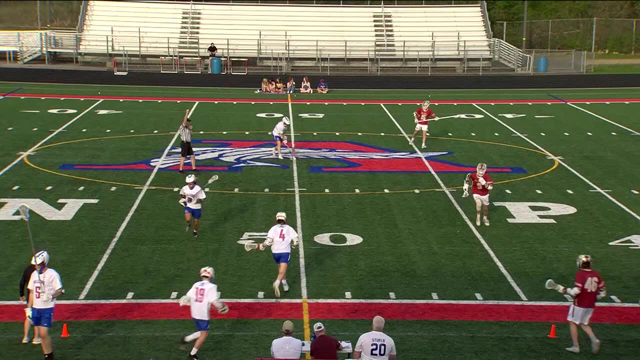 They've won 60% of their face-off wins And this will be critical here. Whoever gets that controls the ball and is ever controlling the ball, And it's awarded to Armstrong. False start on Armstrong. It's a beautiful night for lacrosse here in Plymouth 77.. 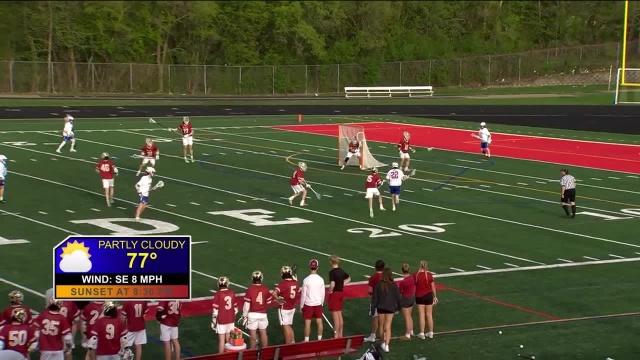 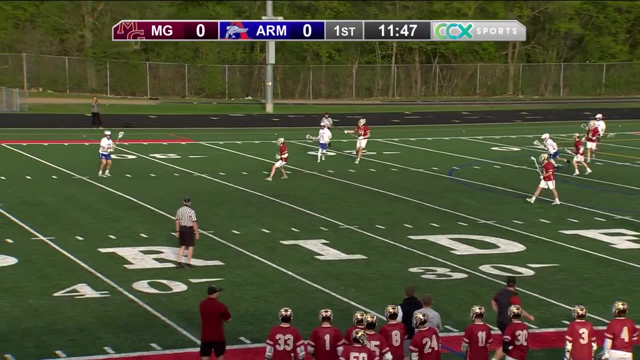 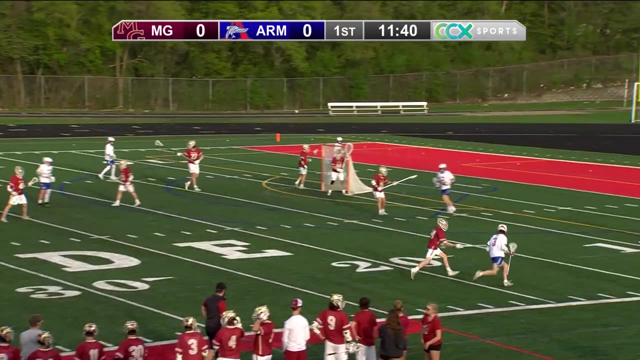 Wind out of the southeast at eight miles per hour. Lights on, but have not really taken full effect just yet, as we are underway with Jamison Essent bringing in deep. And then they get it out for Max Coe, the senior midfielder. Near side, Jack Olsen, freshman: 20 goals and 13 assists. 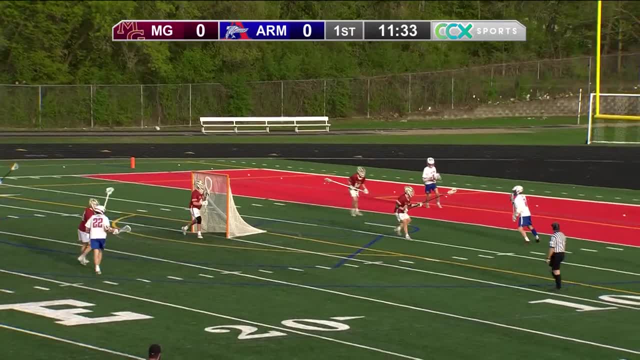 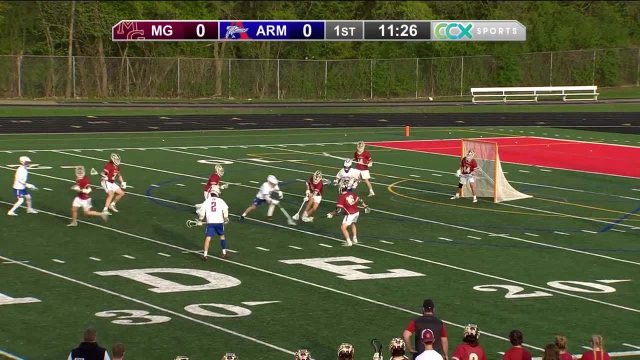 1-2-3, that's the numbers of all of their attackmen And the main one, Nate Albrecht, has it right here, Albrecht, leading scorer last year with 40 points, And he's got. 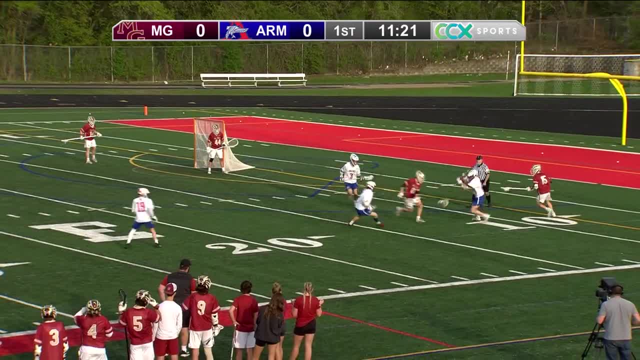 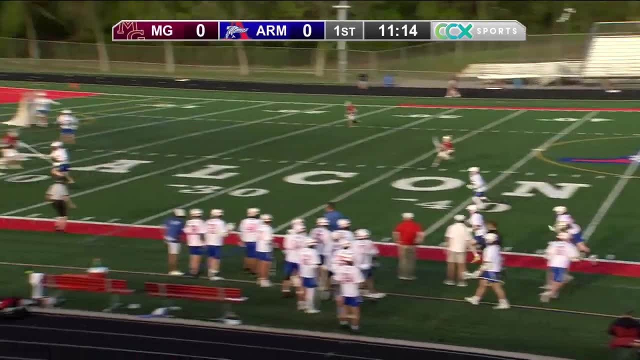 24 goals and 17 assists already this year. As the turnover is forced initially And then it's scooped up by Lucas Bakke, Maple Grove, trying to clear, And they manage to get it up and get it ahead. Good pass across. 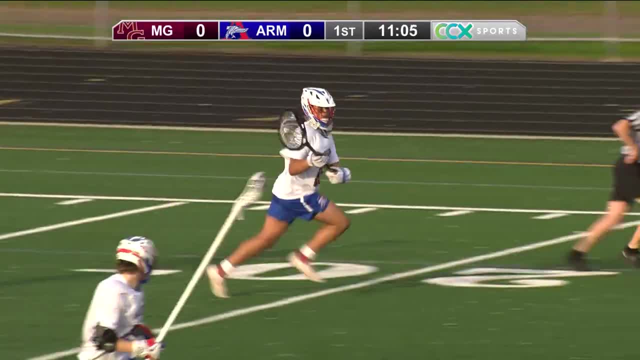 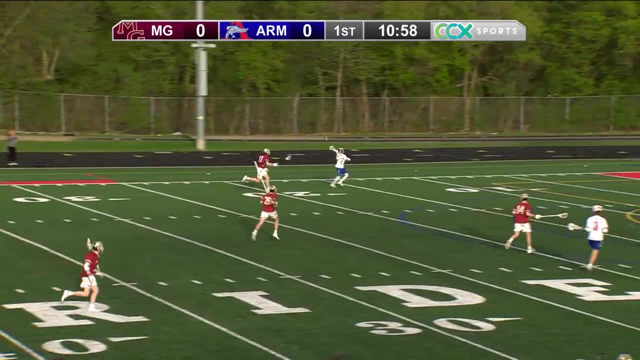 Ducking inside. Big save made by Wells- Whoa Incredible save made by Xavier Wells to stone the attack of Maple Grove And Rory Scanlon who was going for his 25th Half of the season. That was an amazing save. 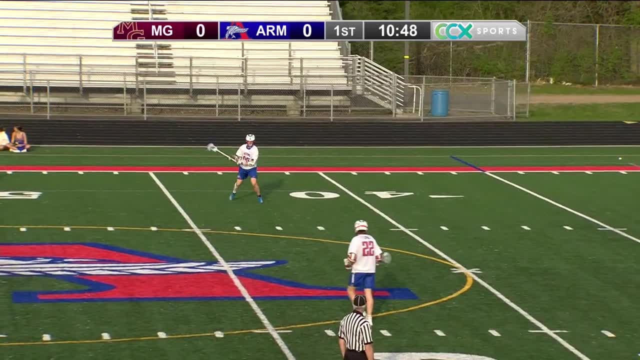 We'll have to see that again. That's Rory Scanlon who's just been lighting it up lately for the Crimson. Just a brilliant save. He attacked, He got aggressive And that's what you've got to be as a lacrosse goalie. 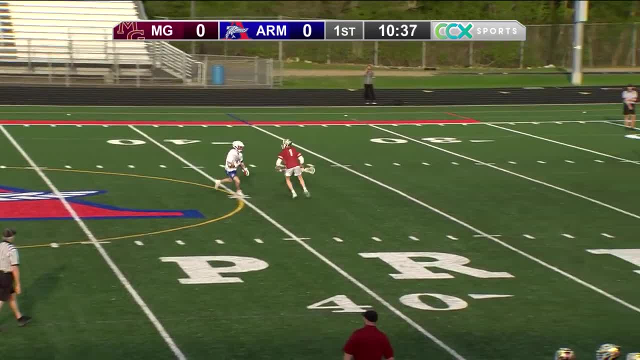 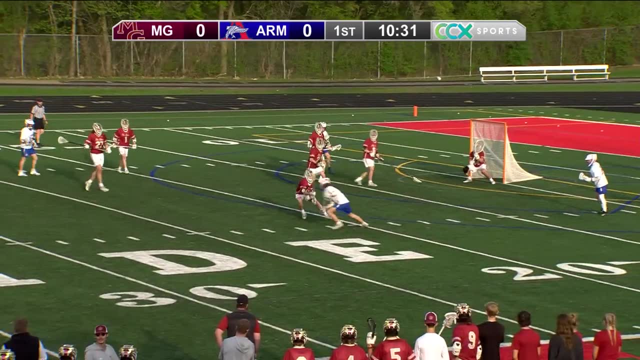 Absolutely incredible to start And we thought it would be a game of high-level players And so far that's proven correct. As Essent gets it Opportunity here, Jack Olsen going down low, And we've got to push with. We've got to push with. 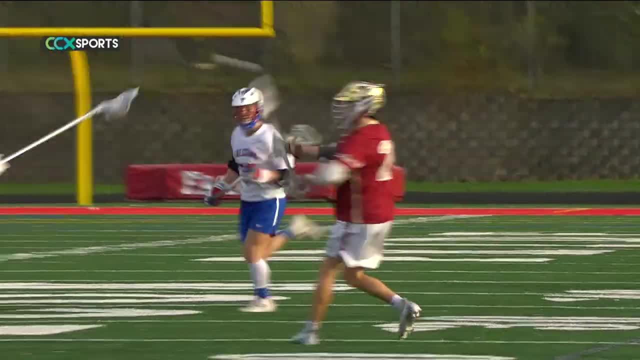 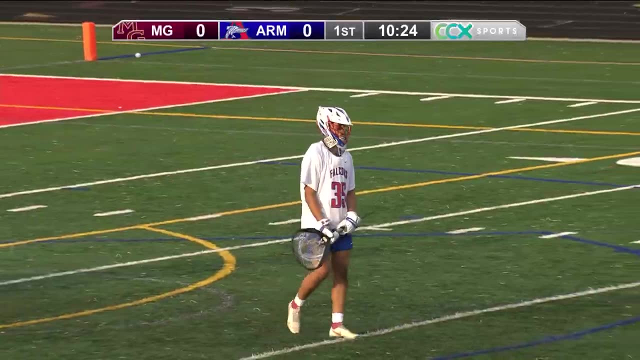 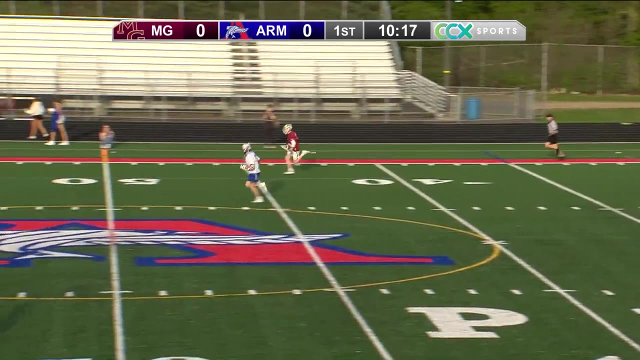 Front behind as we take a look at this save. You see Scanlon actually fed it across And it was number 20, Ricky Peterson going for goal number 31.. And so Xavier Wells with an incredible save. Wells going to Division II, Mars Hill in North Carolina. 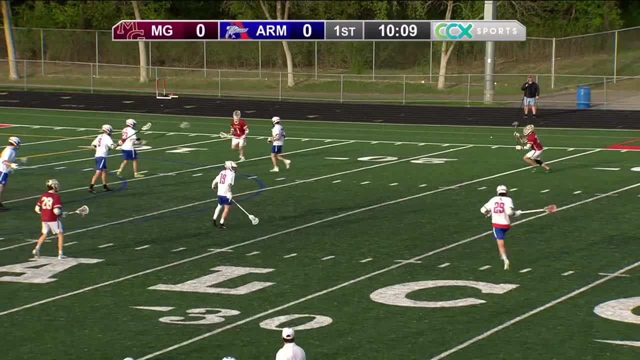 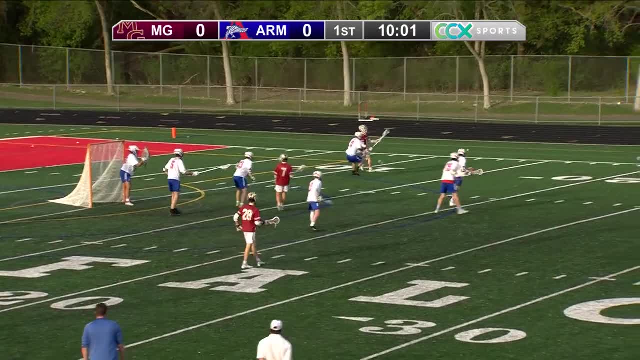 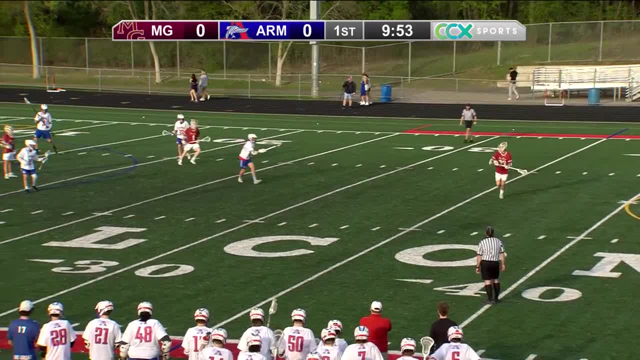 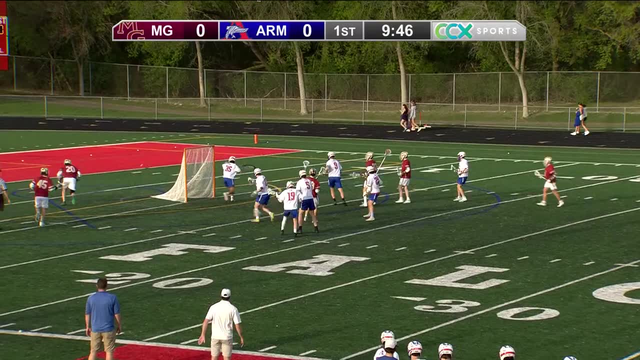 Going to Quincy next year. So a lot of college talent on this field. Of course. Maple Grove- still pretty young as a team. Ricky Peterson- just a sophomore Opportunity here. That's Scanlon, who tried to pick out the upper corner. He's going to Springfield. 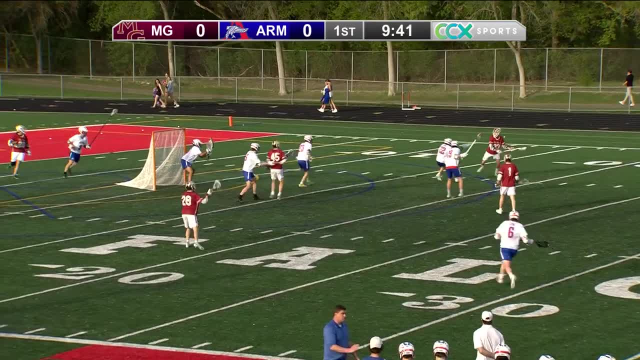 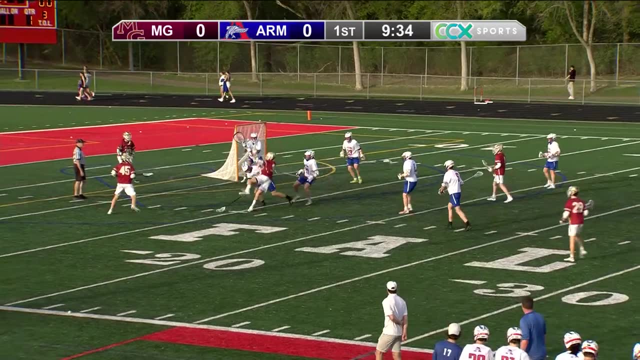 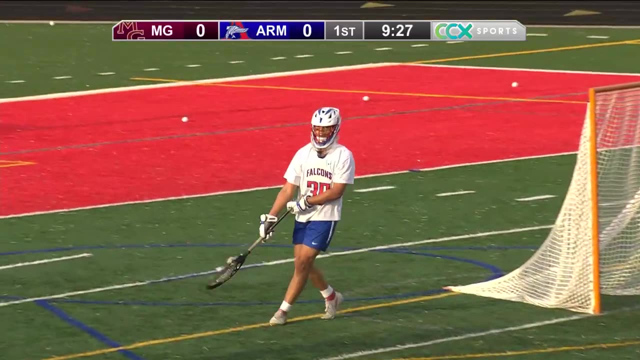 Division III powerhouse As Maple Grove controls Scanlon. It's a cutter Big check delivered by Pappas. He popped him And Wells rakes it into his crease. Very good defense for the Falcons. They let that one slip through their goal. 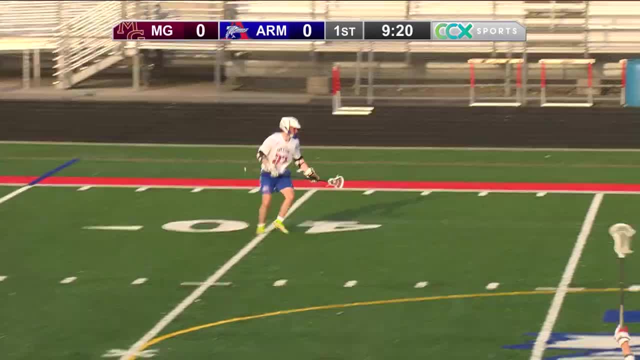 He saved it on that, And the rest of them picked it up now and playing good defense. They've got to control the ball, though We both know that That's going to be here. Both teams can score, And who's ever got it the most is going to score more. 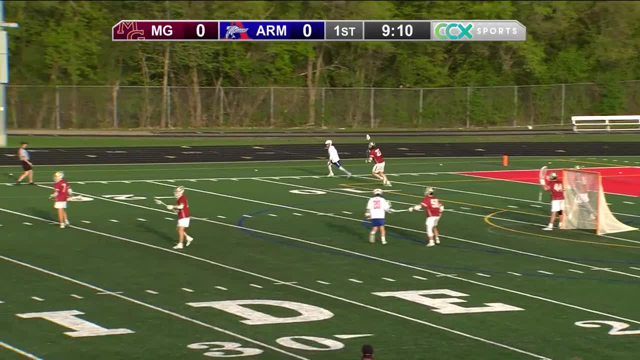 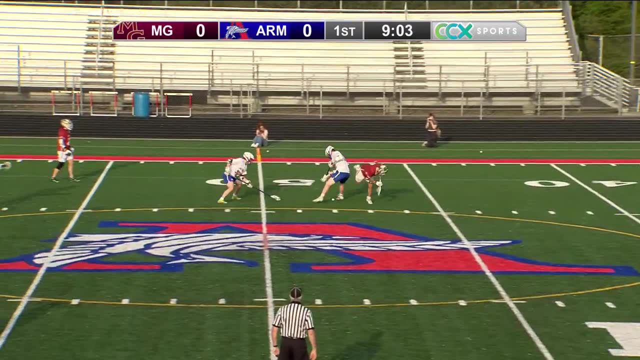 Riley Hansen Helped get it across for Armstrong. As Frankie Annis gets a touch- 19 goals, 6 assists for him- He tries to roll it back to his teammate, Big number 50, Logan Marsh Marsh recovers. 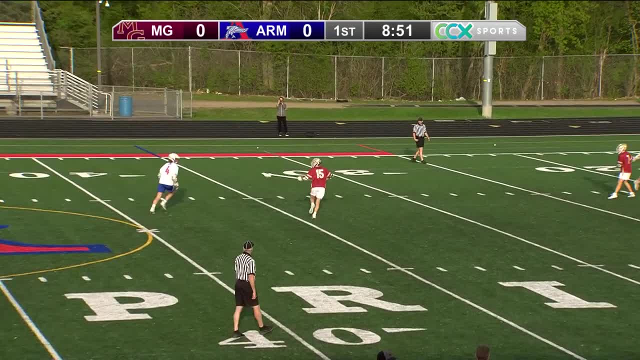 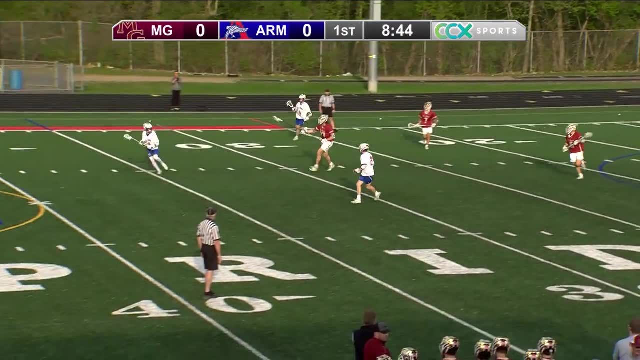 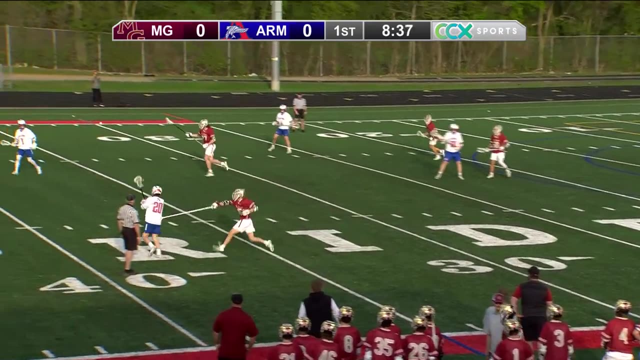 That was a solid hit too. He ran into him. He just bounced off Marsh 8.50 to go First quarter Still scoreless between Maple Grove and Robbinsdale Armstrong Annis having a little tough time throwing it. Sometimes the stick can play tricks on you. 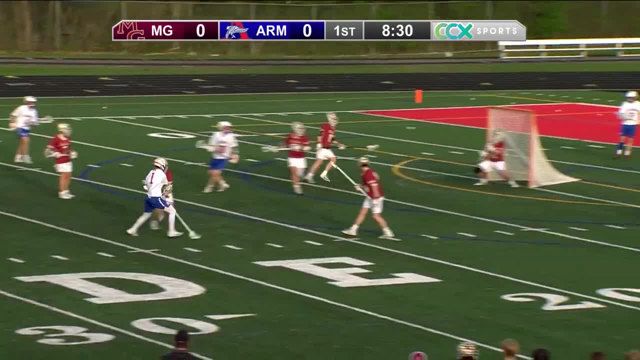 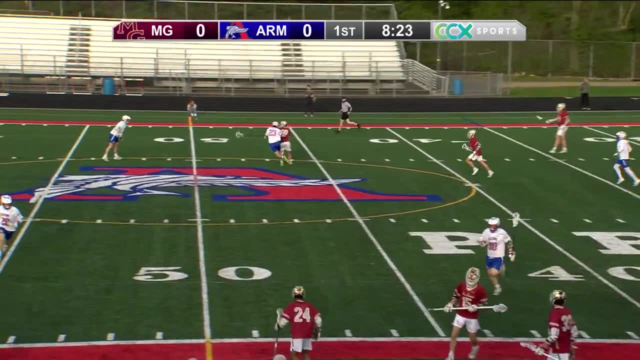 Look at the defense Way out there by Jackson Bennett. the sophomore Annis gets a step, Fires right into the big catcher's mitt, the big butterfly net. That's the word I was looking for of Hank Farniak. 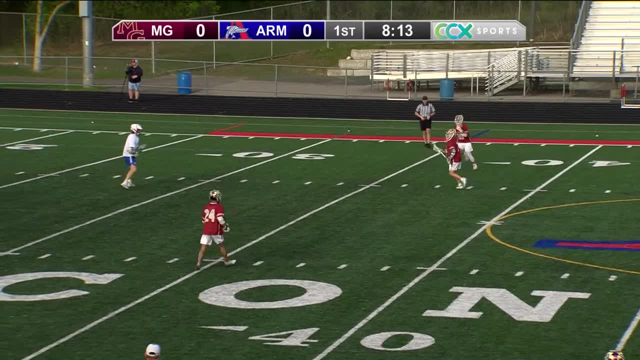 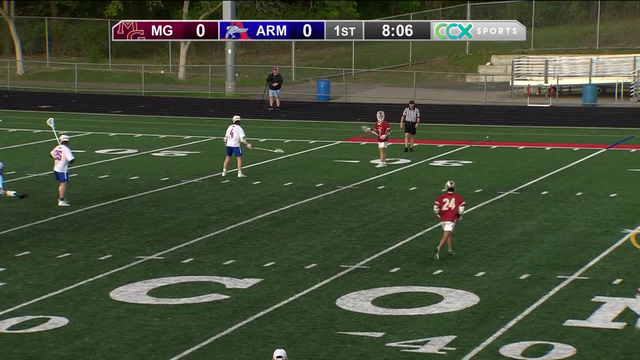 Farniak on the season 6-1.. A 6-1,, 8.81 goals against the Falcons, Average in a 5.93 save percentage And a goal scored. Yes, and a goal scored, Which is really unusual. 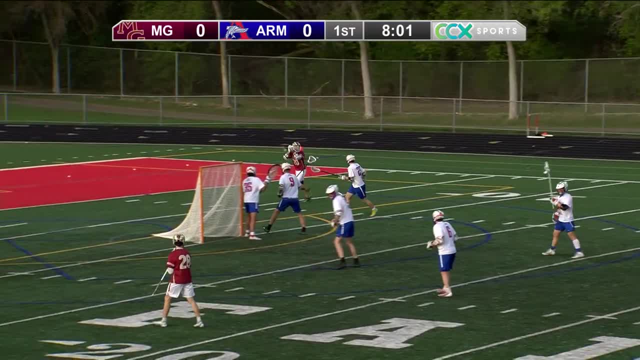 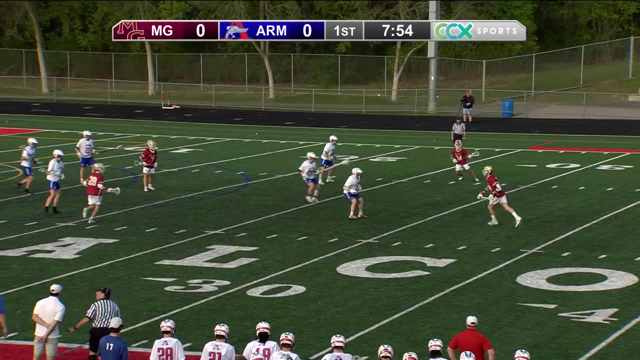 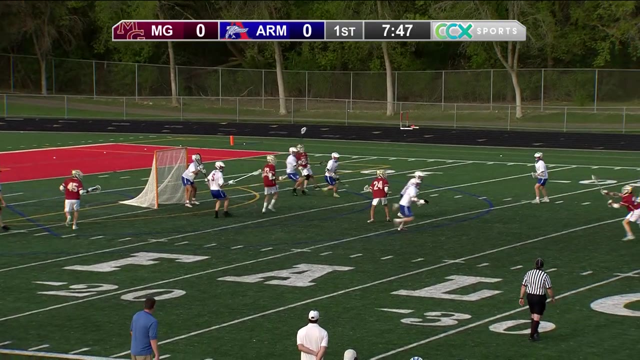 Not something you often see. Yes, Josh Thompson gets it for Peterson. Now Maple Grove tries to strike first Scanlon Up top, attacking downhill. Worked behind for Peterson from X Out high looking for Scanlon and he drops it. 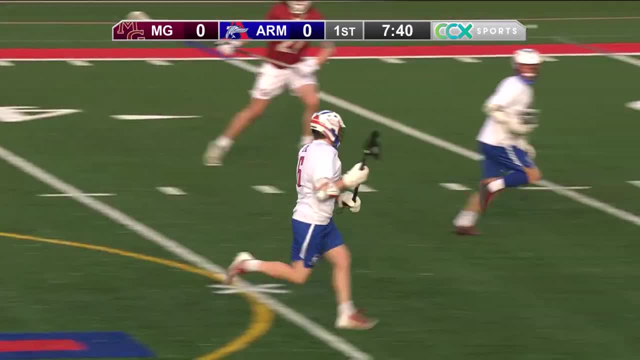 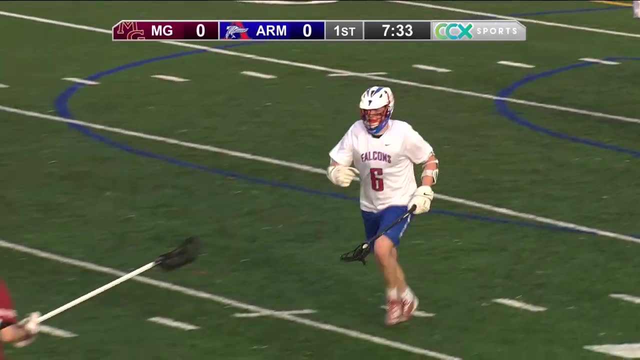 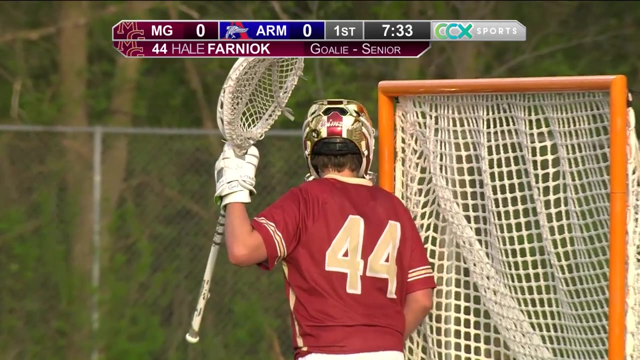 Opportunity is jacked. Bailey scoops it up, Bailey cradling, No one's going to stop him, or no one has stopped him. Finally, a last-minute intervention, But Armstrong backing up. well, and they have taken over possession. 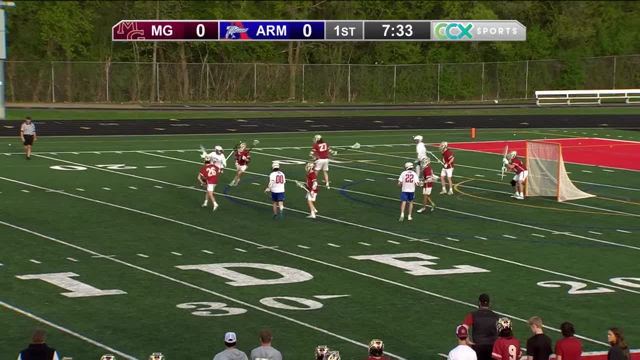 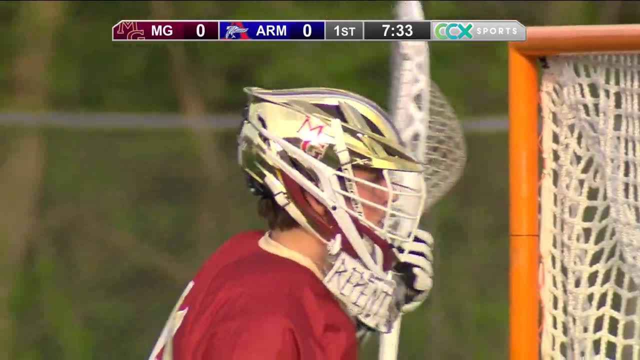 Farniak, a senior goalie who in the game last year made 14 saves and a 7-5 win. That shot goes whistling wide and it will remain with Robbinsdale-Armstrong. Farniak's done a good job this year. 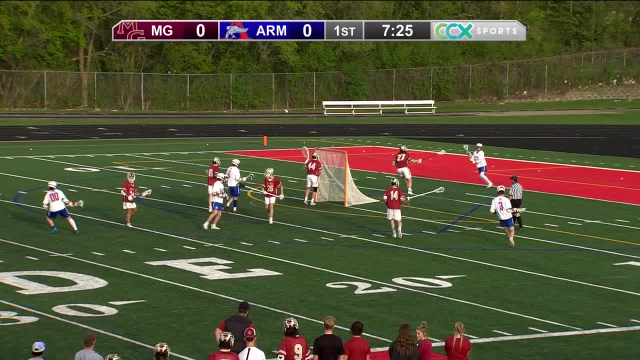 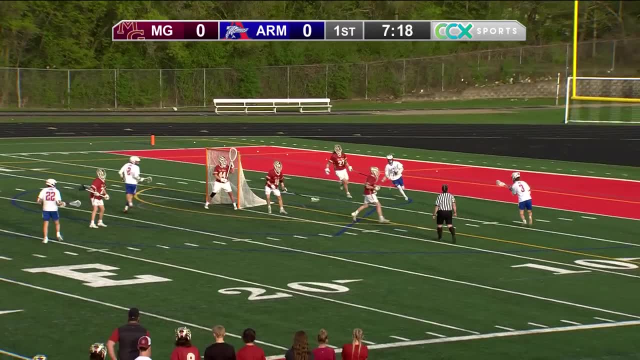 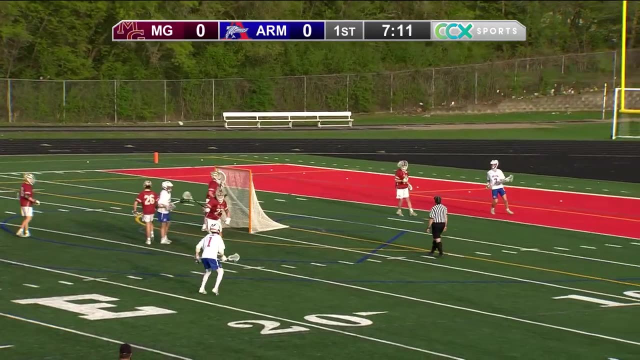 He's got a 6.81 save percentage, which is pretty good for lacrosse. Usually it's a 500 or a little below. Yeah, he is definitely a good presence in there. Wouldn't be surprised to see him play at the next level. 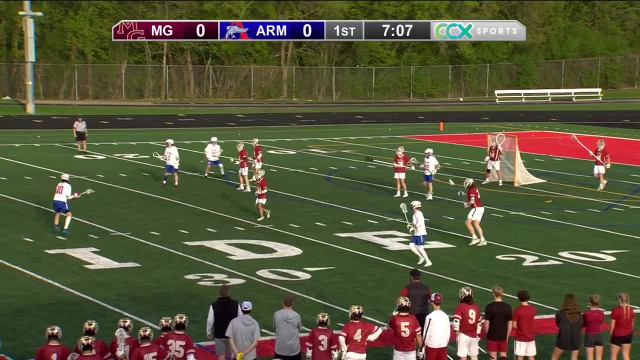 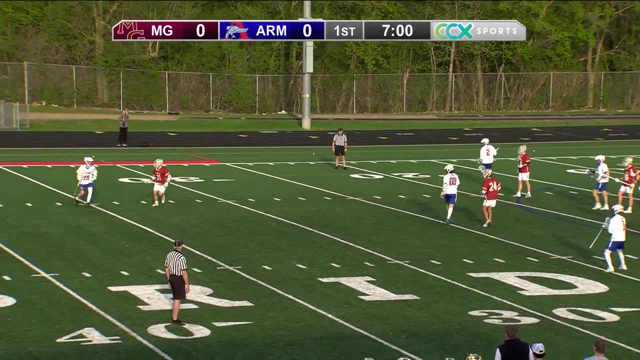 A flag is down, so we'll have our first EMO And it should go the way of the Falcons. That's Sam Cassidy. double zero Back in the game, Backs it out Maple Grove with the short stick, watching Brady Northrup. 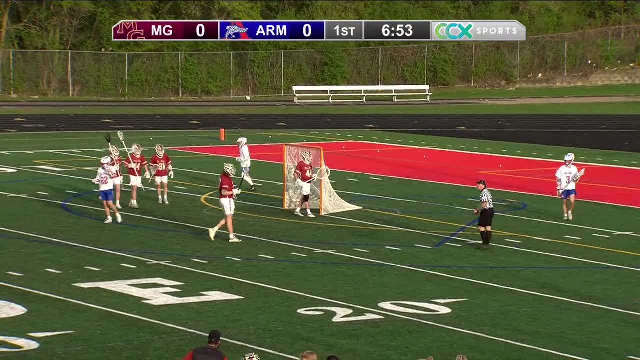 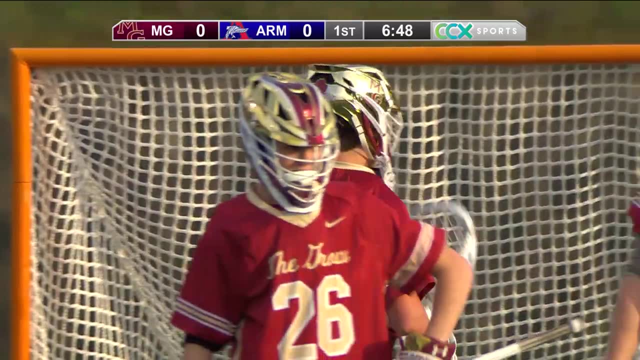 Northrup splits defenders, gets free Bounce shot goes wide, Farniak may have gotten a touch And now the penalty will be called: It's like a slash Yep. Joey Eisler, the Carthage-bound senior. 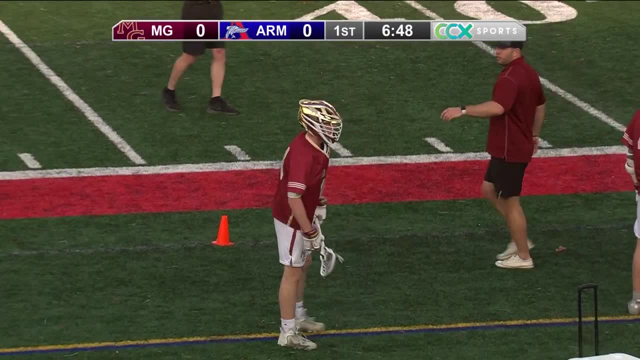 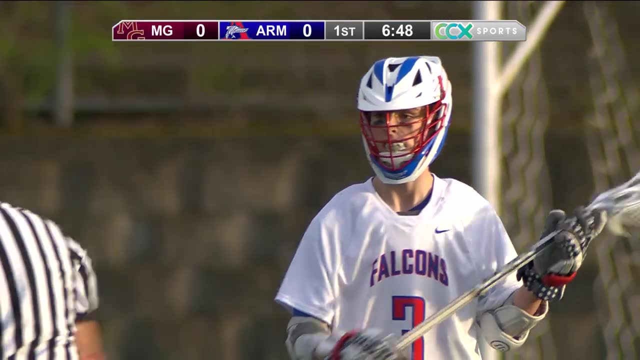 You know, it's kind of nice to see it on too, with all these kids now getting an opportunity to go to play- And the East you know where. lacrosse is a huge sport And we're developing talent enough to play in that environment. 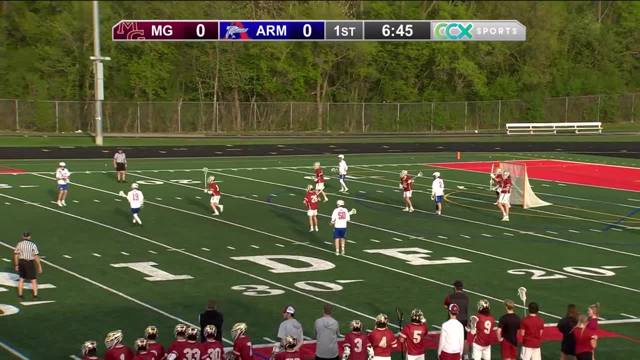 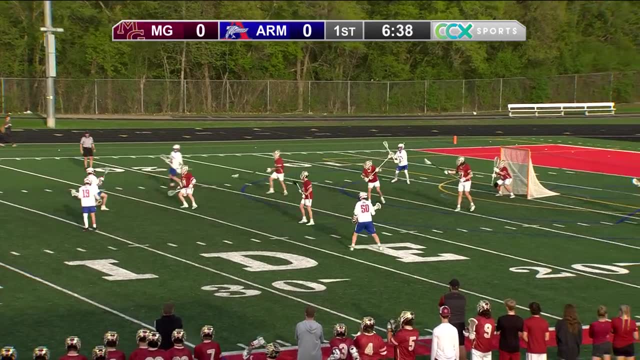 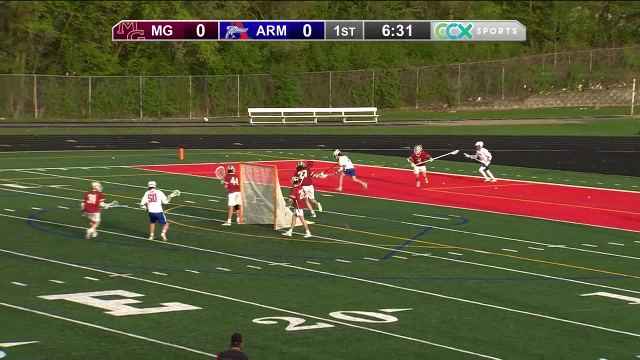 That's right. So the first penalty on a slashing penalty on Eisler gives the EMO to Robbinsdale Armstrong, And now they have an opportunity to get on the board first here at home. That pass errant Battle for the rock eventually won by Jack Olsen. 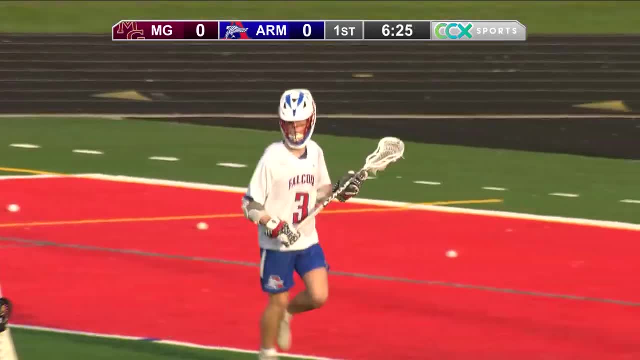 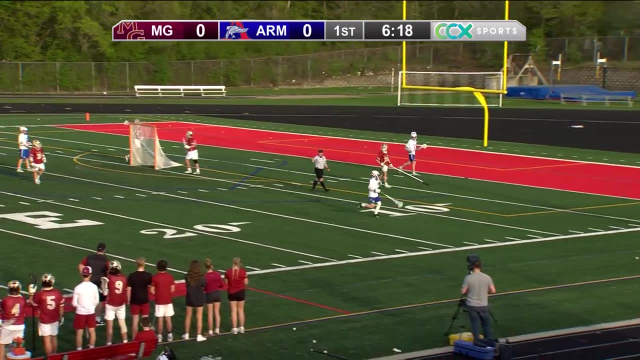 And Olsen And Olsen- And you see him up close, like right there. Does look like a freshman but obviously has some tremendous stick skills. There's a shot that's whistled wide. So Robbinsdale Armstrong has had the majority of the effort so far. 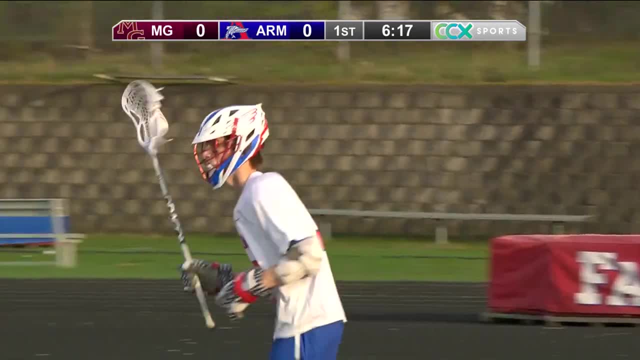 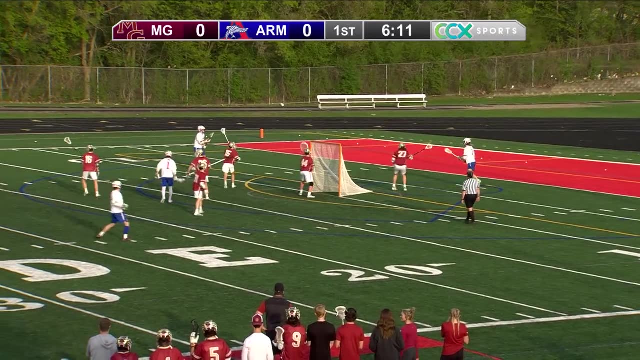 But none of the success, as we're still scoreless. Olsen will reenter play on the EMO, Like we said, you know both these teams are offensively oriented, But the one that plays the best defense is probably going to come out on top of this. 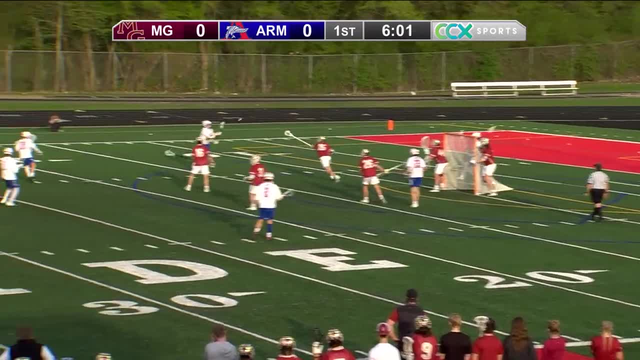 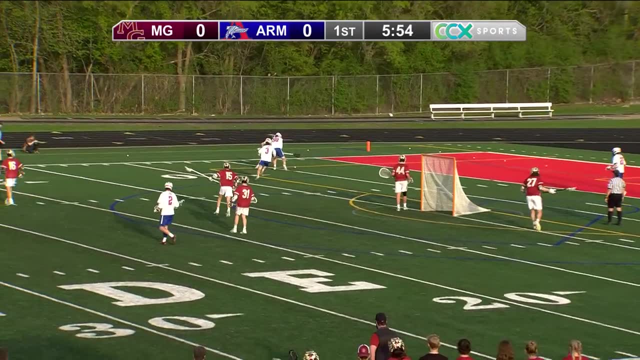 Because you know really, that's what wins these games. Yeah, very often A little give and go And Farniak makes the save That might have gone off the side netting- actually Hard to see from our vantage point. 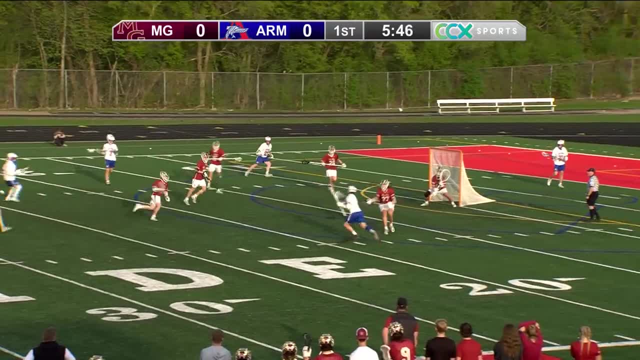 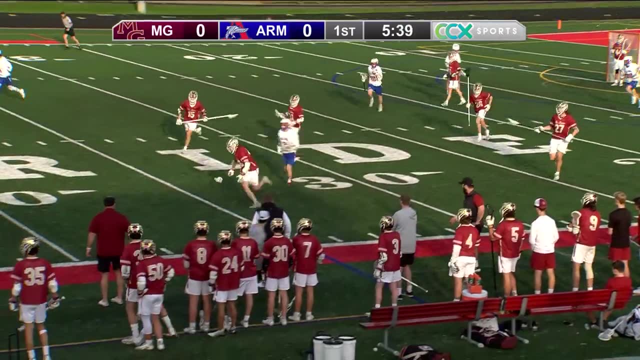 Battle for the ground ball eventually won by Olsen. They ping it around quickly. Albrecht ducks inside. Big save by Farniak. Boy used his helmet that time. He's using everything he can to get that ball out of it. 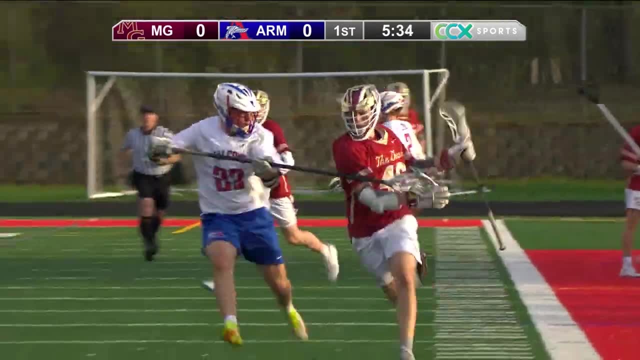 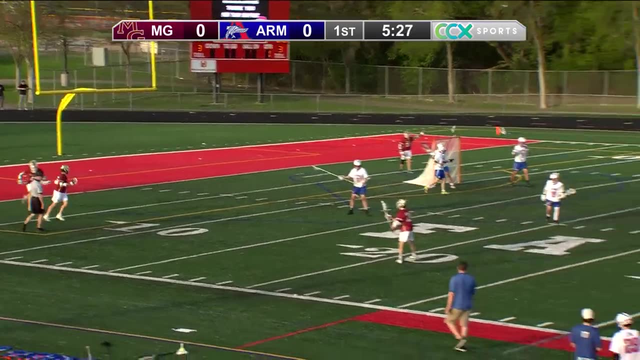 Boy. Maple Grove needed a break here, By God, Whatever. Whatever it takes, Each goalie has now made a tremendous save to keep this a scoreless affair, As the penalty is just about set to expire And it looks like has expired. 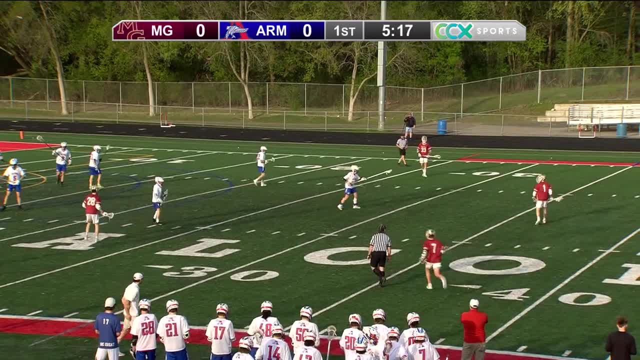 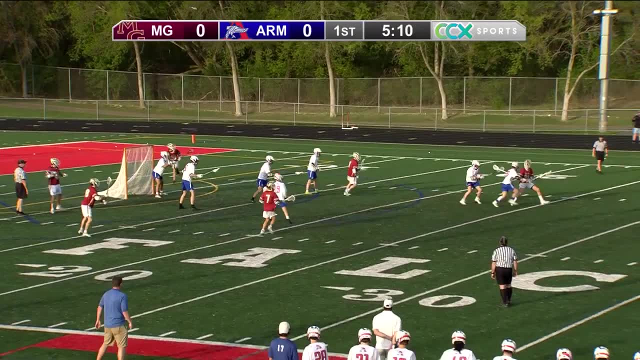 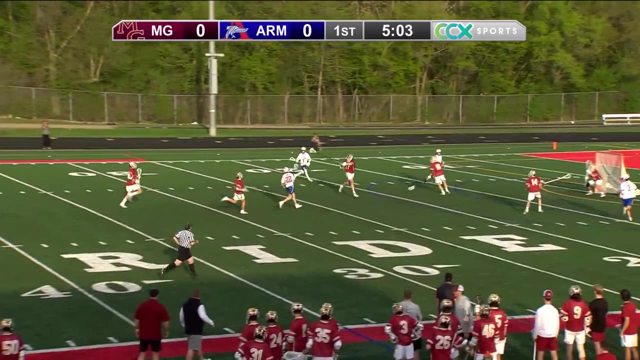 So Maple Grove kills off the first man advantage for Robbinsdale Armstrong, And now they'll go to work on the offensive end. Two highlights of the game have been tremendous saves, But great defense, again played by Robbinsdale Armstrong. And here come the Falcons in transition. 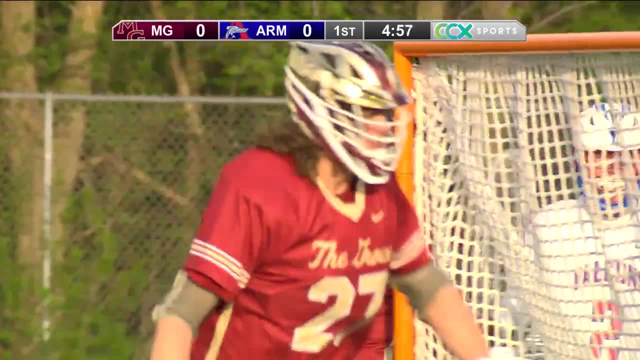 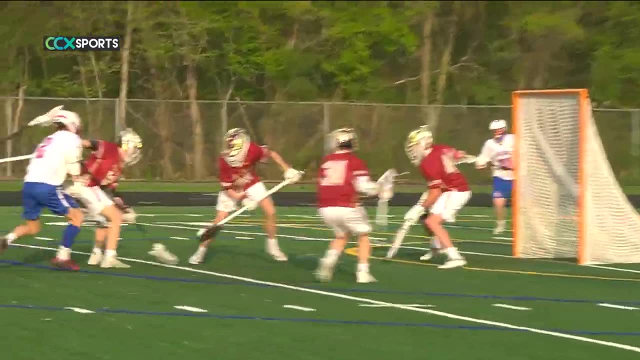 Now, on an errant pass, Flips it over its intended target And it'll go all the way. Oh, They say it was deflected, actually As Albrecht. you see the jump shot And just a tremendous save by Farniak. 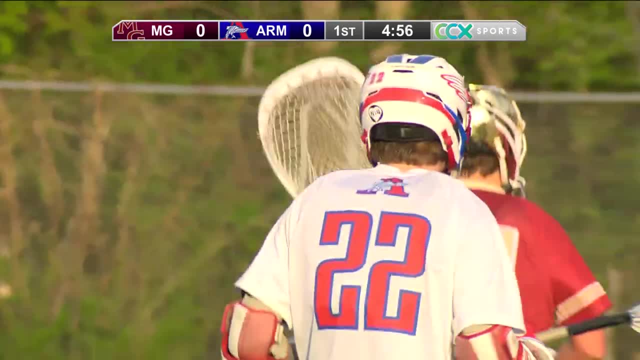 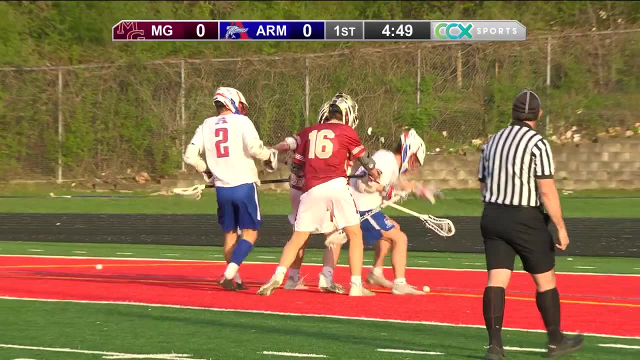 And the Maple Grove parents. I should say displeased with the call right there, But they're going to say the pass was deflected. That's why it remained with the Falcons- The ref right there saying that it was deflected. 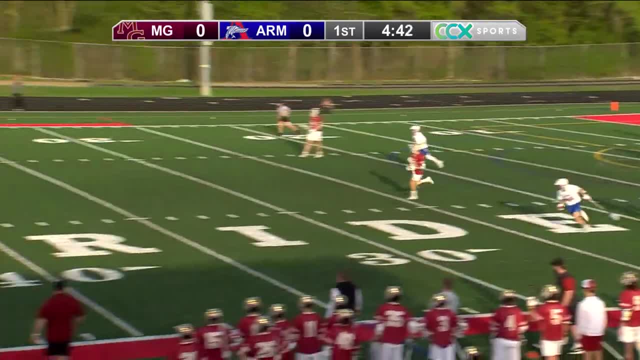 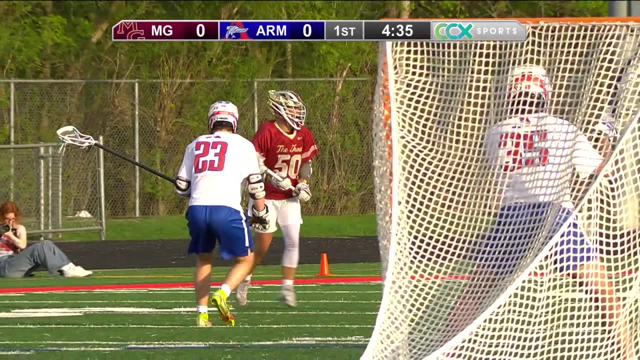 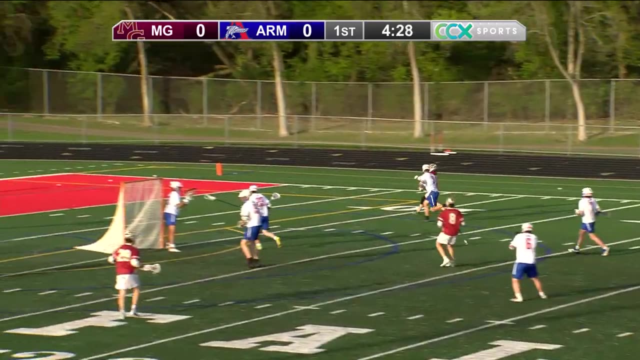 Good recovery here by Shane Rask, the junior defenseman. And now it's Maple Grove's turn to get out in transition. Logan Marsh gets a touch, And now he'll back it out And flip it for Tyler Steinkopf. Get it in the stick of Peterson. 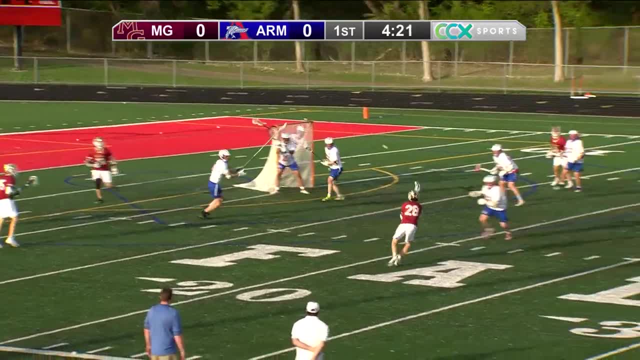 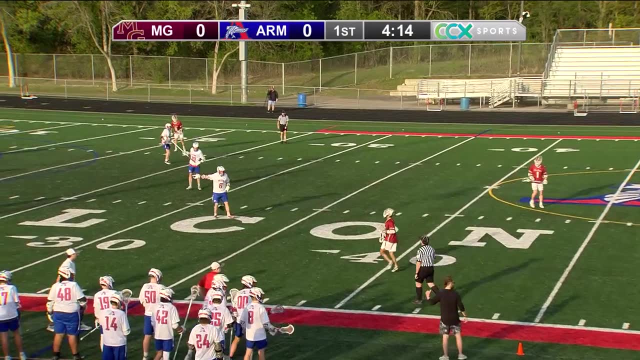 It's usually not a bad place for it to be- Not at all. Peterson out high looking for Scanlon Maple Grove, not taking as good a care of the ball as I think your son would like to see in the early going, But they have it here. 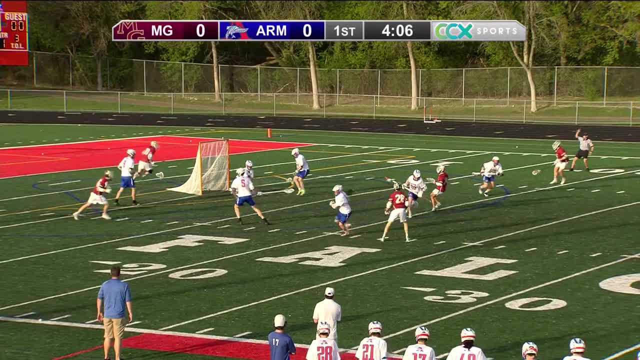 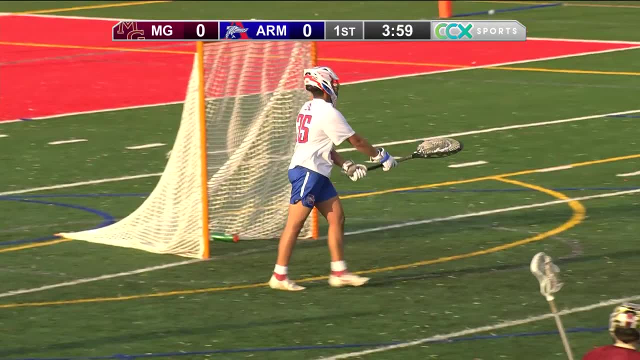 And Scanlon, no one's going to step to him, So he'll fire a shot. Another tremendous save made by Wells. Mr Wells determined that we are going to make this a game, a big game. And when you get defense like that, goaltending like that, 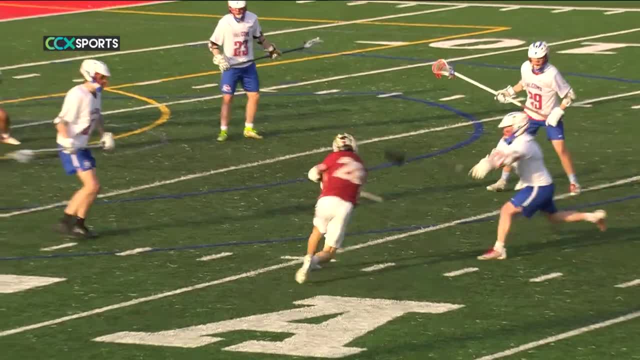 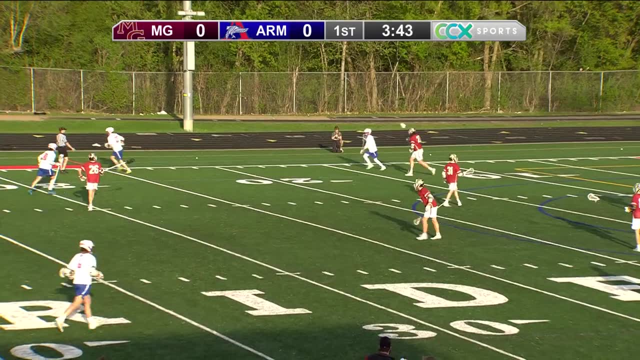 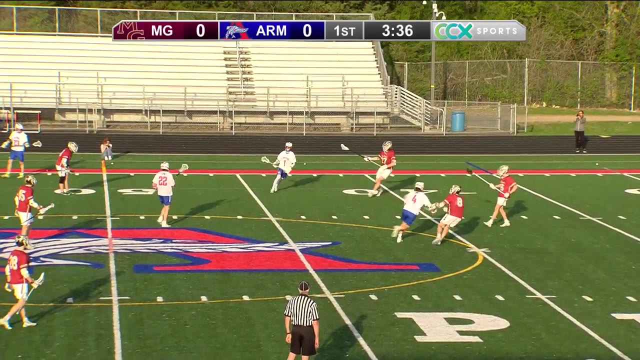 boy, it is nothing but fire up your team. It just gives them more than enough confidence. Oh my goodness, The saves so far by these netminders in the first quarter. Wells is not the biggest netminder either, but he is quick and certainly obviously an intelligent goaltender as well. 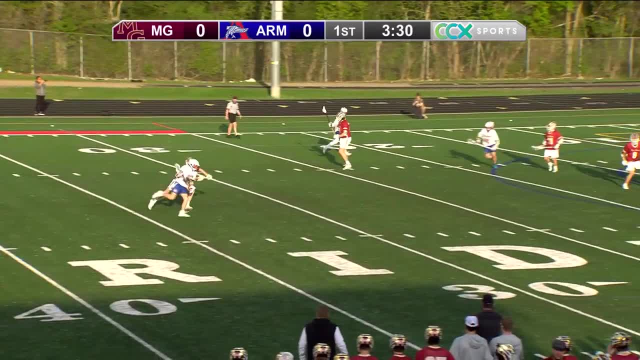 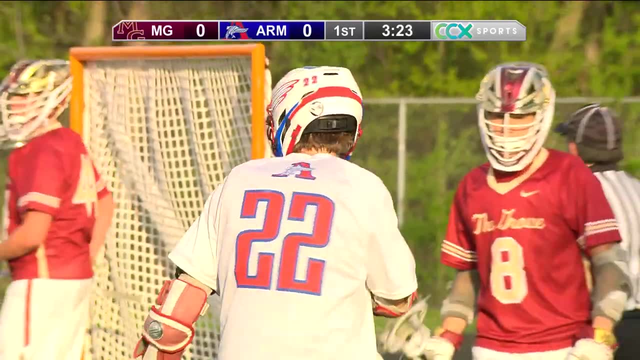 And so now it's back with the Falcons, And that's the thing is. each of these saves have led to a change in possession. Chance here, weaving his way through and scoring Jamison Essin- his 17th of the season- as he danced through the Crimson defense. 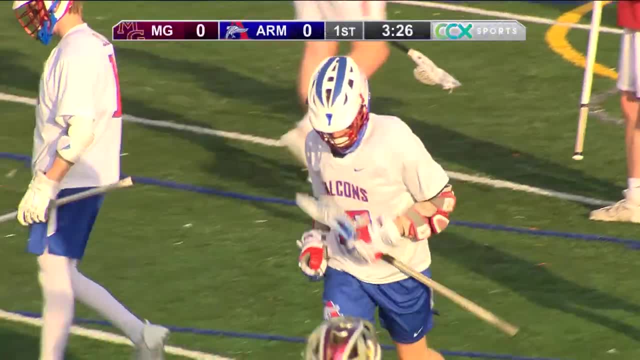 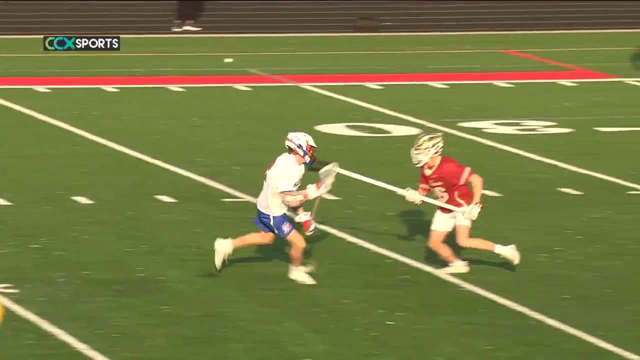 Boy, really, really nice moves here. Put on a little speed. He kind of changed the speed here and there to get by the D Got in tight and he put one down low. Just a nice shot in Nice move right here. 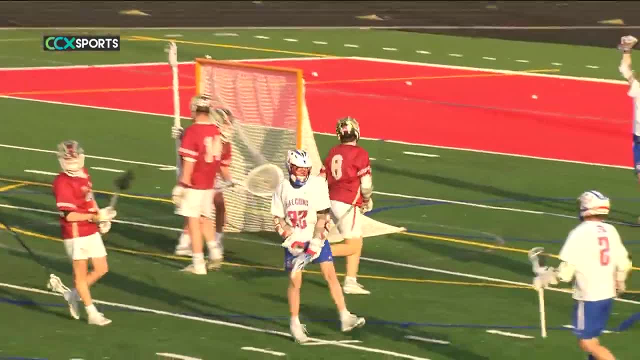 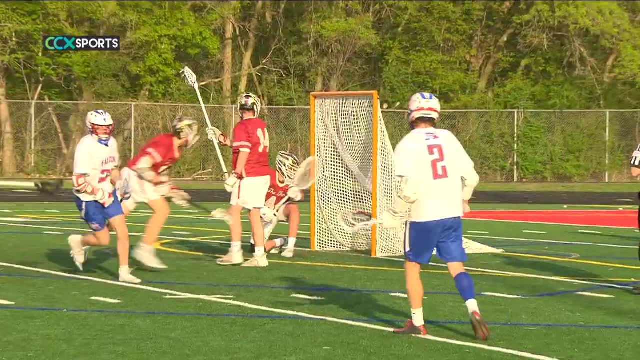 And that is why you hit the body and you don't go for the stick. Exactly, That's why coaches preach that all the time, Because, right there, everyone went for the stick and he just protected it. well, The ball was unassisted and it's 1-0 Falcons. 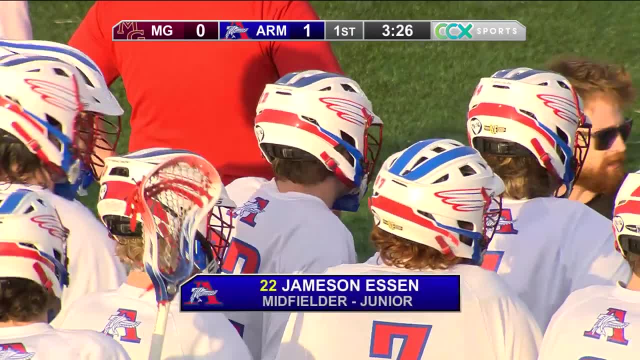 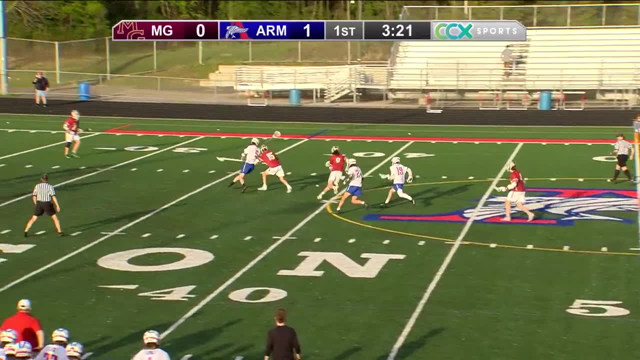 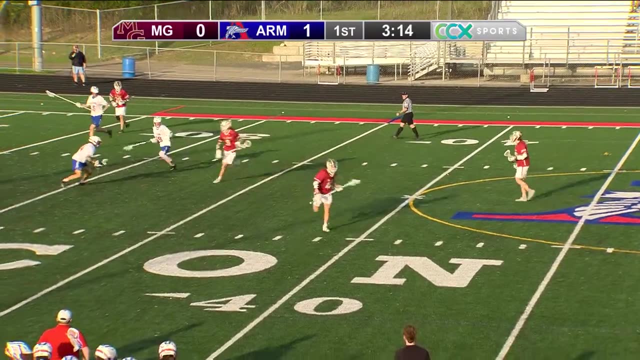 He never switched hands on that. He kept it all in the shooting side. Jamison Essin, the junior midfielder- It's a really impressive move- Leads the team in ground balls as a penalty flag flies. And it'll be the first EMO here, as once again, Shea House wins the draw. 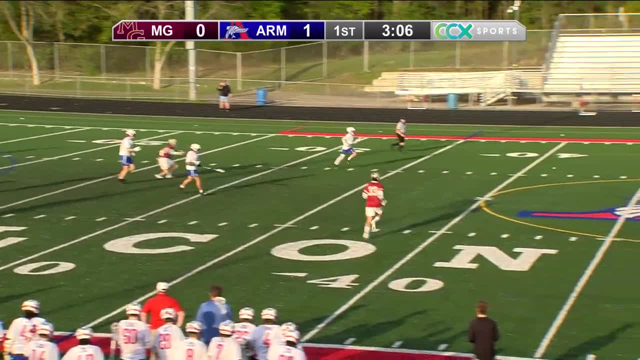 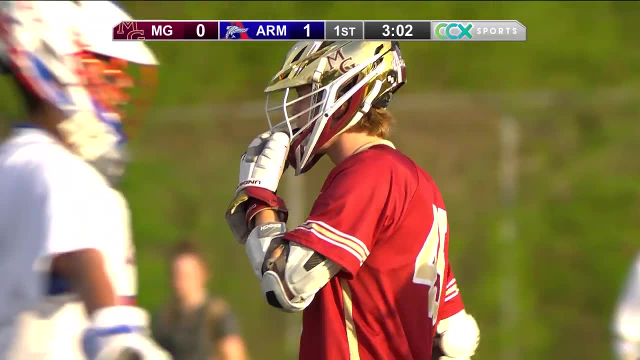 Face-offs. by my count even 1-0 the score, but the whistle blows the play dead. You saw it and you see that with the scramble for the ground ball And the face-off, It's been an area too that the Crimson have had to work on. 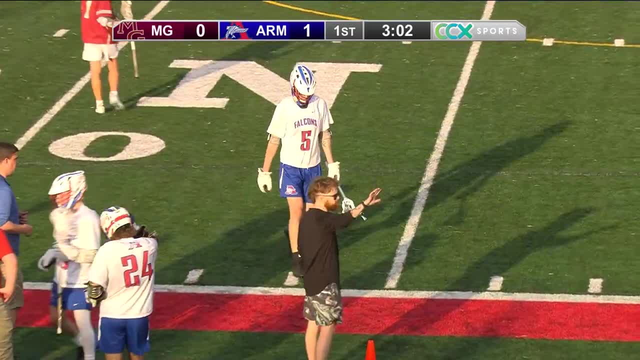 They have not done very well. They're around 47% on the face-off wins, where Armstrong has done a very good job at 61%. So if that changes the game, that's going to go to the Crimson's favor obviously. 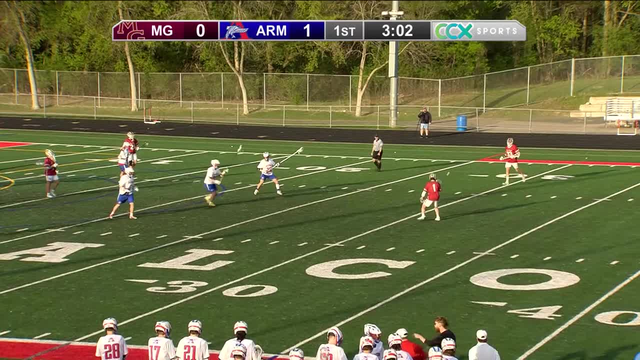 Coach not talking to his player, just kind of calming him down, saying, Hey, that's part of the deal, We'll work it out, Don't worry, We'll catch you back. Yeah, and it's so hard sometimes because you want your kids to. 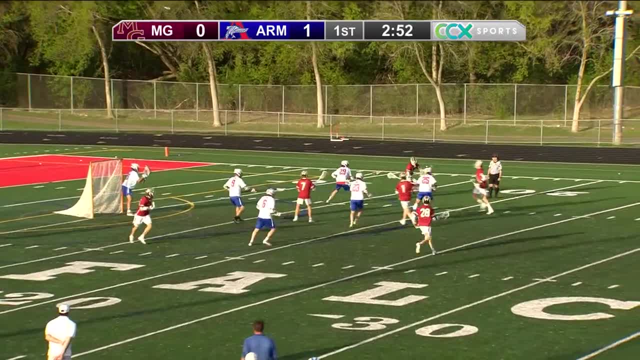 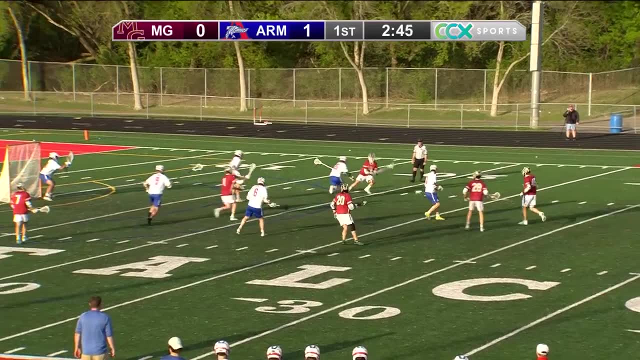 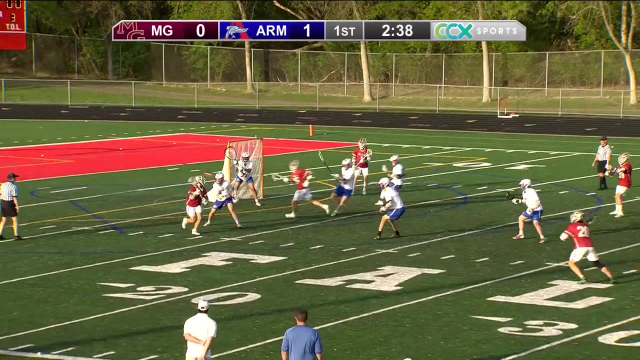 play aggressively But Crimson go to work on the EMO. Obviously Patterson, Peterson and Scanlon will be two of the focal points. you would think Scanlon holds up top for Peterson Worked down low. Steinkopf feeds across. 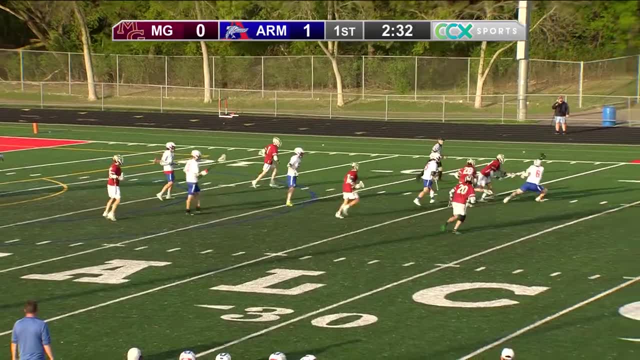 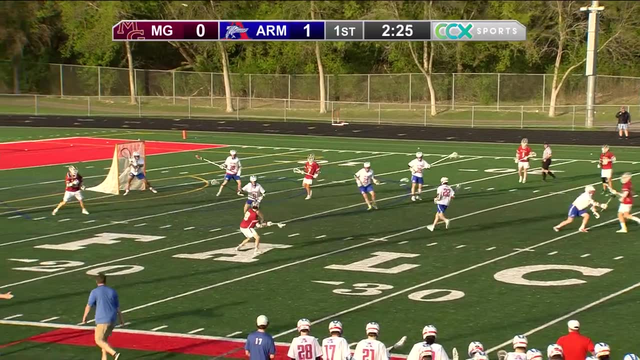 There's a sidearm shot off the post Wrung by Tanner Brendan, the senior midfielder with 12 goals and 12 helpers. He recovers. He uses it now, Scanlon, There's a spout shot and they score this time. 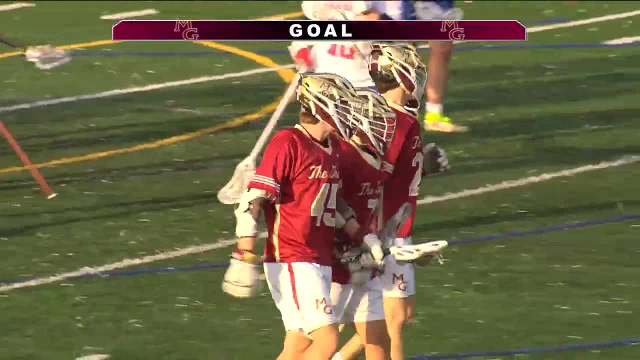 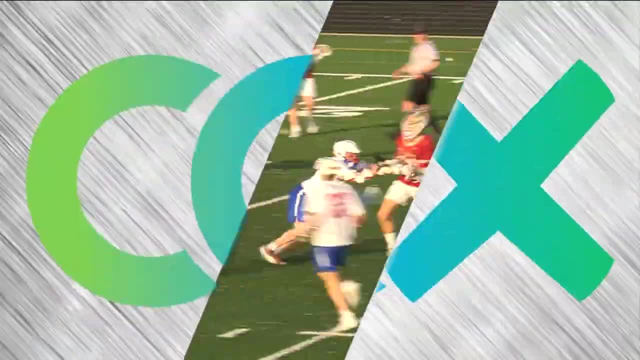 And it's Landon Bakke with his 14th of the season on the EMO to tie us at one Boy. that was kind of a key goal here from the looks of the saves, not only from the goaltender but from the goal post itself. 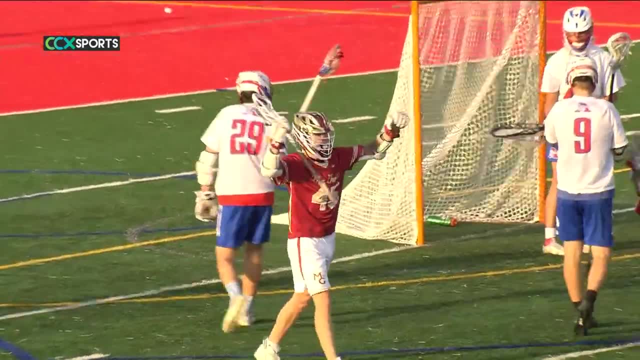 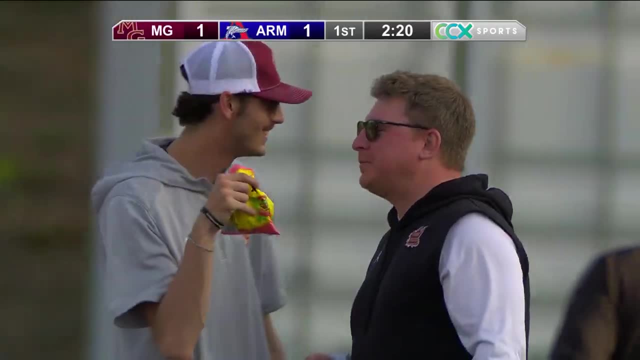 It looked like it was going to be a tough night. but he got a nice slow shot, used the D as a screen there and pumped it low and bounced it through the legs of Xavier Wells And nice goal. Nice goal by the Grove. 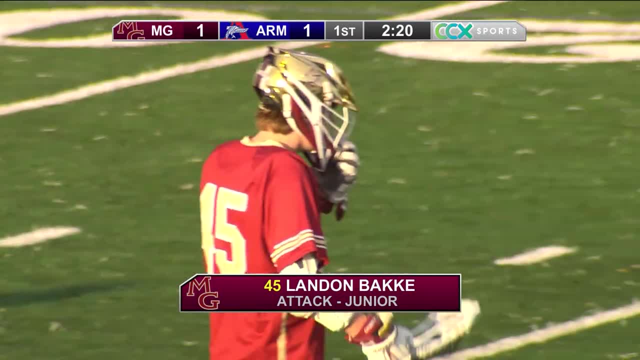 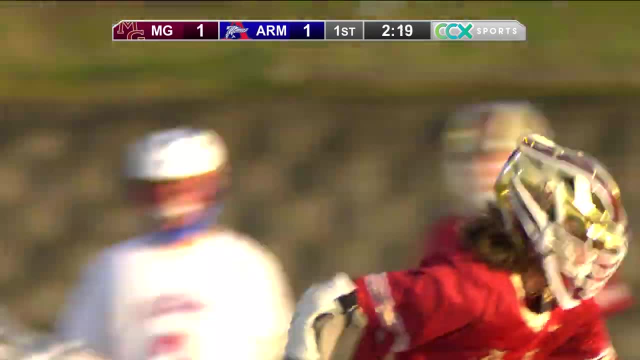 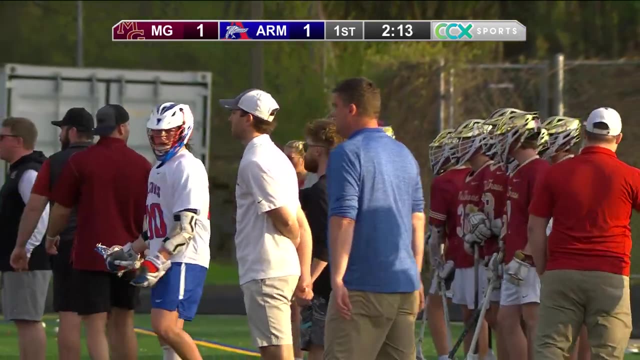 Bakke from Scanlon at 220 of the first quarter to tie us at one. for Scanlon his 12th assist of the season And another false start on Maple Grove, so it's going to be Armstrong's win. That's how they've gotten both their face-off wins here tonight. 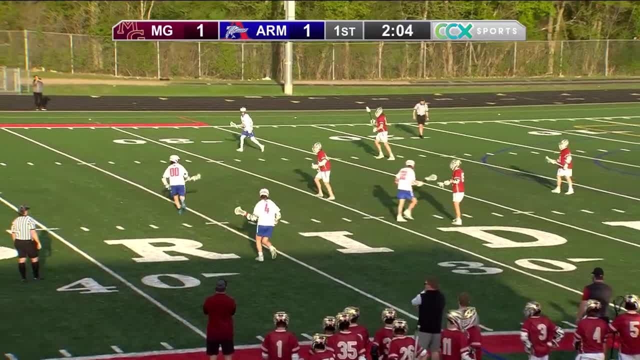 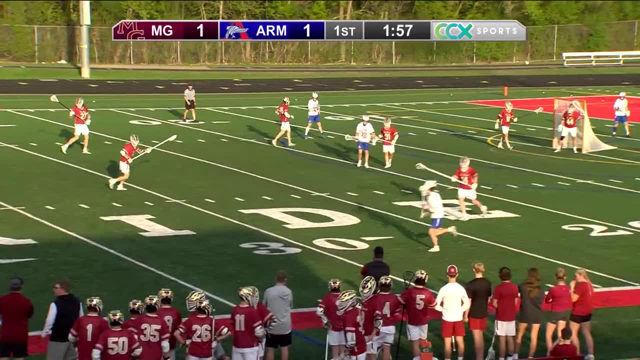 1-1 our score. Our late first quarter and the game so far has been a defensive struggle and it's been as competitive as you and I thought it would be. Yeah, There's not a lot of room out there, but I'll tell you what both teams got: some jump. 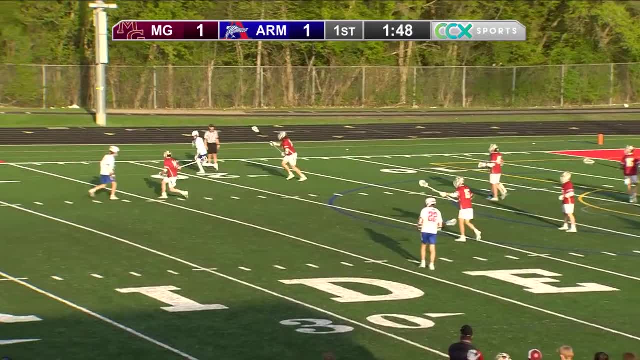 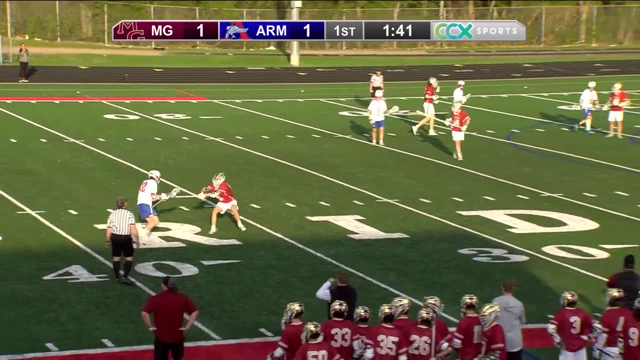 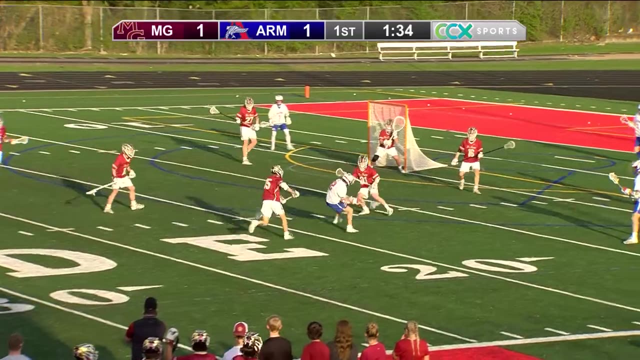 I mean, this isn't a slowdown game at all. I saw an incredible play the other night where someone rolled the ball casually like that and then one guy And then the other guy came and stole it. He was so fast. Another bounce shot. 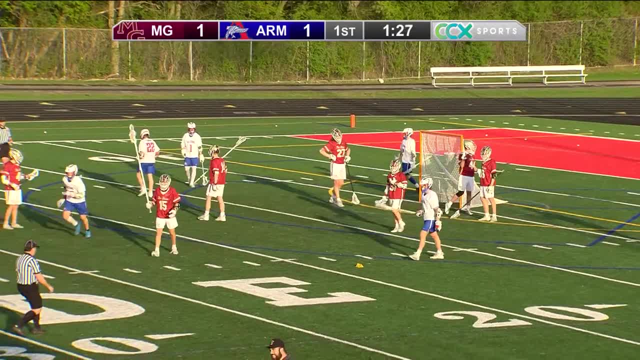 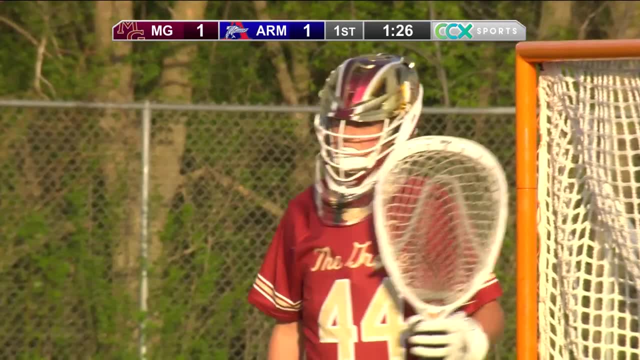 Farniak makes the save as Eason Essin was looking for his second, but the flag flies anyway, and so for the second time tonight the Falcons will have an extra man. Looks like Lucas Bakke the D is going on for a minute and a half for a trip. yeah. 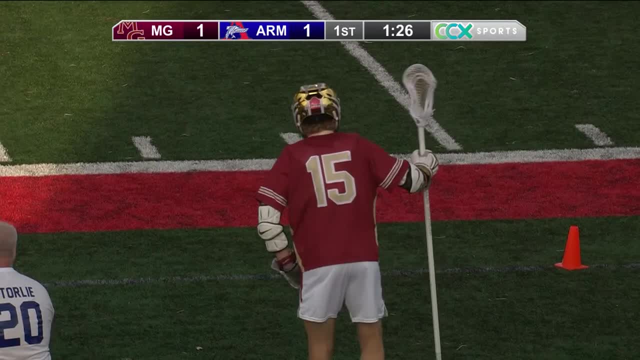 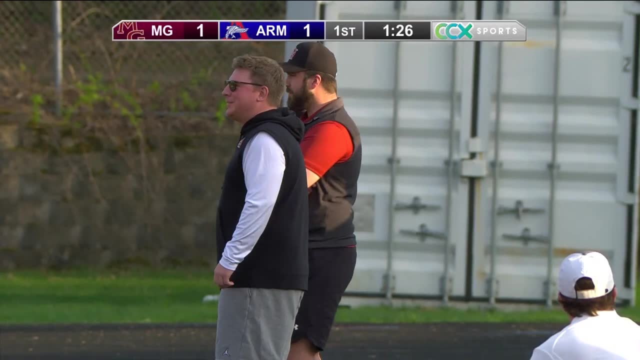 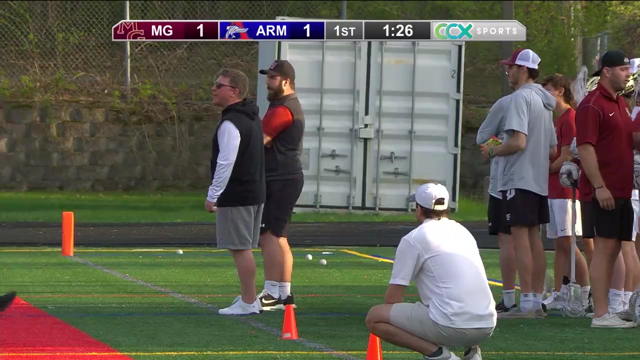 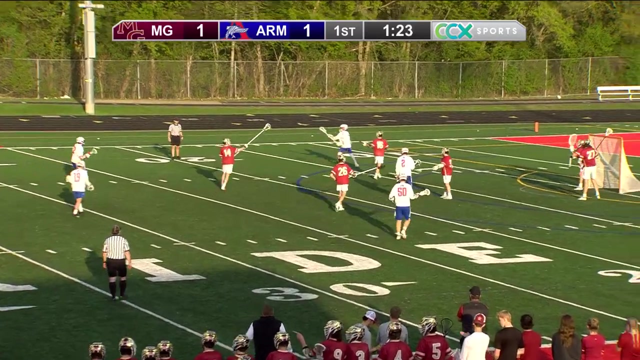 Well, you could see it there. He got that stick in between the legs and you know it's just like hockey. You got to be responsible for your own stick Coaching staff asking about that. So one minute for tripping, and now we'll see if Armstrong can answer Maple Grove's EMO goal. 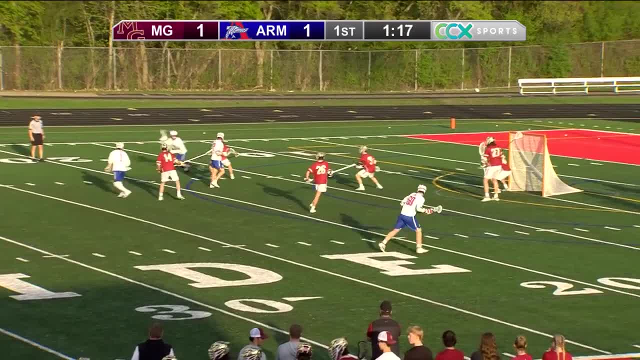 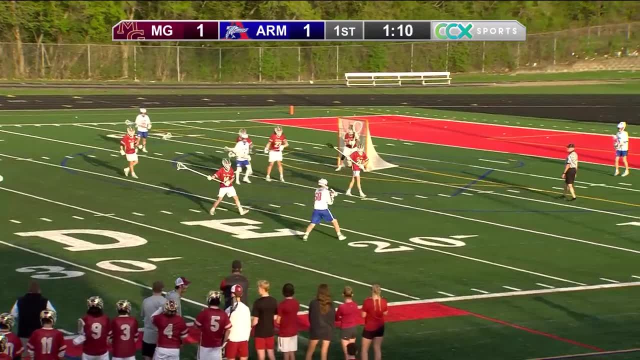 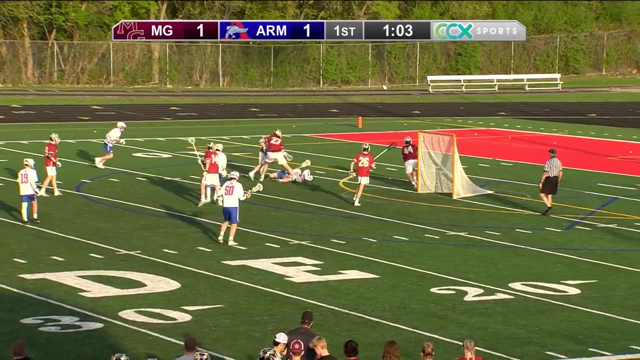 with one of their own, Albrecht, dancing and dishing, Dishing, Looking to find an opening on those slides. Get somebody to overcommit, That'll give him an extra man open. Olsen gets it back initially, but Farniak comes out to grab it. 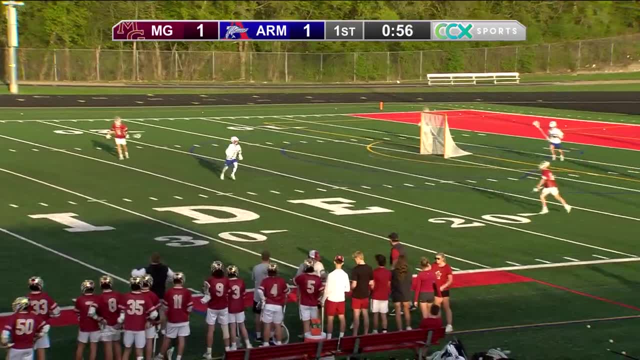 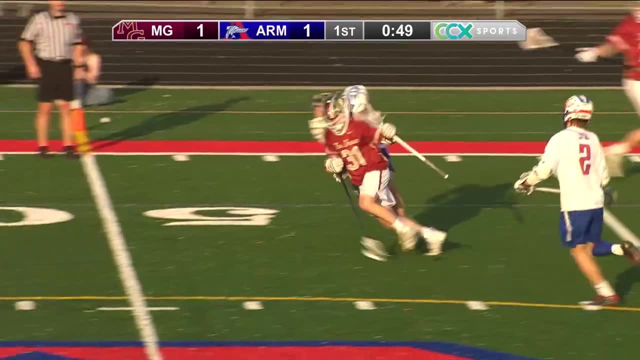 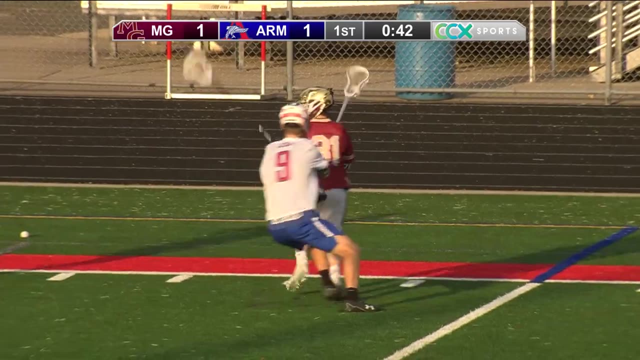 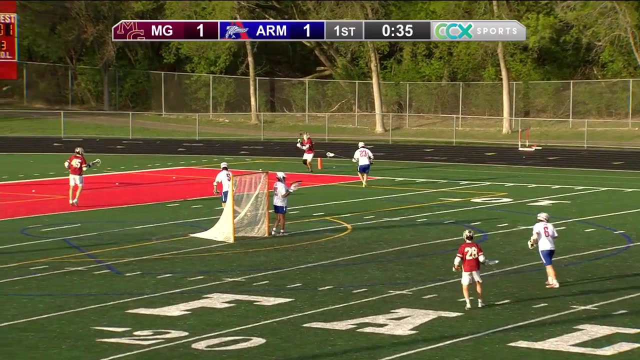 And now Maple Grove will try to kill off some time with under a minute to go here in the first quarter. Good presence here by Connor Kasbaum. Scammer Peterson, rather, will track it down and scoop it to himself in the corner. Brandon Bakke is big, big talent. 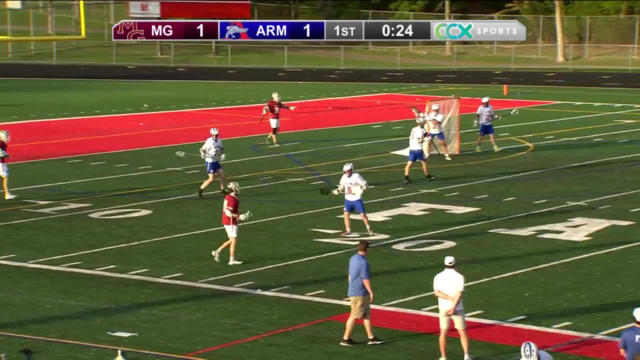 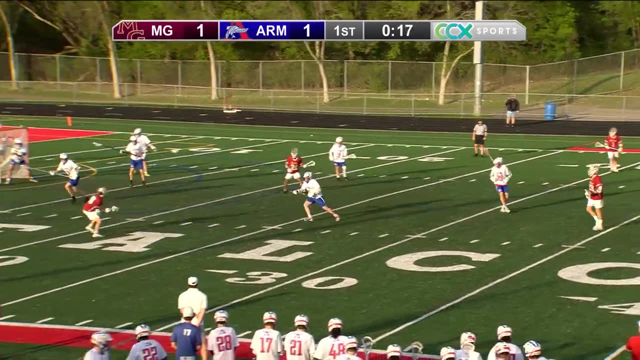 Bakke and Brendan, big strong guys, But obviously Peterson, really talented, is just a sophomore and he's more physically mature, I'd say, than most sophomores. There's a shot by Scammer and he just pulled it wide. 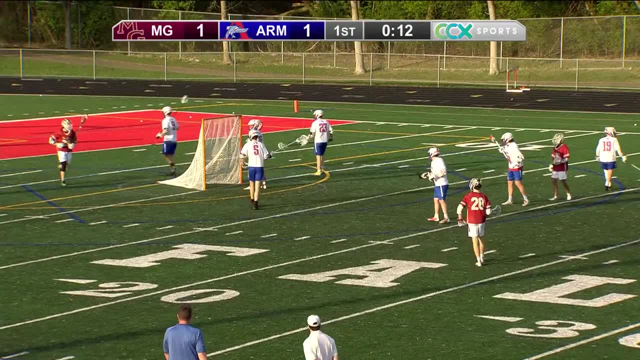 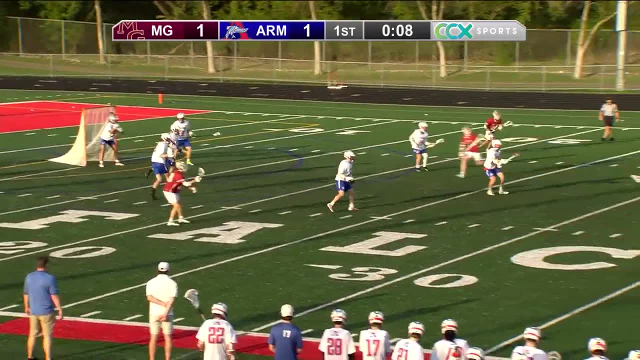 No one stepped to him. That was: those Falcon D are big. Wow, Yeah, Man, that'd be tough to get around, That's true. I mean, I'm talking about the size of Maple Grove's attack. Nine seconds to go. 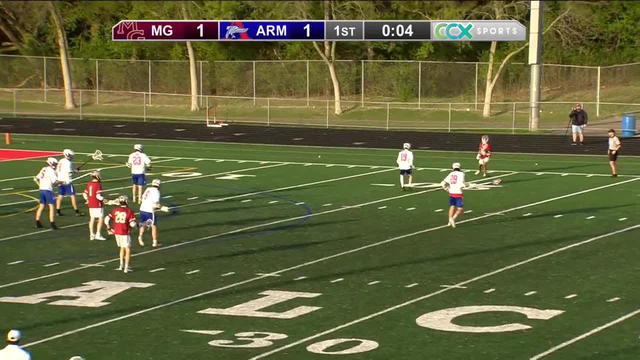 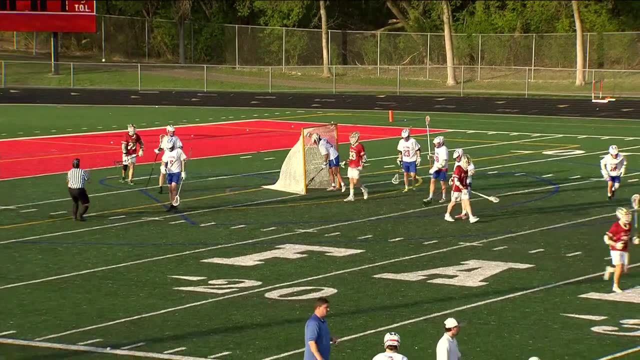 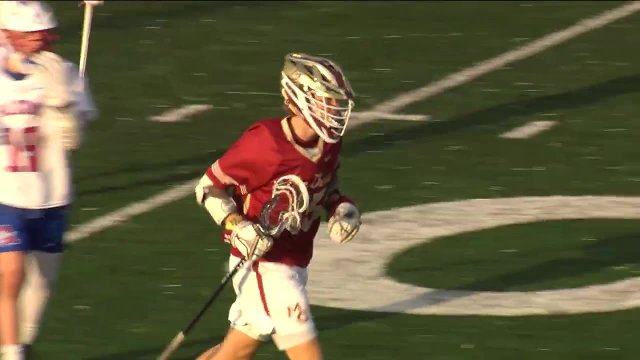 They've got to hurry if they want one Pass is a little high, scooped up by Domingo, Behind, as time expires, Maple Grove, unable to get a shot off here before time expires. But an entertaining first quarter of lacrosse finds us all square and one. 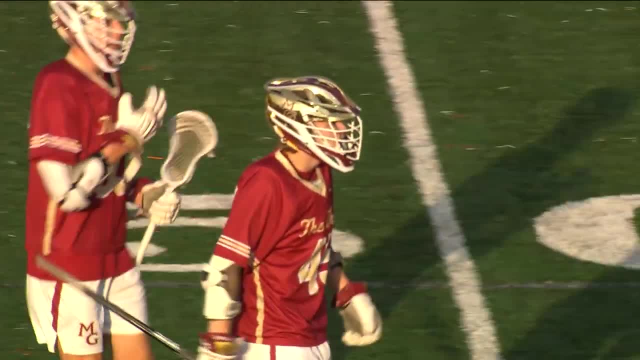 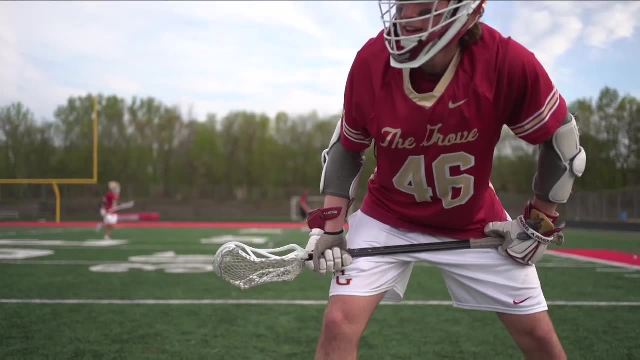 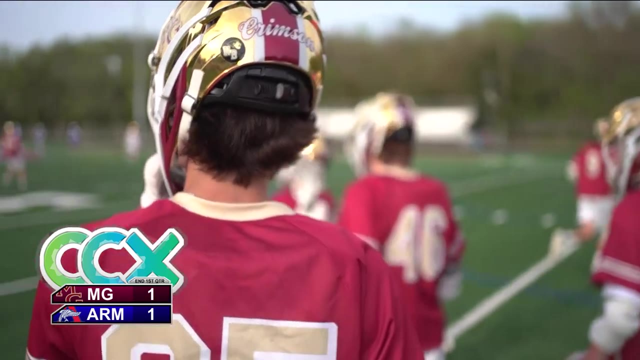 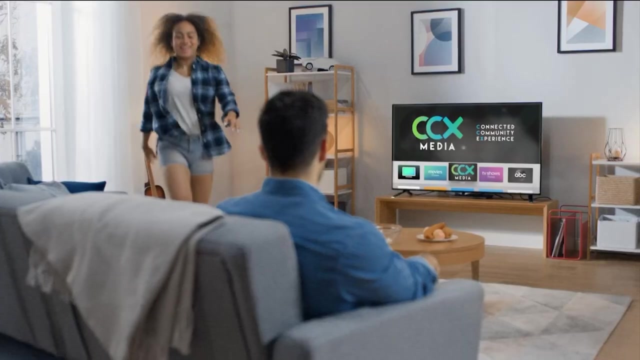 We head to the second Second quarter in a moment here from Falcon Stadium in Plymouth on CCX And under three. Come on. CCX Media, your source for great local programming, is available on Amazon, Fire TV, Apple TV and Windows. 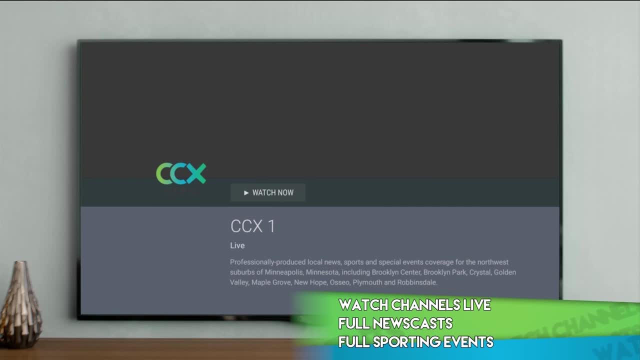 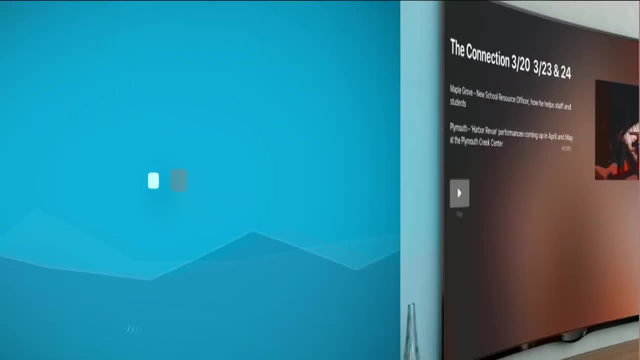 roku. our free app allows you to stream all three of our channels live. you also have access to a large on-demand library including full sporting events and daily newscasts. to find us, go to the store, search ccx, and download our free app. then sit back and enjoy all of your favorite local 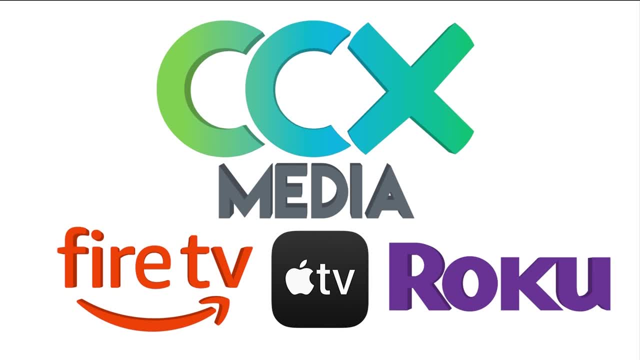 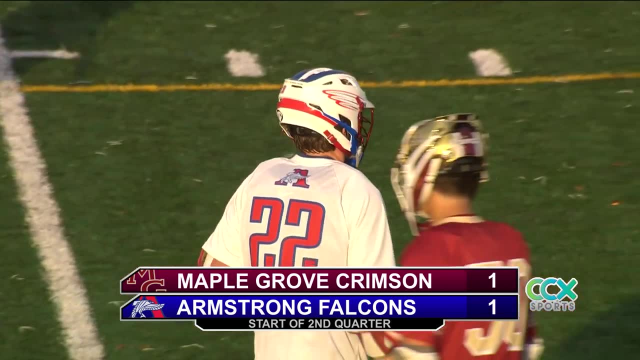 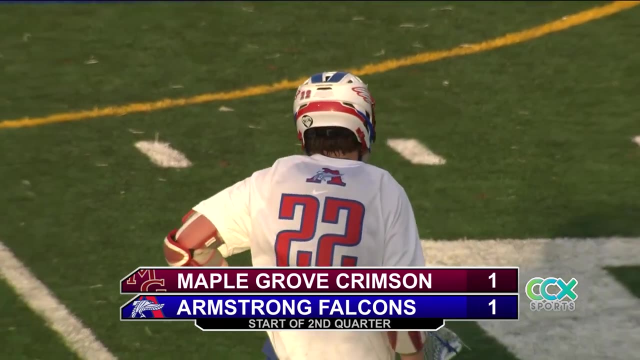 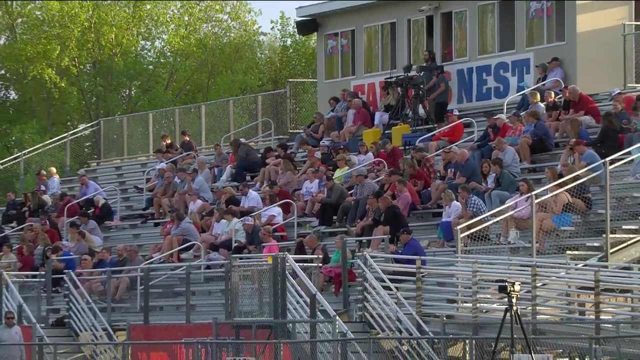 content: the ccx media app available on amazon, fire tv, apple tv and roku goal scorer jameson essen, who had the lone tally for armstrong in the first quarter which gave them the lead. big crowd on hand tonight, obviously a lot of fans knowing what is at stake here at the falcons nest and 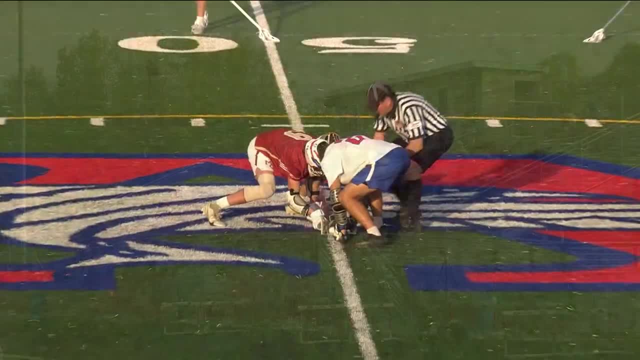 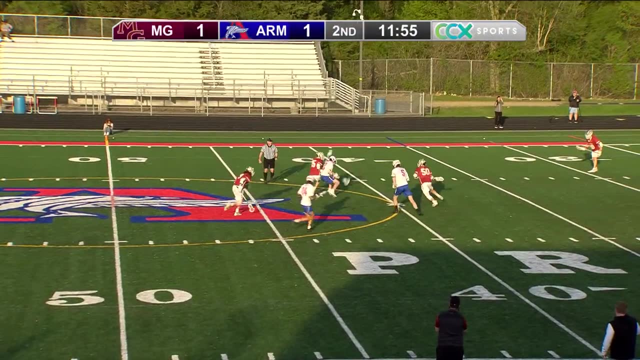 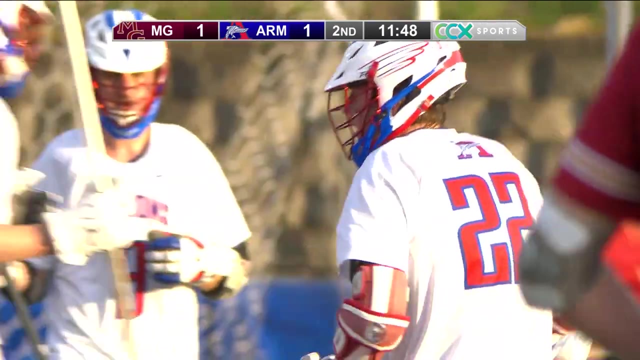 robinsdale armstrong got on the board, but maple grove answered on the emo a little over a minute later, so it was more or less tied for most of the first quarter. face-off is a push, so it'll go the way of robinsdale armstrong. they've won three of the 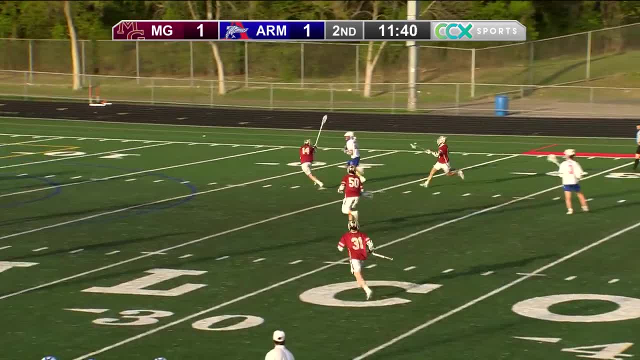 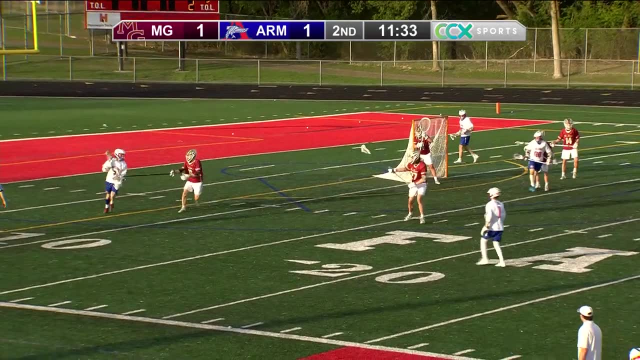 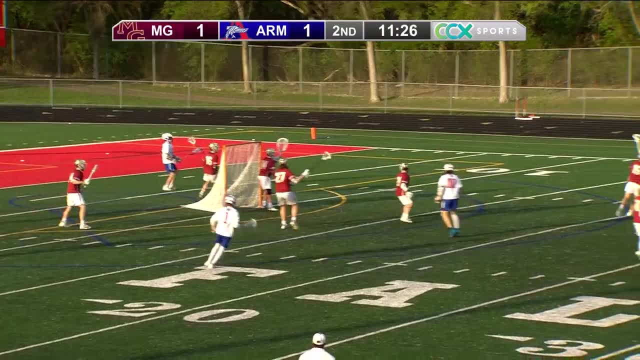 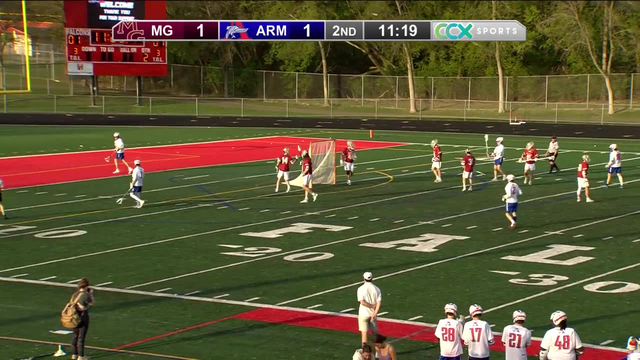 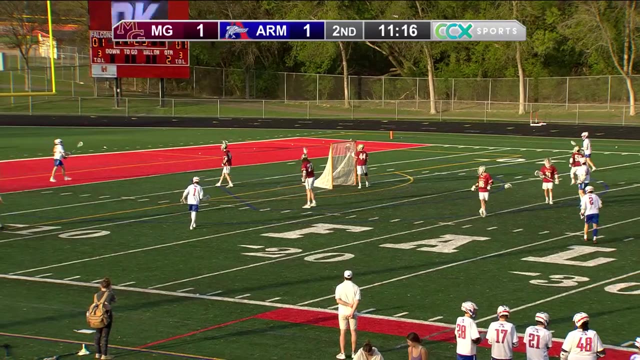 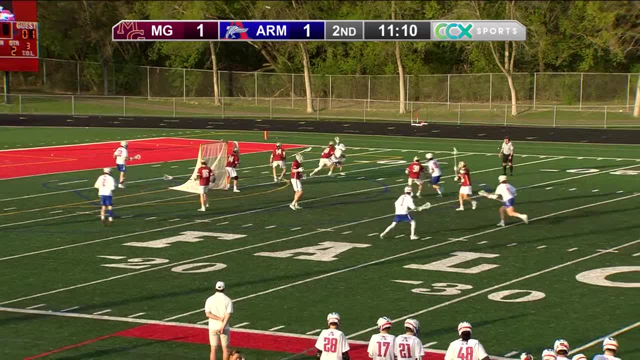 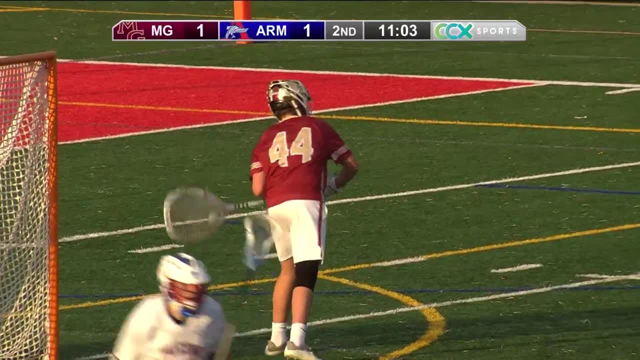 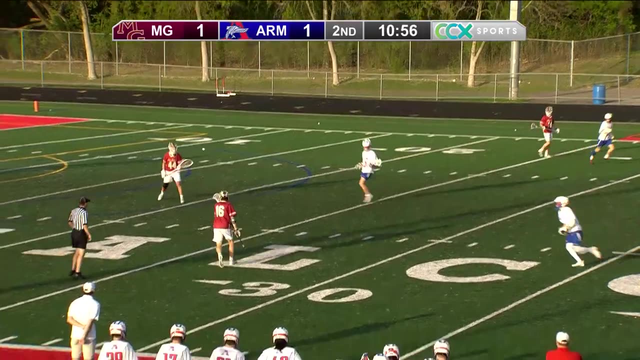 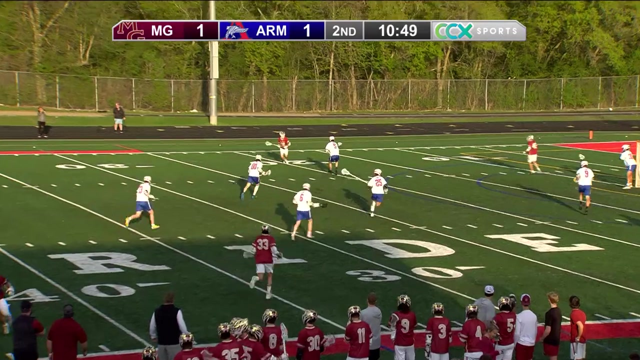 having that much of an impact on varsity. says something. olsen, lefty cradle and farniak says thank you very much. collects the shot and rolls it out in transition. 10-man ride employed here by robinsdale armstrong. shane rask chucks it forward. oh beautiful, fine cross field there. by briggs leiser. 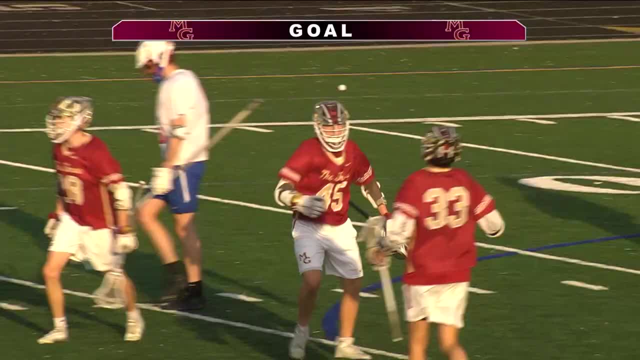 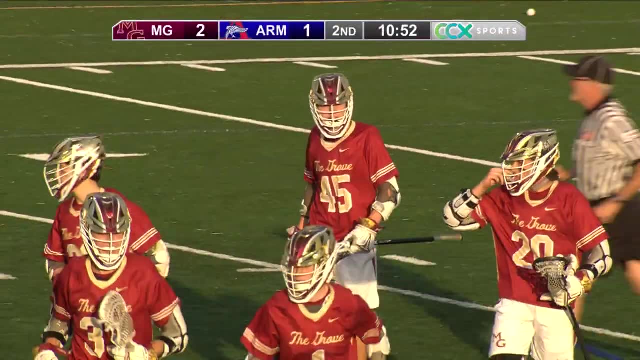 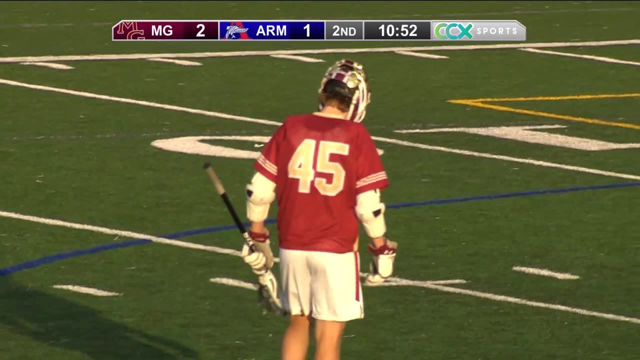 there's a shot to score. it's the second of the game for landon bocky sneaking around from x and finding the upper 90. boy. second time he came out on the left side of that down the middle of the that net again and they found him. three just fabulous cross field passes that moved the ball. 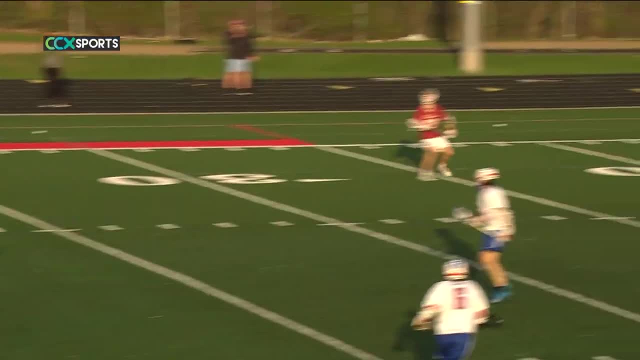 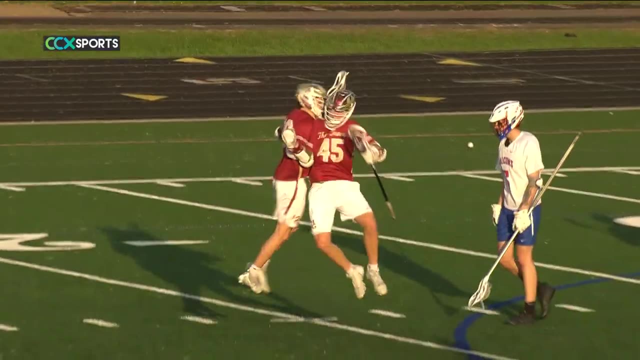 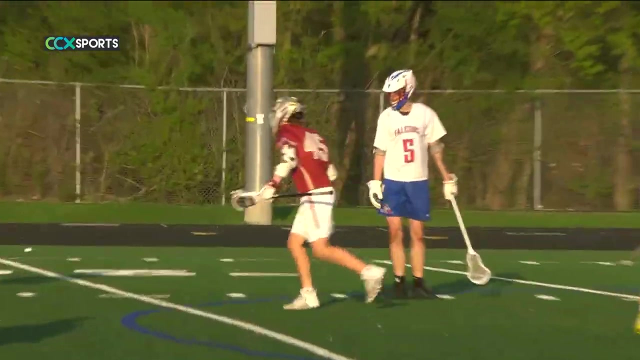 down for the crimson and set up the score. there's that long pass across and everybody's trying to compensate for and they forgot about him. second time today it's been baki from scanlan and it makes it two to one. maple grove boy, nice shot to caught the upper part of the short side there. 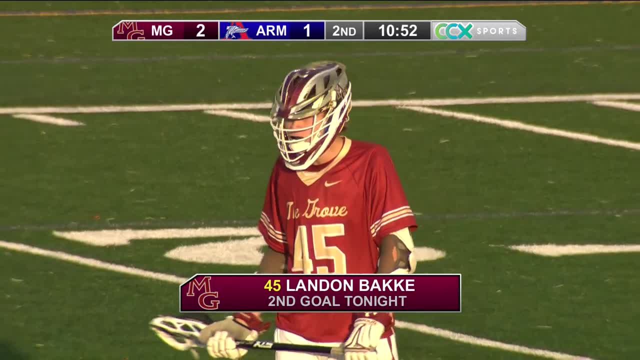 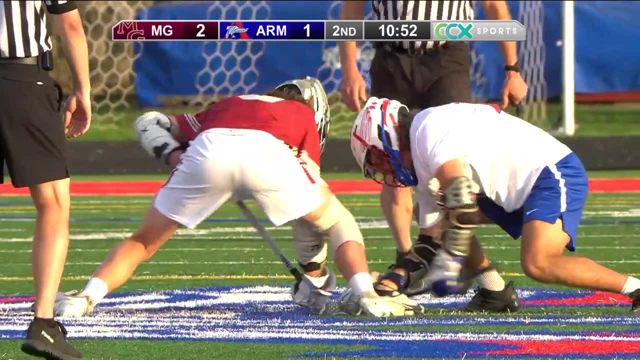 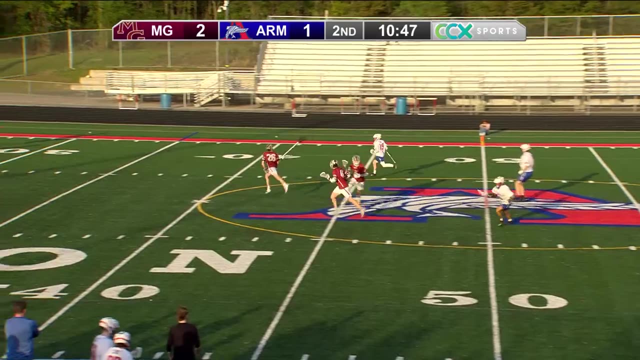 that's a tough shot. second goal tonight for landon baki came in with 13.. he's got 15 now on the season and for scanlan assist number 13.. as once again robinsdale armstrong wins the face-off. but again that. 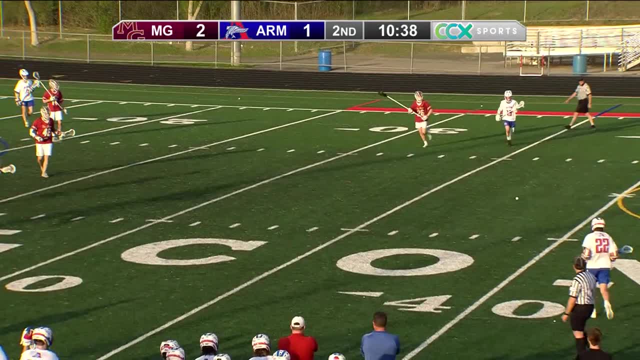 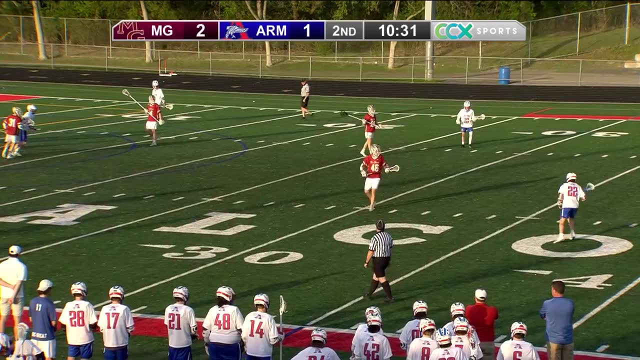 really has not. you know, when you see teams get in a make it, take it mold, that's when, yeah, we're trying to come back. that's when it really matters. but so far it has not. you know, we've got a lot of, but if you keep giving it to him, sooner or later something's going to happen. yep, as essen. 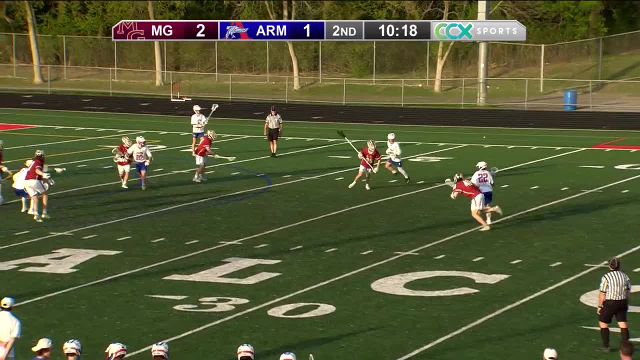 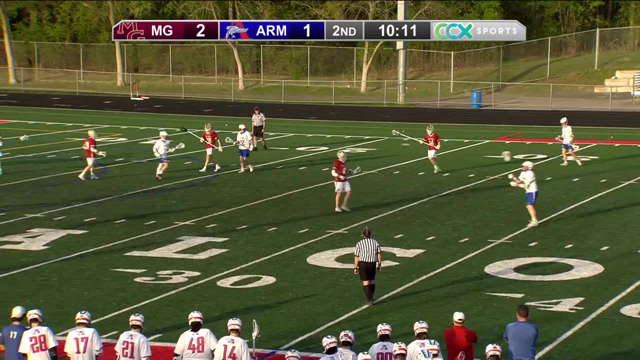 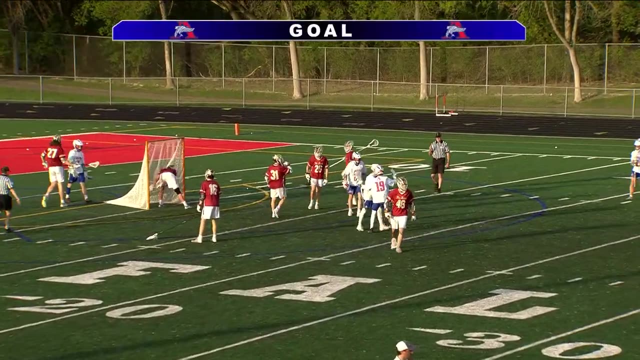 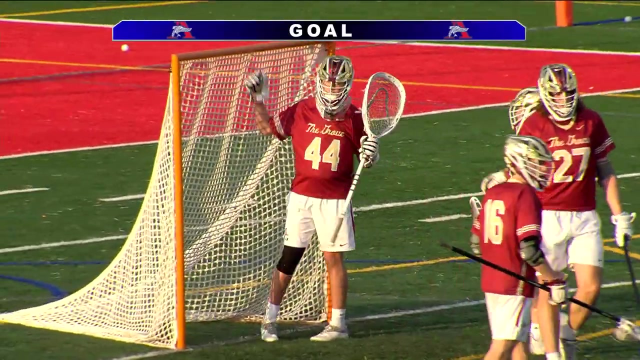 collects right near the logo at midfield against the short stick. downhill olsen forced back. they know how good he is. you'll see anis inside and he scores going low to high to tie us at two. great move on the d, faked right going down low and he stopped and came right back. put the d right. 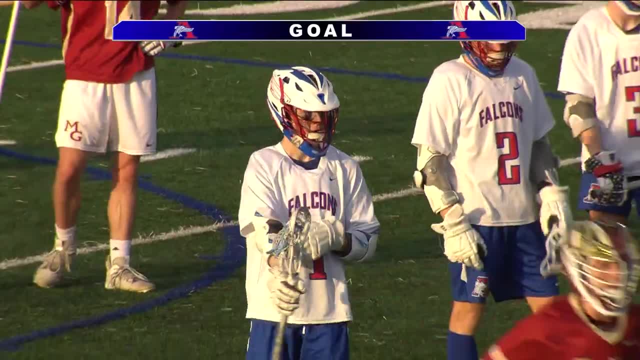 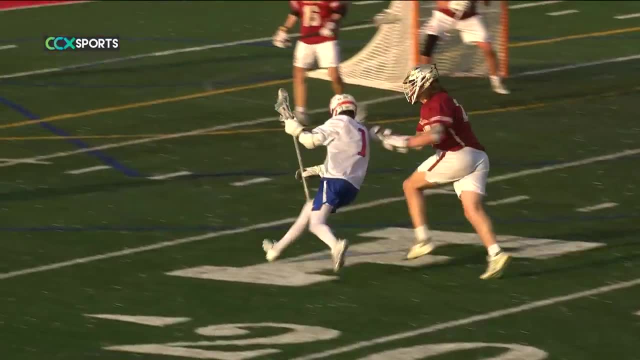 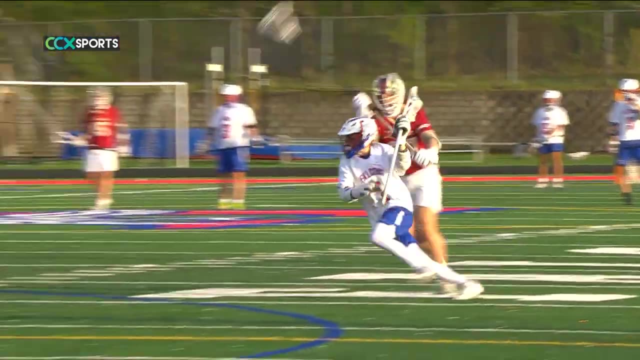 out of his jock strap and got himself a nice open shot. he, correct, did a nice job, going low, low to high. well, it was a beautiful move to sweep low anyway. and then, yeah, just ducked underneath the onrushing help of shane rass, and, uh, basically maple grove had the lead for about 47 seconds before. 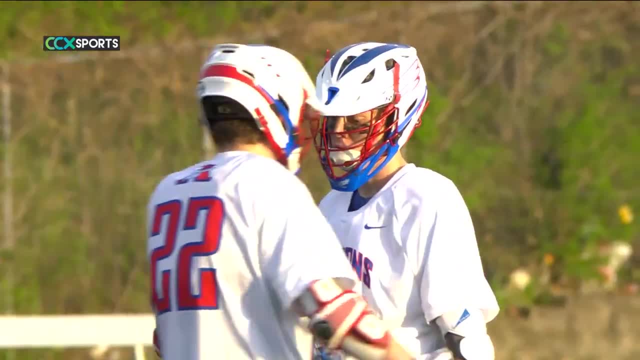 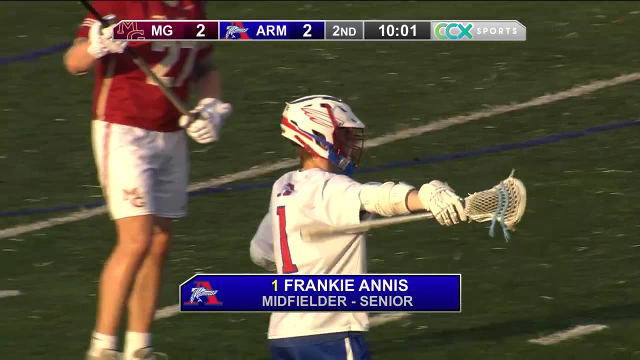 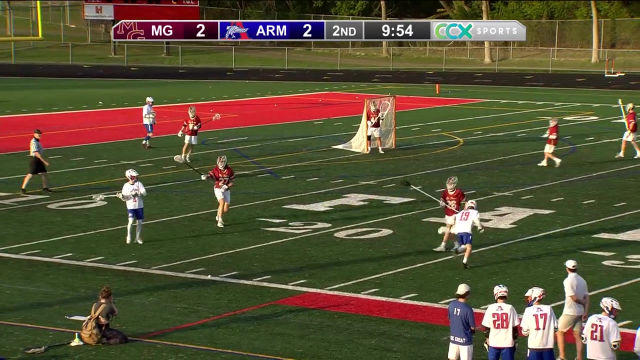 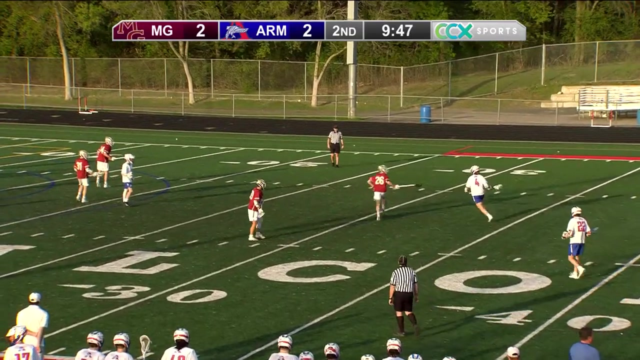 robinsdale armstrong answered and has us tied once more. dan, buckle up. i think that's what it's going to be like all night. i think you're right back and forth counter punches between these two nwsc heavyweights. fifth face-off win for robinsdale armstrong here tonight. well, there was no secret before the season. 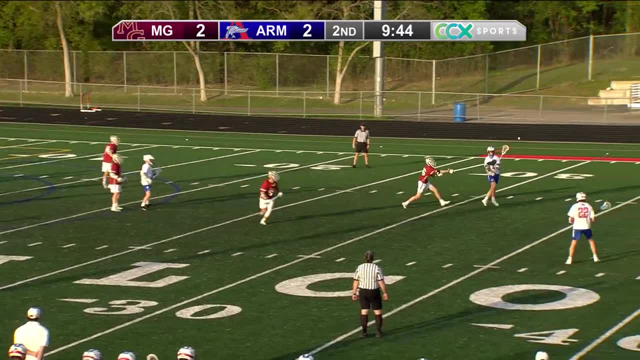 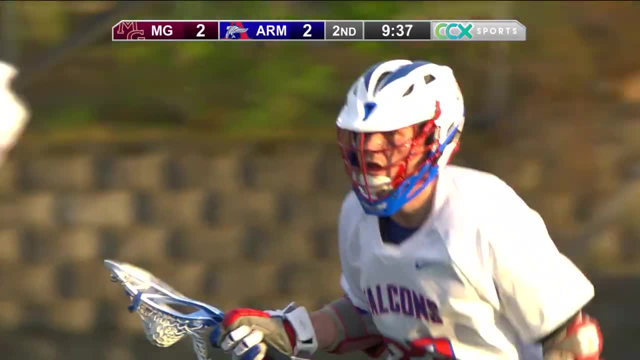 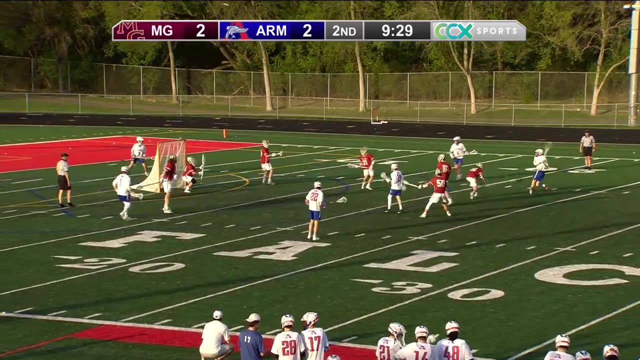 started that these two would probably be the two contending for the conference crown here. and uh, she's found the number one spot as well and kinda of uh shedes her trap. hospitality at the beginning to herهit's proven to be true. this is a heck of a game in real barnburn. heck of a section. two is 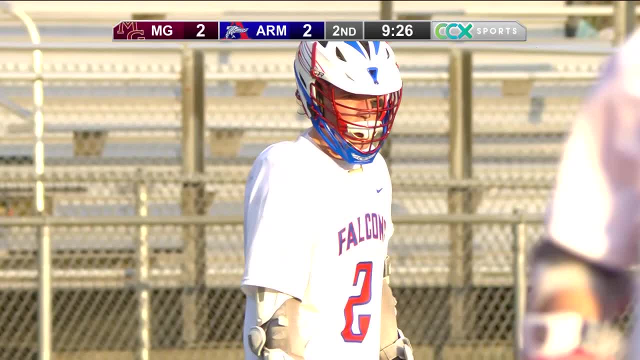 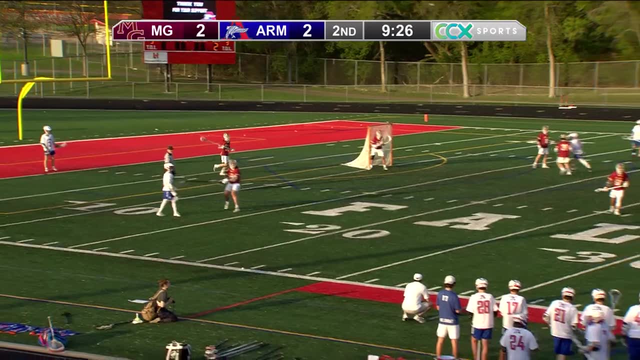 you have two lake conference powerhouses and wisetta. i suppose benilde is not a late conference powerhaus. scratch that. there's a shot from all brecht as he was moving to his right and he misses everything. but uh, yeah, loaded section five when you look at wisetta. and maple grove and armiesstrong and benilde st margaret's- obviously the biggest one, the defending state champions three: eat nous and bennelt st margarets is the only three has 8 winner. i think that will end up having the 8 win. so if they're996CE and 158c, move, yes, these three. 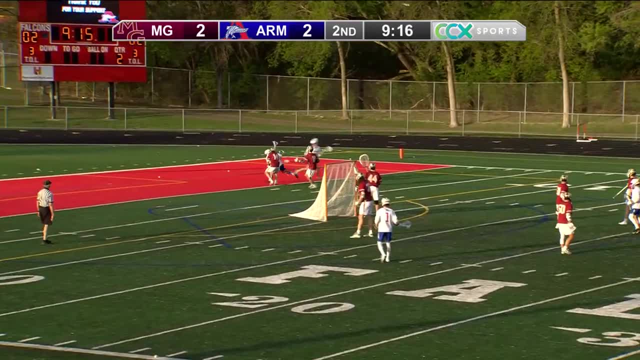 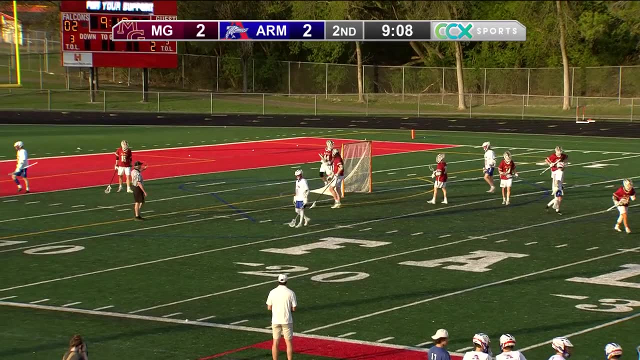 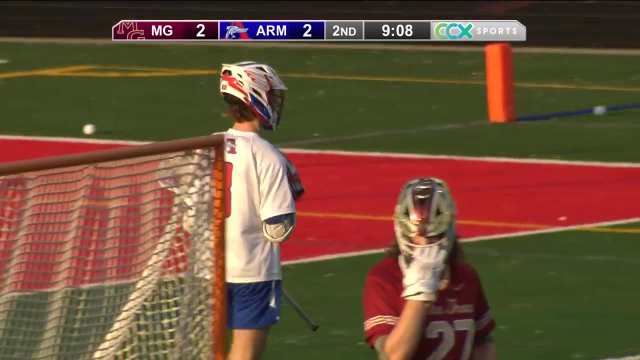 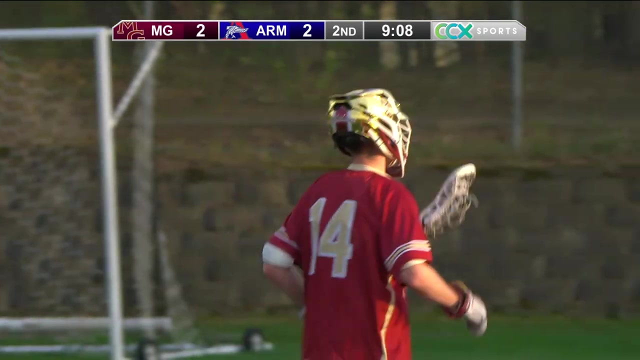 time defending state champions. and all three, uh, all four schools, rather three. and oh, bounce shot as a flag flies into the crease, jack olsen missing the net. but uh, it's gonna be the third penalty of the night taken by maple grove: the short stick. now i spoke too soon, not as. and joey heisler, joey. 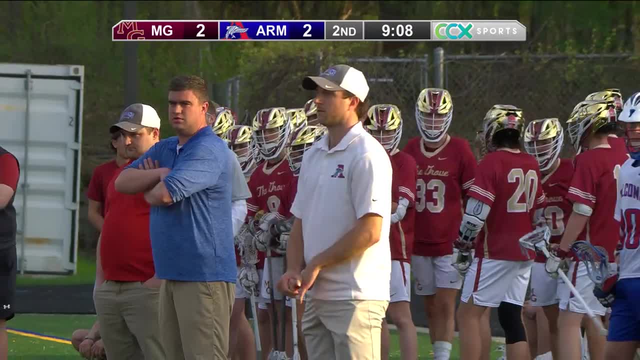 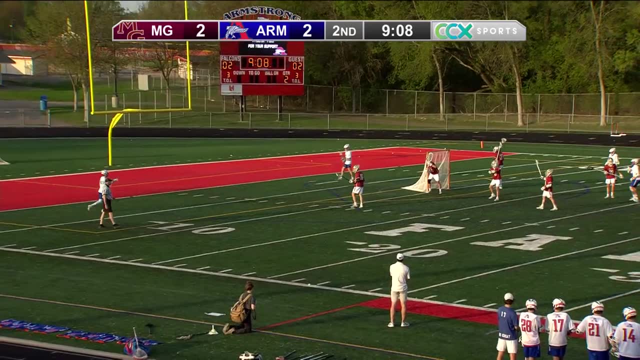 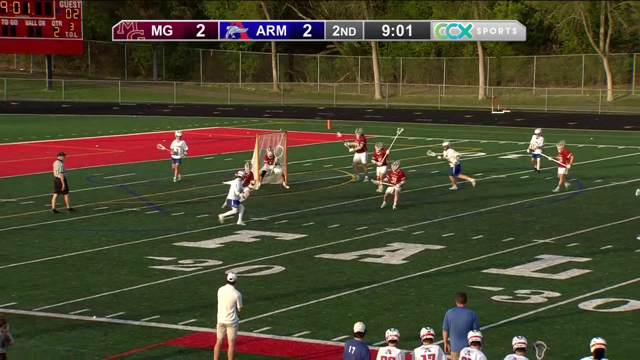 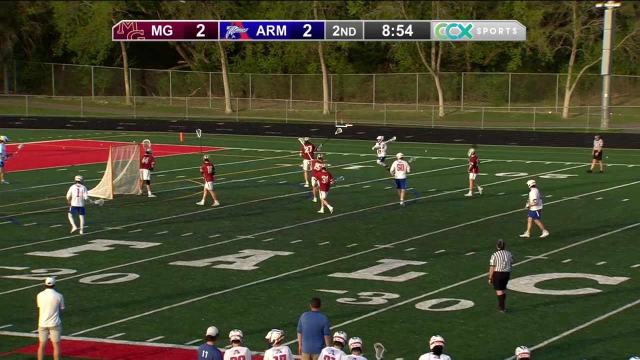 eisler his second penalty of the game, icer bound for carthage college in kenosha, wisconsin. next year cciw conference where i used to coach basketball- believer, really, yeah. assistant coach for milliken university back in the day- milliken, michigan, decatur, illinois- oh, yeah, okay. 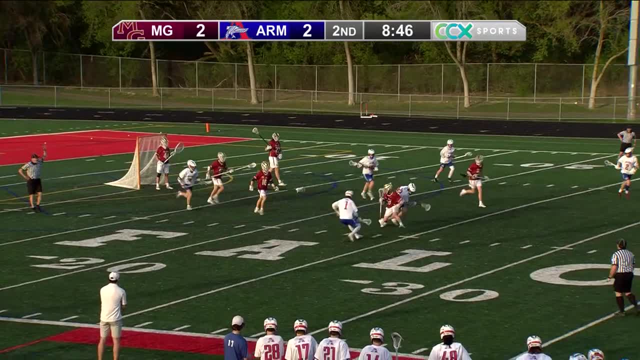 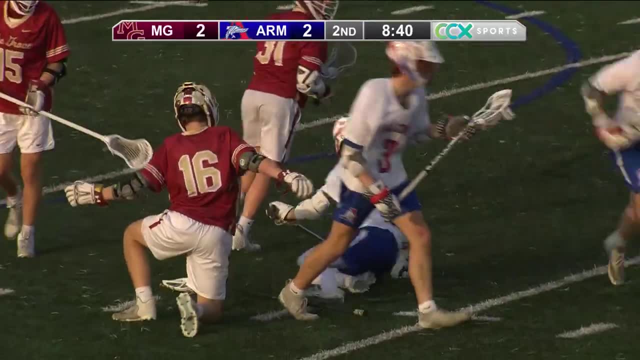 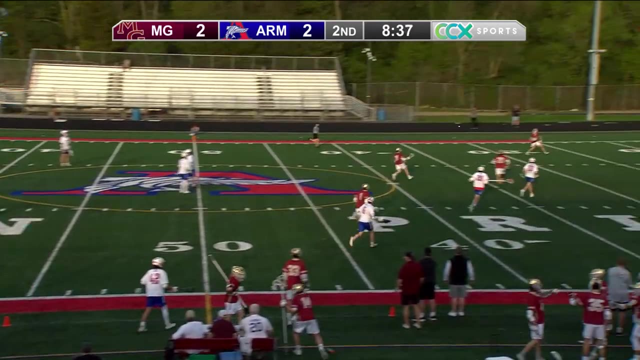 former home of the decatur staley's. way back in the day, great stick in the passing lane to intercept it. now a heap of bodies the edge of the box and it's going to be maple grove ball. and just out of curiosity, just who did the decatur staley's become? chicago bears, correct. 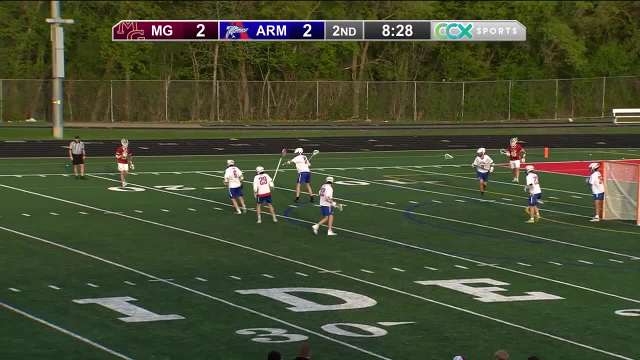 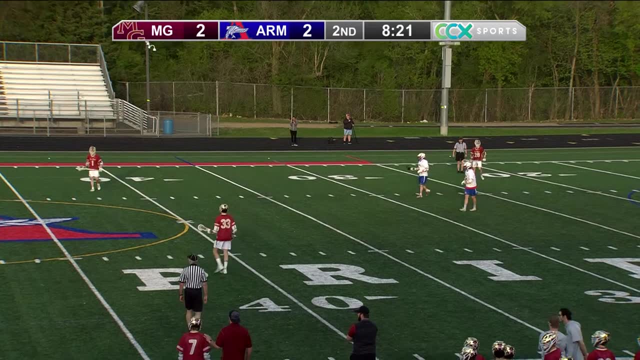 and they remain so to this day. eight and a half minutes to go before half two to our score here on ccx, armstrong and maple grove, both these teams coming off big, comfortable victories last night. these games, they come thick and fast this time of year, don't they? well, it's short season, you. 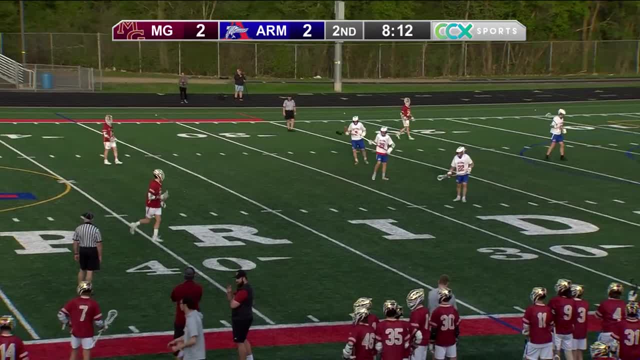 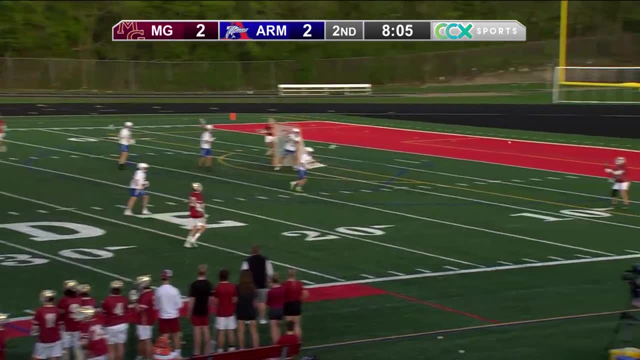 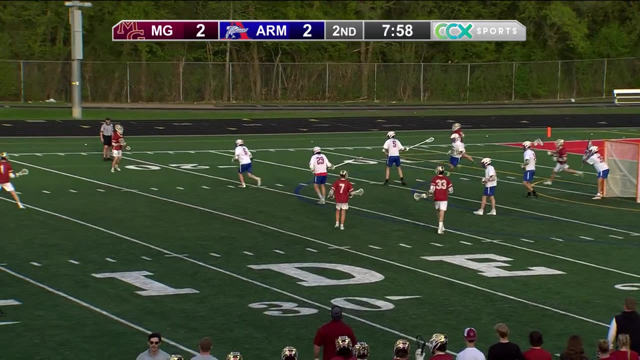 got to get as many of your games in as you can. i think you get 12.. and then they got to have room for sections before we get through the end of memorial day. peterson, a pie for scanlon steinkopf. and then they got to have room for sections before we get through the end of memorial day. 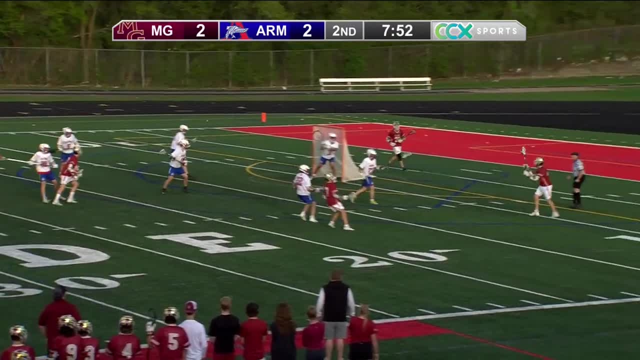 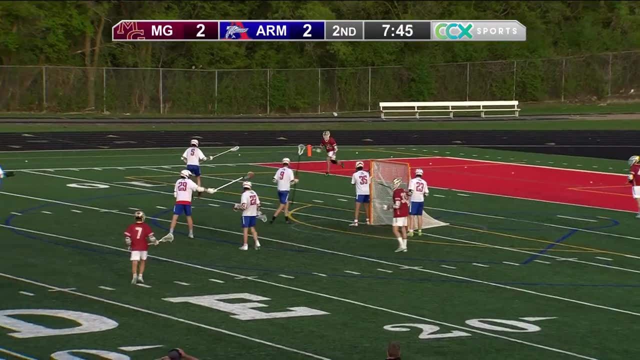 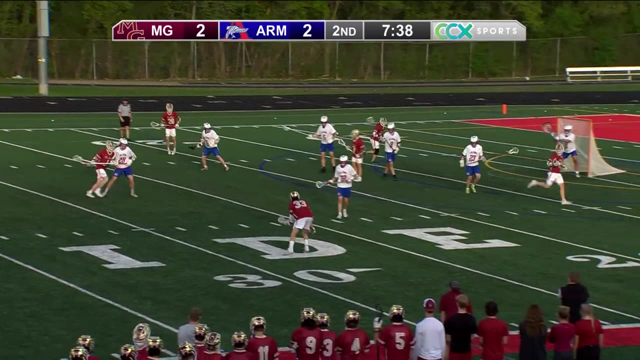 peterson up high for scanlon steinkopf. first time we've called josh thompson's name peterson, trying to track it down. they seem content to they're not pressing out too high. i think they respect the driving ability of this maple grove team. 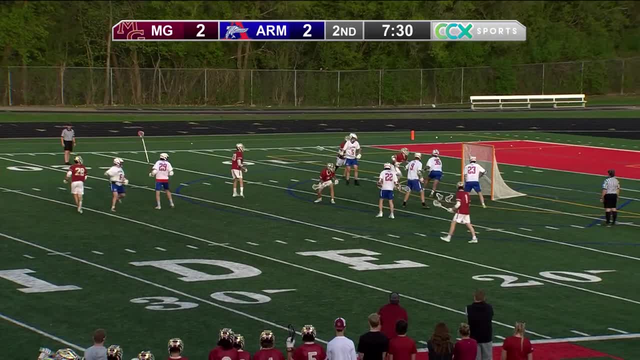 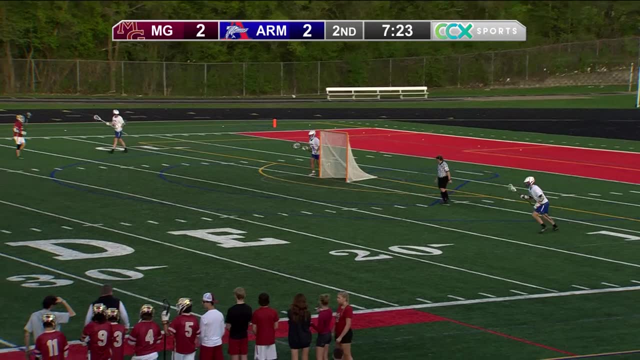 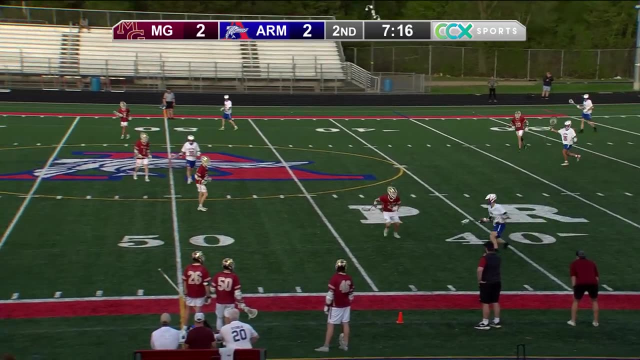 we're back to even strength sidearm shot comfortably by xavier wells. wells numbers this year and one and eight four, three goals against average. how about this save percentage? 644.. yeah, very impressive. by my count, that's his third save of the night. farniak's made two. 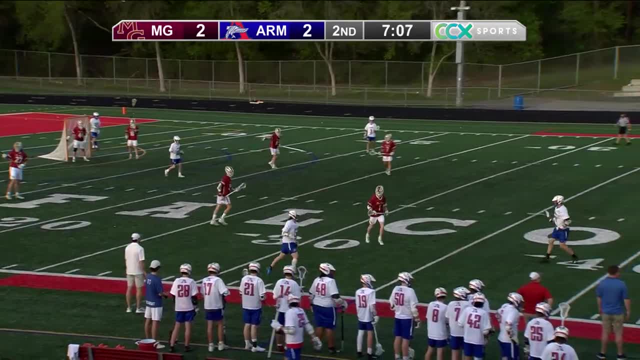 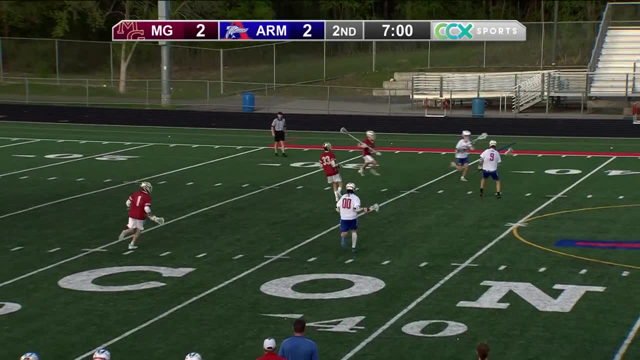 these are unofficial stats, of course, but well, you know you're kind of surprised, you know, because we always talk about the offense of these teams. they're all both having 13 goals of games, but the defense actually has been the real story tonight for both teams. yeah, the goaltending, the defense. so 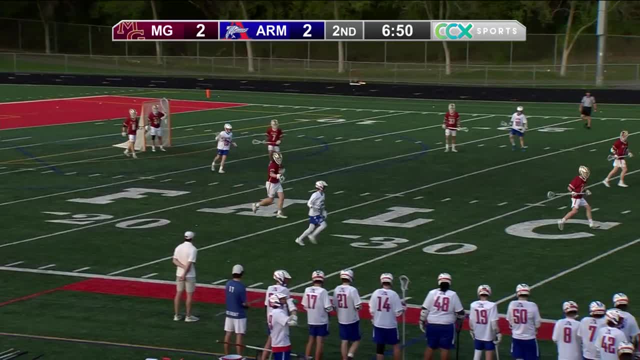 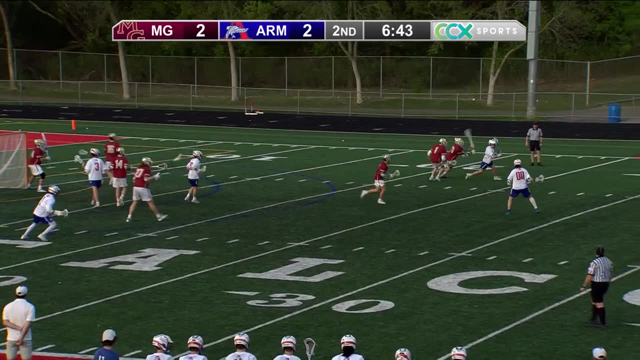 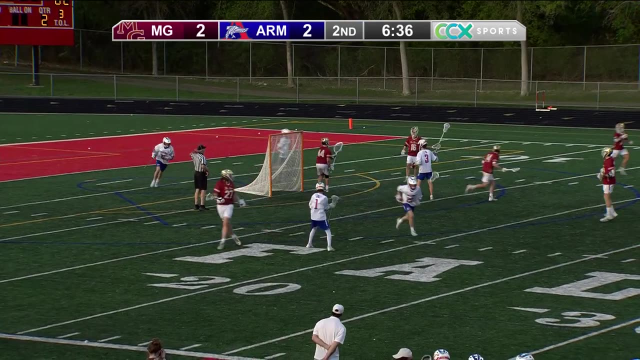 thisiele overwhelmed them. so this case they've got ahit any left free體. talk about the offense in the pregame open, but you to your point. yeah, farniac and wells are no slouch in between the pipes. assen draws the slide, spins away from it still spinning, bouncing, and farnia makes the stop. 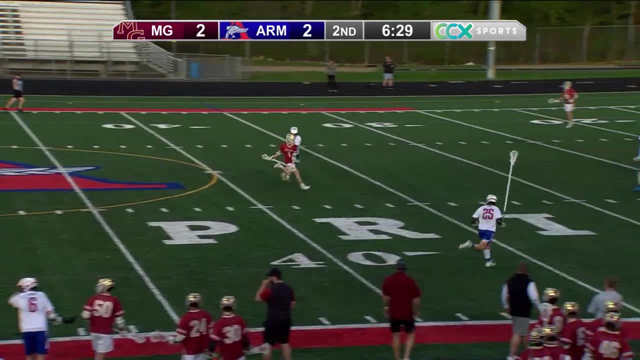 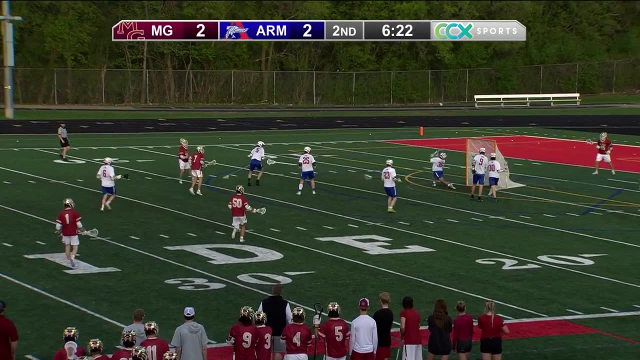 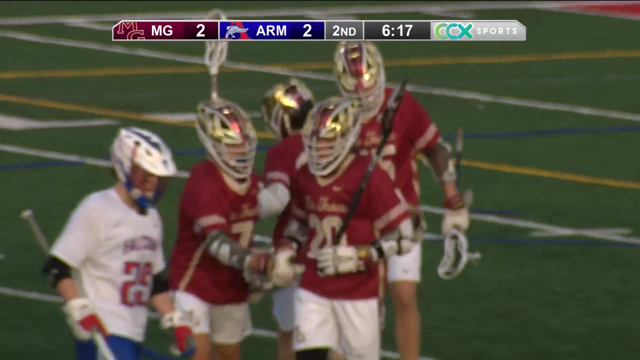 that would have been another circus goal from essence. instead it's outletted by maple grove. here they come, in transition with steinkopf, who the one thing They don't, just let their basket make the save. Nothing making the save. there, Rory Scanlon rips the back of the net off. a beautiful feed out high by Peterson. 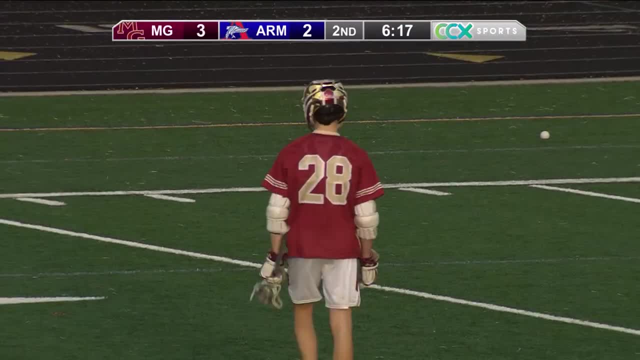 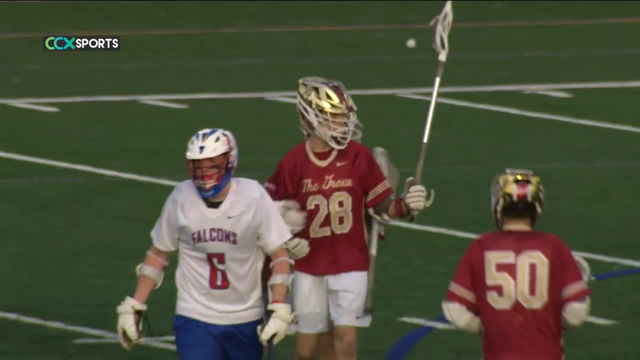 In transition. you've got to find the shooters, and Armstrong was made to pay when they didn't, with Scanlon scoring his 25th Goal and two assists tonight. now for Rory Scanlon Boy, you can't let Rory Scanlon wind up like that. 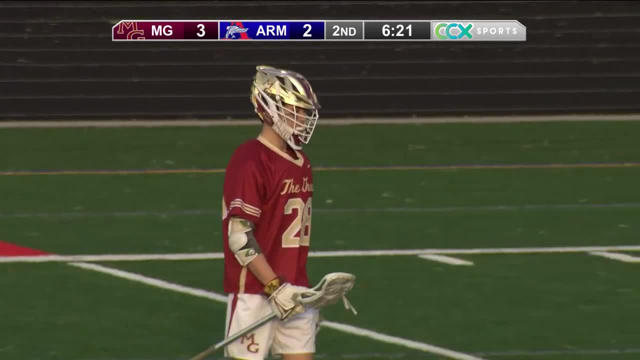 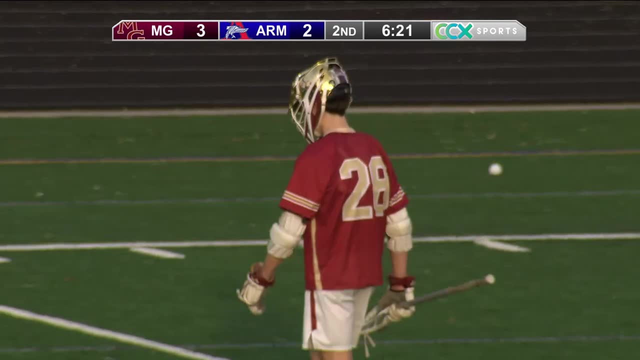 My God, he's got a bullet, as you can obviously see, and it just found the back of the net really fast, Goal coming at 6.21.. 3-2.. Maple Grove once again regains the lead. Scanlon from Peterson. 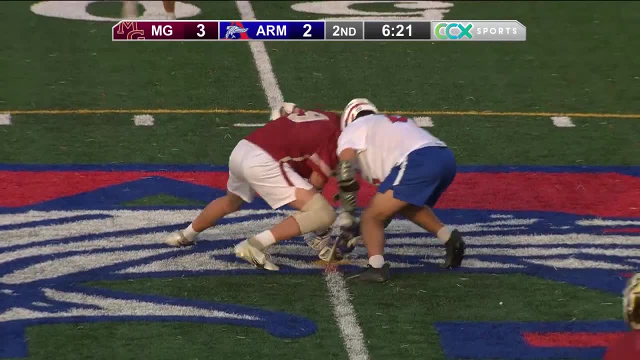 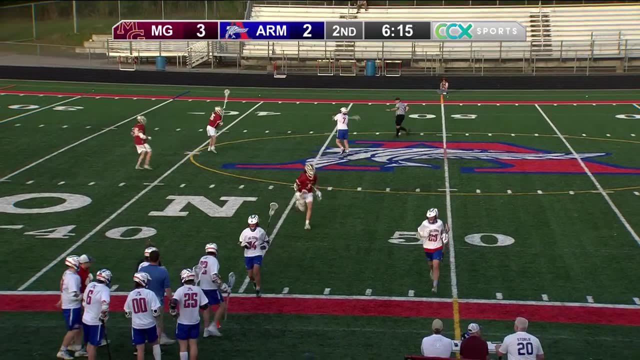 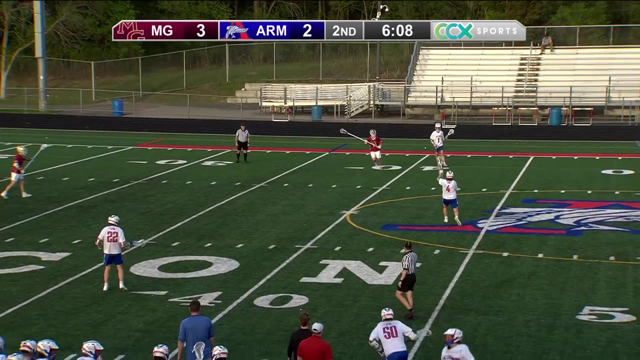 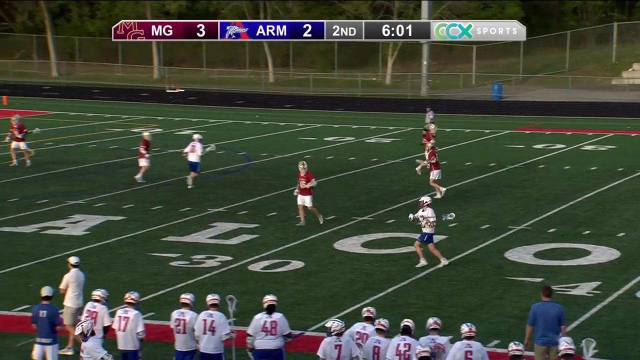 How many times have we said that this year? But yeah, Scanlon didn't even need to get his hands free, He just wound up and crushed it. Max Cole After, once again, Armstrong. the thing they can point to is how often they're winning. 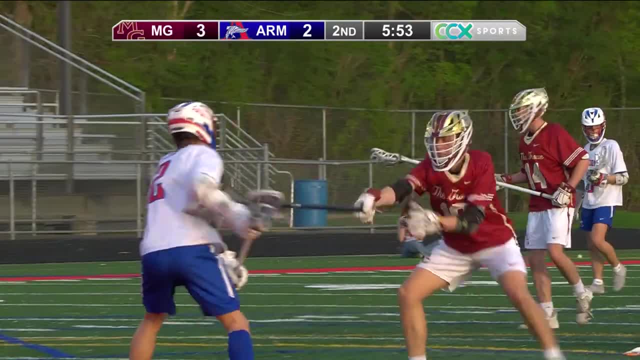 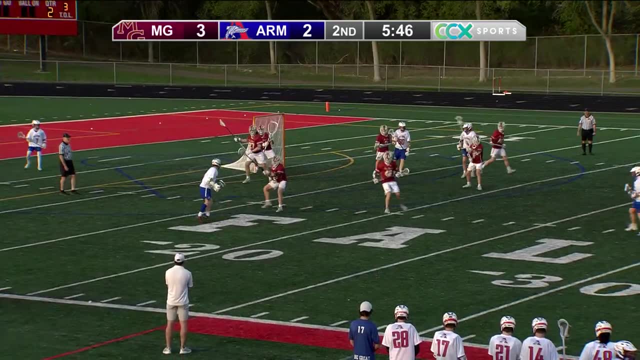 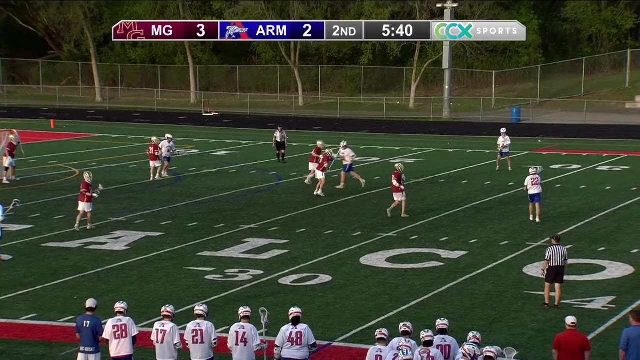 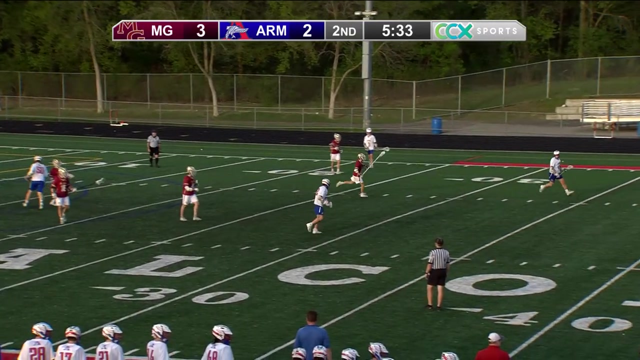 Six of seven at the faceoff spot and that's helping them get this possession on offense. as Albrook dances behind goal, Watched closely by Rask, Backs out, Correcting traffic as it's worked around right to left, Cole up top for Essin. 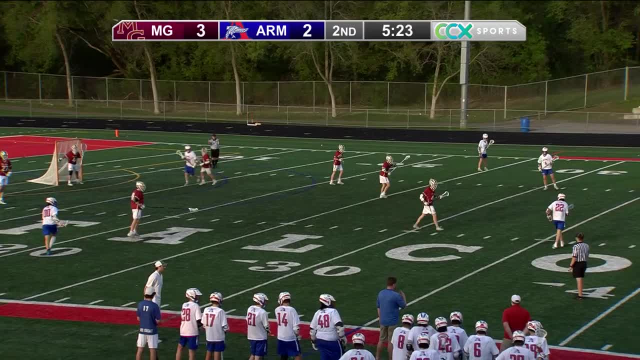 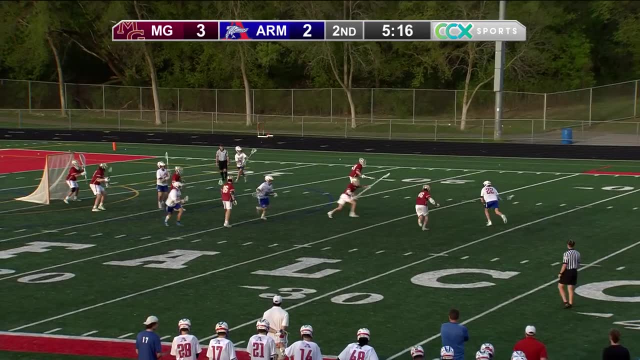 Cassidy, Now Maple Grove, willing to press out a little bit higher and push out as Essin attacks downhill against the short stick, Draws the slide, tries to feed it through a tough window and it calls right to Forniak or Farniak. 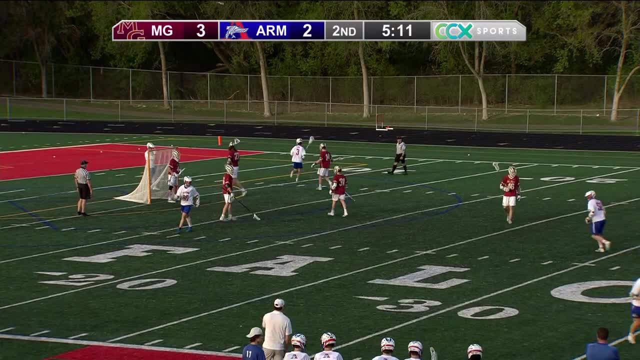 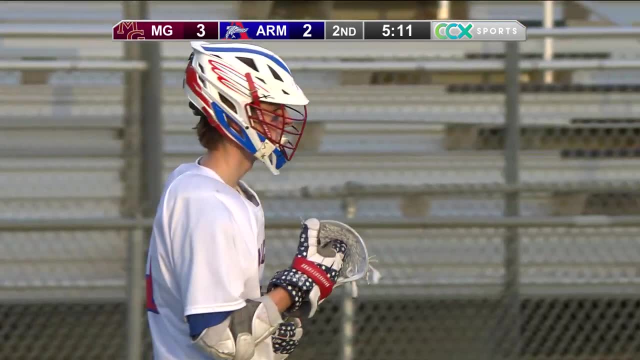 But Olsen, the diminutive freshman, was a willowy freshman. We'll call him Willowy. He's not diminutive, He's willowy. He was shoved down in front of Kreese, and so possession remains with Armstrong, as they'll roll it to Albrecht. 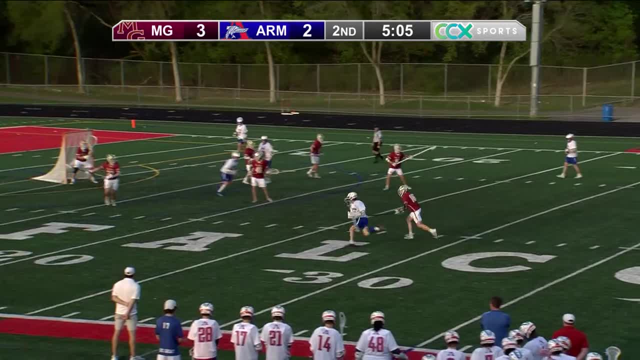 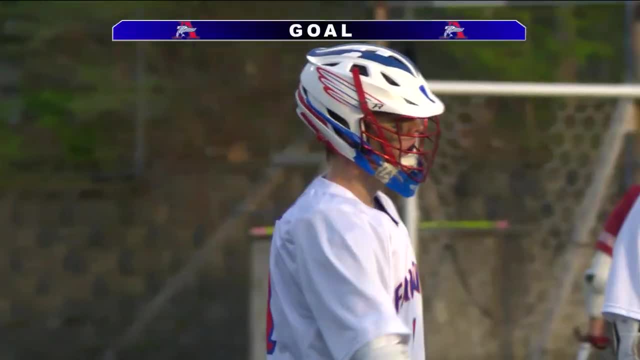 out of the box. You're in the five-minute mark of the second quarter, Sneaking around from X and they score. It's Frankie Annis, goal number 20.. Or, beg your pardon, goal number 21,, as he has his second of the second quarter. 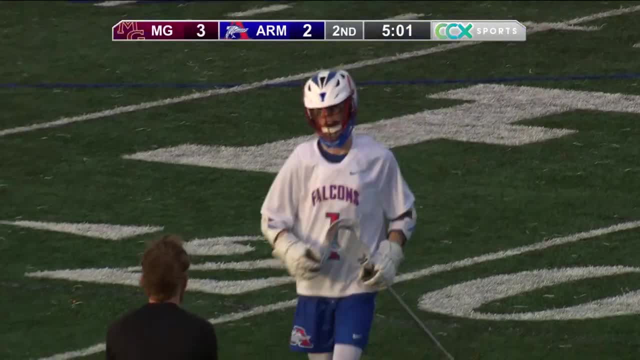 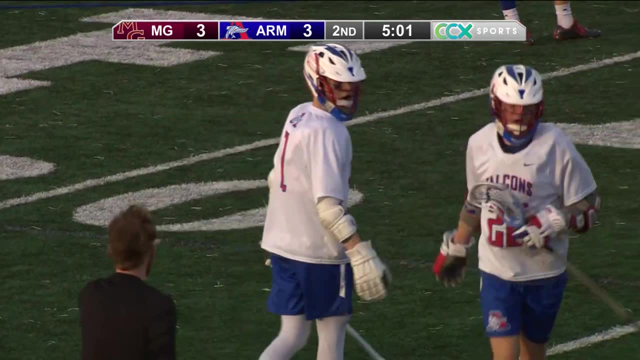 And once again we're tied And these two teams just keep trading goals. He was wide open too. They made a nice play finding him. Maple Grove pressed up top with the long stick, but that pulled it away from down low. 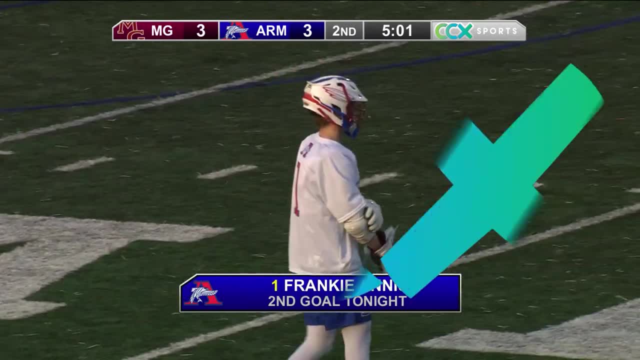 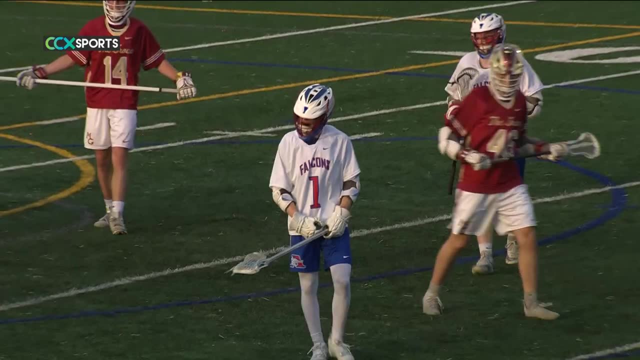 Frankie Annis got open and by God you don't leave him open because he'll put the ball in the back of the net here. Albrecht drew the slide, as you saw there 27.. Jackson Bennett coming over to help and right there. 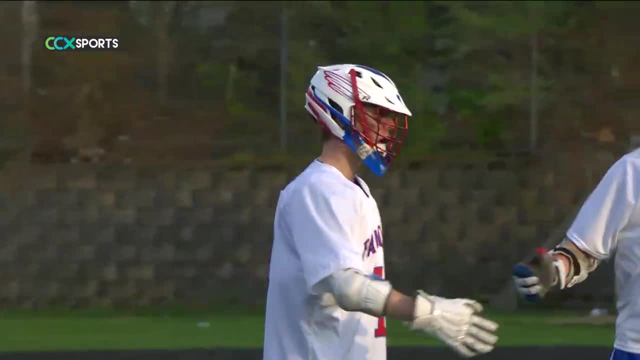 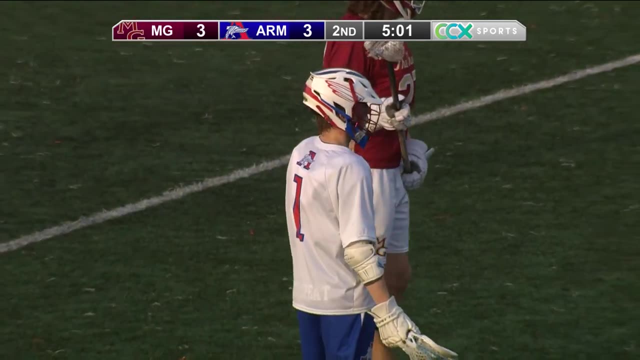 And again Maple Grove enjoys the lead for about a minute 20 before we're tied again at 3-3.. And that's the thing about Armstrong. Every time Maple Grove scores, Armstrong seemingly gets possession on the faceoff and then can do things like that. 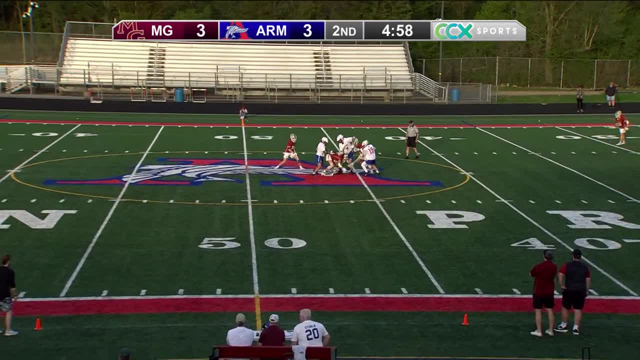 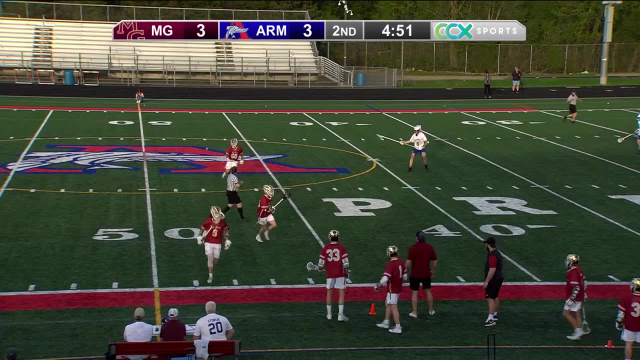 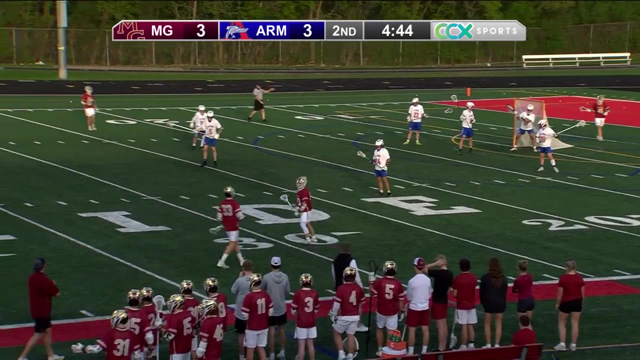 A lot of lacrosse left to play, though Another whistle stops playing. It goes the way of Maple Grove. Annis with a couple goals, tonight, Bakke with a couple goals. You know guys that have good numbers, but not necessarily the top, top guys. 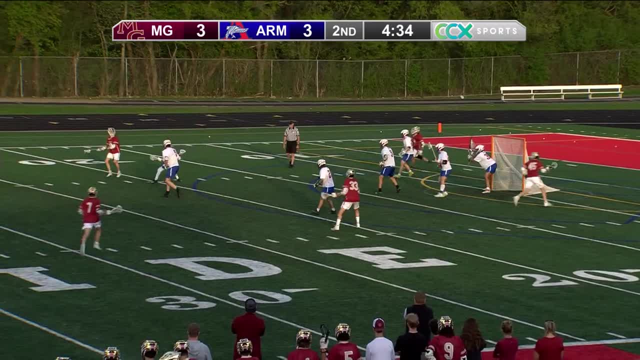 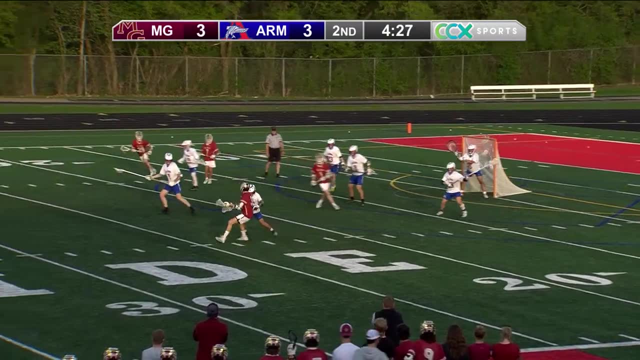 And everyone getting involved offensively. as Peterson goes back for Scanlon. If you're going to get involved in this game, everybody's got to pitch and do their part and do what they're supposed to do. Brendan dodging Tries to feed it outside. 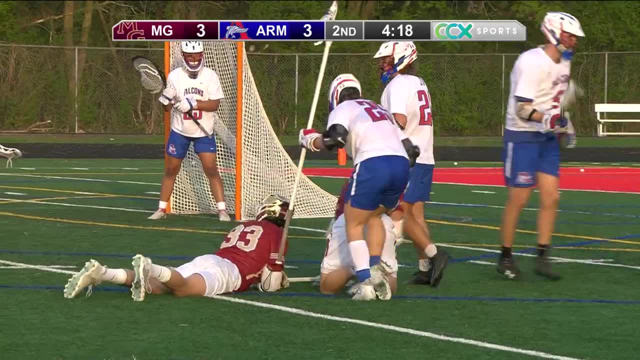 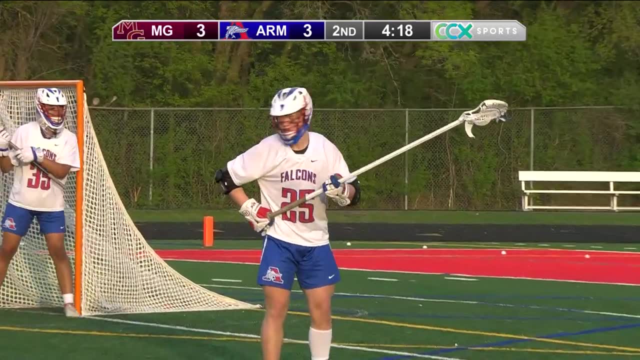 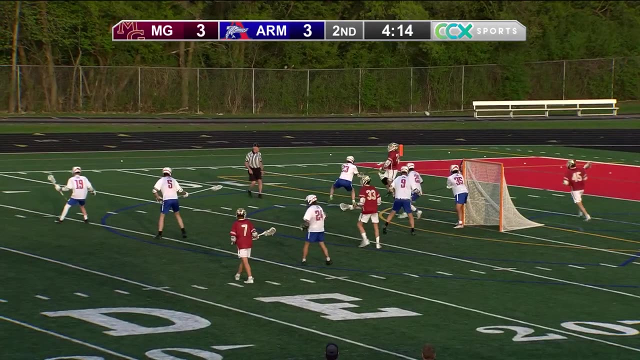 Ball's loose, I think Got crunched between a couple defenders. Looked like a chip shot That held a green. Yeah, Great backspin on it. It remains with Maple Grove, as Peterson reenters play Easy to spot from far. 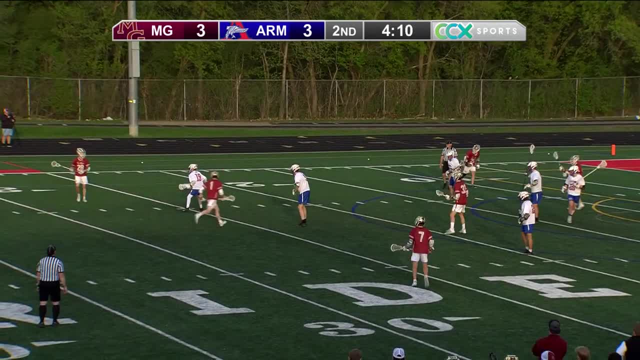 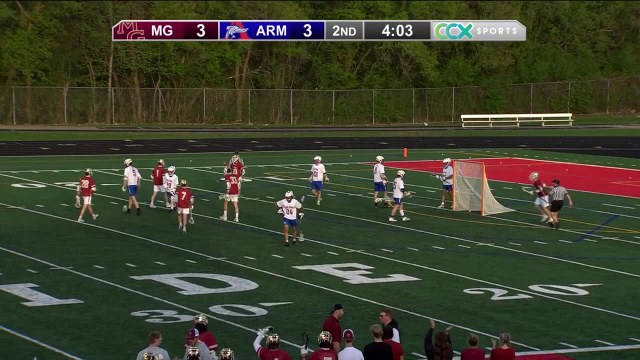 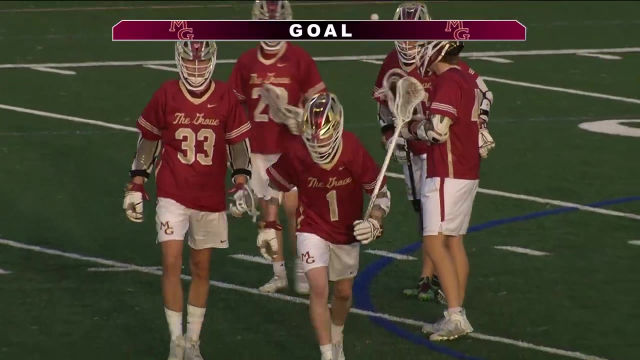 He's got those distinctive green shoes, Scanlon, with the short stick on him, Turning, shooting and scoring. Not the angle you'd expect Tyler Steinkopf to hit the net from, But he bounces it home And it's his eighth of the season. 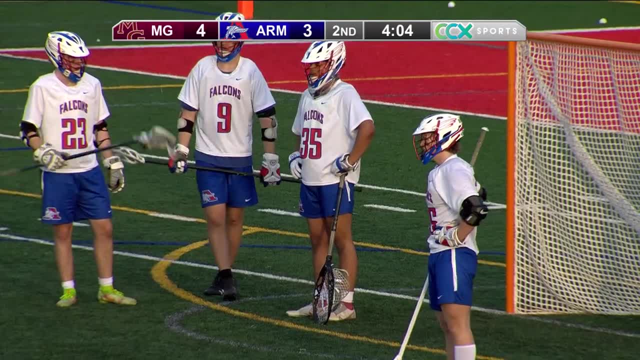 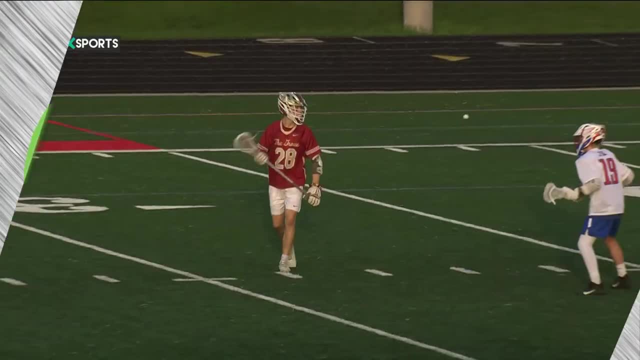 Maple Grove regains the lead. Usually you don't encourage a shot from out there, but there can be no yelling at him because it went in the net. But a bounce shot can be really difficult for a goalie to save And Scanlon gets his third helper of the night. 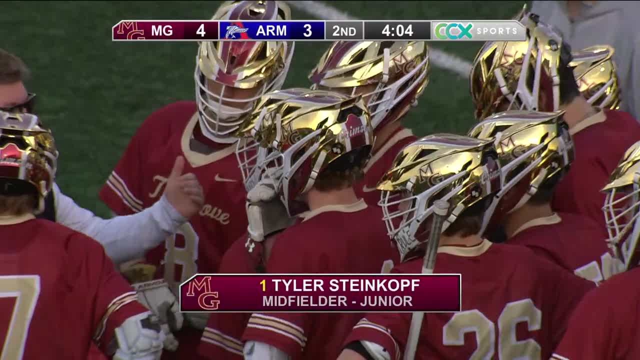 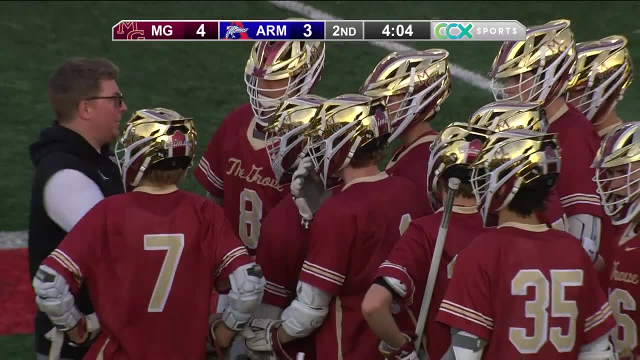 So Scanlon now with three assists and a goal And, interestingly too, neither team has taken a timeout, though they both have too. We haven't had that sort of contested possession where you often see timeouts taken. Well, you know, both teams are playing really good. 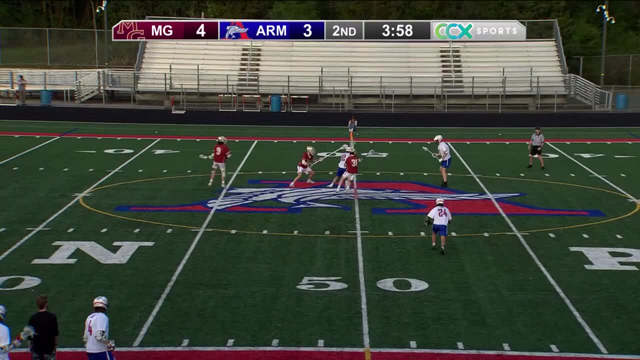 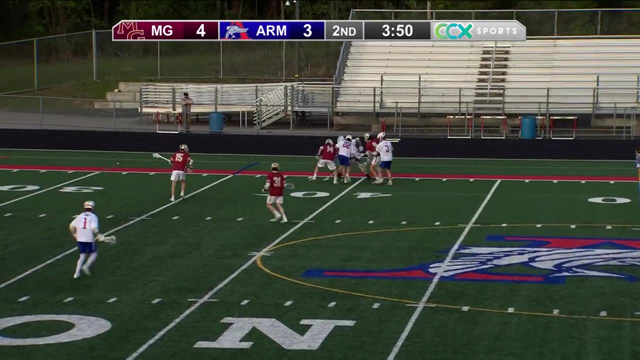 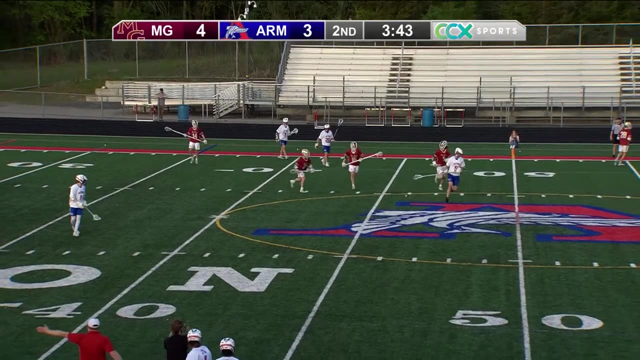 There really isn't any reason to call a timeout right now. Just keep encouraging the kids, Keep playing, And we'll see what happens. Essen had possession momentarily. Then he had it raked away from House out there as well. Great, Scoop it up and may have stepped up. 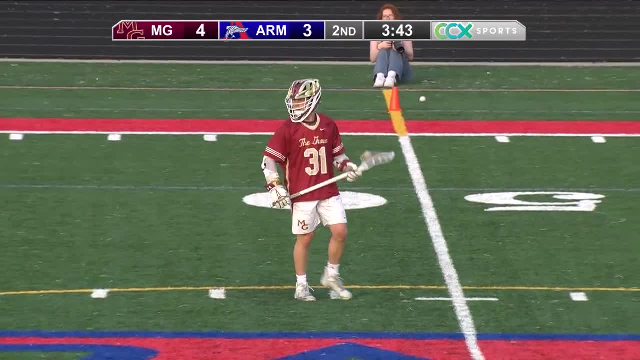 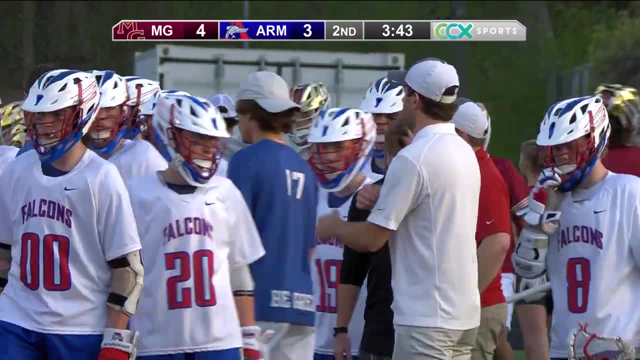 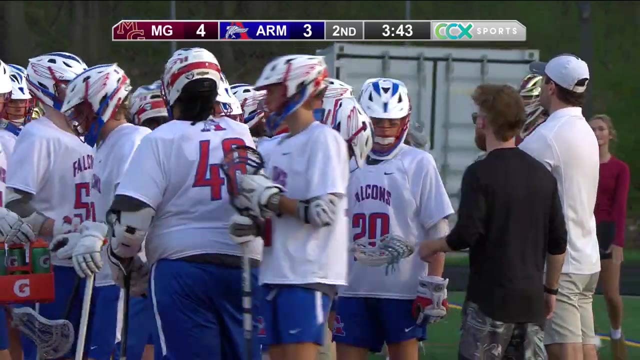 I thought maybe that Armstrong would have taken a timeout, but it goes back to Maple Grove. This time we do have a timeout taken. I almost willed that into existence. I honestly didn't even see exactly which team took the timeout, but it'll be Maple Grove's ball. 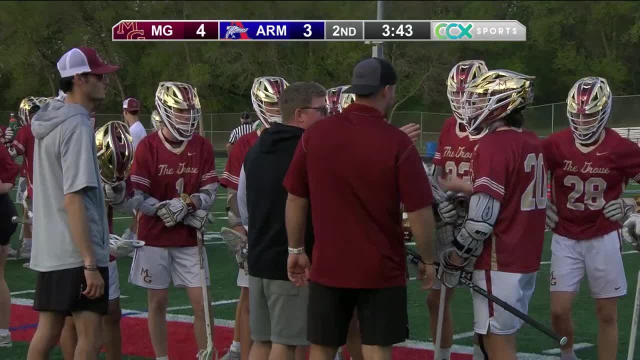 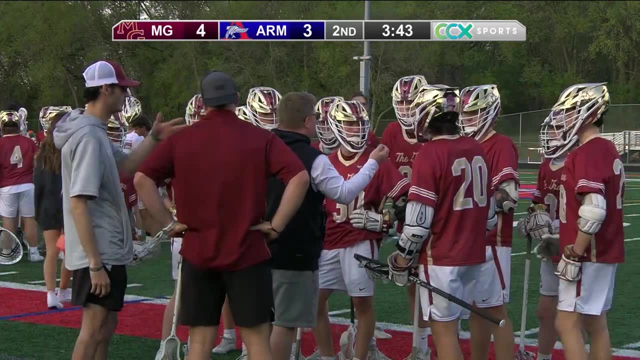 Out of the timeout. Well, yeah, this game so far, Dan has been, as advertised here in the first half, Two of the better teams in the state. Like I said, even though Armstrong isn't rated, they're certainly in their top 11, if any way. 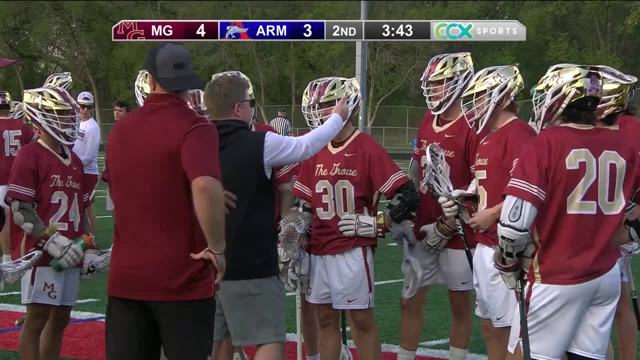 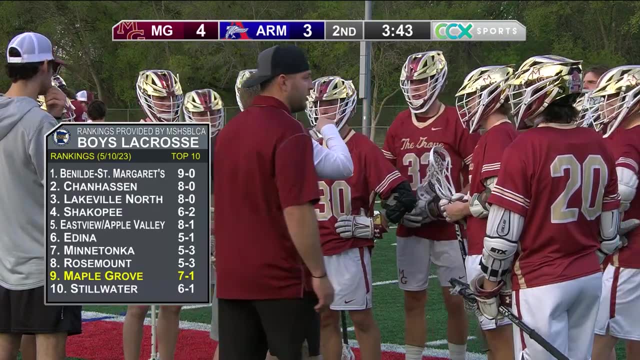 I'll give them that much, But you know this is the big one, though This is for the conference. As we take a look at the rankings in the boys' lacrosse, Maple Grove, number nine, They were five and they dropped down to nine. after that loss to Chanhass 13-6.. But they again bounced back last night in a big way over to Tino Grace And they find themselves in the top ten. But a lot of teams with some pretty gaudy records. 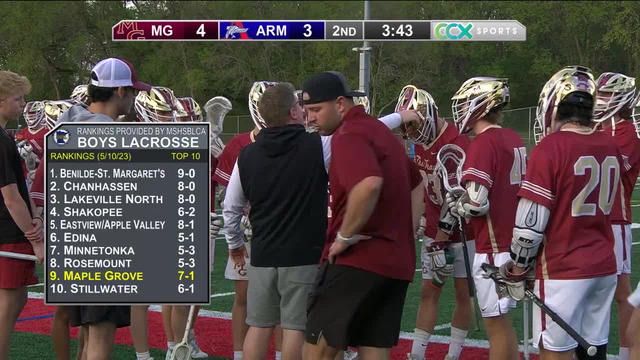 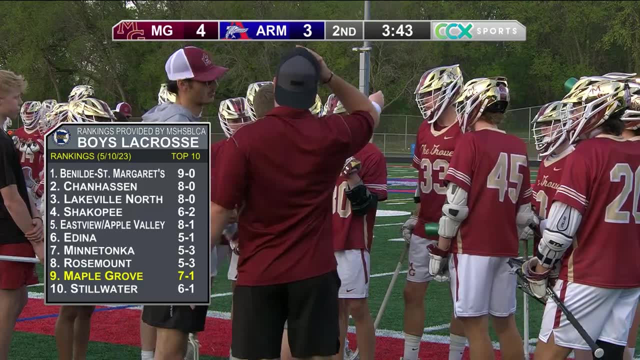 and even like Minnetonka and Rosemount, have just played loaded schedules so far. So I think the biggest surprise on that list- for me anyway- is Lakeville North: 8-0 and undefeated in the top three. They've had good teams recently, but nothing unbelievable. 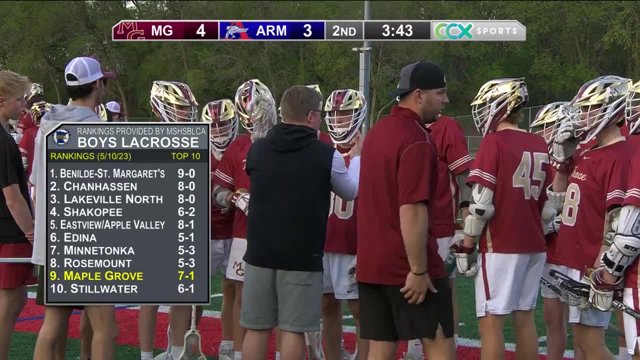 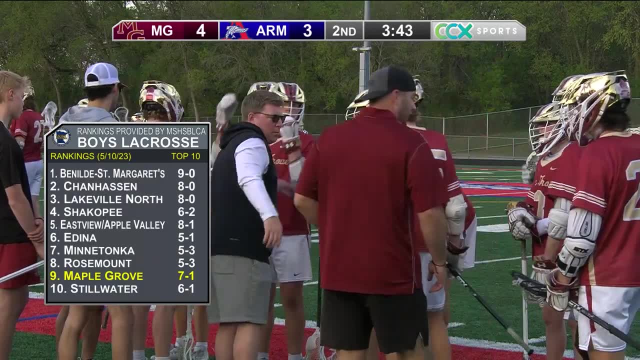 And you know Eastview-Apple Valley, the combined Apple Valley Schools co-op- in the top five as well, coming off a big overtime win over Shakopee the other night. Yeah, and Shakopee is really good. Those two losses are kind of a misnomer. 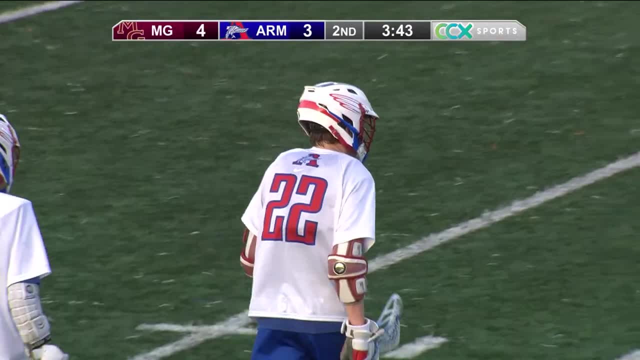 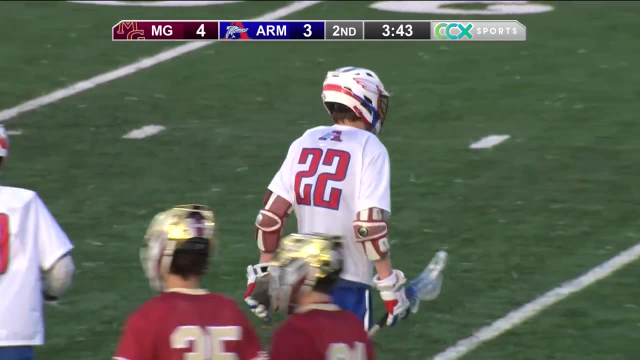 because they're playing that kind of schedule. Yes, and that's the thing. Just even playing in your conference, never mind the non-conference stuff you're going to play- you know a loaded schedule. You talk about a loaded section, right? 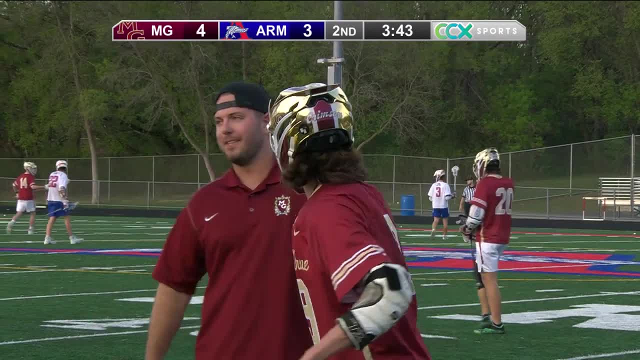 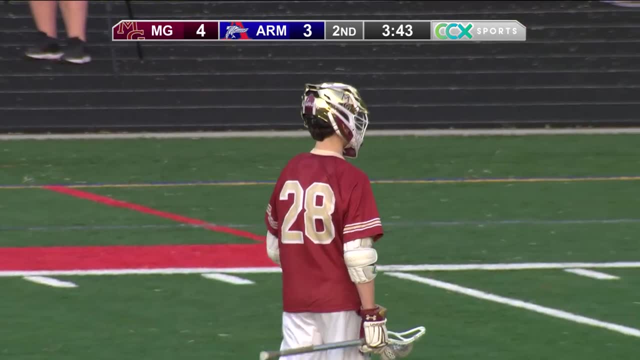 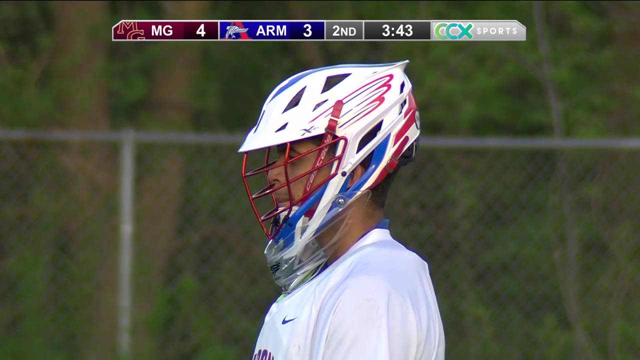 You've got, you know, Edina and Rosemount and Prior Lake. But Prior Lake has taken its lumps so far, losing its first three games after graduating. so much talent from that team that took Bonilla to overtime. Xavier Wells has certainly kept his team in the game tonight. 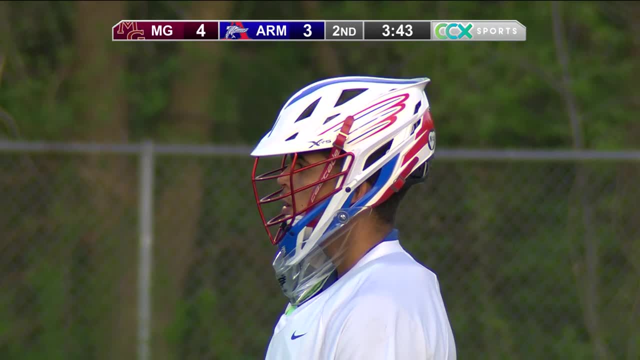 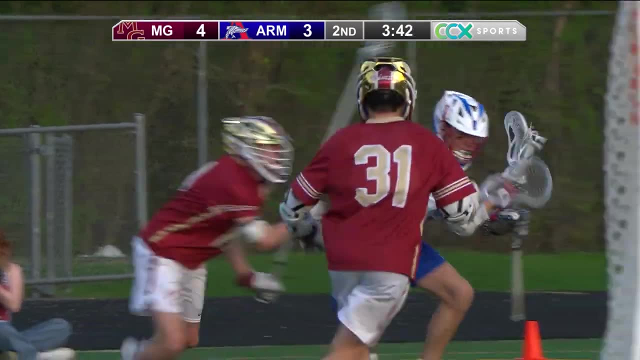 with four, saves a couple of them, incredible. I wish we could see some of those on ESPN tonight, for heaven's sake, because they were fabulous. my gosh, Yeah, they were terrific. As Olsen re-enters play: it's hard to tell just from up here. 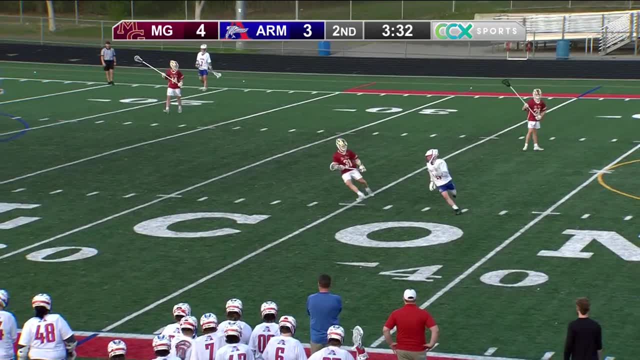 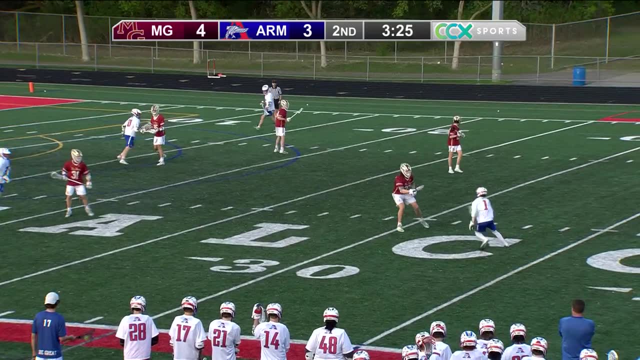 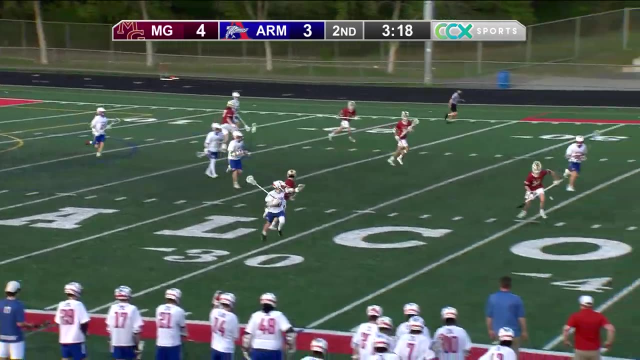 who actually had the ball, So it must have been Robbinsdale-Armstrong that took the timeout. And now the Falcons have it here with inside of three and a half minutes to go before halftime. On a hat trick, there's a shot into Farniak's stick. 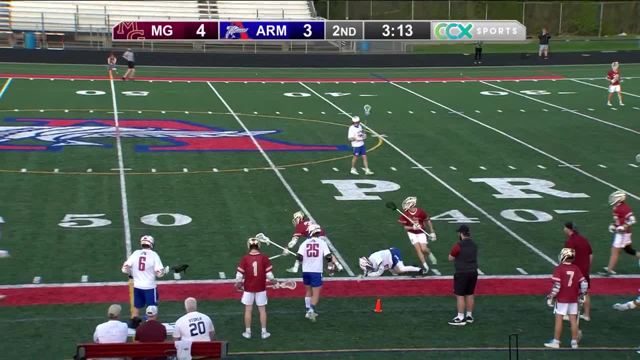 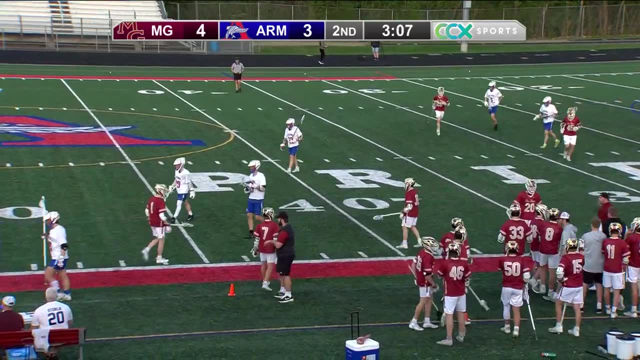 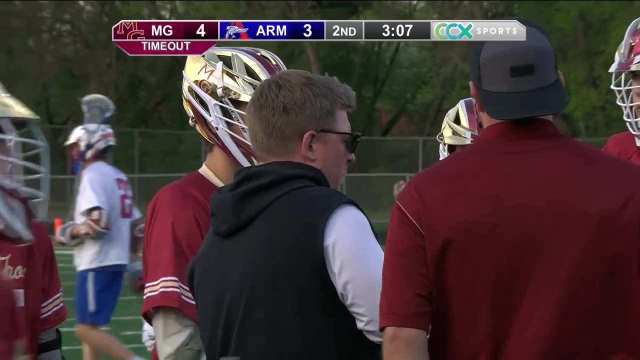 as Frankie Annis was looking for his Third goal of the quarter. Good recovery, and this time it's going to be Maple Grove that takes a timeout. Yeah, good call there before they lost possession of the ball. Yeah, and that's exactly what I was talking about before. 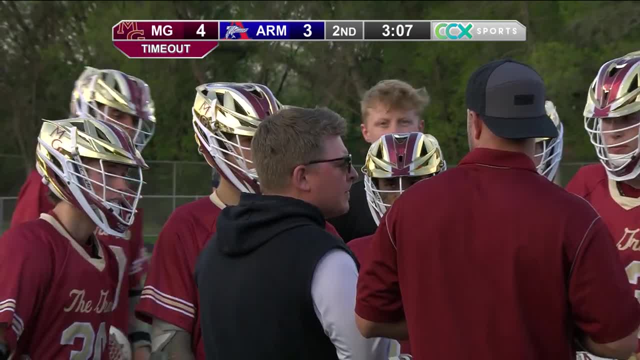 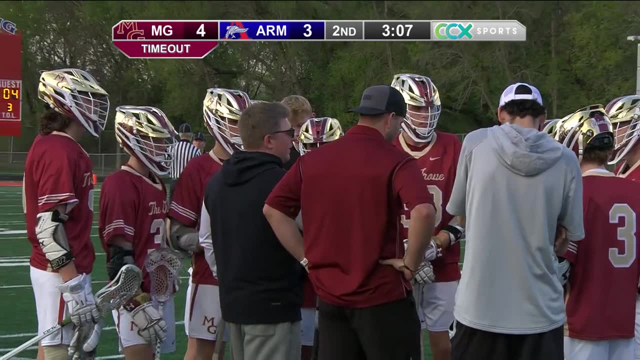 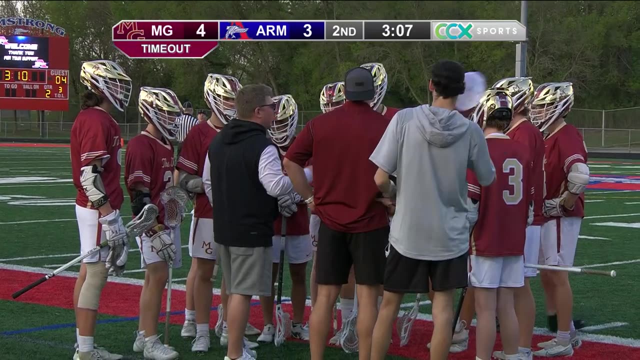 as far as Connor Kasbaum got the ball, They tried to retain possession on the clear, and that's when you take a timeout. Each team left with one timeout- One timeout remaining. We'll see if they actually use it here, but what a gorgeous night. 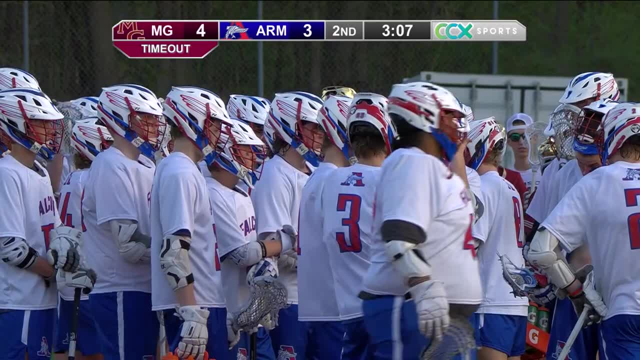 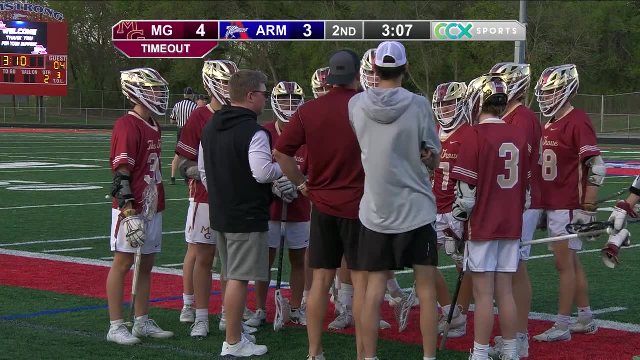 Beautiful, beautiful night for La Crosse. The clouds have cleared, but it's been sunny most of the day and temperatures were really nice, and it's only what these kids deserve after so much tough weather in April. Yeah, absolutely No practice time. 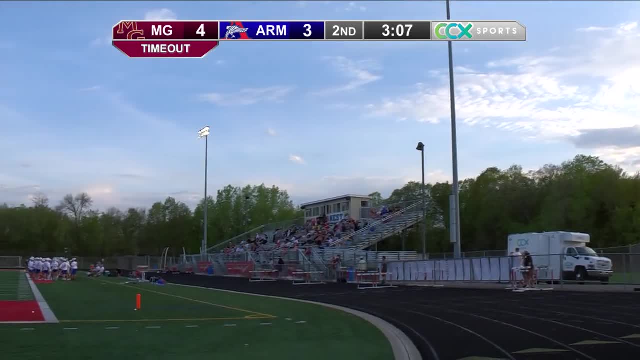 It was really hard to try to get some dome time out in Maple Grove. I know for them and you know. 10.30 at night, for heaven's sakes, Yeah, no, it's like ice time in hockey, right. 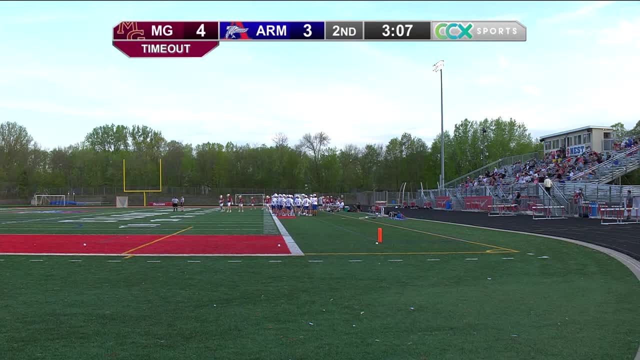 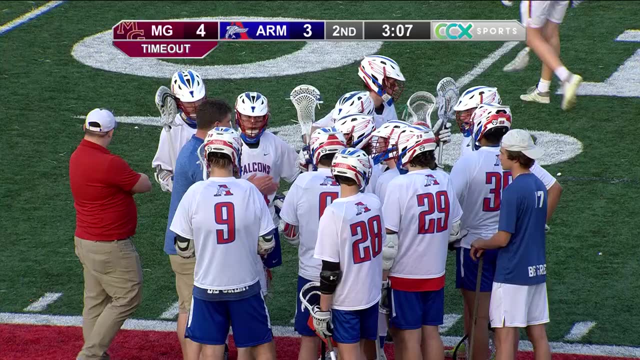 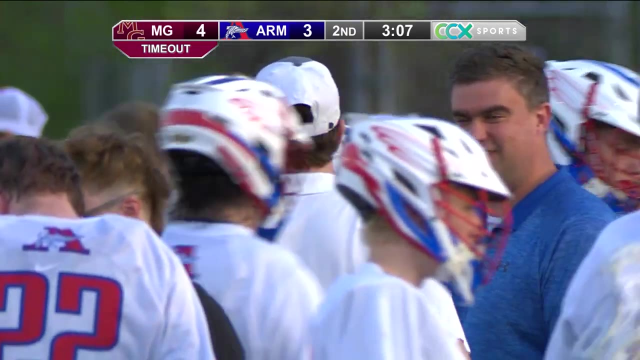 There's only so much space available and you kind of need it, and so you do what you can as a coach, and especially a new coach like Coach Ficken, coming over from Rogers after eight seasons leading the Royals, Has to be thrilled with how things have gone so far. 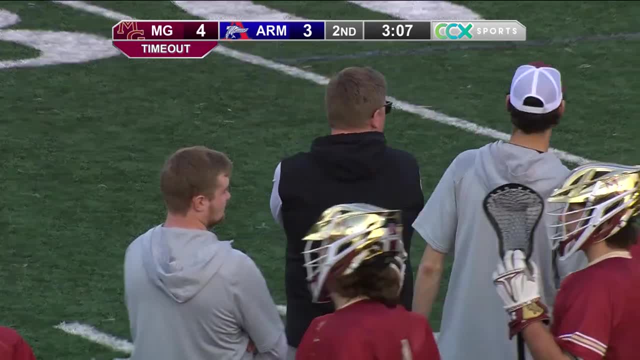 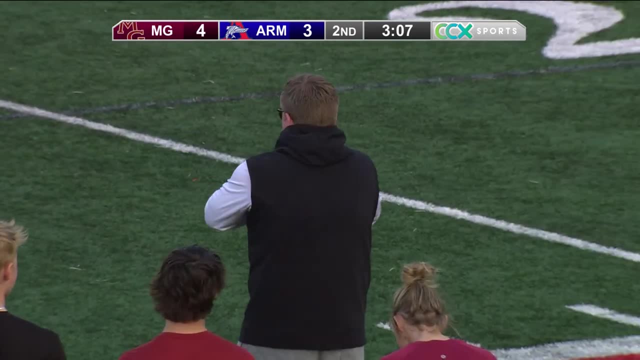 Seven and one winning everything they've been expected to win. and, And you know, all but two of their games are conference battles, so they only can do so much there. and then And then, of course, their non-conference games. 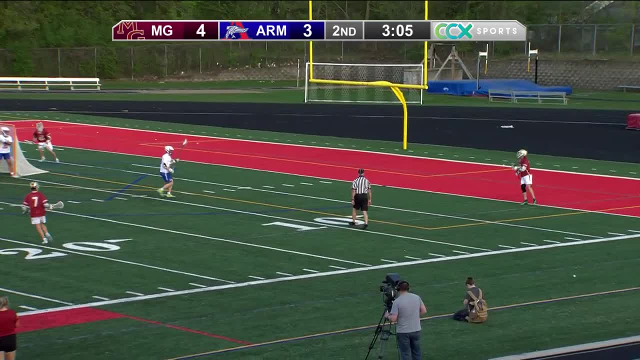 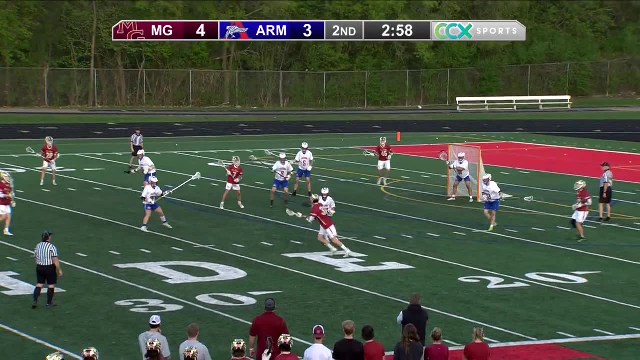 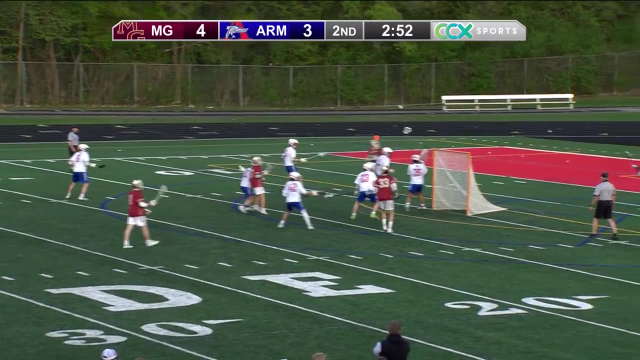 one of which was against Chanhassen, which has turned into a real perennial powerhouse. Peterson from X, out high Scanlon on the far side watched by the short stick. They get it to Peterson. Peterson at X- Opportunity here. 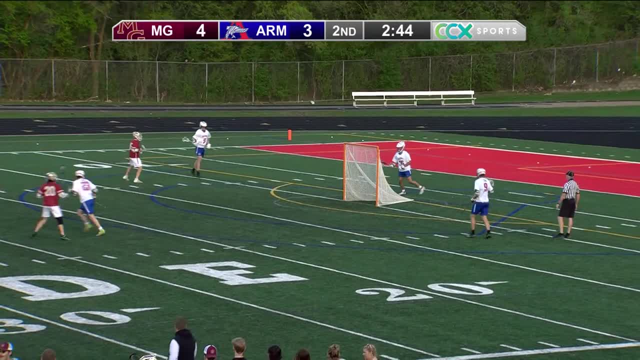 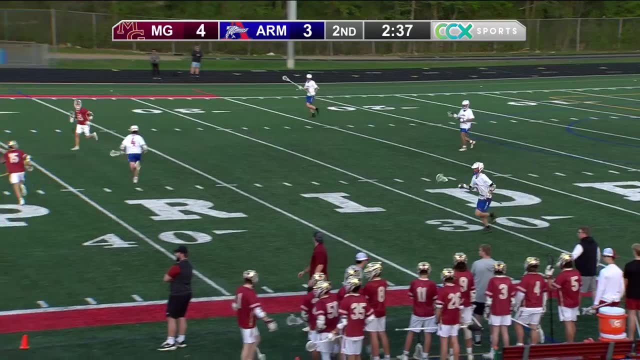 and another big save by Wells to stop Brendan who had a good look at goal from from close range. Boy Wells is quick with that basket, though I'll tell you a straight-on shot probably is not gonna beat him there. 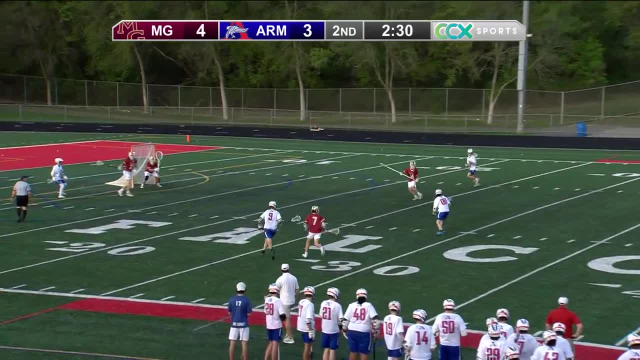 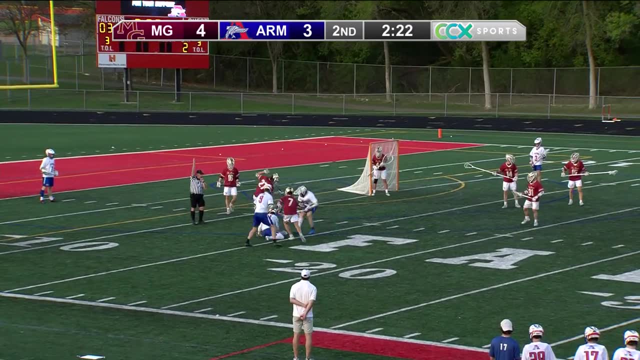 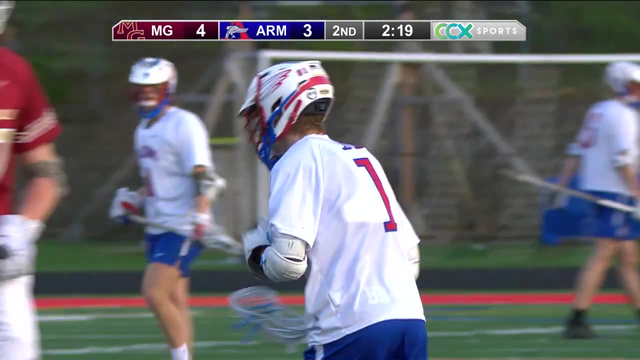 You're gonna have to bounce it. Keep wanting to call it a butterfly net- That's probably not the technical term. but transition opportunity here. Bounce shot Farniak this time With his turn making a big save. the hold with possession keeps it. 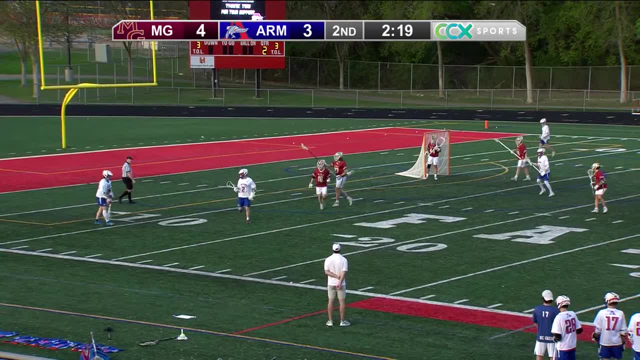 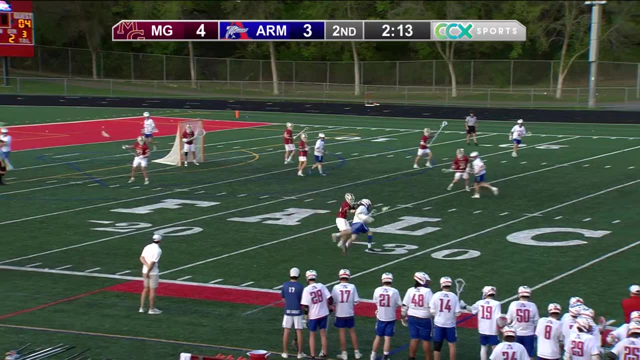 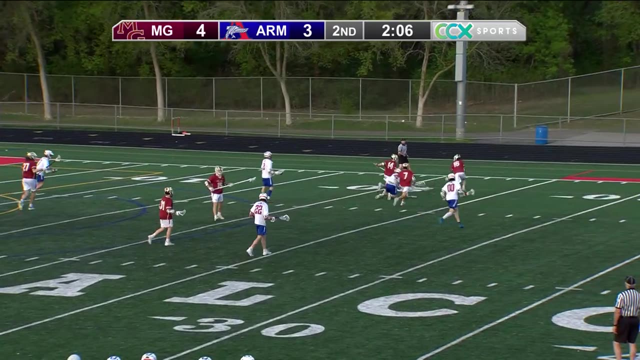 Yep with Robbinsdale-Armstrong As they'll flip it to Nate Albrecht and Albrecht goes to work. Albrecht, shadowed by Rask, Big slide coming over from Josh Thompson to dislodge the ball. 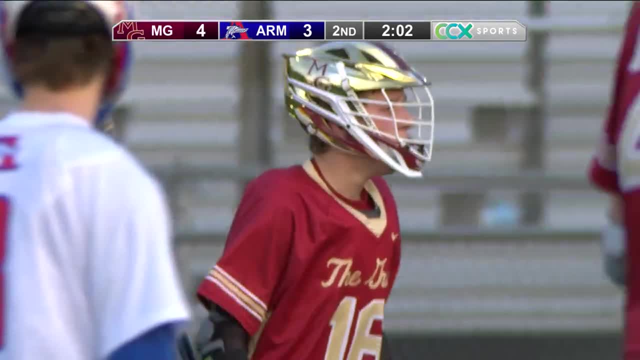 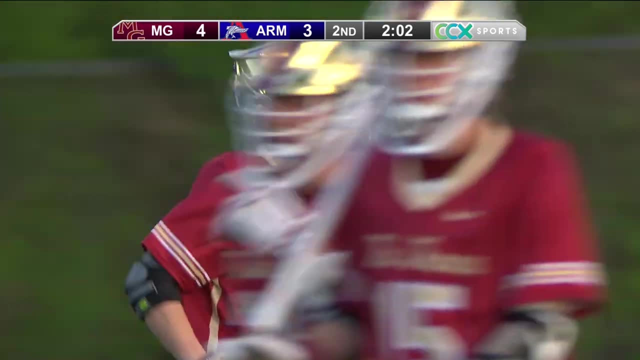 Now a flag comes out and Maple Grove, I think, is just gonna have taken its fourth penalty. So that seems like a fairly tight whistle tonight. as Rask Yep takes that one, No doubt Coach Ficken, He's not happy, trust me. 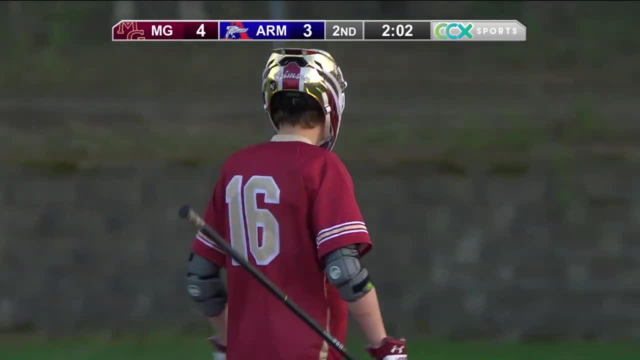 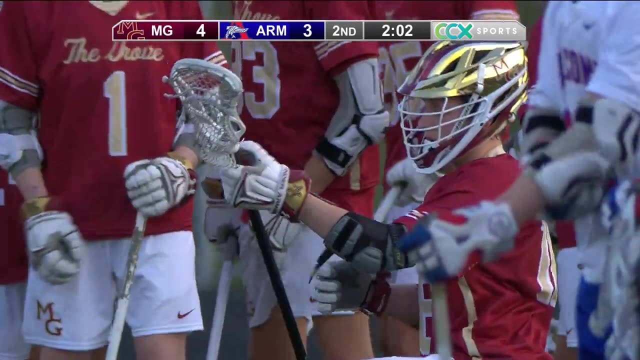 Yeah, He's frustrated at either the Raps or his team for taking those penalties. He's getting a little red around the cheeks. That's a bad sign. But you know there went an explanation. this time He lets the assistant coach handle it. 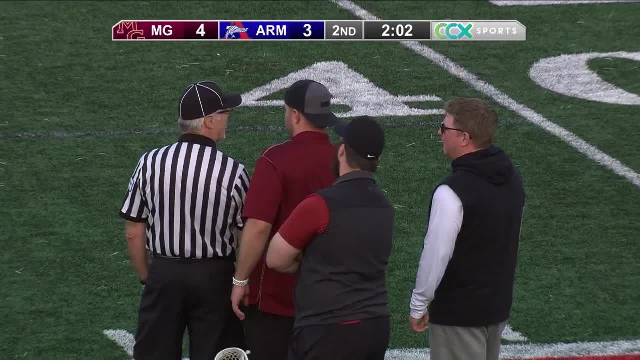 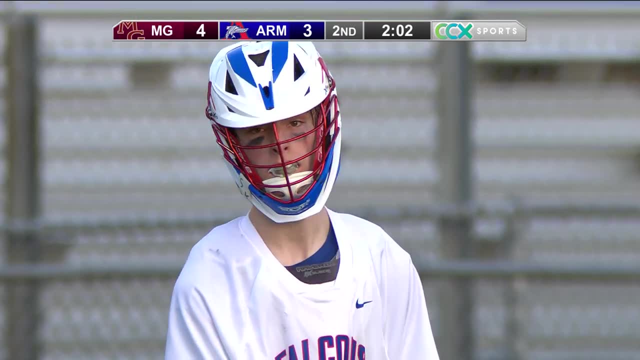 He's gonna stand beside it. I think he's a little too irritated, which is smart thinking, But it is what it is. Holding is the call. and really, Robbinsdale-Armstrong has not scored with the extra man tonight, but you can't give a good team. 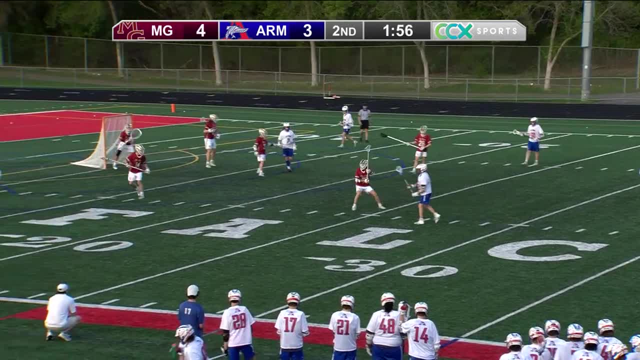 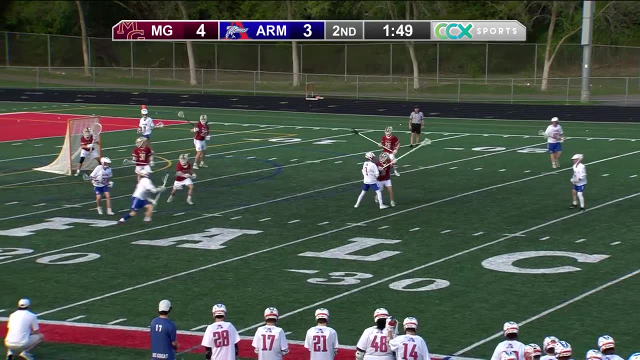 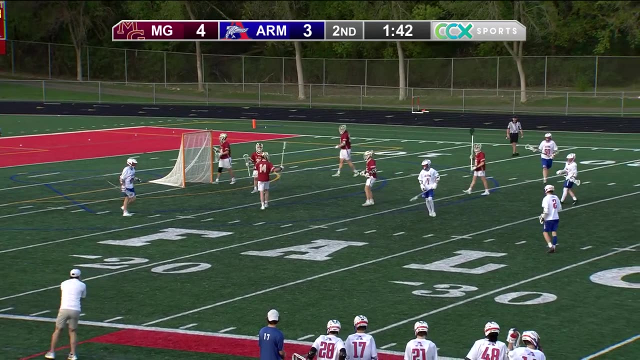 like Robbinsdale-Armstrong. too many EMO opportunities Exactly before they'll make you pay Annis on a hat trick. A little wheel route for Albrecht. There's a shot that goes wide. Brady Northrup looking for his ninth goal. 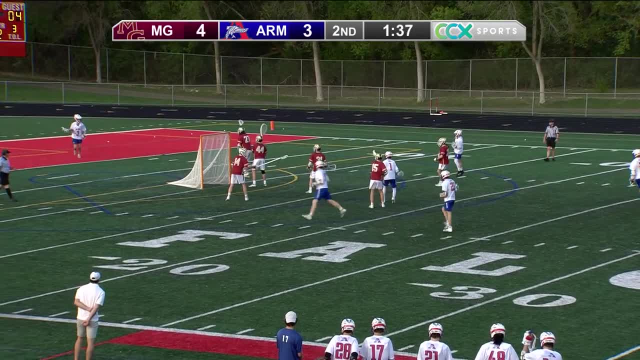 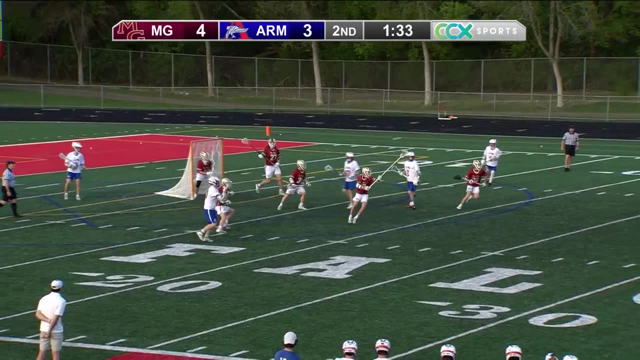 Another freshman, So Northrup and Jack Olsen- both freshmen giving this Armstrong team valuable minutes, Which means it's gonna be scary for the next few years too. with Armstrong They're gonna be pretty doggone good because they're good now. 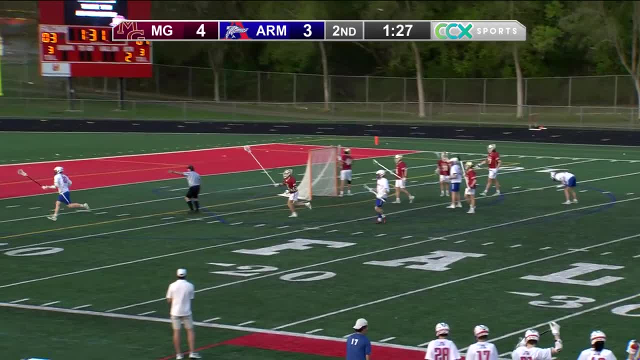 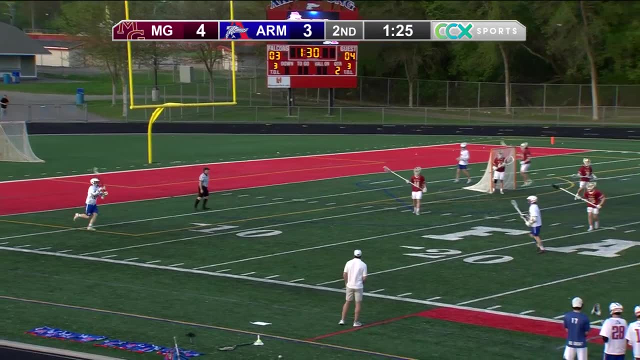 Yeah, no question. There's a sharp angle shot and that one, always going high, Stops the clock with a minute 30 left in the half. Well, what I like about him too, and being young as they are, they're very aggressive. 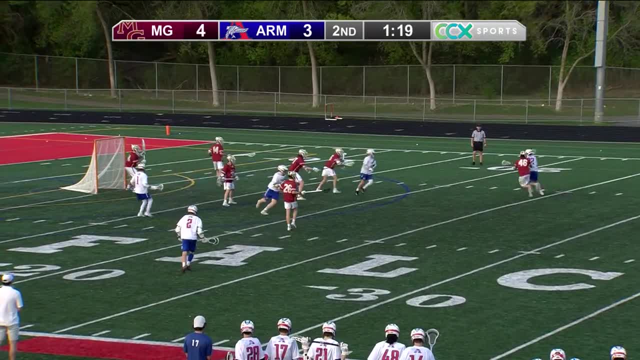 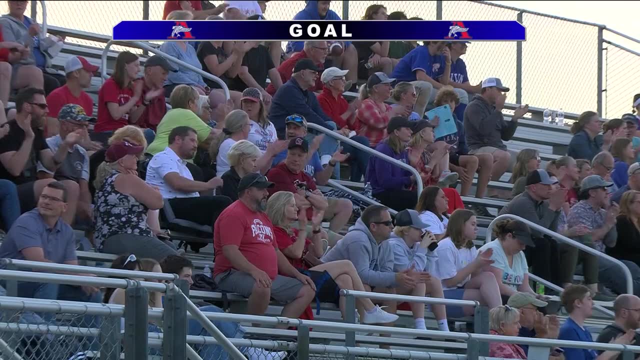 and I love aggressive players. I mean, if you're gonna make a mistake, make an aggressive mistake. Essin somehow beats Farniak over his right shoulder And we're tied at four with that EMO goal. Low-high shot. 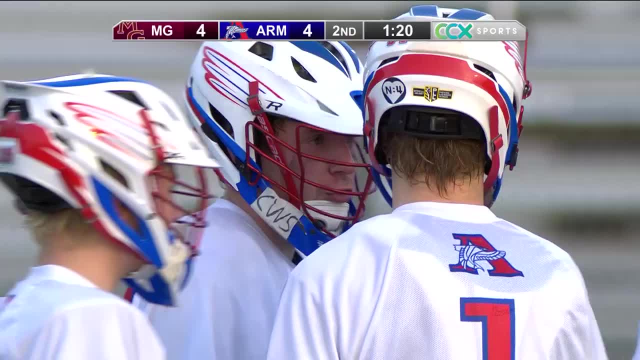 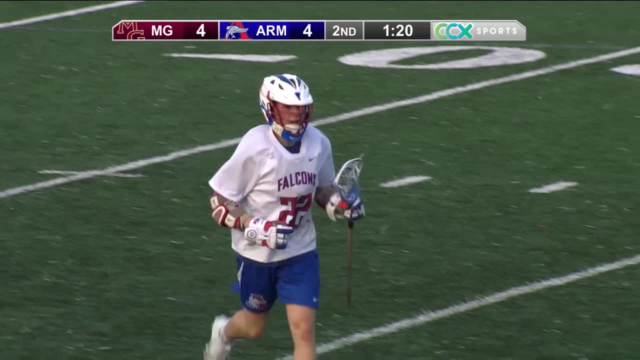 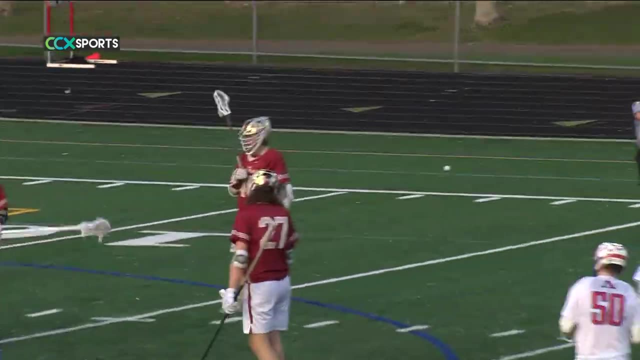 Found the upper part of the net. Just a really good shot. He got a lot behind it, Created some room for himself And made a nice play and scored Essin his second of the game- Unassisted. That one there first on the EMO. 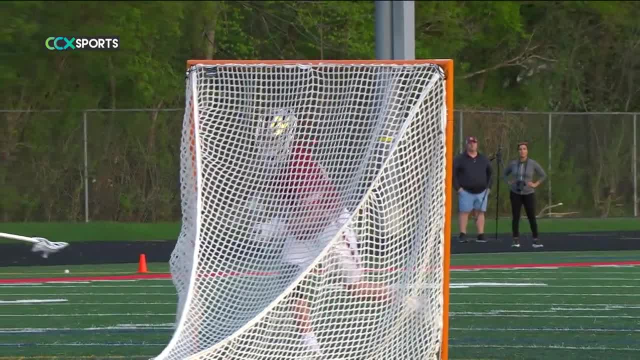 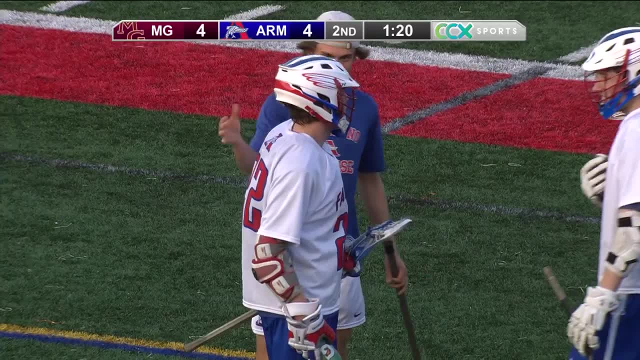 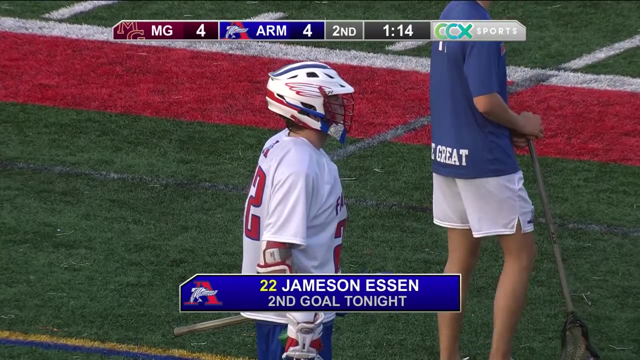 With 1.20 to go in the half and it would not be at all a surprise if we were tied Essin, a modest celebration. That was a heck of a shot. That is a hard shot to complete, Yes, Difficult save for Farniak to make. 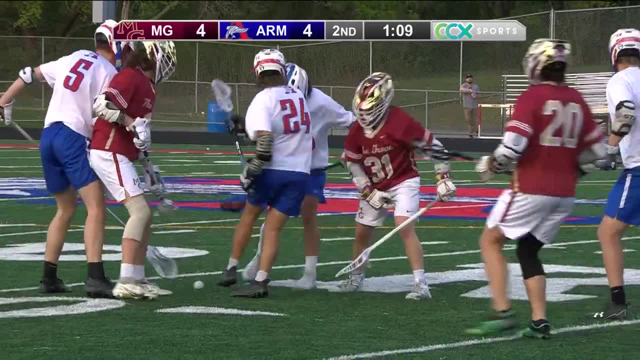 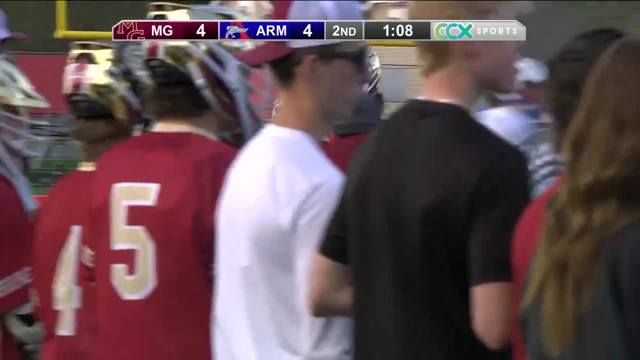 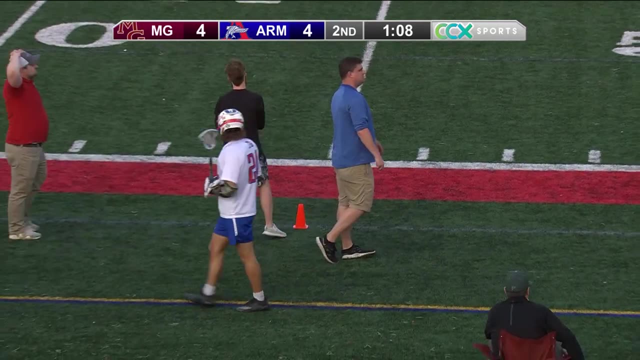 no question, No flag out. but well, no, there is a flag out. Got some Maple Grove parents here in front of the Pest Box Finally going, finally, finally. Yes, Oh boy, It's gotta be a penalty. 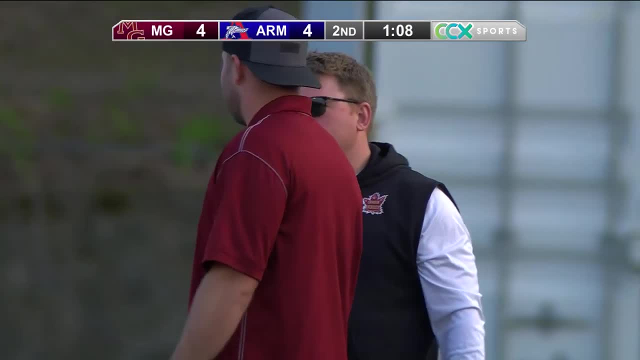 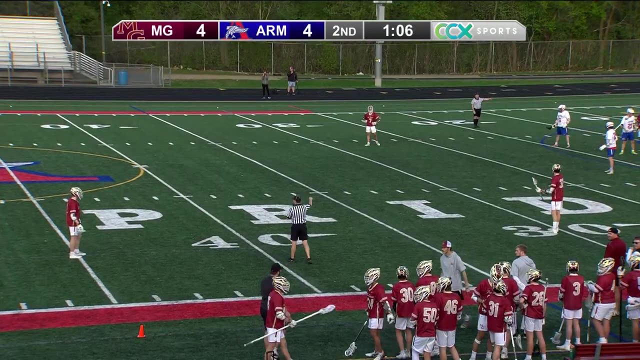 Come on. Well, good opportunity for the Crimson here, though with a minute six left, to kind of get take a lead again, And so they got the extra man. We'll see what they do with it. Essin Berry committing the infraction. 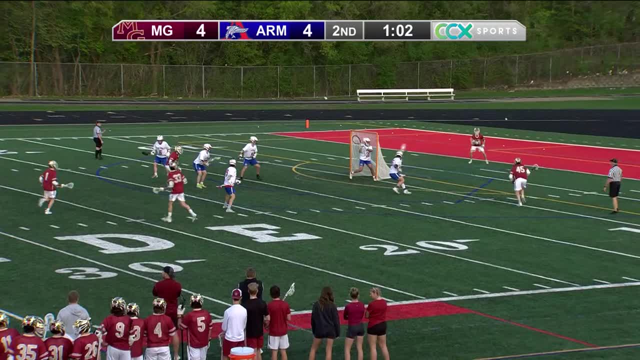 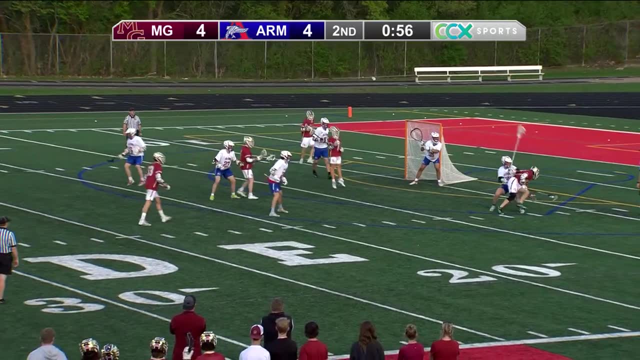 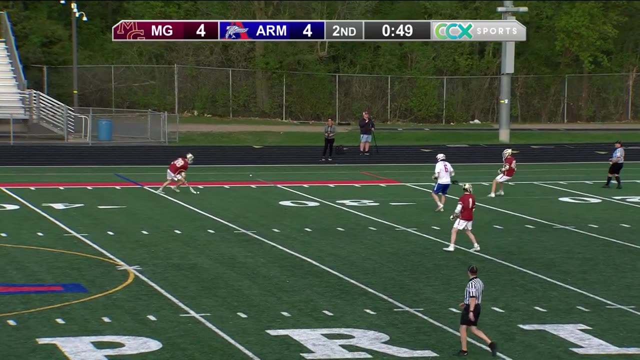 the sophomore defenseman. So Brendan and company go to work with EMO with a minute to go. So the penalty will expire right at the end of the half as Peterson flips it around back out. Errant pass will be collected by Scanlon with 45 seconds. 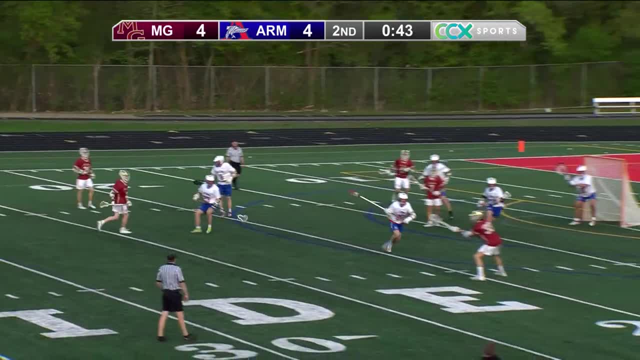 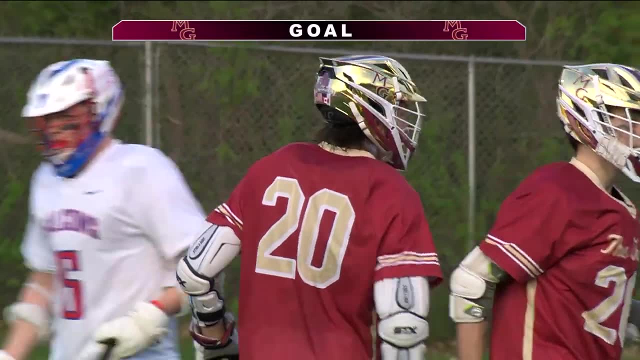 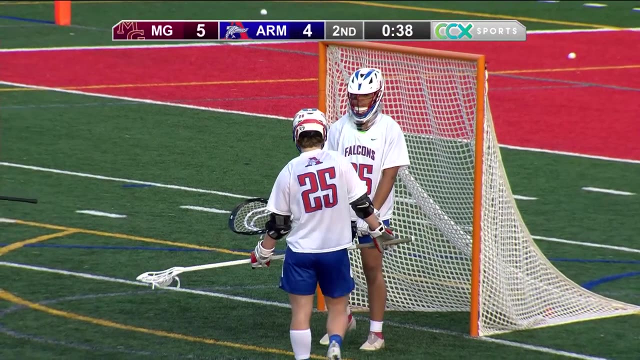 and counting left Steinkopf: Brendan Peterson jumps out scores. Maple Grove regains the lead with 37 seconds to go before half. Boy, what a great shot that was. He beat to the upper short side high corner to beat Wells on that. 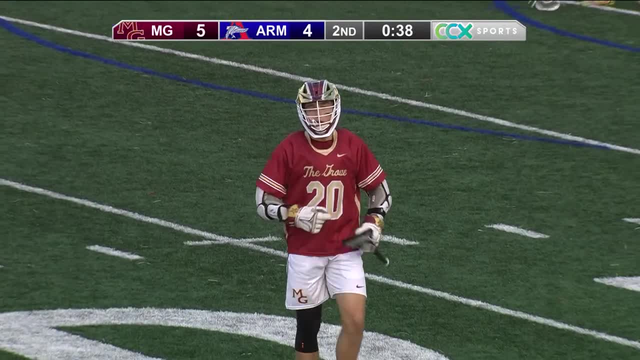 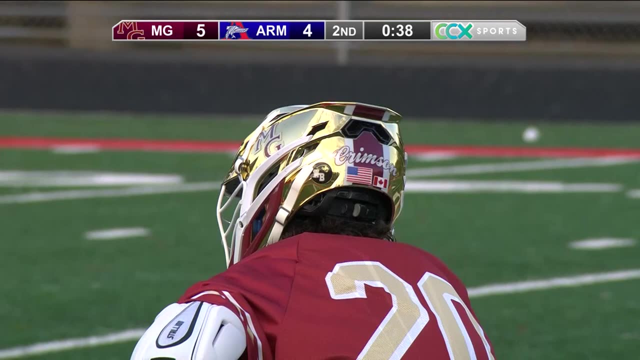 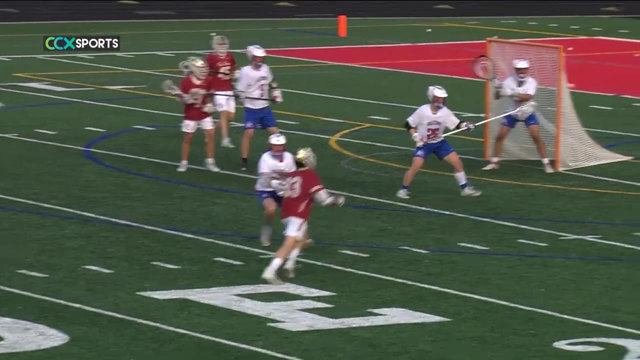 And that was that great shot. There wasn't much Wells could do about that. That was just ripped. Yeah, that was a. that was a tough one. Another EMO goal for Maple Grove, their second of the night. Give the assist to Brendan. 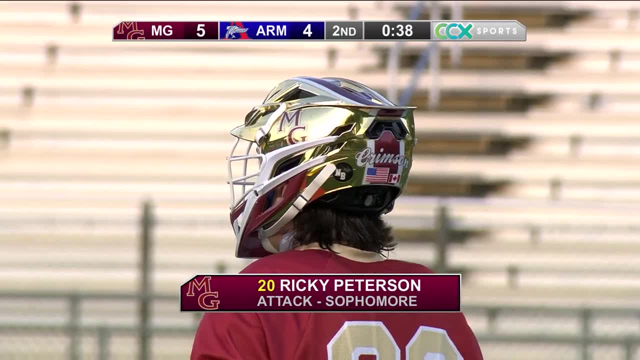 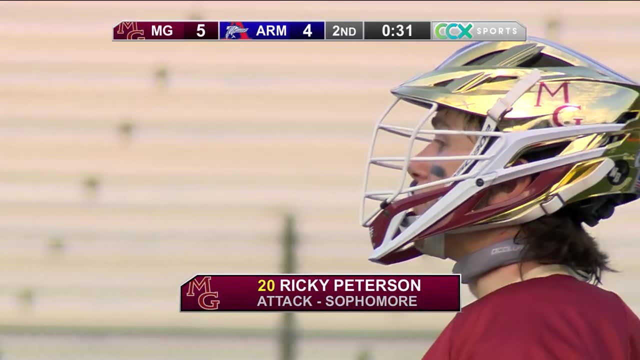 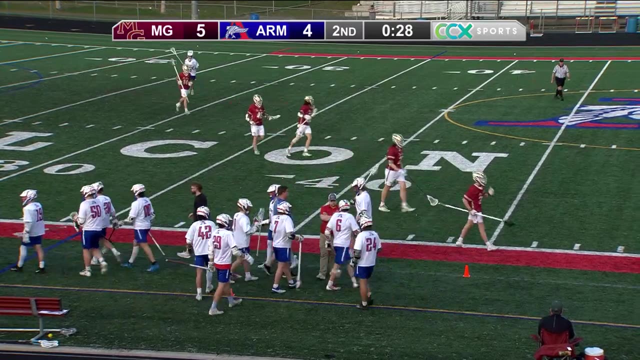 No, I don't think they actually did give the assist to Brendan, but Ricky Peterson, goal number 25 of the season, his first of the night, And that gives Maple Grove the lead with as Robinsdale Armstrong wins the face off and then takes timeout. 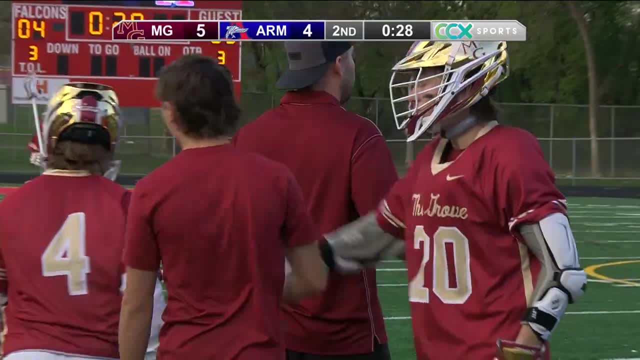 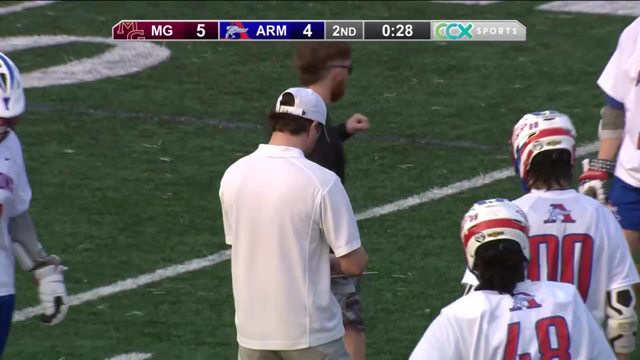 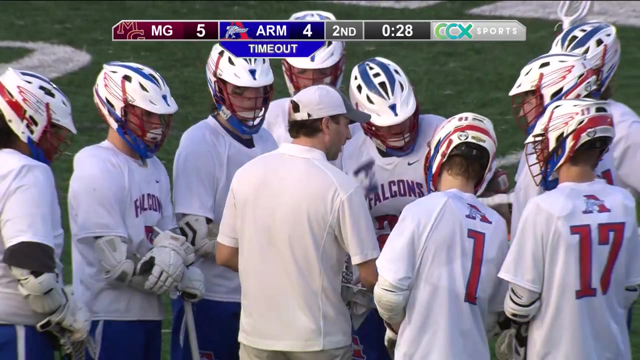 Robinsdale Armstrong tries to answer With 20 seconds. 28 seconds left. Yeah, perfect use of timeout. right there. You win the face off, you take timeout, you draw something up in the huddle, and that's certainly what Ian Murphy is doing. 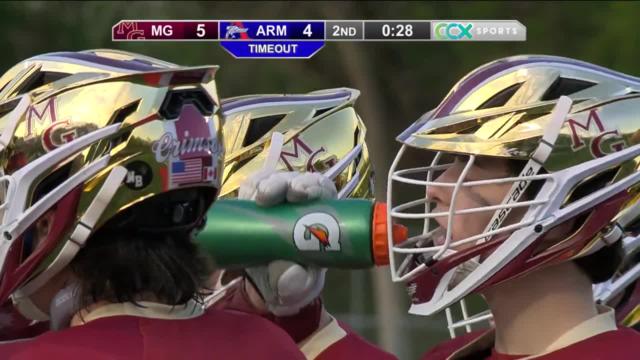 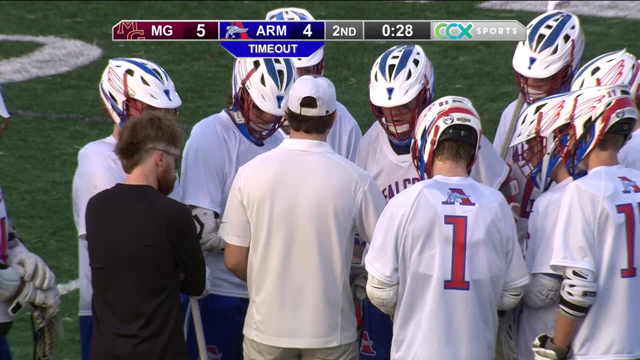 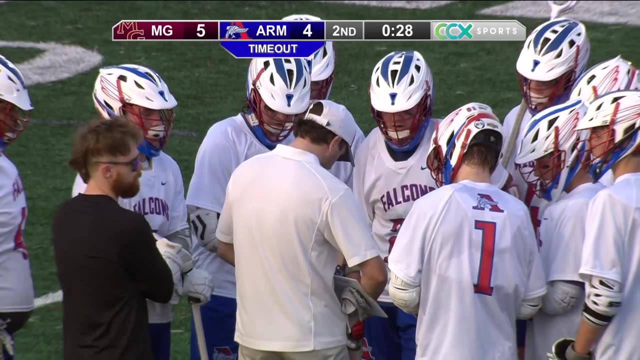 as his boys are huddled around him. And it's been unbelievable. You look at the score sheet. Armstrong started off the scoring, Maple Grove answered with two straight, but then, ever since, it's just been two teams trading goals, And every time. 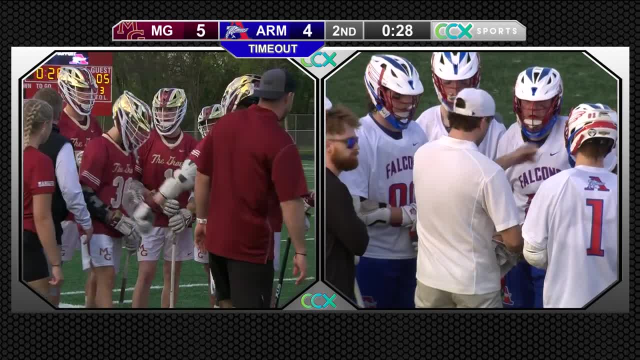 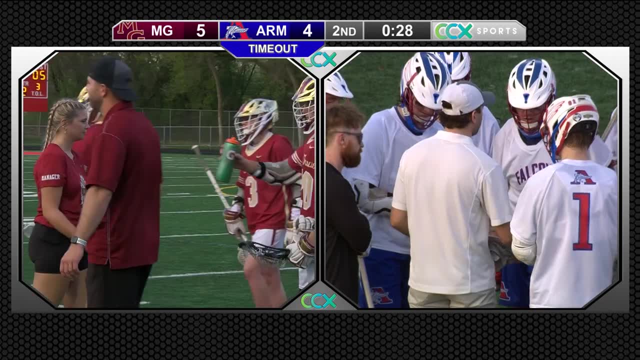 they trade goals and it's just a series of punches and counter punches in this game. And you know, usually lacrosse is really a game of runs. obviously, Dan, but no team has really gone on a run So far. the most, as we said. 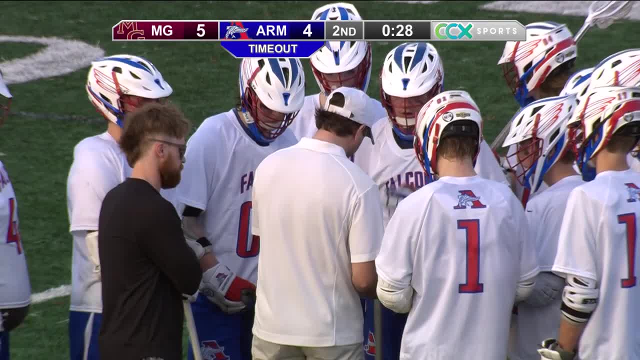 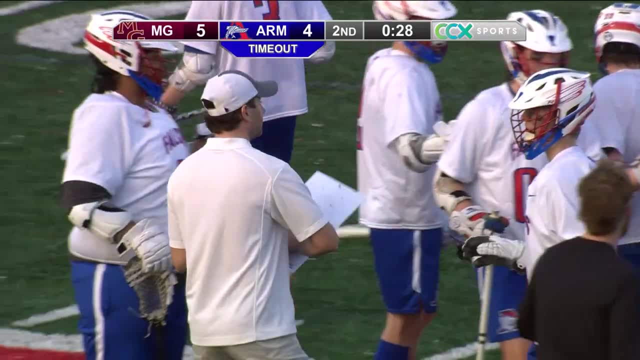 was Maple Grove scoring two straight over the first and second quarters Got a feeling that this is going to go down in the last two minutes and the goalie that makes the save that's needed to be made is going to be the team that comes up out on top. 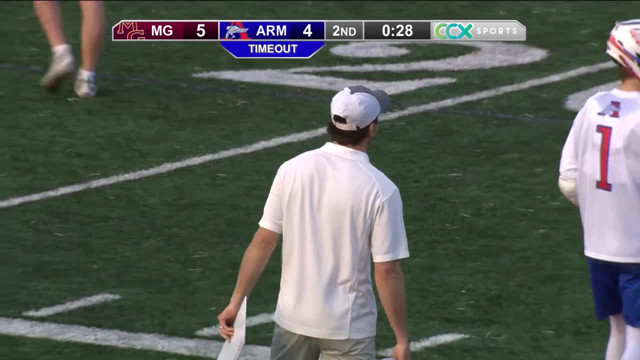 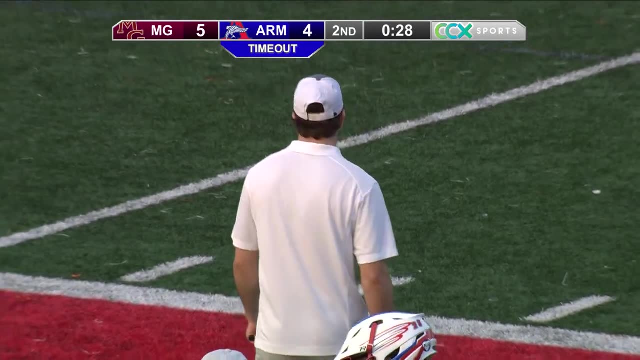 I wouldn't be surprised at all if you were right. Well, as we said before the game started, this is the big one, the biggest one they've played all season. And boy, I'll tell you, both teams are they ain't nervous man? 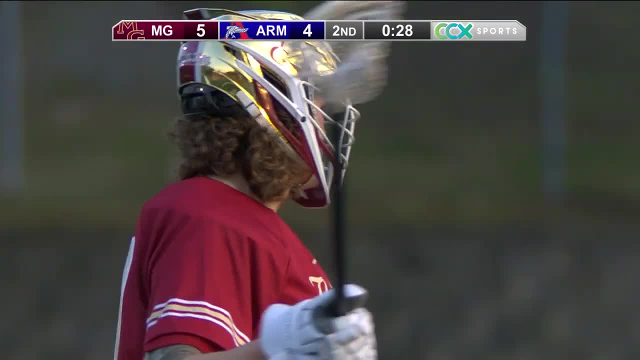 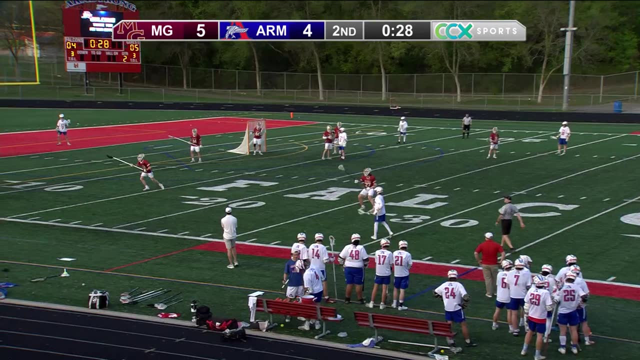 They're playing. It's been good to see No short sticks, no tight grips on the sticks. They're just playing their games, both of them, Yeah, and you don't know, especially with all the, you know- the kids being aware of the stakes of this game. 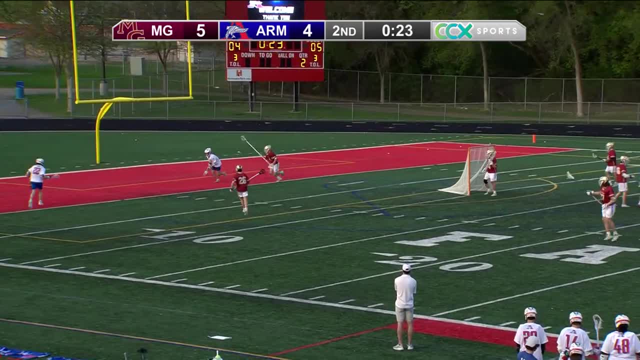 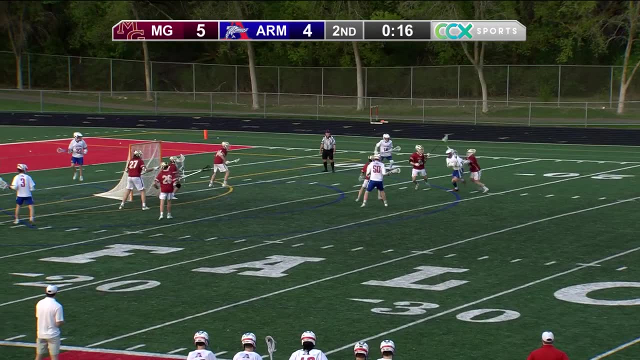 you never know how kids are going to react and how they're going to play. if they're going to play tight, make a lot of mistakes, but it's been a really well-played game and you love to see that Albrecht gets a step dances by defenders. 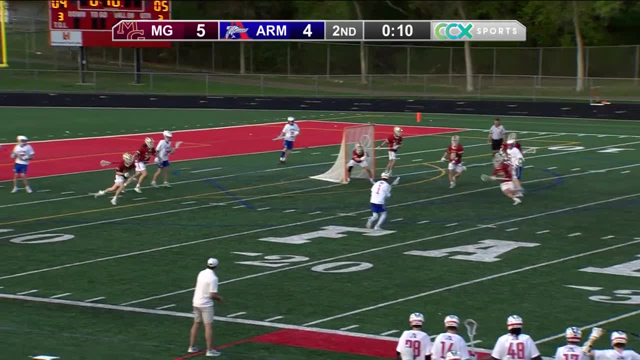 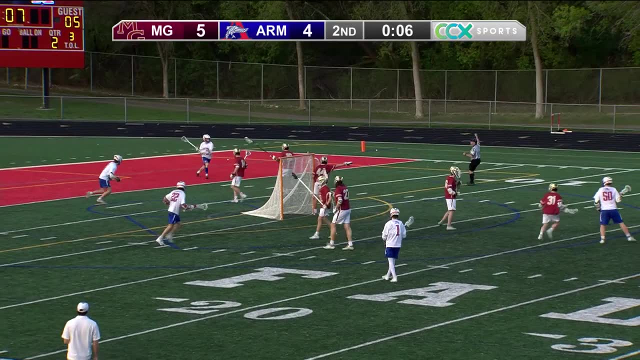 behind the back shot and he misses the net. Maness looking for the hat trick and he misses the net That goes by the left post. Oh man, if Albrecht had done that, he would have scored that one. 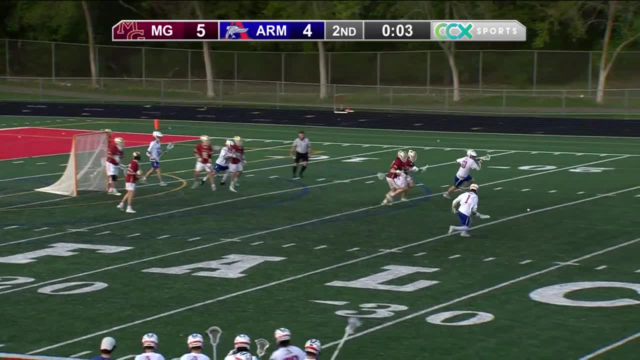 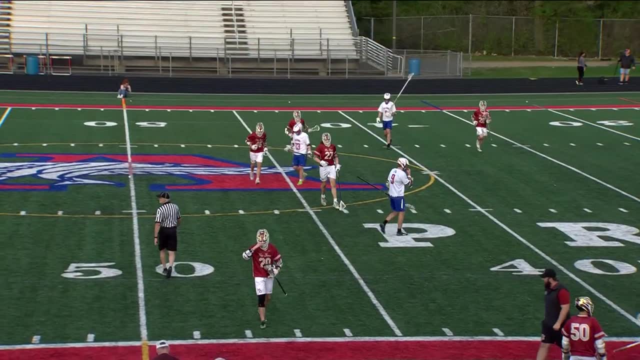 I would have come out of this seat. Man, oh man, What a goal. that would have been Three seconds. two Time will expire here in Plymouth in the first half, And what a first half. it was Back and forth. these two teams went. 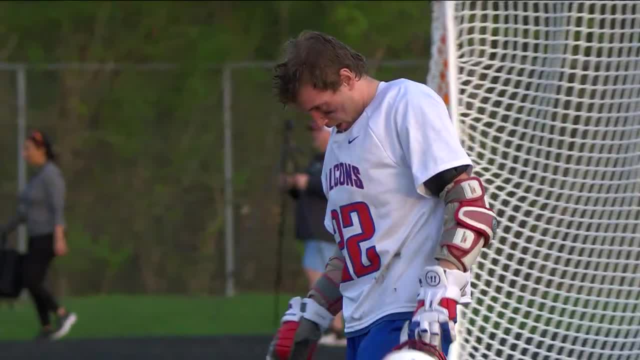 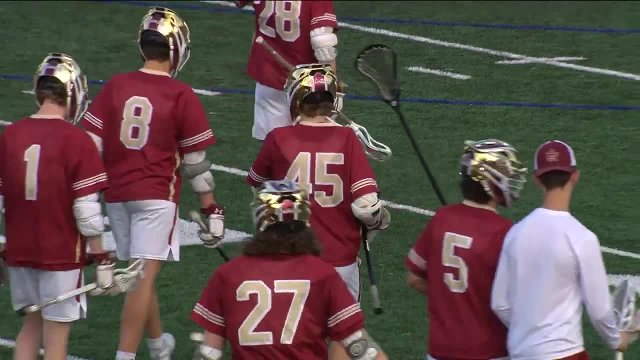 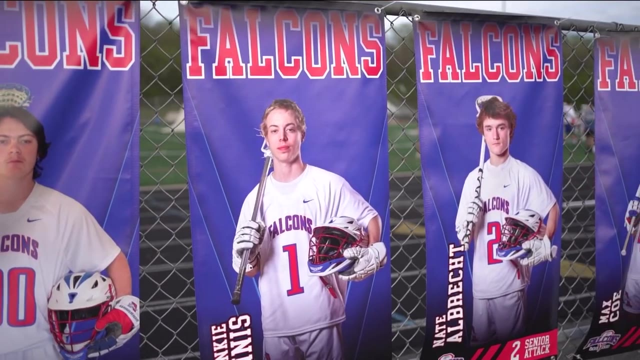 Maple Grove scoring the go-ahead goal with 38 seconds to go in the first half, Essen with a couple goals, Annis with a couple goals, Ricky Scanlon with a goal and three assists. And we'll all take a breath here at halftime. 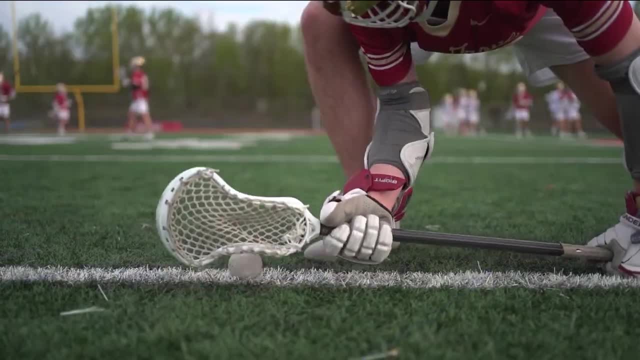 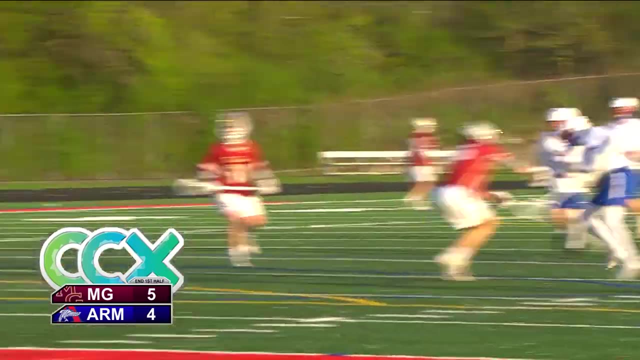 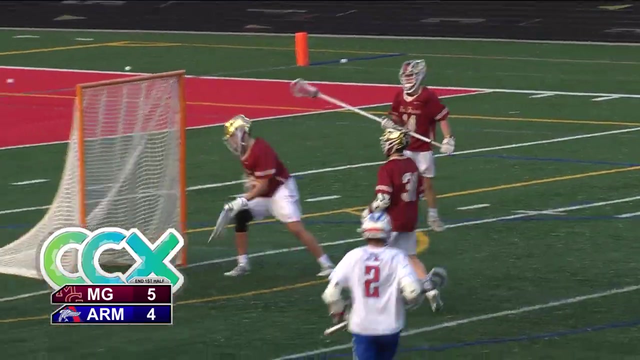 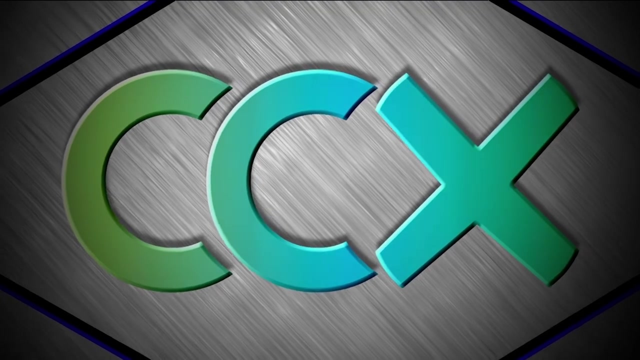 as Maple Grove. the ninth-ranked team in state leads Robbinsdale Armstrong on the road here at halftime five to four on CCX. CCX Media, your source for great local programming, is available on Amazon Fire TV, Apple TV and Roku. 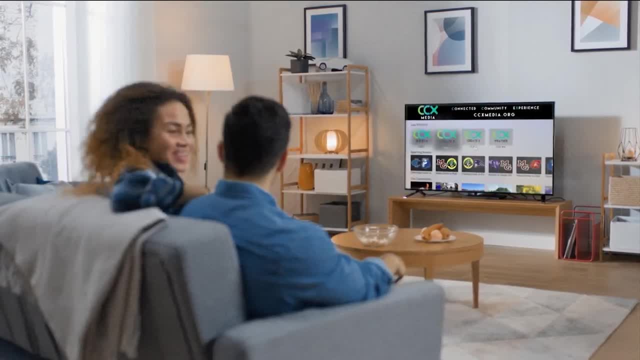 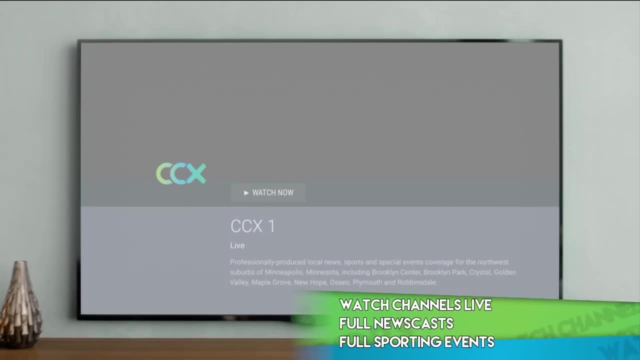 Our free app allows you to stream all three of our channels live. You also have access to a large on-demand library including full sporting events and daily newscasts. To find us, go to the store, search CCX, and download our free app. 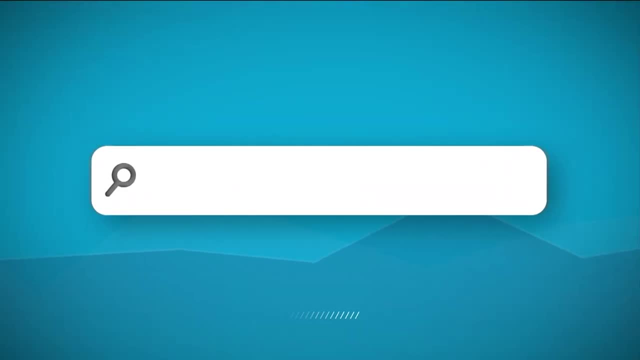 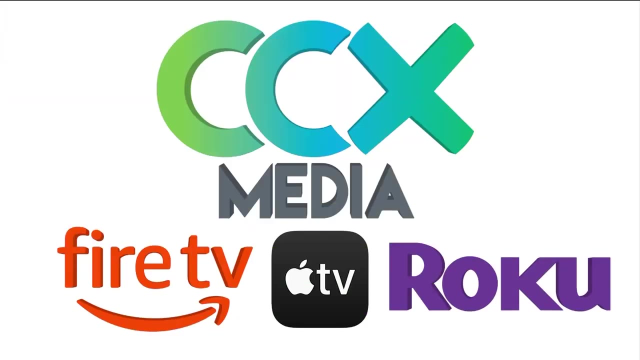 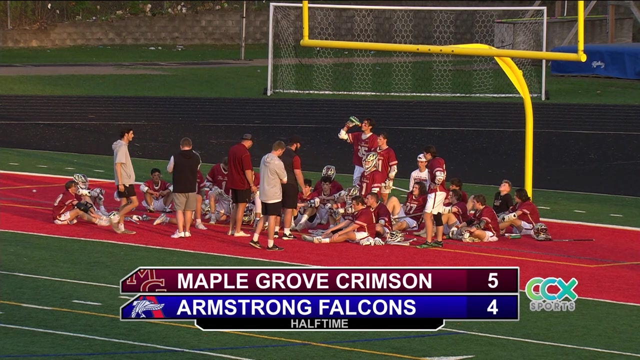 Then sit back and enjoy all of your favorite local content. The CCX Media app, your source for great local programming, is available on Amazon, Fire TV, Apple TV and Roku Five-four- our score at halftime here at the Falcons Nest in Plymouth. 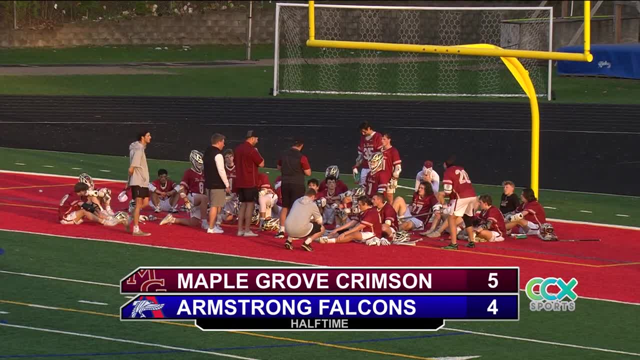 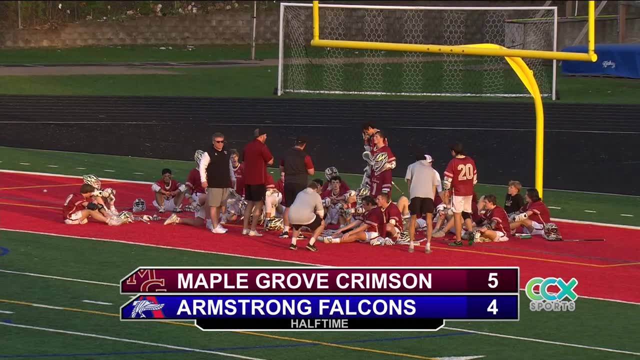 Bill Hupp and Dan Ficken for CCX Sports And a very back-and-forth entertaining half of lacrosse. We just witnessed the Crimson retaking the lead just 38 seconds into the game. We'll be right back. We'll be right back. 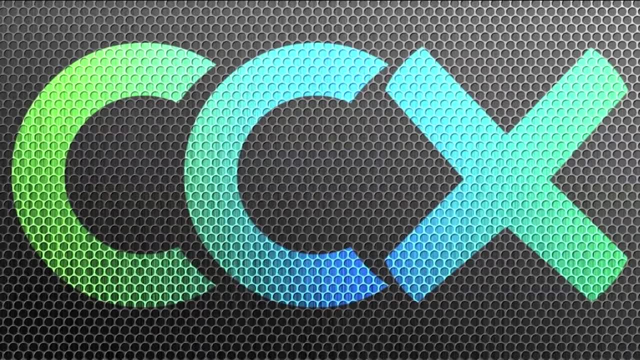 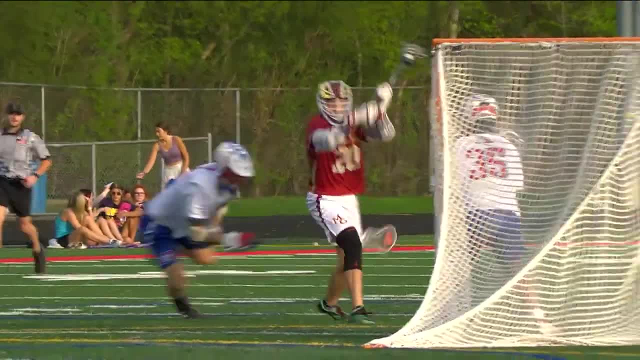 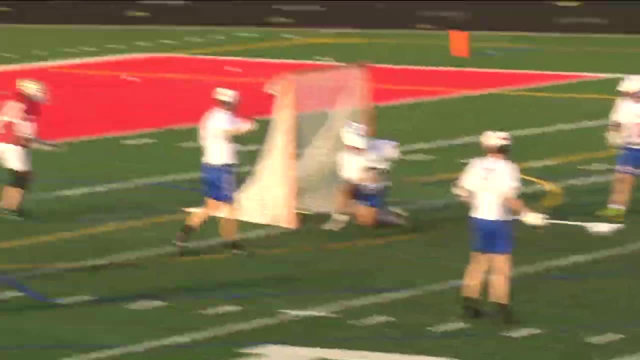 We've got 30 seconds to go before halftime as Kyle Ficken talks to his troops And we look at first-half highlights. And again, very entertaining first half: Great goaltending here, as you see Xavier Wells getting in the act And then Hank Varniak. anything you can do, I can do better. 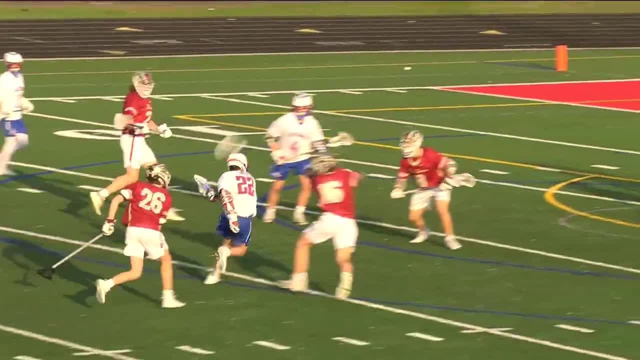 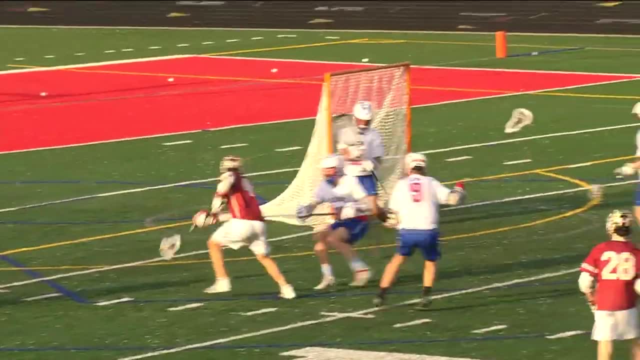 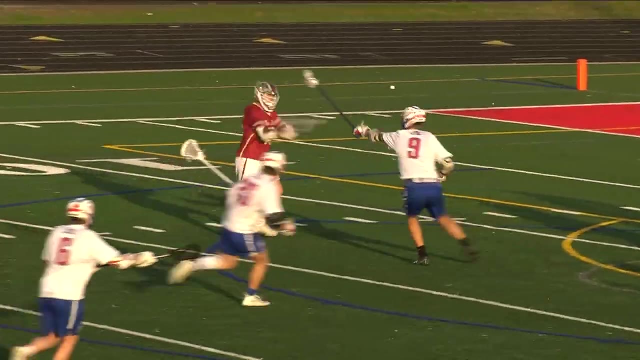 Wells making another tremendous save. Then the goal scoring started with Jamison Essin driving downhill. Every time Robbinsdale-Armstrong scored, Maple Grove seemingly had a response. That was one of their two EMO goals And again any goal that was scored here in this first half, Dan. 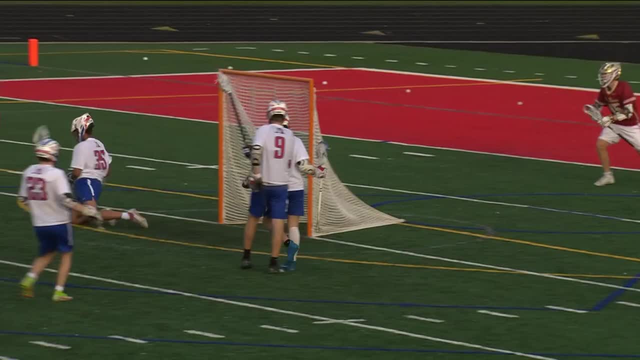 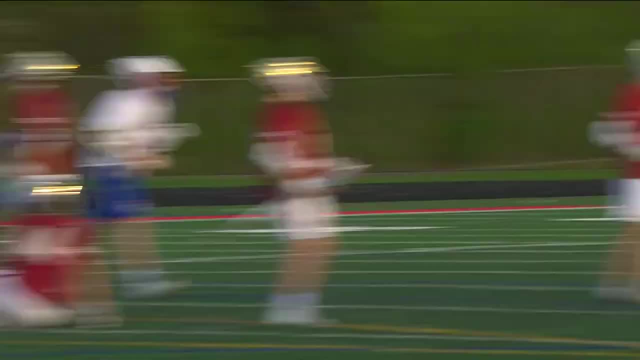 it seemed like was unsavable. Yes, As Scanlon had all kinds of time and room to let that one fly. Most of the scoring took place in the second quarter, as we were tied at one after one quarter of play, But ultimately, 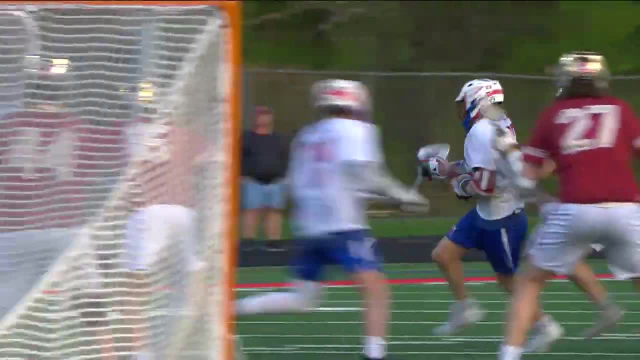 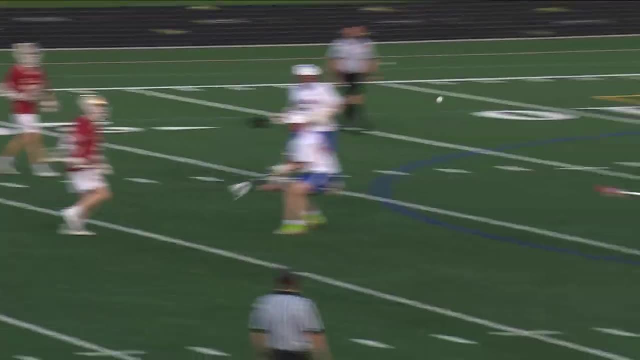 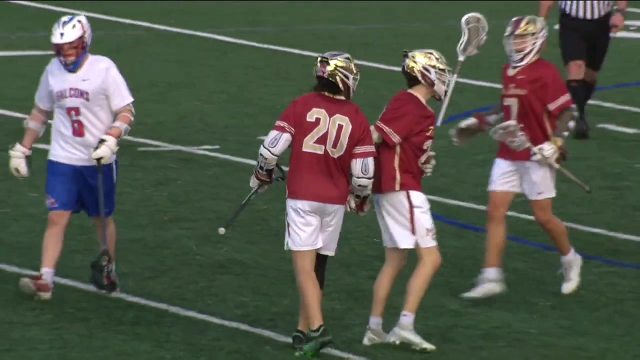 it feels like it has that feel of a one or two goal game at the most, And we saw some really good shots, including that one from Jamison Essin. So much college talent on the field And then a sophomore Peterson jump shooting his way into the lead for the Crimson at five to four. 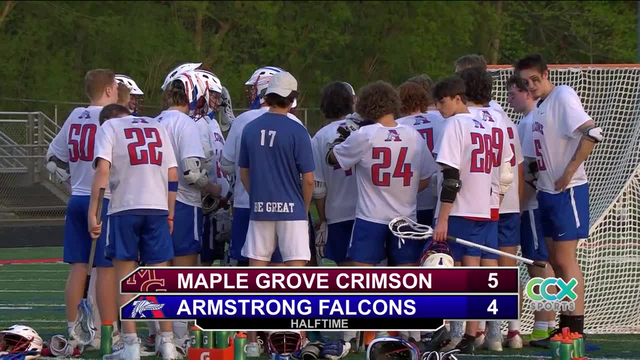 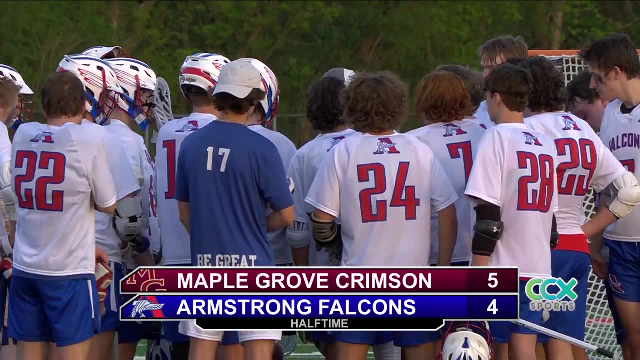 Boy, just some unbelievable bullets coming out of these players. Just you know, goalies really don't have a chance. They were getting, just you know, some really good shots coming through them. Yeah, no, We expect more quality to come and halftime adjustments as well. 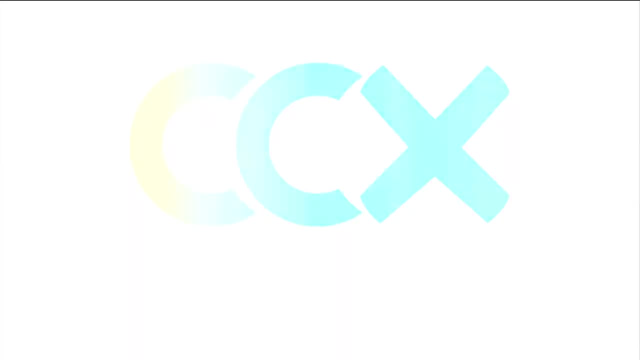 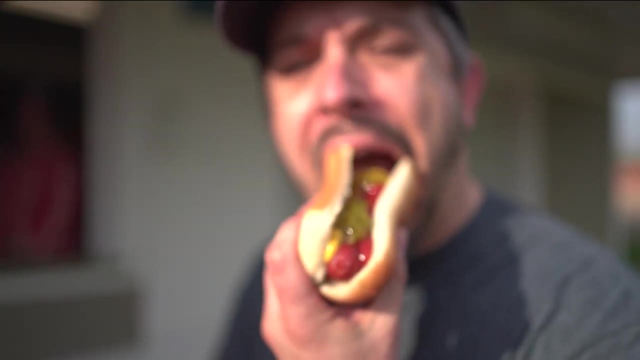 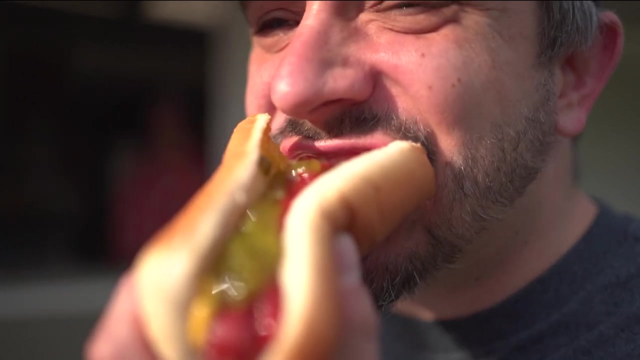 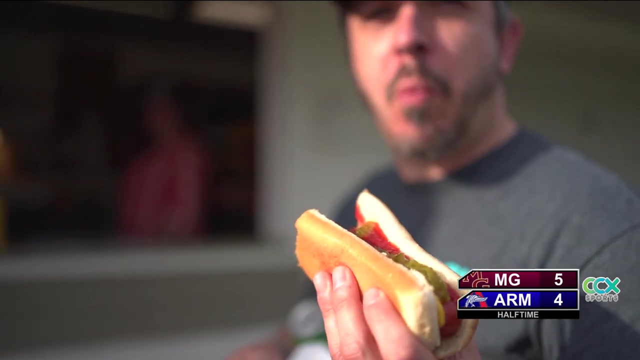 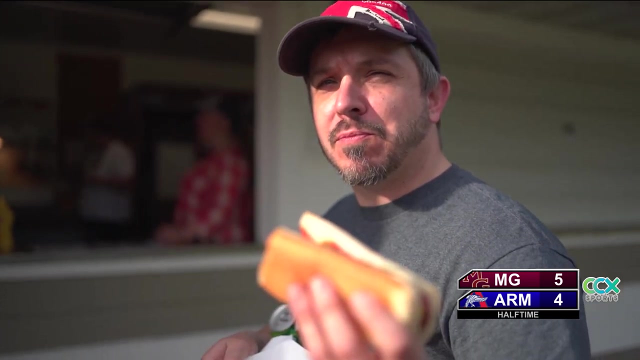 Be back in just a moment from Plymouth and the Falcons' nest, Back with second half action. Get your popcorn ready. It should be an entertaining one. in the second half We'll be right back. CCX Media, your source for great local programming. 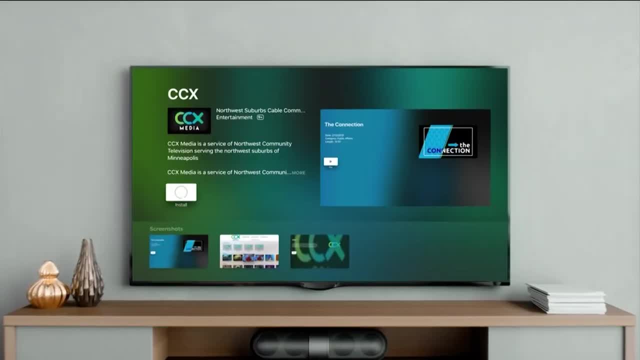 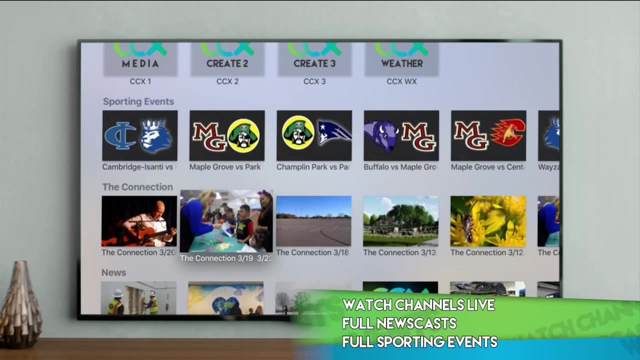 is available on Amazon Fire TV, Apple TV and Roku. Our free app allows you to stream all three of our channels live. You'll also have access to a large on-demand library including full sporting events and daily newscasts. Just go to the store, search CCX and download our free app. 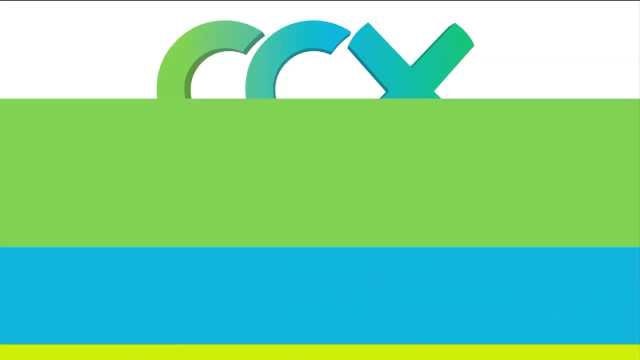 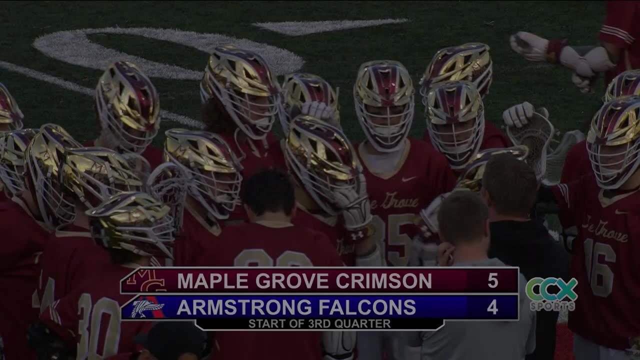 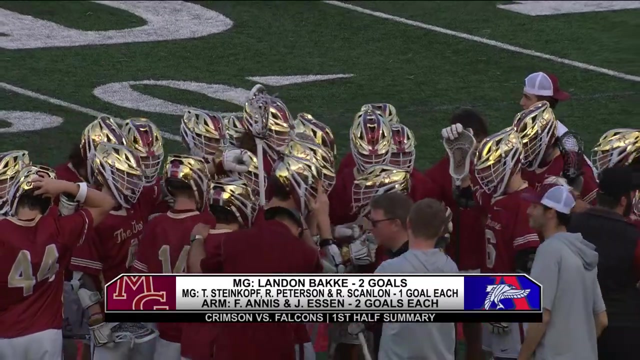 Then sit back and enjoy all of your favorite local content: The CCX Media app, available on Amazon, Fire TV, Apple TV and Roku. Start of the second half here in Plymouth. Buckle your seatbelts, grab your popcorn, get ready. 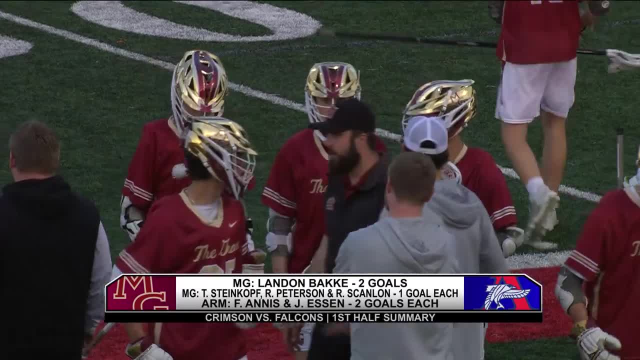 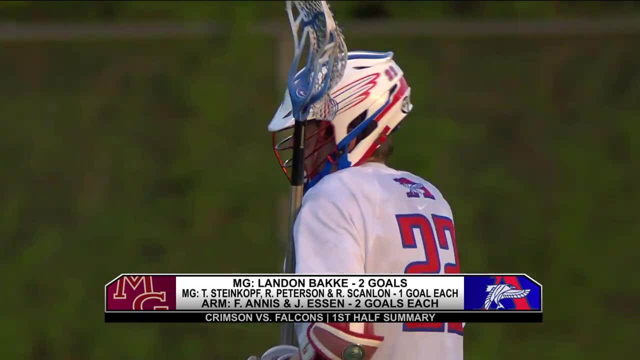 because it should be good. Multi-point scores for both teams: Essin and Annis, each on hat-tricks for Armstrong, Landed Bakke with the first two goals for Maple Grove, and then Peterson, Scanlon and Steinkopf with a goal apiece. 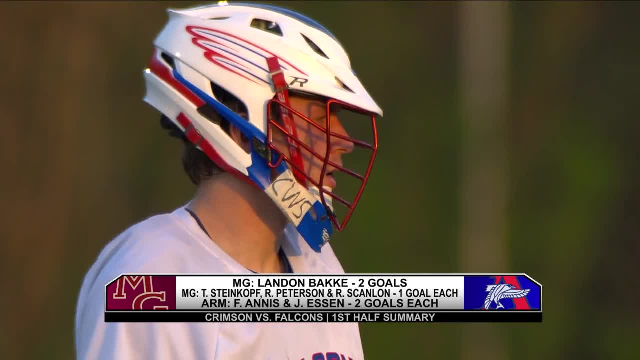 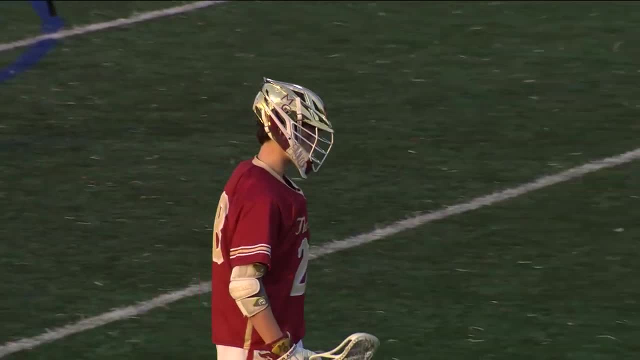 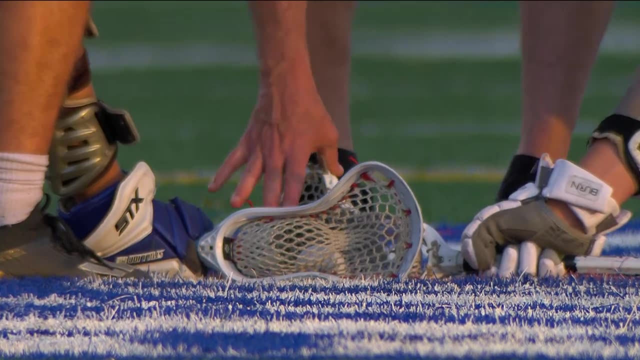 And certainly Maple Grove, despite being just dominated in the face-off circle just two of nine. But that has not ultimately mattered too much, As Rory Scanlon, the Springfield-bound senior attackman, has really chipped in with a goal and three assists in that first half. 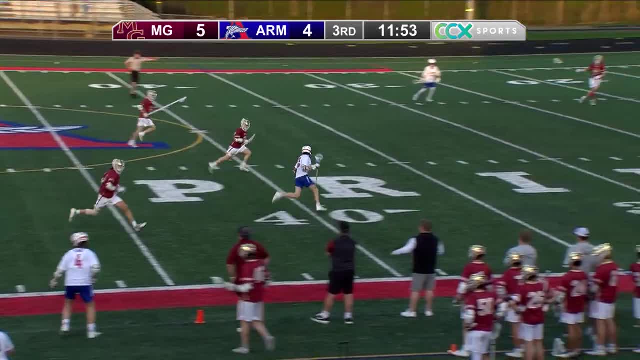 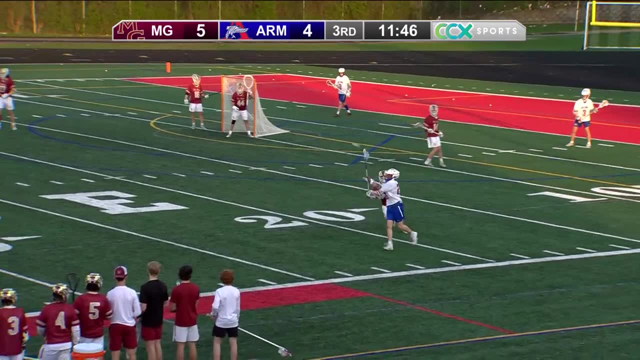 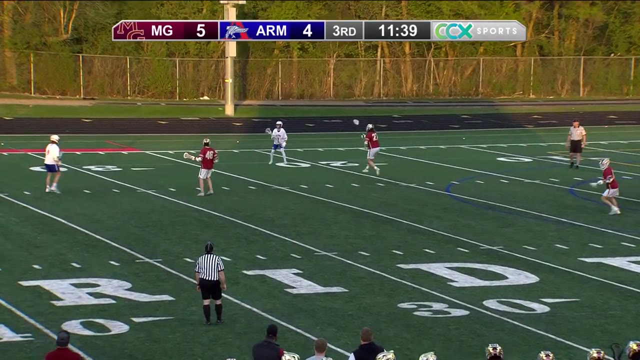 Once again Armstrong wins the face-off. Essin has been a ground-ball machine tonight. He's got two goals and he gets a touch in the box and starts the show for Armstrong here in the second half, Crossfield pass finds its way to Max Coe. 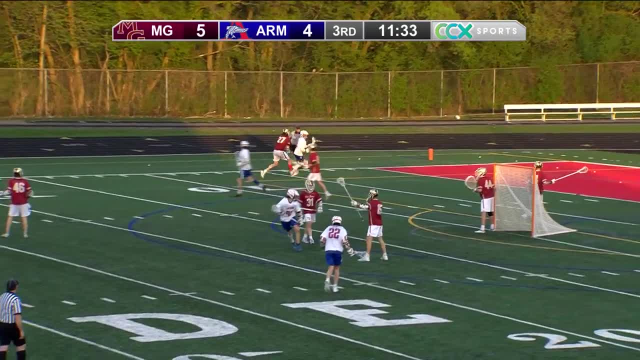 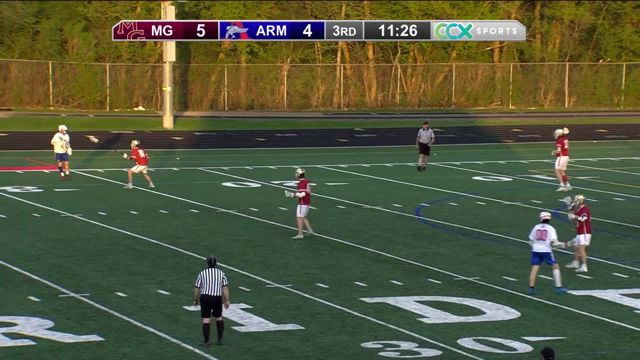 Annis, watched closely by Jackson Bennett. I don't think either of these teams are going to slow things down. I think they're both going to try and keep playing at this frantic pace they've been playing at. Albrecht gets a step. 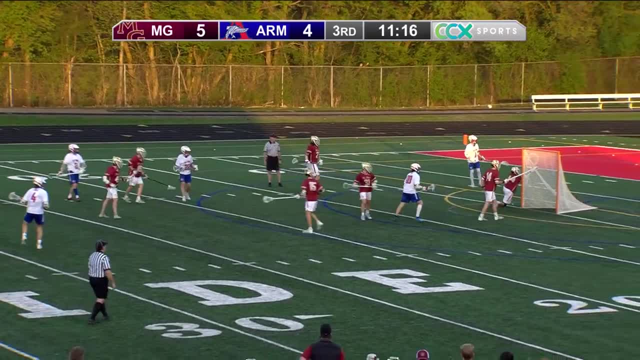 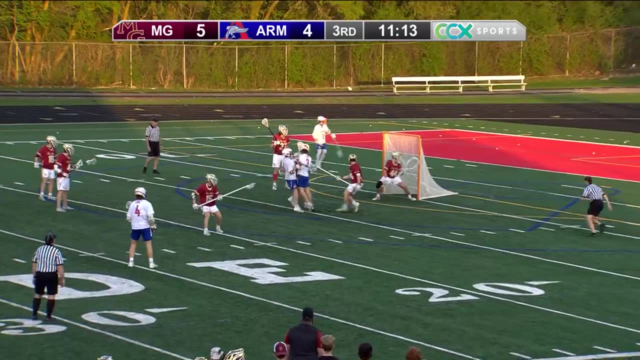 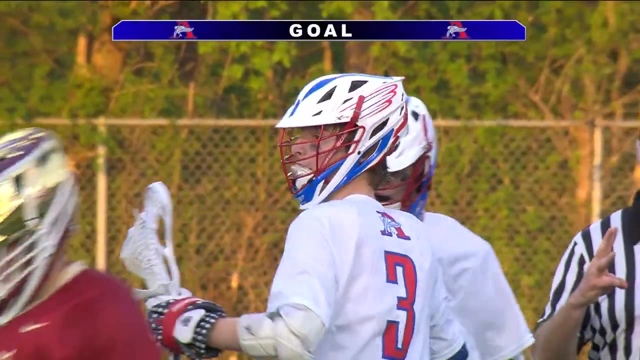 Rolls off the slide by Jackson Kuznick and the shot goes wide. But it remains, with the Falcons Coming right out shooting and scoring. Nice goal by the freshman Jack Olsen, His 21st of the season. Just snuck around from X and bounced it past Farniak. 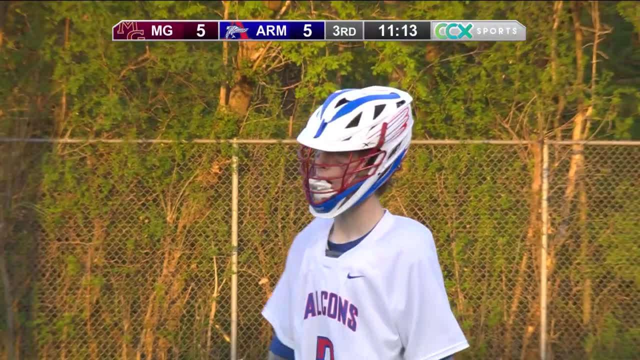 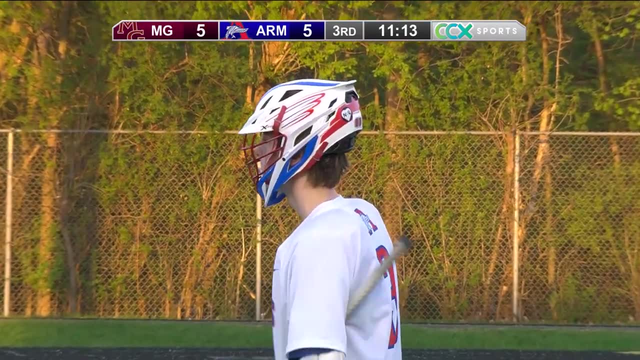 And early in the second half we've got a tie ball game once more. He ain't playing like a freshman. Oh my gosh, What a great set of speed there coming through and just a great shot going down low And beating, I think, on the short side of Farniak. 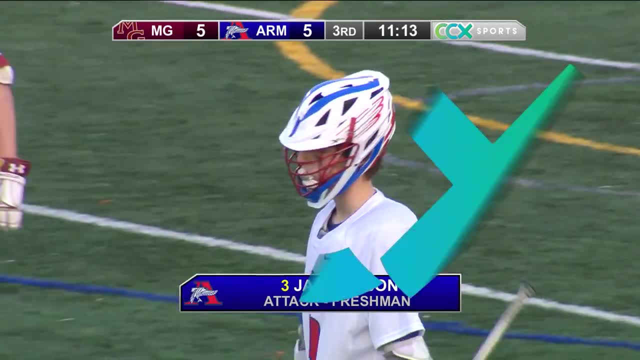 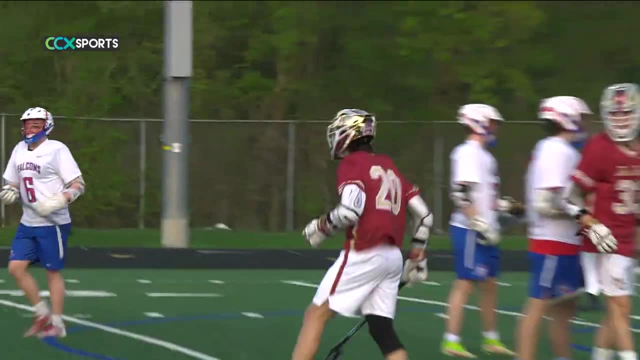 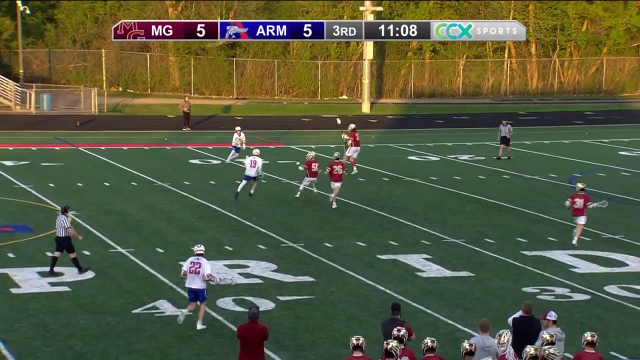 On the restart, 47-7. Seconds into the second half. That's the jump shot goal by Peterson late in the first half, As once again, Armstrong wins the faceoff Ninth faceoff win of the game And Annis has it, and this is the make it take it thing that we were talking about there. 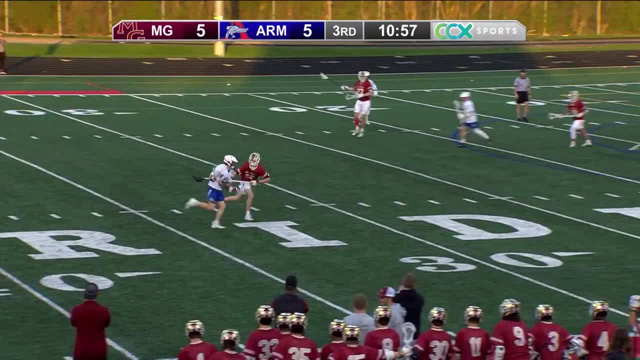 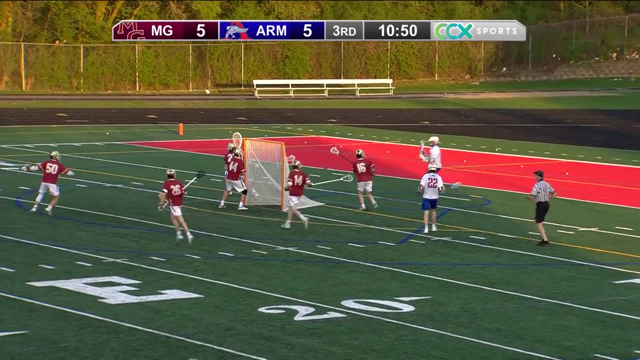 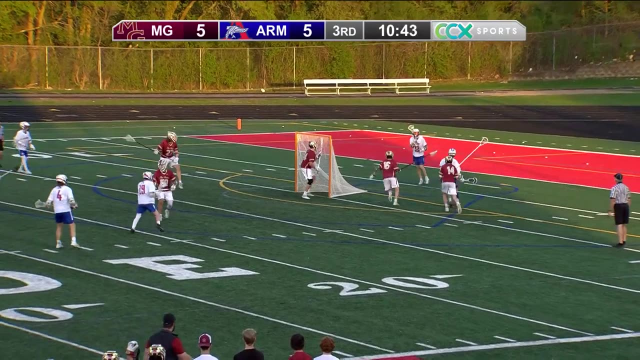 As Essendon possesses. at the top. Essendon, with a couple goals, Nearly, gets tripped there, Somehow retains his balance. Goal on extended Albrecht, switching hands, Spinning that rock, Flips it to Essendon. He's always got his head up. 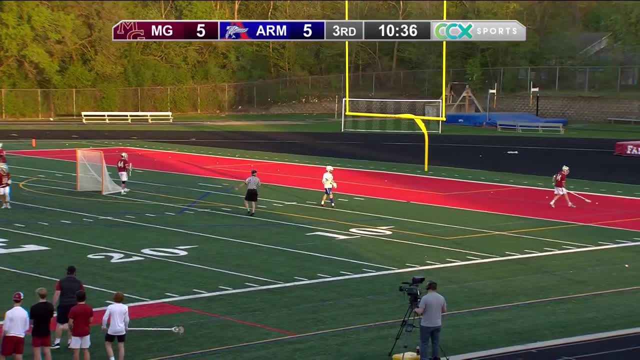 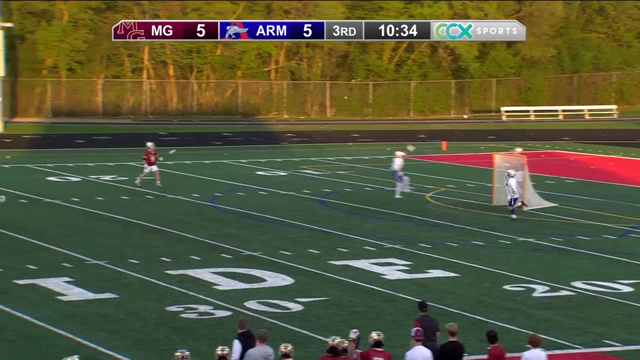 There's a bounce shot that goes wide. Maple Grove closest to it. Good hustle there by number 14, Joey Eisler Trying to make up for maybe those first couple first half penalties. But Eisler was closest to it, so it turns back over to the Crimson. 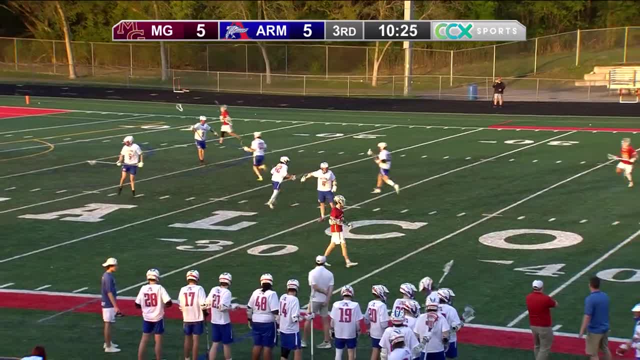 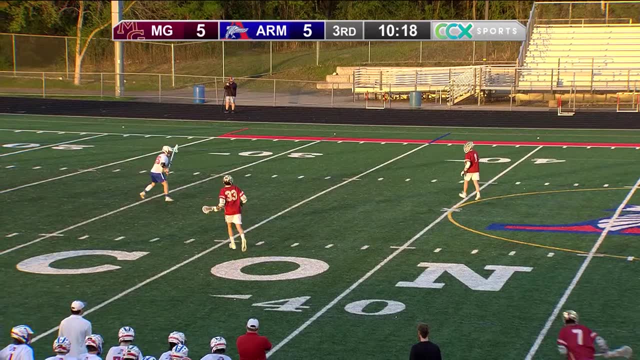 Great find ahead for Scanlon. They do that cross field clearance pass so well. Saw that in the first half and it led to a goal. They're usually rotating their midfielders around out there too, so they're moving to different spots. 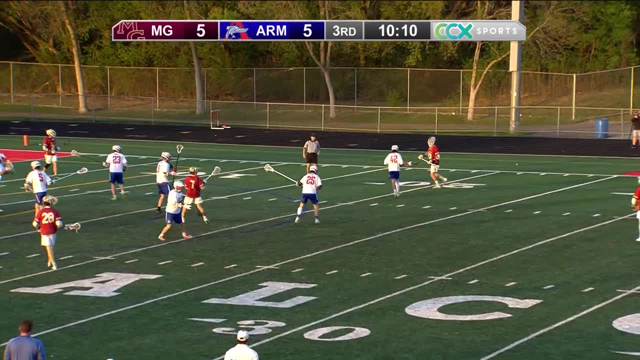 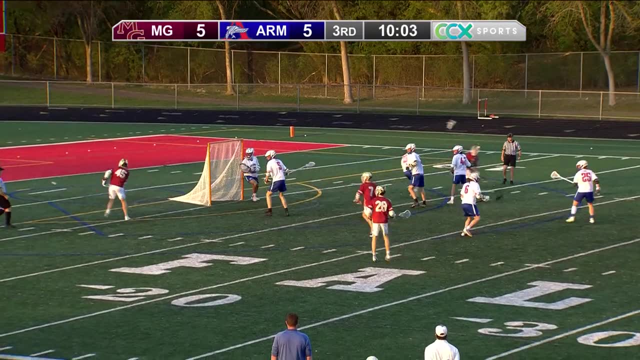 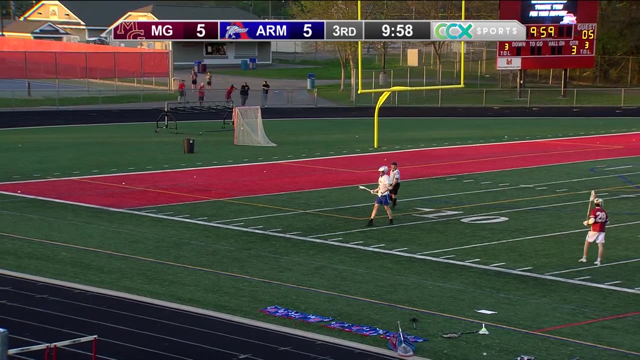 So somebody's filling a space. so wherever they throw the ball, sooner or later a Crimson player will get there. Brendan Behind for Peterson At X. Peterson Sharp angle shot. That was a bit of a prayer, But Farnie, or rather Bakke, closest to it. 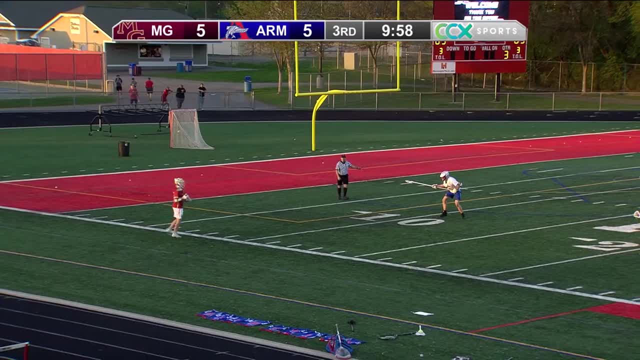 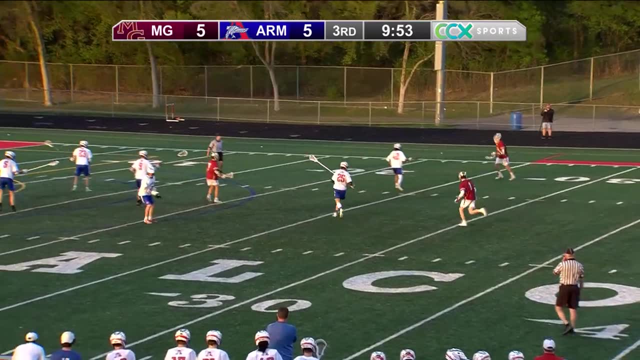 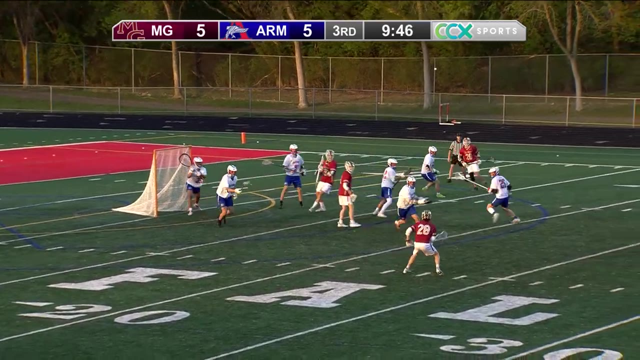 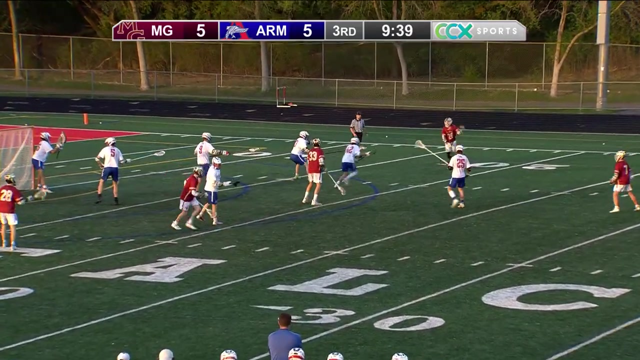 so it remains. with the Crimson, Shiny chrome helmets glittering in the sunlight, The light's not quite taking full effect yet Sun's starting to set behind our press box, Cross field pass snagged by Scanlon Maple Grove continuing to patiently possess. 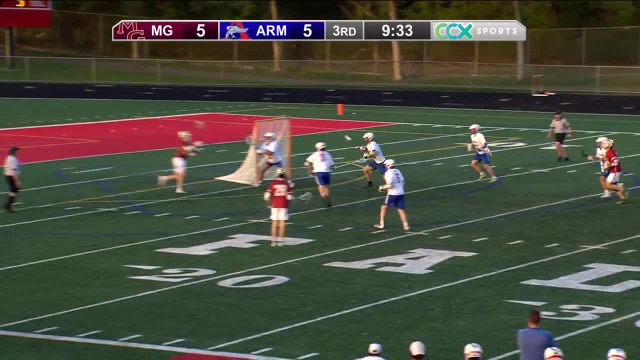 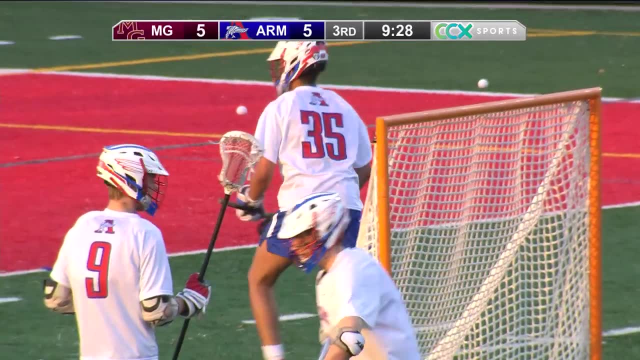 It's Peterson Has inverted to the top Steinkopf sneaking from behind. Oh, nice save. And a big save made once again by Wells. Wells fired up as he stoned Bakke who was coming trying to sneak around from behind at X. 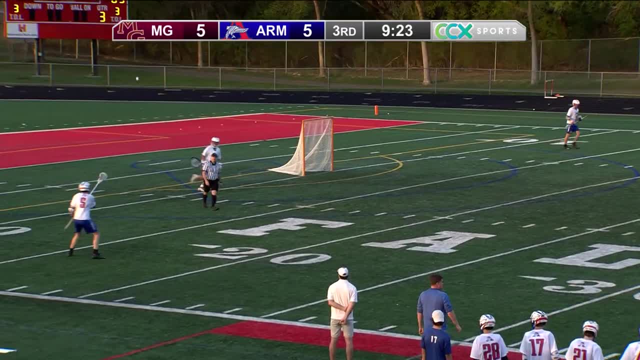 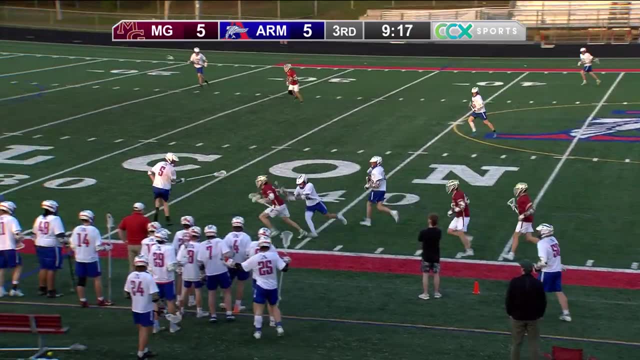 Boy Wells is really the real deal. He hasn't let up one bit. Boy, what great goaltending we're seeing on both teams tonight. But boy Wells has really stood out. Now they try to clear it, and a great job by Scanlon. 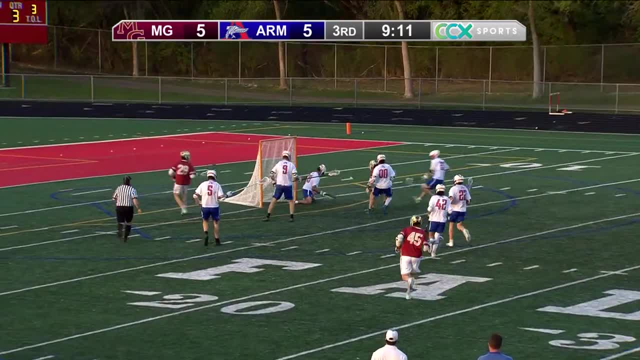 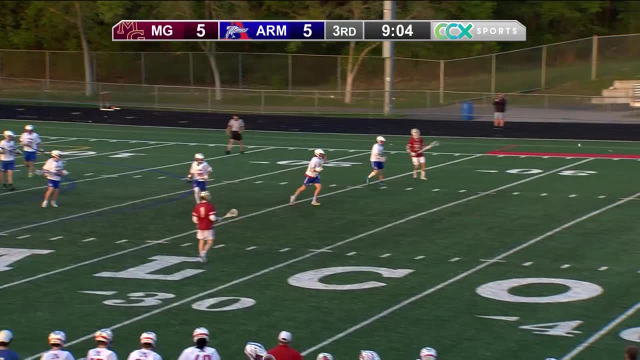 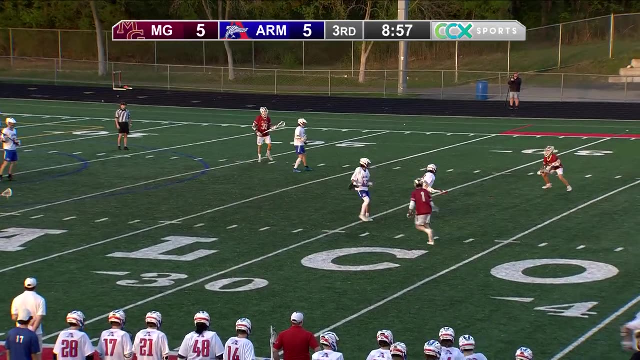 To force the turnover. Rory Scanlon, bearing down on that, Feeds across Another tremendous save made by Wells, This time stoning Peterson- Oh my gosh, Incredible- from Xavier Wells, who's had five highlight reel saves here in this lacrosse game. 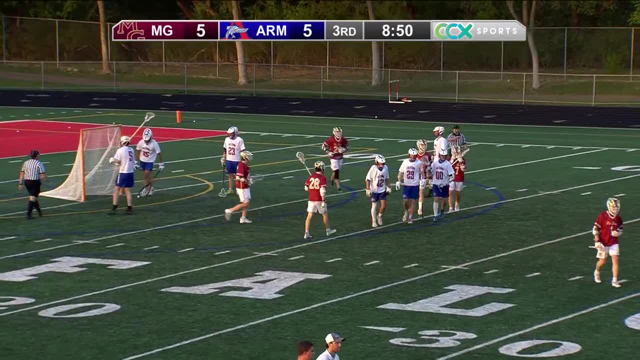 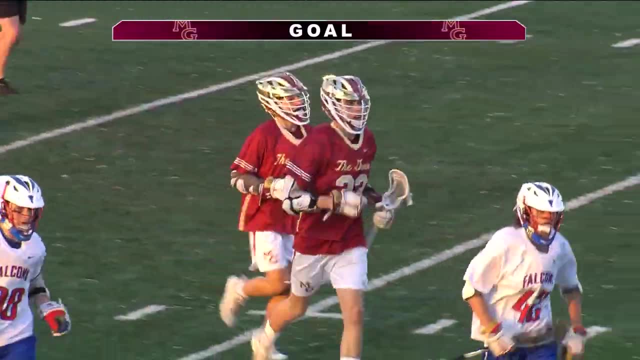 Not saving that one, though, as Tanner Brendan lights the lamp for goal number 13 of the season. Well, if he first he don't succeed, Keep shooting. Well, here's the lesson, Dan: Shoot from the outside, because you're not beating Wells up close. 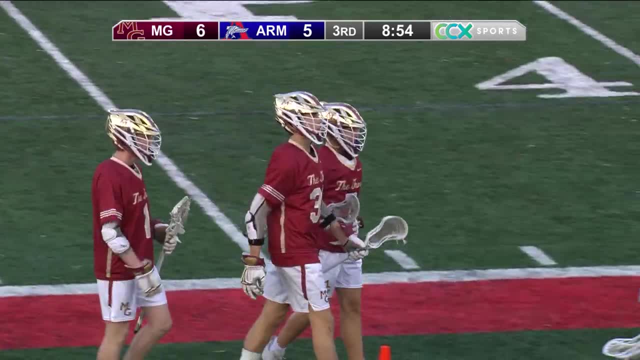 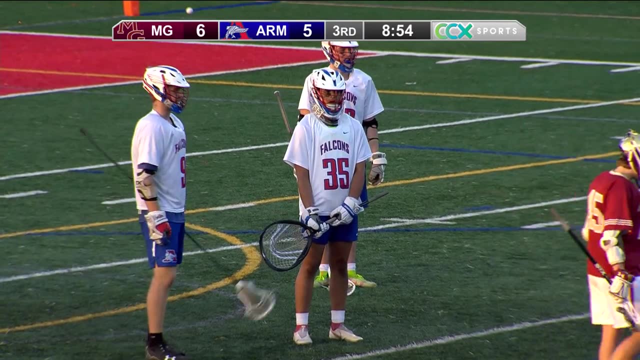 No, He comes out and just attacks aggressively and he's done a tremendous job. He's been the player of the game so far. I don't care if he just got scored on, He's been tremendous. Oh my goodness gracious. 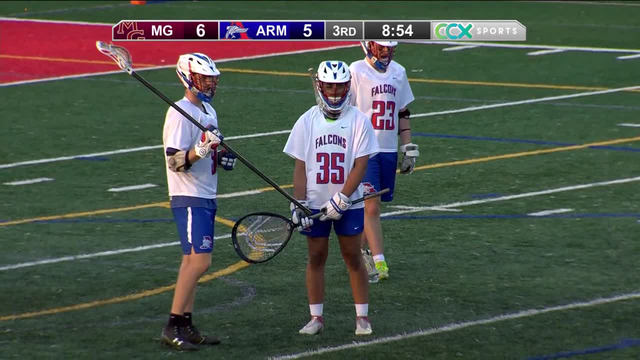 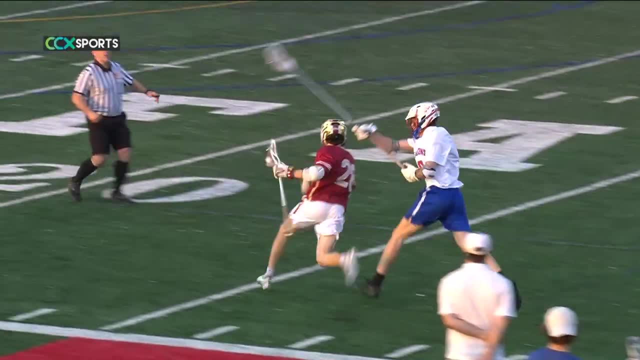 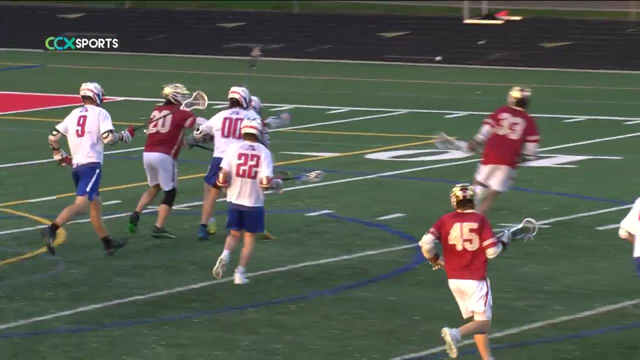 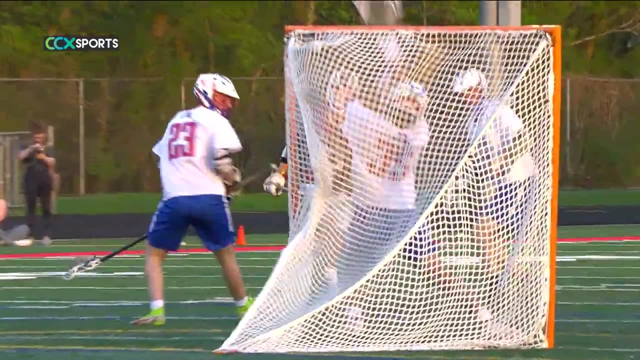 but a brilliant pass across. a little high maybe, but Peterson tried to just sort of one-time it in, quite a quick stick it, as they say, And then Brendan the lefty and that's just a perfect placement, Yeah. 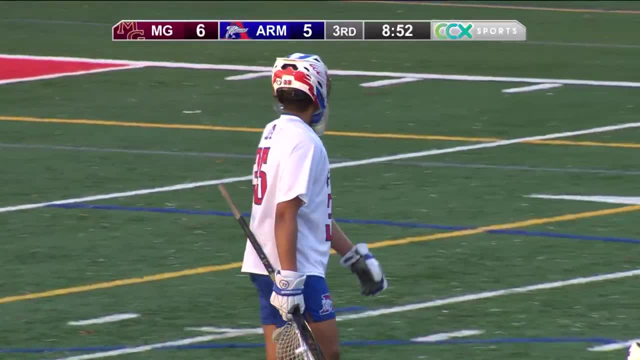 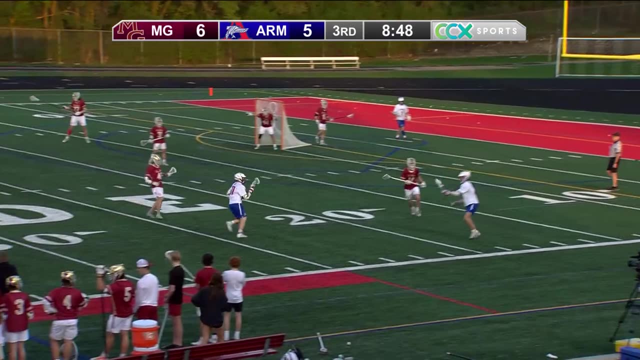 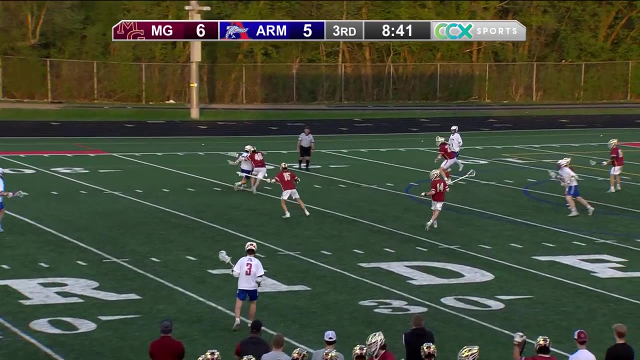 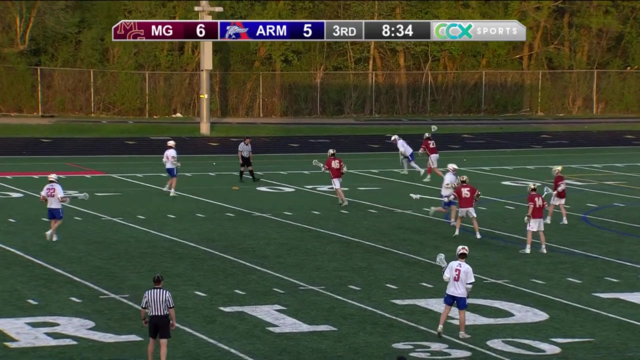 Right there in the upper 90.. Just at the crossroads of the bars there, Perfect shot. Yeah, no saving that one, As Brendan has given his team a 6-5 advantage Here. early in the third quarter, Another face-off win and another flag, as Jackson Bennett shoved down Max Cole. 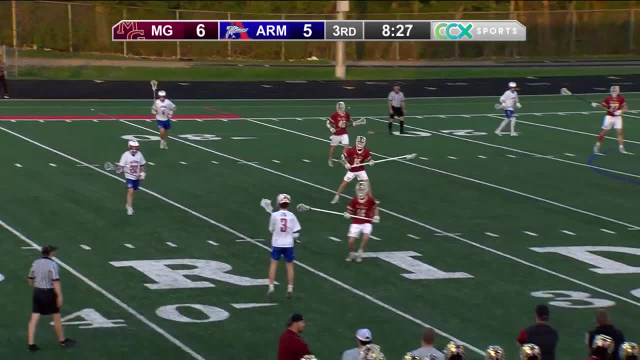 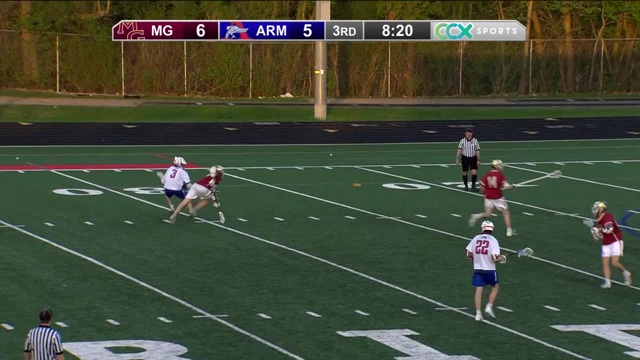 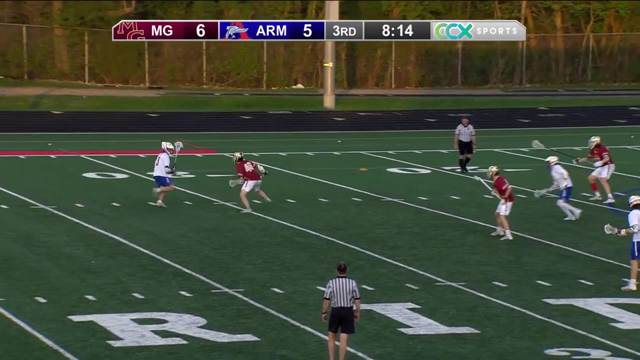 Now Armstrong will try to get one and then take the EMO Olsen backing it out Hardy with a goal in this half. Olsen seems to have a really good lacrosse IQ, especially for just a freshman. He uses his head, He's controlling it well. 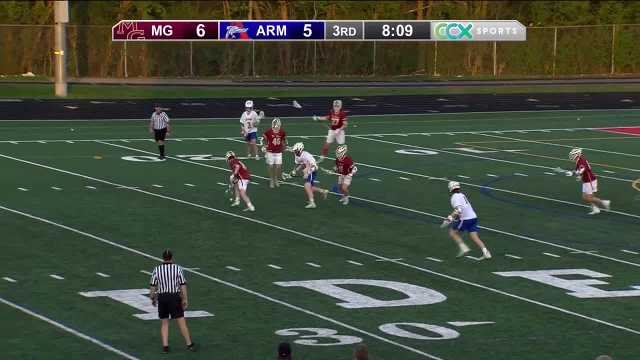 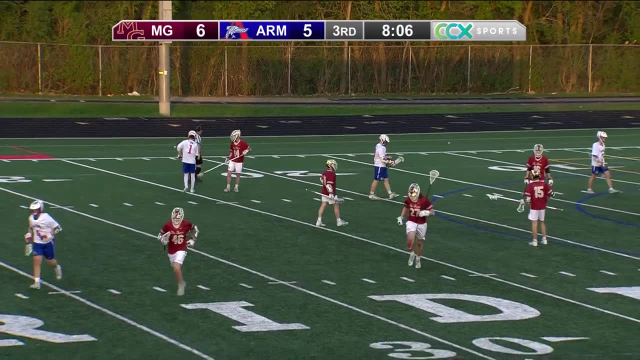 Knows when to go and when to back off a little bit. You know you can see the pace there. Oh bad pass, Yeah, Not just as I say. a great lacrosse IQ Tries to thread the needle to Logan Marsh, which was maybe ill-advised. 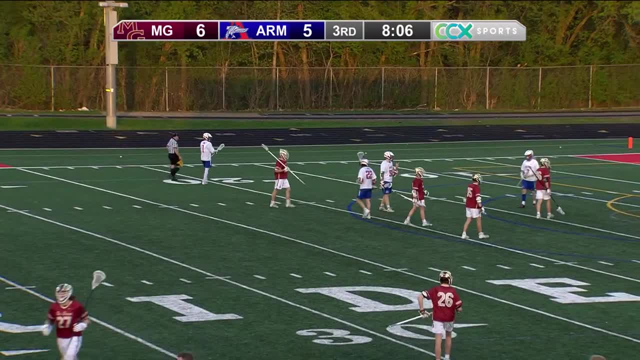 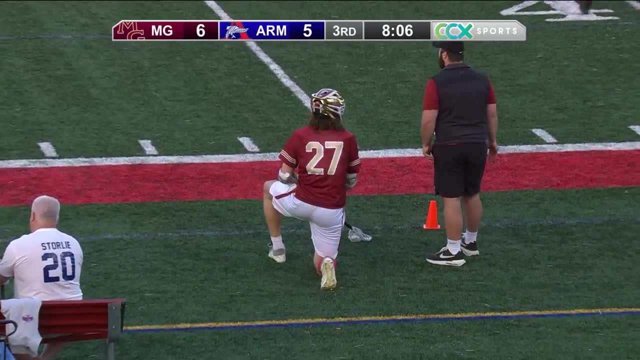 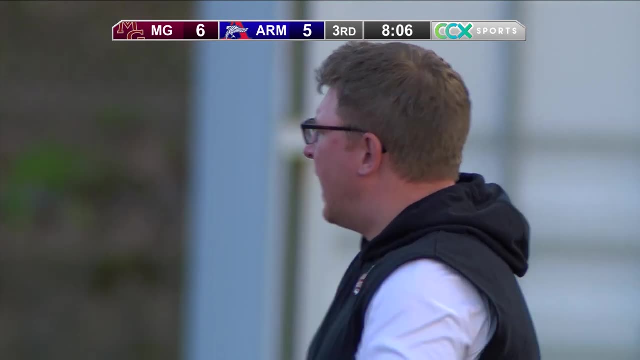 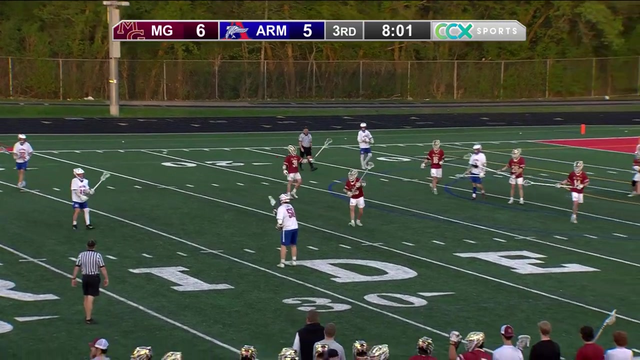 And now the penalty by Bennett: We'll send him to the box and He'll take a knee. Meanwhile, the younger Fickett, Hand on hand, shaking his head, The studious, looking with those glasses He is kind of, which makes him not like his father one bit. 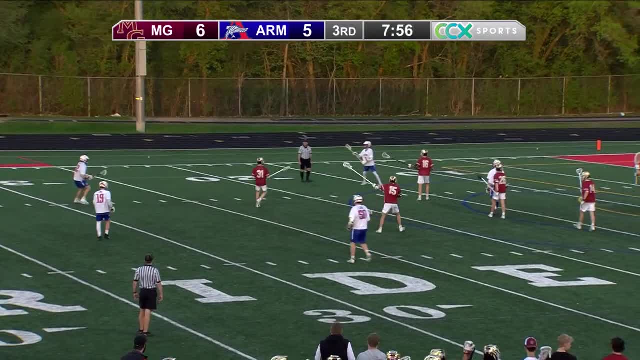 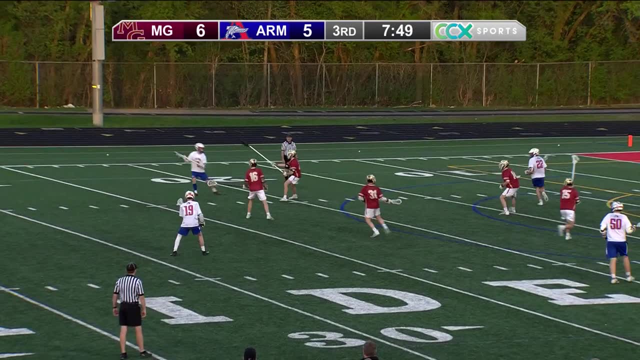 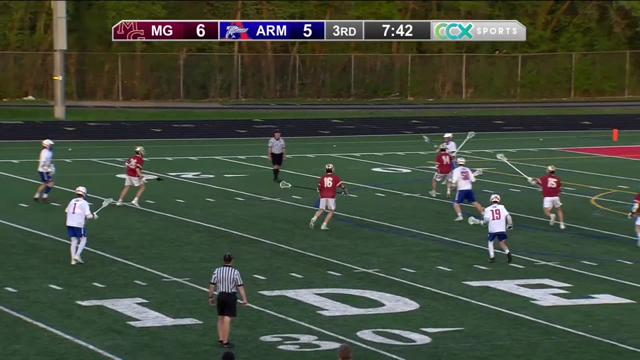 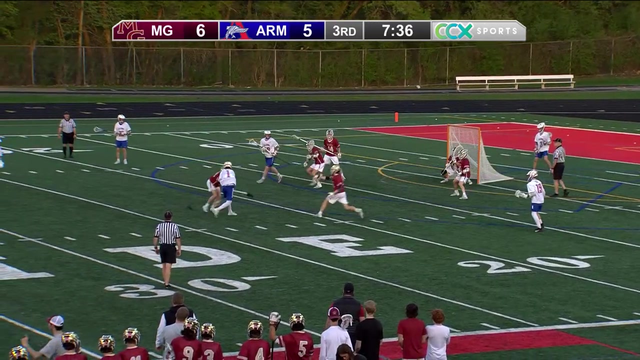 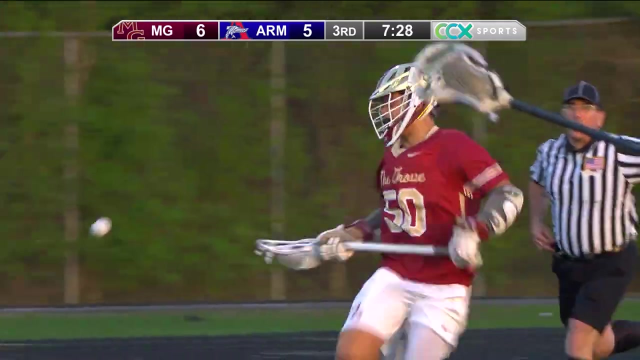 There you go, Jen, It's all yours Eight minutes to go. Hello to Mrs Fickett watching at home: Albrecht directing traffic to space it out, Annis and he play catch Essendon behind for Olsen shot here by Annis right into Farniak's butterfly net and he clears it ahead through Briggs Leisner and then Leisner loses it to Berry. 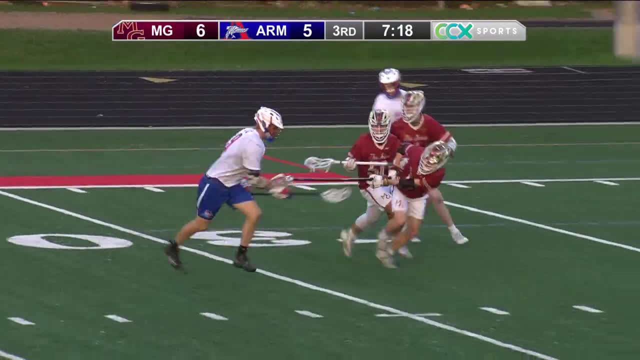 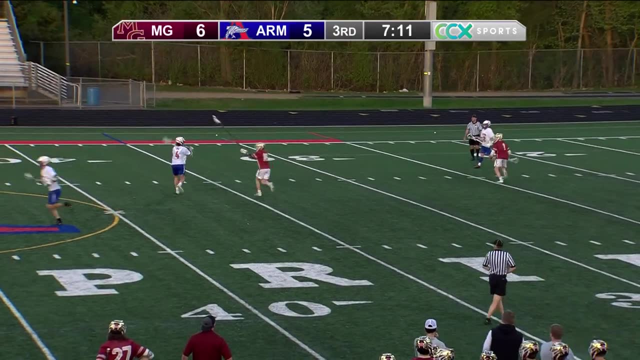 I beg your pardon. That's Aiden Robb the long stick, middie the junior- It's a big load out there and he's continuing to carry the rock- Finally flips it back for Coe. Nice job by Berry, That was impressive. 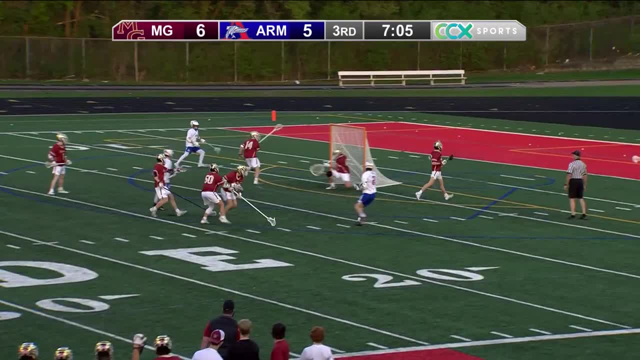 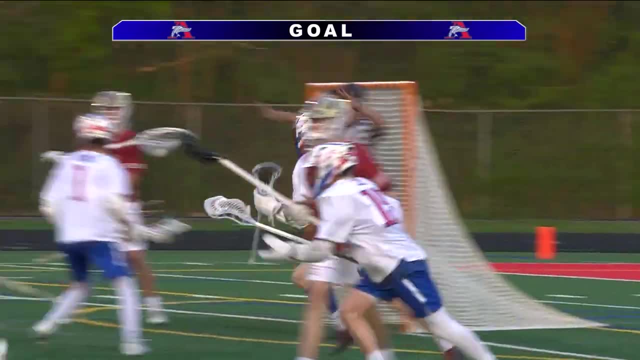 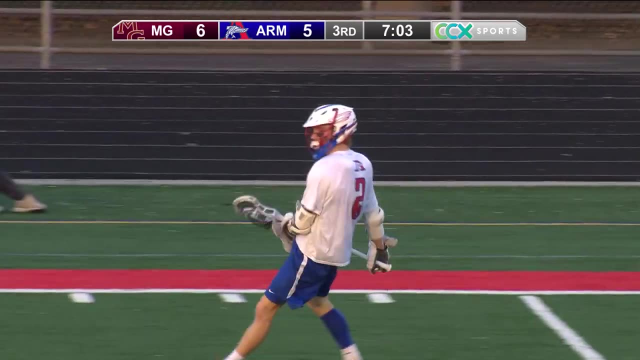 He did a nice job for a big guy, Albrecht, downhill with a head of steam, Goes across his body and scores. He loves shooting while moving to his right. Oh, they're waving it off. They're saying no goal, Really. 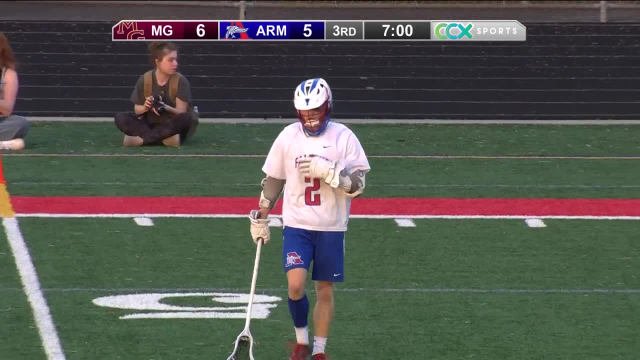 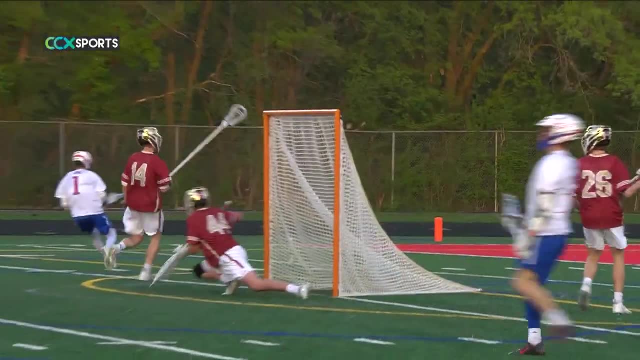 And I am to be honest, I'm not sure why. I don't know if a guy was in the crease. Hopefully see a replay a little bit. I'm still not sure why that goal was waived off. Nobody was in the crease. 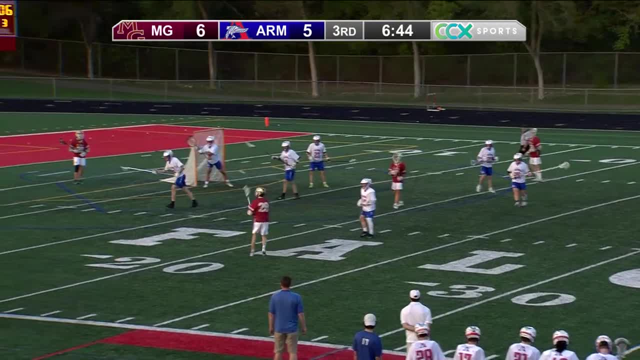 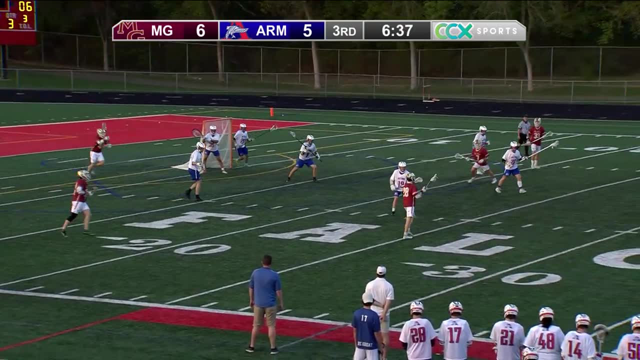 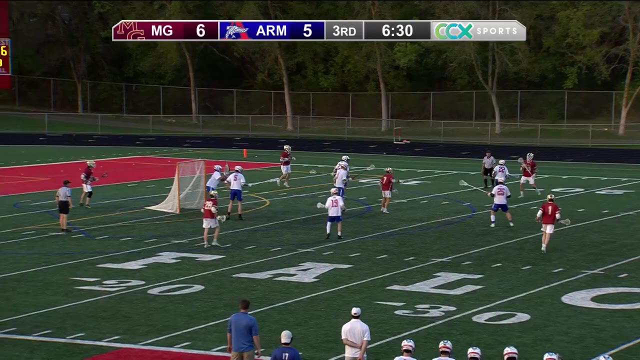 No, but it was waived off. Wow, So there goes that We thought we were tied at six, but instead it remains a one goal. Crimson lead: Peterson, Scanlon, Steinkopf. Well, the Crimson were smart there and just starting to play the ball again and just get rolling before anybody could rethink it. 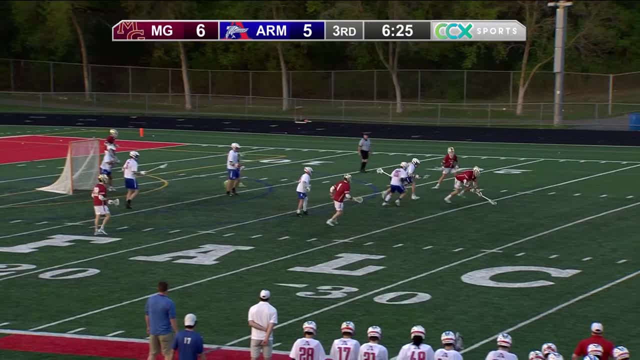 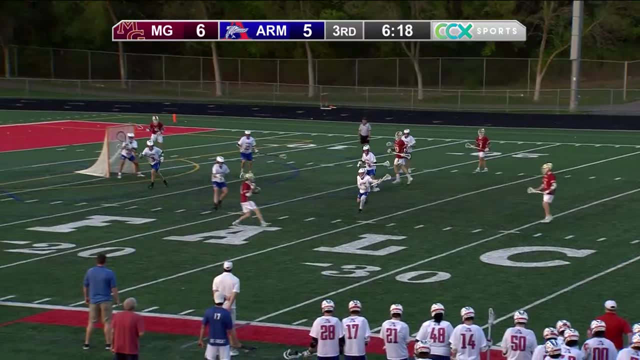 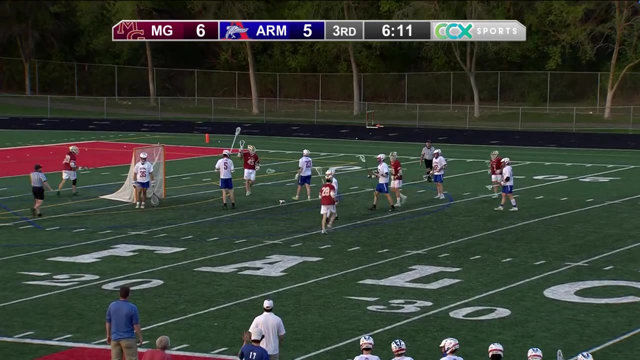 Yeah, Brendan Steinkopf. Oh, he tries to slip a pass. Passed Essendon, That didn't work. Crimson able to recover, though, And Steinkopf gets it for Scanlon. There's a shot and a score. 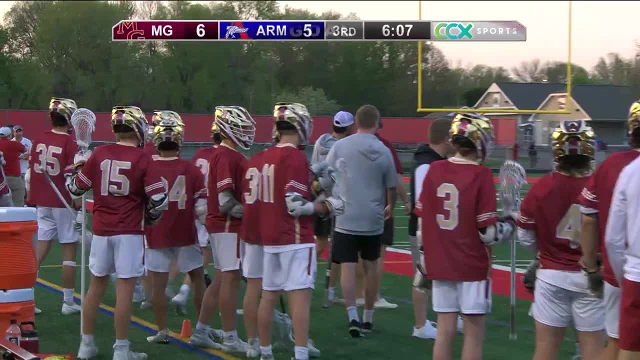 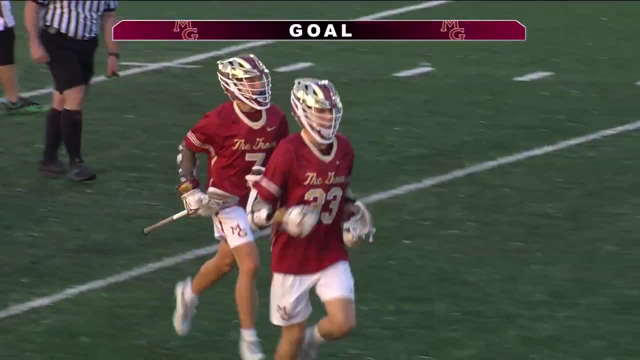 The physicality of Tanner Brendan as he somehow stood in there, took a hit and still scored. He's got the last two for Maple Grove and they have their first two-goal lead of the night. Yeah, used the screen that time as he took that shot, as the body was on him. 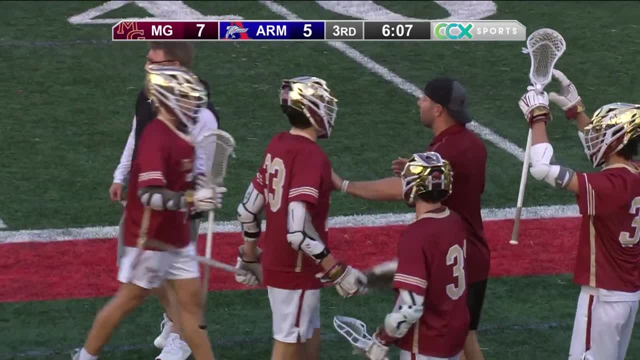 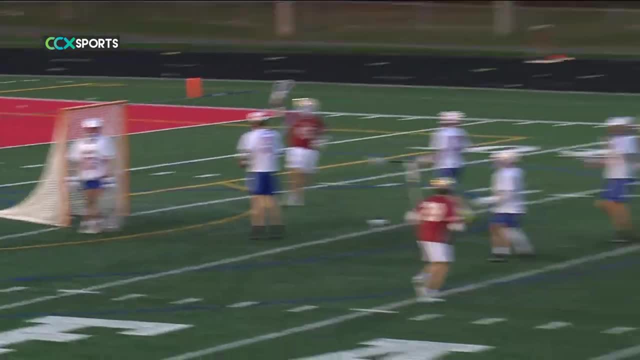 There was another guy in between And I think it surprised Xavier Wells there. He didn't see it coming on him For sure. Yeah, number five was in front there and kind of blocked it out. But jeez, nice shot. 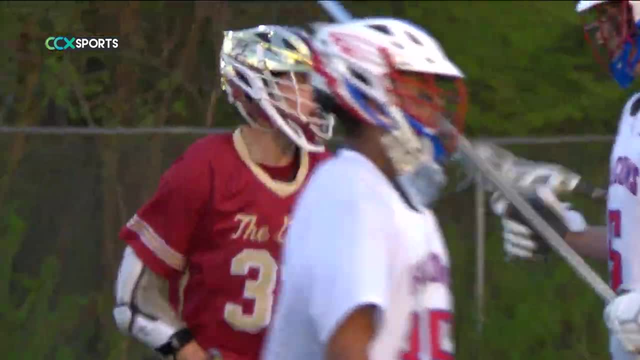 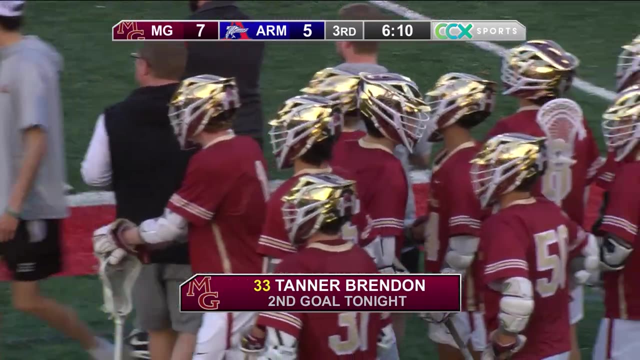 Talk about getting hit and putting it where you should: Jeepers Steinkopf gets the assist there And Brendan just a little bit taller. But yeah, he stood in there knowing he was going to take a licking And did not matter. 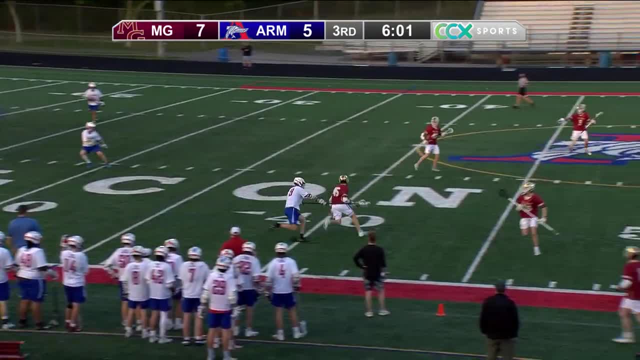 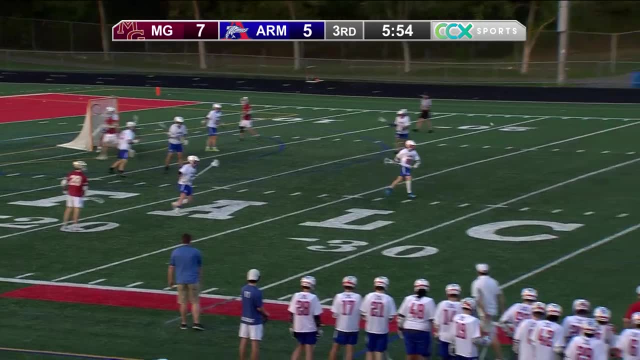 Maple Grove wins The rare face-off with a two-goal lead. Now they have a chance to maybe put a little cushion between them and the Falcons. Scanlon Waits reinforcements from the box. Yeah, the Grove is getting out some of the new kids. 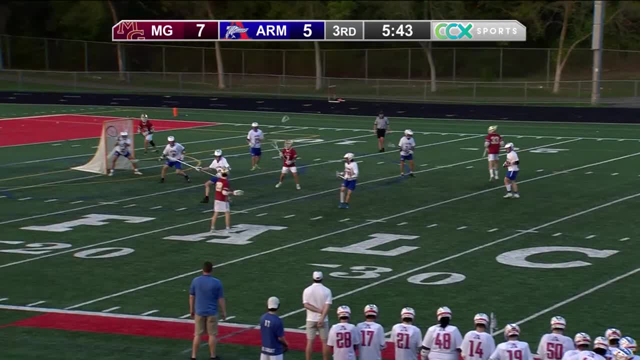 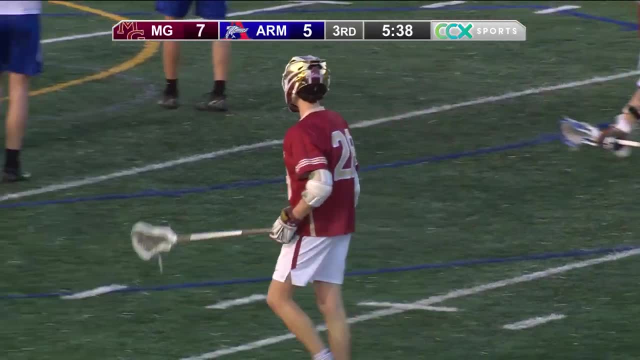 Some are getting tired out there. They've been out there for a while, so we've got some new players. Scanlon steps up and rips. it Didn't close him down fast enough And Scanlon was able to get his shot off. 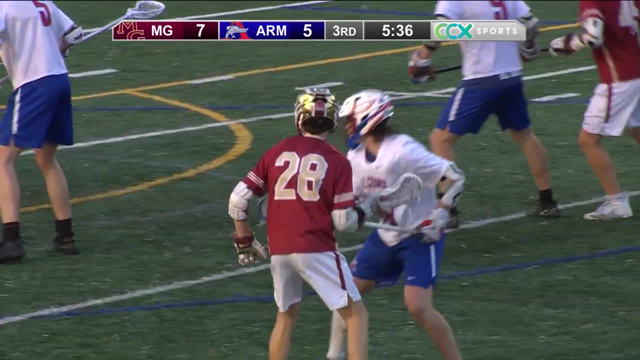 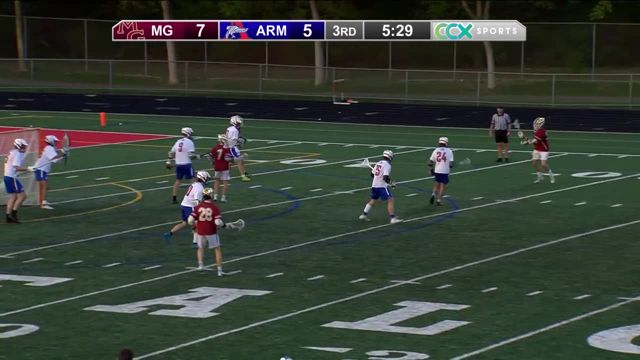 He hit one One like that in the first half, Not that time. Well, he likes winding up. When he sees the opportunity, he takes it every single time. Peterson has his pocket pick by Riley Hansen, but he recovers Brendan on a hat trick. 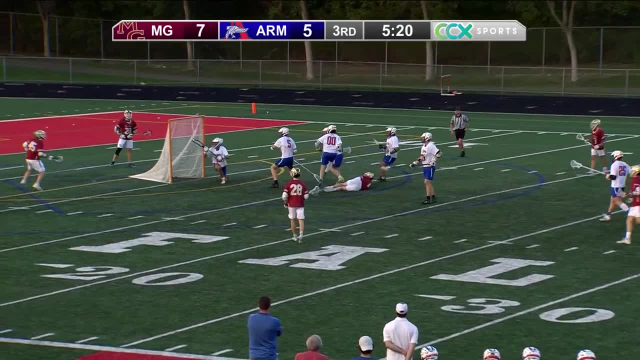 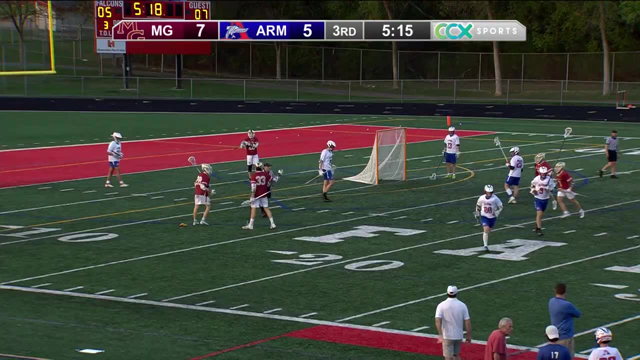 On a third-quarter hat trick, no less. Steinkopf ducks inside, Bounce shot. as he goes to the turf, A flag flies And his shot missed. It was going to be Crimson Ball anyway, But now it's going to be a penalty. 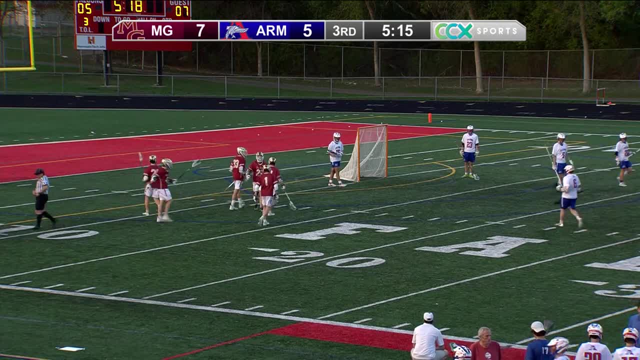 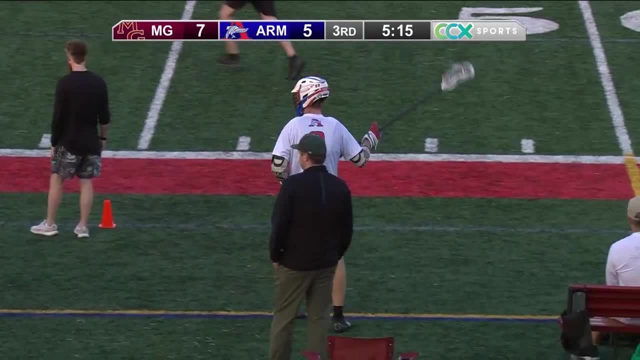 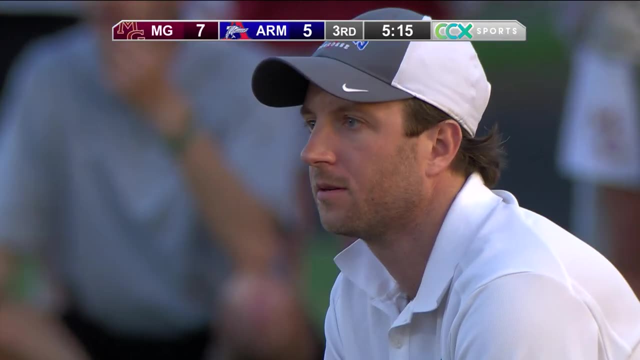 Armstrong taking their, by my count, fourth penalty of the day as number nine, Jonah Pappas has taken a couple of those. He's given his coach, Ian Murphy, something to think about, with Murphy's team trailing by a couple goals here in the third quarter. 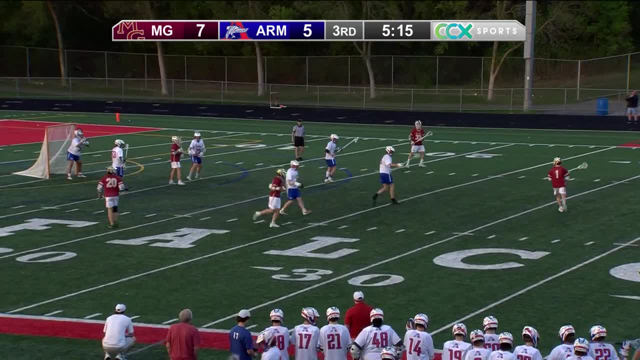 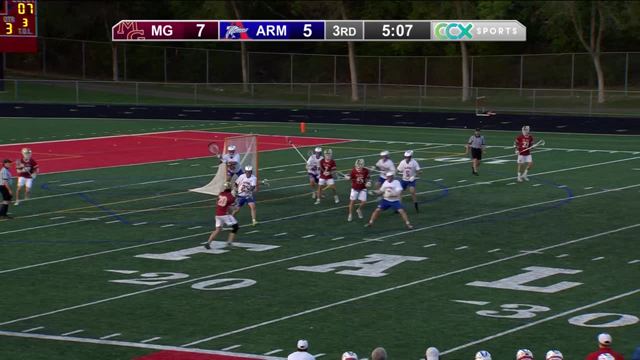 Well, the quickness of the Crimson right now is just kind of beating the long sticks And it's hard to see because of that long stick. A long stick is such an advantage. But Crimson are really quick, Peterson, He's already scored on the EMO once today. 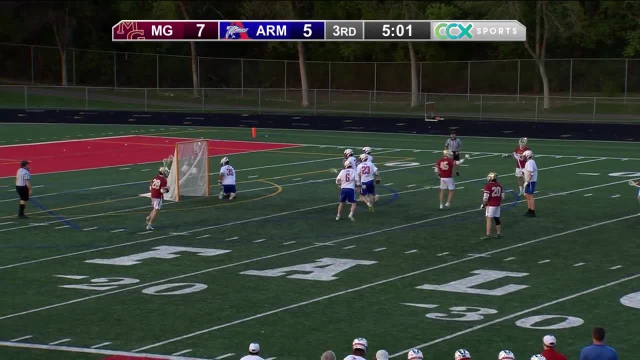 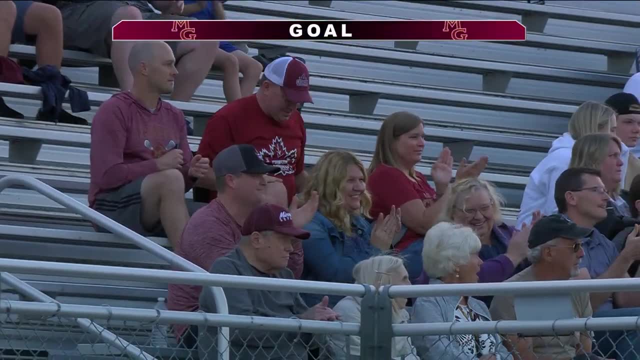 Gets it back. Steinkopf In front, Bakke Bounce shot Scores. Wow, Landon Bakke's got a hat trick. It's another EMO goal for Maple Grove And their largest lead of the game at 8-5.. 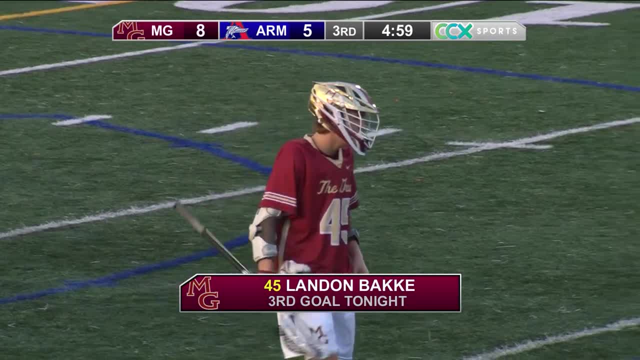 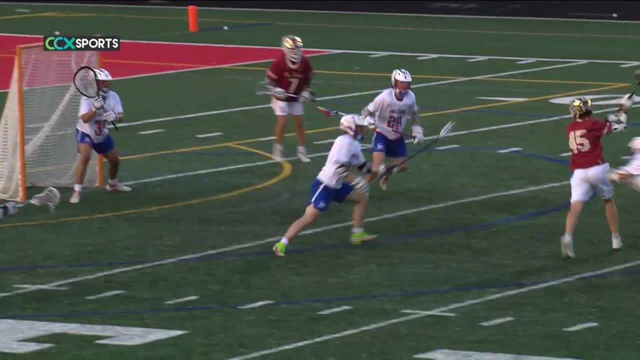 Didn't waste time that time They got that power play rocking and rolling. right now, I think that's going to be Steinkopf Steinkopf who gets the assist, as they're really just popping it around. Yep 8-5 Crimson. 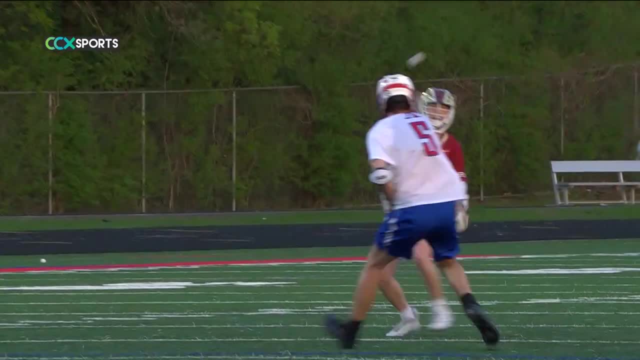 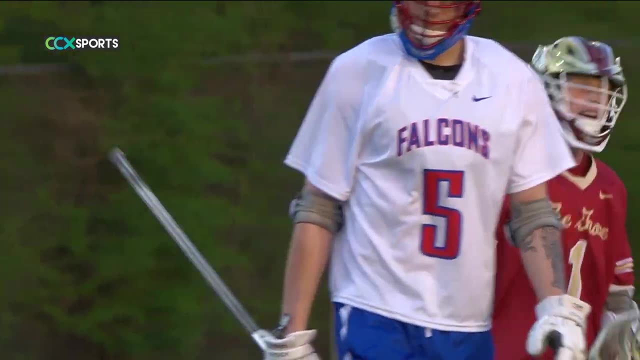 They've scored the last three And they're starting to pull away here on the road Trying to maintain control at the top of Section 5 in the Northwest Suburban Conference. Right Yeah, but they're getting it in the box And you're getting good shots and stuff like that. 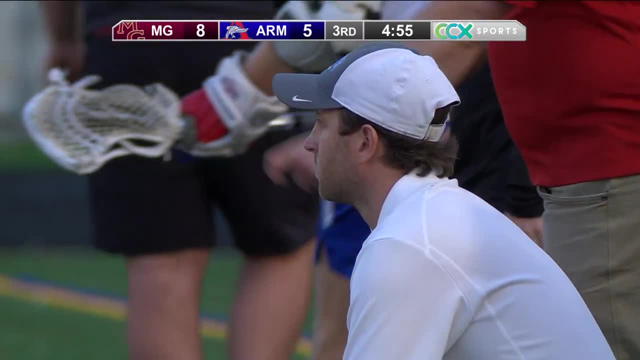 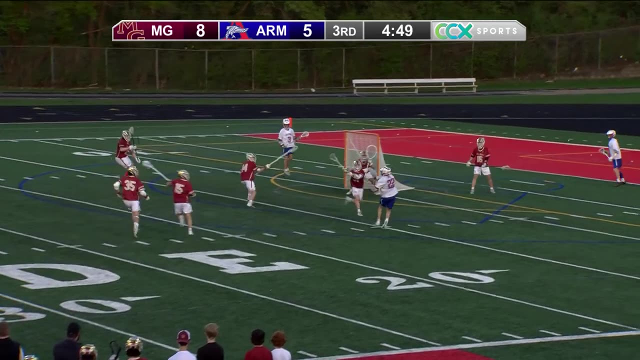 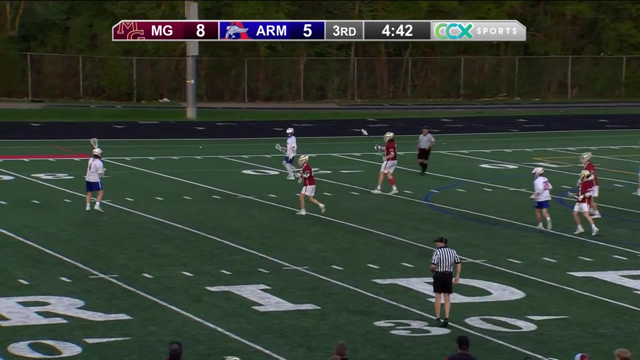 So a nice ball shot that found the 5-hole And Maple Grove loses another faceoff, 11-4.. 14 is Armstrong unofficially. as Essin gets a step, Goes back, Coe puts on the brakes. So Essin, I thought could have maybe taken the shot there. 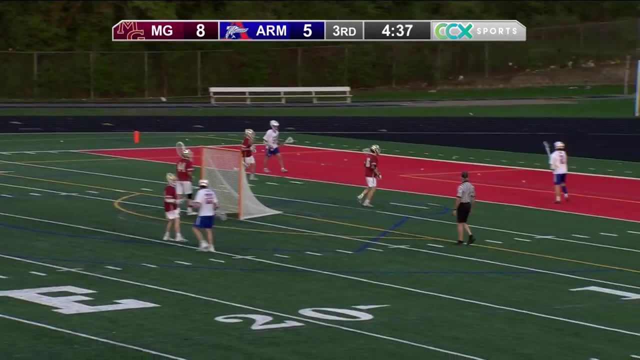 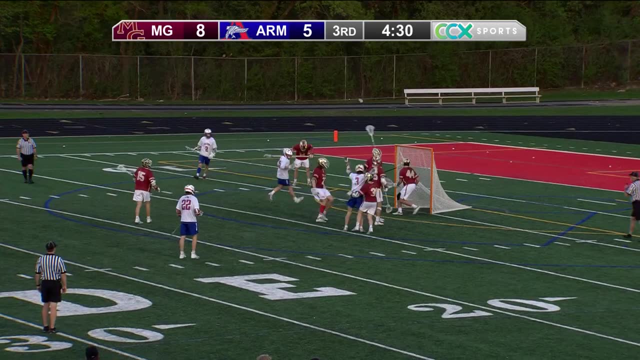 But he decided to pull it back And Annis resets for Olsen behind Albrecht, who's got a goal tonight, for Olsen Fakes Scores. Beautiful move by Jack Olsen, His second of the quarter And his 22nd. 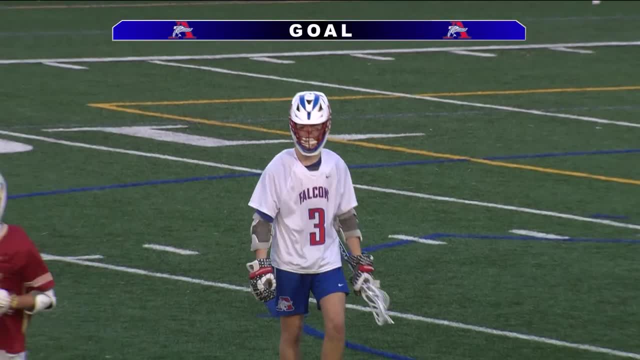 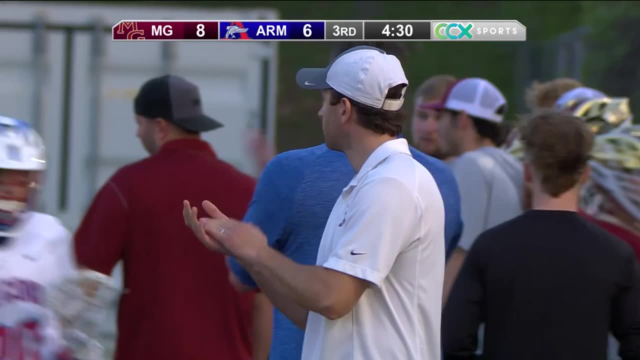 Second of the season. You know what's scary here, How good he's going to be. Yeah, the stick fake Got Farniak down And he just deposited it right over him. Man, oh man. He has been very impressive for the Falcons tonight, boy. 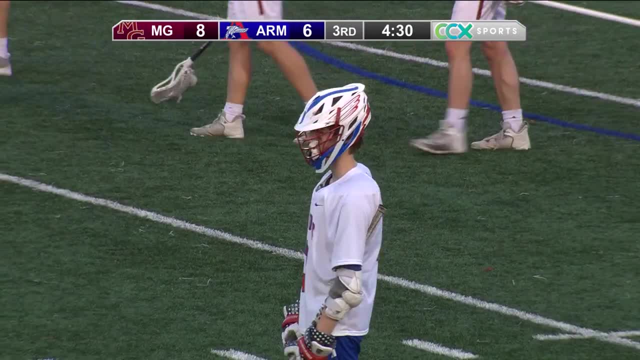 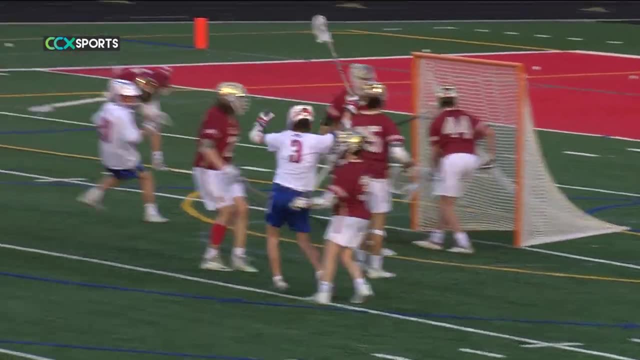 I'll tell you, Olsen has been really good. He's got both of the goals here. Oh, great move there. Just he may fake the pass And he came back around and got it off real quick. You'll see it Here. 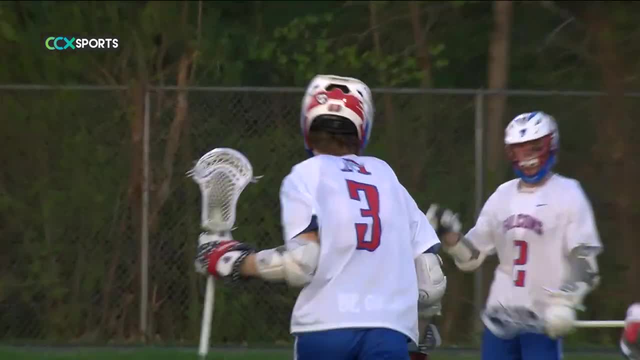 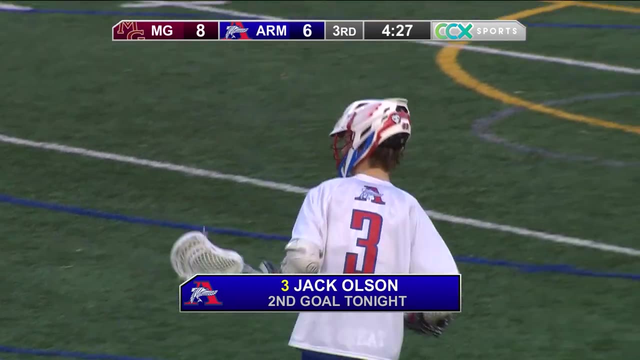 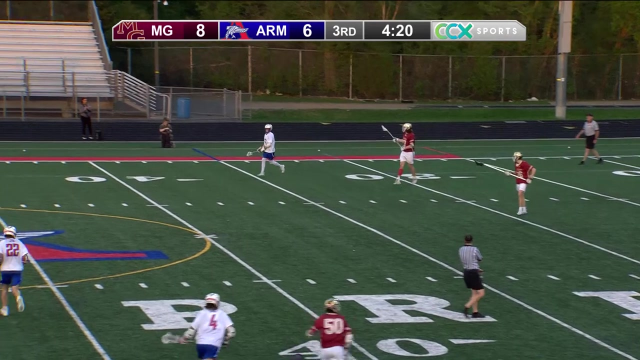 Fakes the pass Bang, And then Farniak goes down, Just puts it right over him: 8-6. now That ends a three-goal unanswered run by Maple Grove And the Falcons. I'll tell you what Winning these face-offs for the Falcons is going to keep them right in this thing. 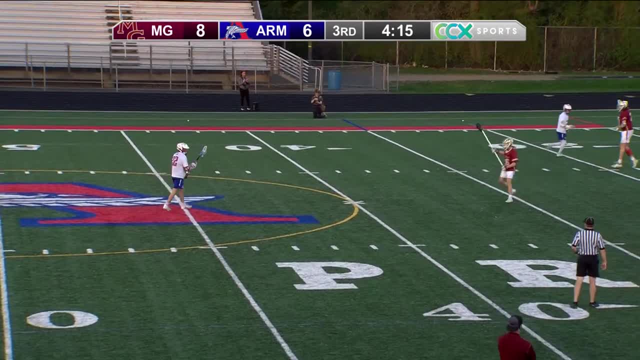 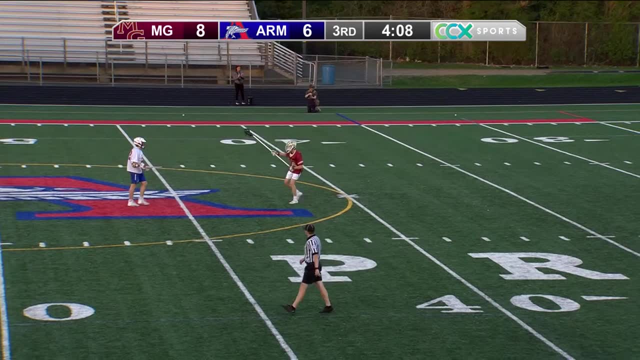 And they'll work their way back. I mean, they're winning them pretty much. what? 80%, now 90%, Yeah, more than that, Whatever 12 of 15 is. Oh man, Oh man. 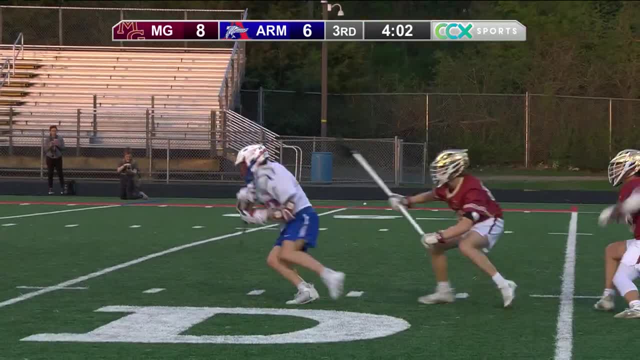 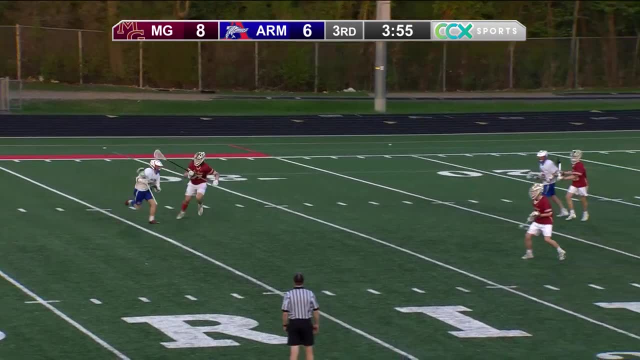 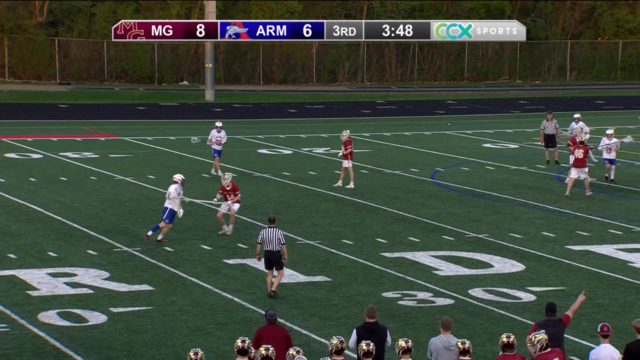 Essendon attacking downhill. He backs it out. He's on a hat trick. I'd like to see Albrecht more involved in the offense here, as Bennett has him. Albrecht, He's so slithery, just kind of slaloming in between defenders. 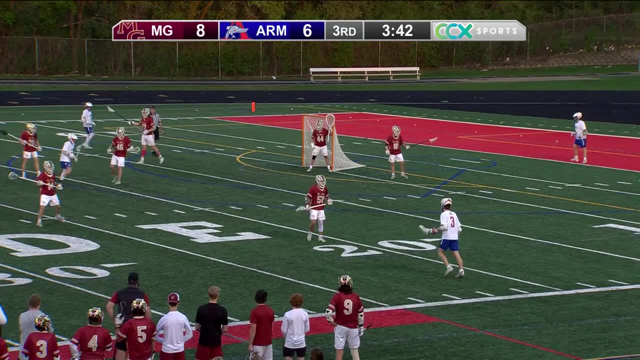 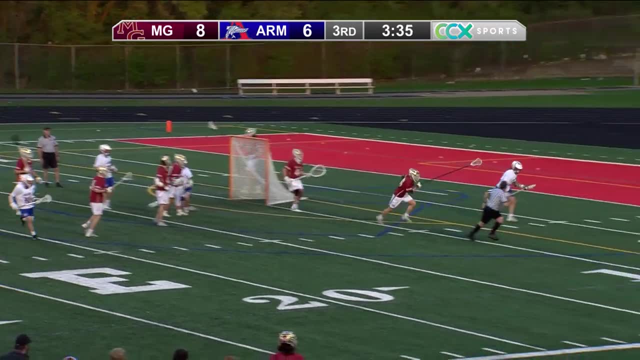 Yeah, you notice he's usually got a real good stick, Usually a big stick on him, Usually the D's on him. They got him pretty well. They know about him. Olsen thought he was trying to get it behind for Coe. 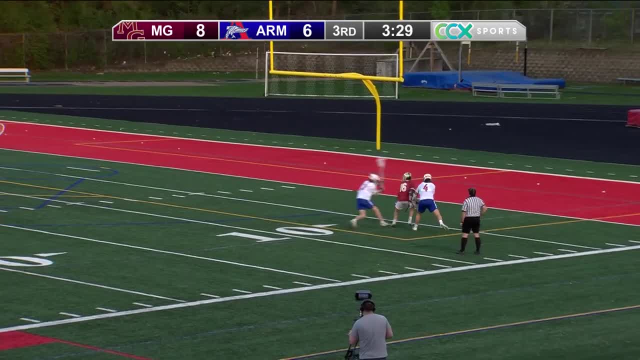 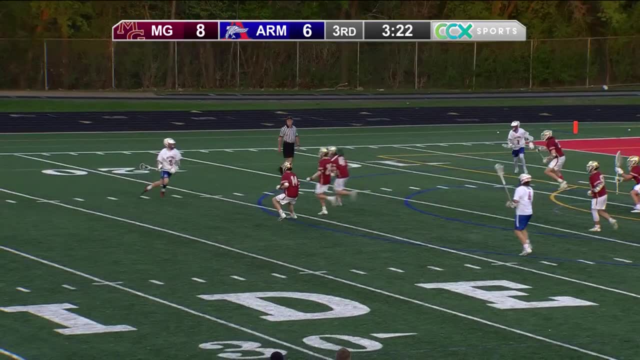 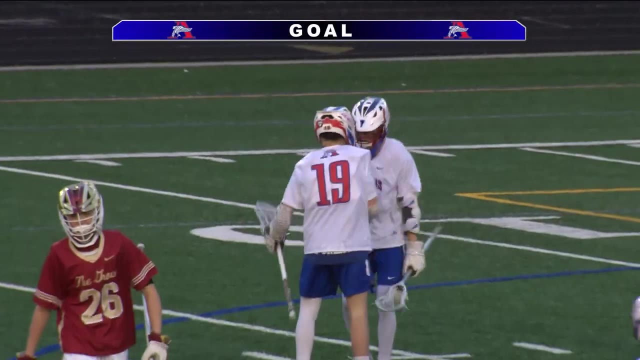 Coe battling for the loose ball. but first to get to it is Rask, And then it's intercepted behind the net. Annis thought about it. gives it back for Albrecht. He feeds a cutter, Nice move. There's a shot and a scar by Brainy Northrup off the great feed from Albrecht. 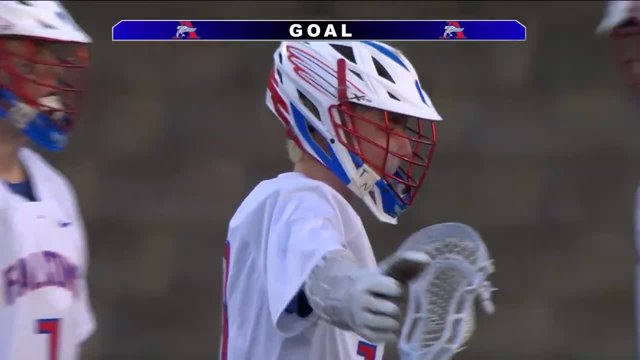 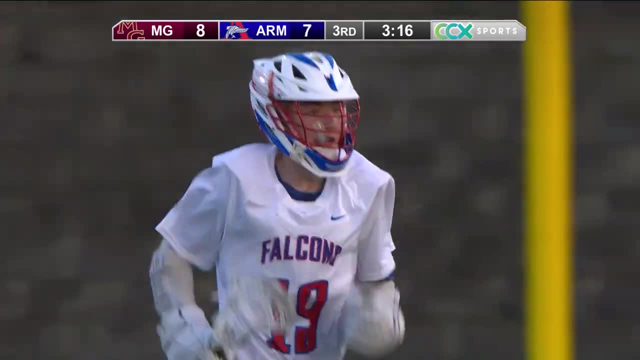 Yes, What a beautifully designed- not even designed- play. just an improvisation from Armstrong, And they've cut the deficit to one goal. Get their eyes up and see what's going on. Created a nice play there. Everybody's in the right position. 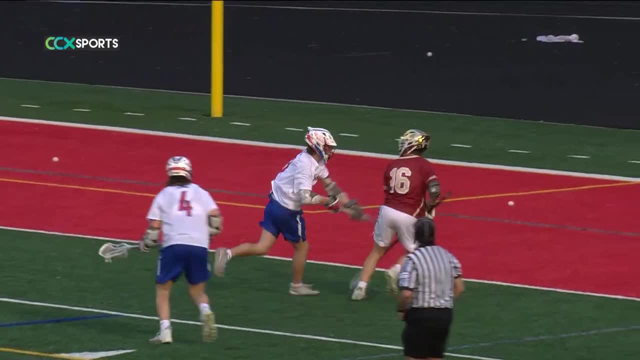 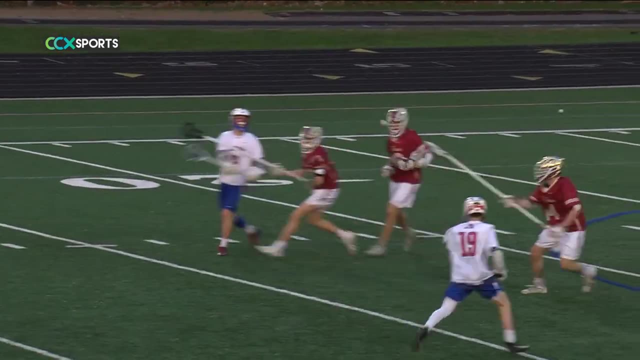 People are cutting. they're using stick fakes. as you see. this, Stolen initially by Annis, thought about it, decided against it. Albrecht faked it, drew the defense and a nice job just to evade on rushers by Northrup. 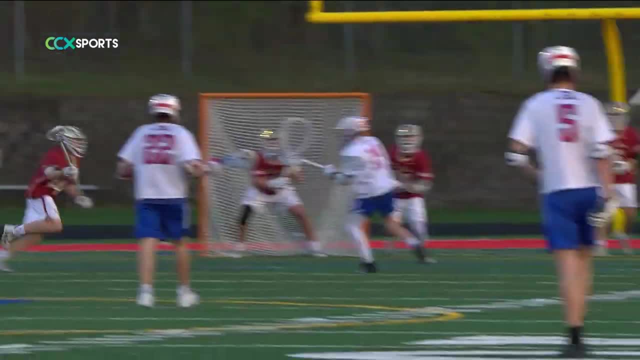 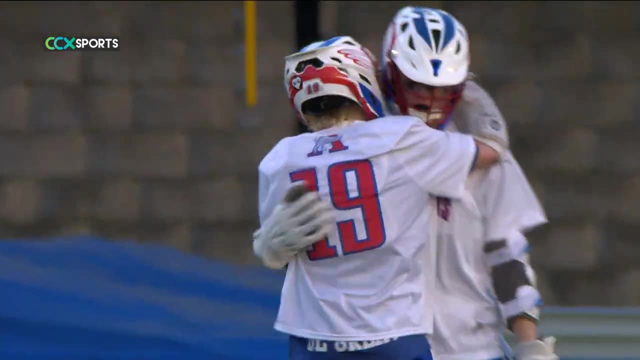 Scores his ninth of the season. right there, That was good defense all the way through. He just made a great shot. Yep Albrecht gets the helper. 8-7 the score. This time Maple Grove wins the face. but what unselfishness from. 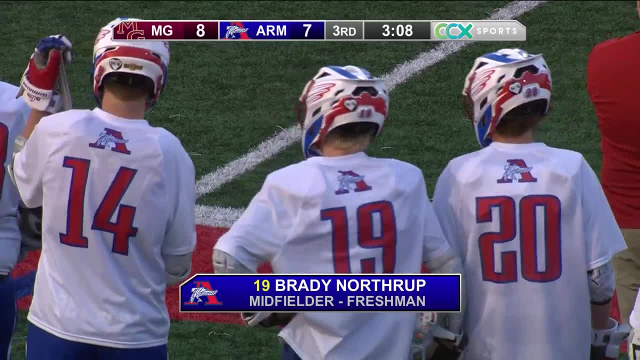 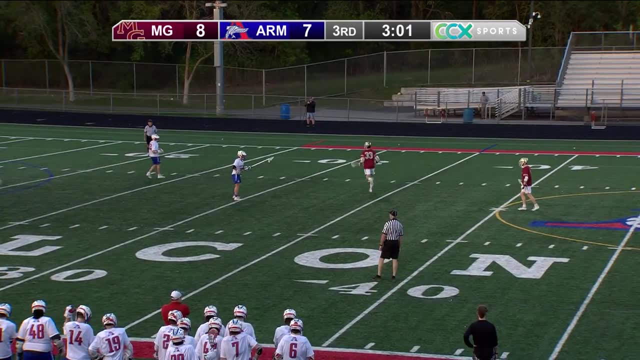 Wow, That was the freshman midfielder with the blonde hairdo. Well, you sure can tell. you know, these are the top teams in the Northwest Suburban and they're playing like it. Man, this has been fun. Yeah, this has been. 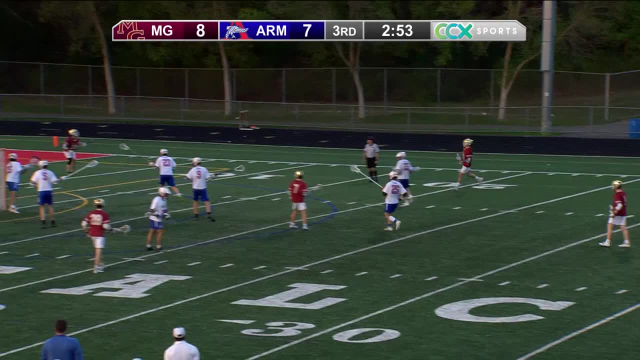 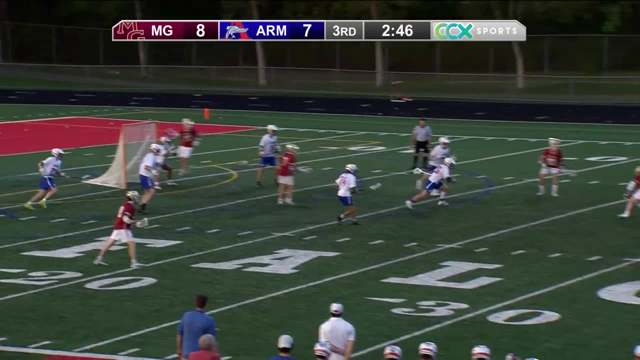 I can't keep saying it. It has advertised, but it has been back and forth. Peterson tries to get that defender hung up on the net, Feeds out high Anxious to get it to Steinkopf, Only for the move. 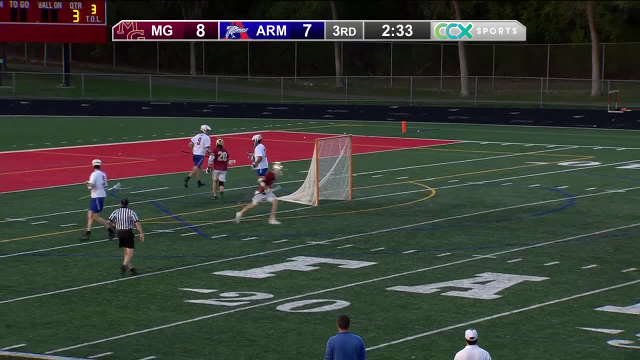 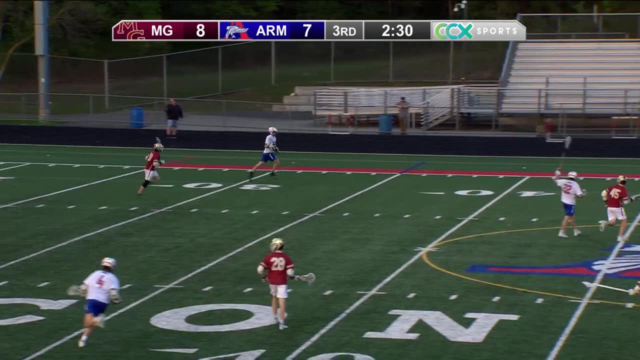 In the crease Peterson Crease violation as he was looking to make the pass. Kind of amazed that we don't see that more often. Yeah, Given, you know how guys are. They're just looking up when they're dancing at X. 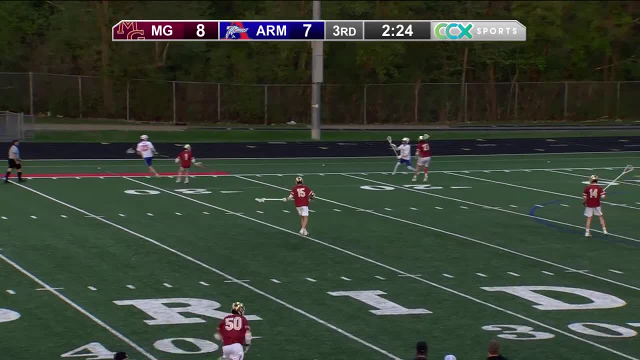 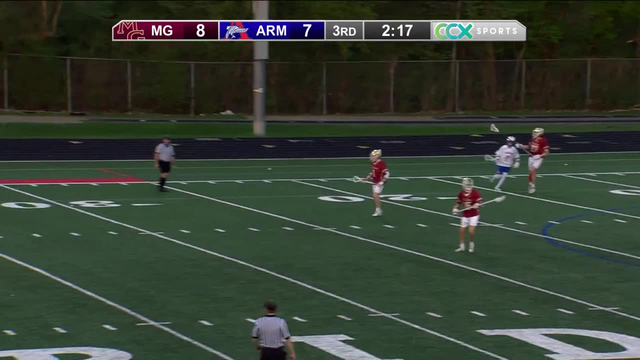 Oh yeah, I think. over the years, though, too, They've gotten used to this game. We used to see a lot of that. We don't see too much of that anymore. And the spatial awareness and the Mm-hmm. 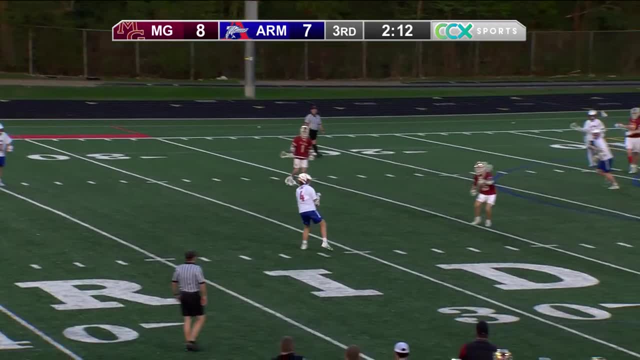 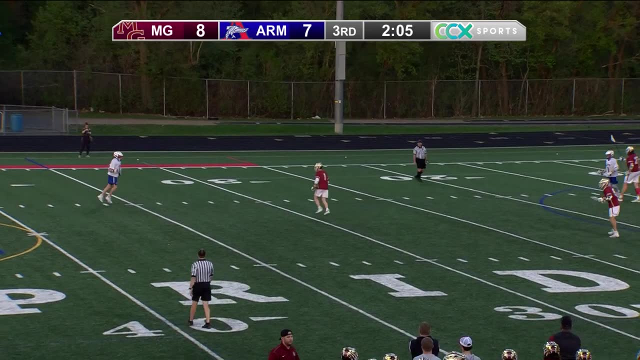 Yeah, There's no doubt about that. Asson over for Cole. Oh yes, Armstrong has answered Maple Grove's three-goal run with two of their own, and now they're hoping to tie the game late here. third quarter Essin. 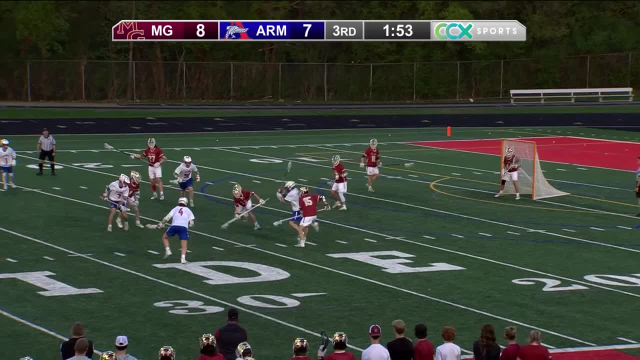 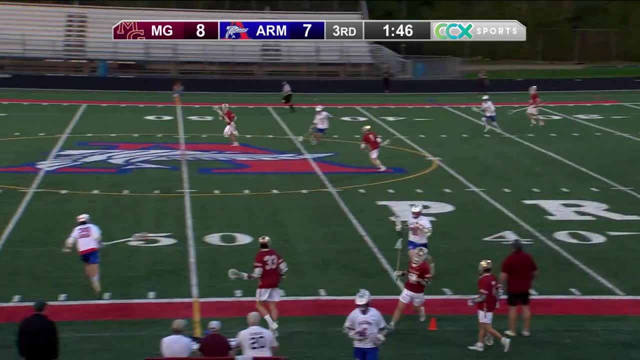 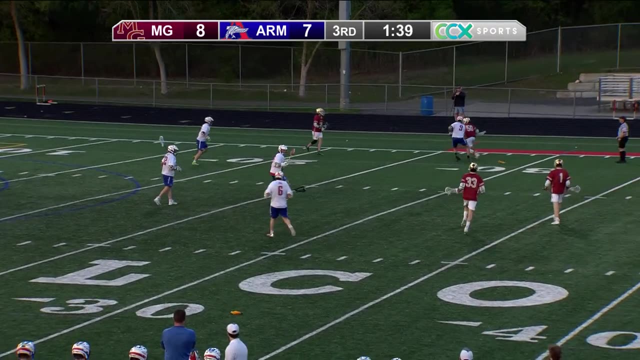 Olsen, who goes down, recovers, Thought about a shot. Steinkopf knocks it away from behind. Great defense by the Crimson Outleted to Steinkopf In transition. here's Leisner. Now a flag flies. 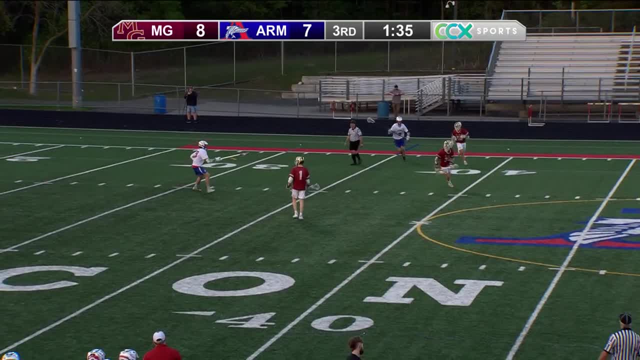 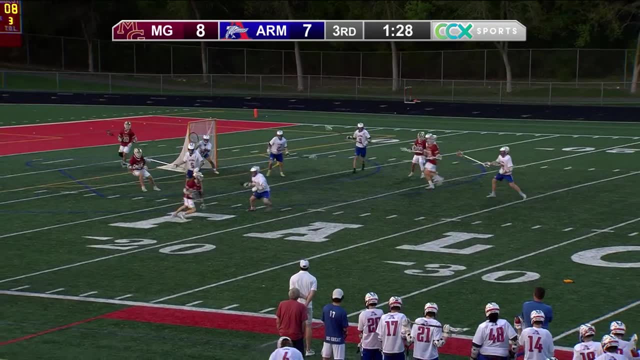 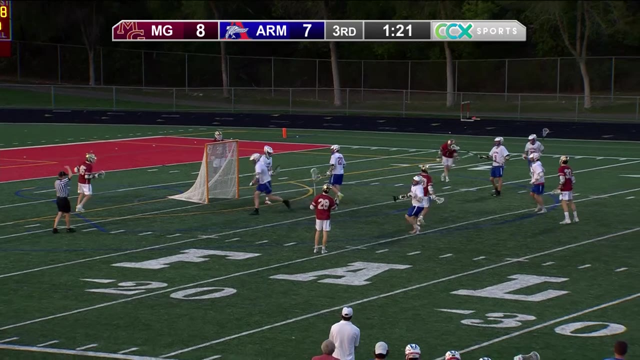 A couple. So it's going to be an EMO once more for Maple Grove Here late in the third quarter, Even though nobody leaves the field, you still, You can make a mistake and you won't cost you because they can't score. 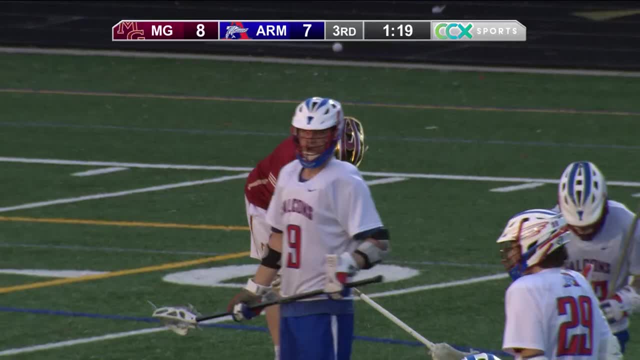 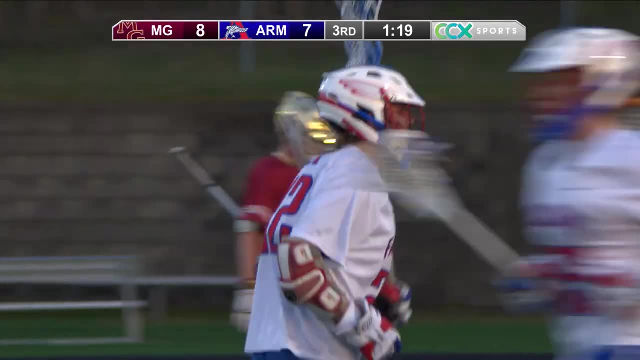 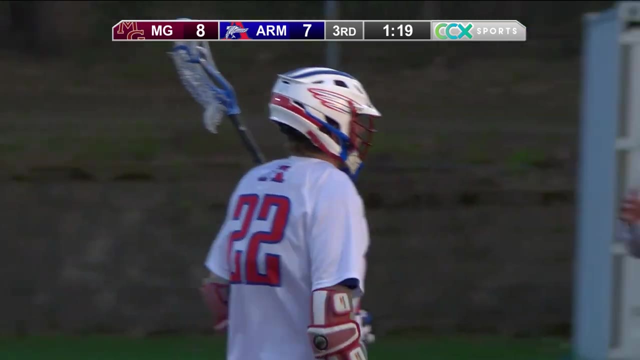 Steinkopf jump shot caught by Wells. But it's a penalty Fifth of the game on Armstrong And still going to count that as a save for Wells? Absolutely, But that's Essin's second infraction of the game, I believe. 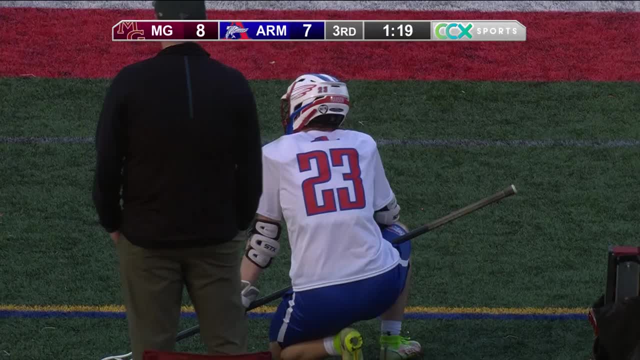 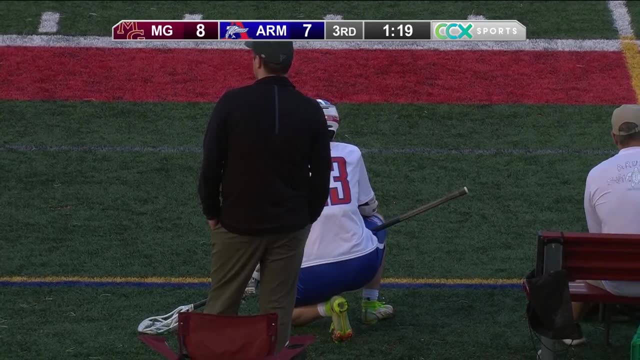 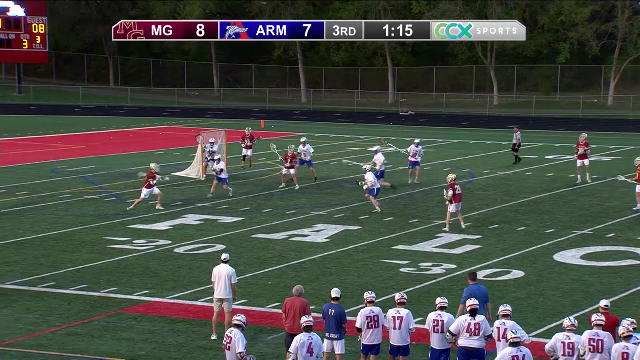 And with 119. Left in the third. Oh, I beg your pardon, That was on Riley Hansen. Ian Murphy certainly disagreed with that call. Slash to the head. That always gets called, it seems. It touches the helmet, no matter how gentle, it's a penalty. 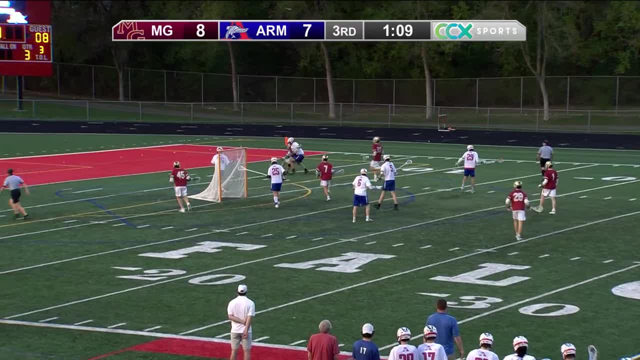 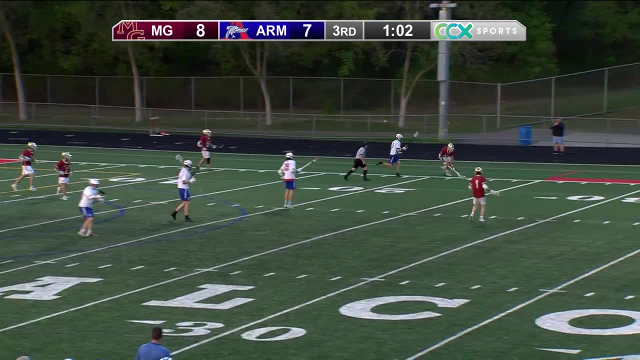 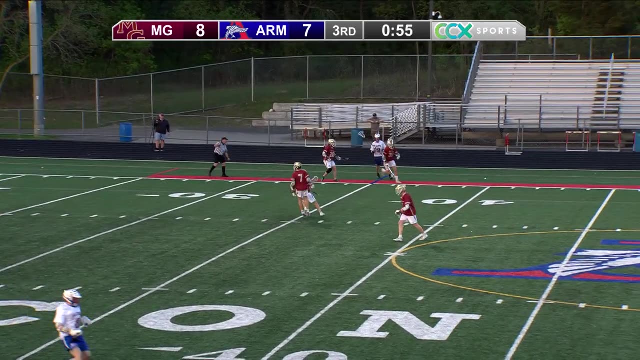 Period: Yep: Brandon For Peterson- a little high Peterson battling with Pappas. Good team ground ball work. Brandon Trying to add to his two-goal total here in the third quarter. Pappas spinning away And he's immediately forced out. 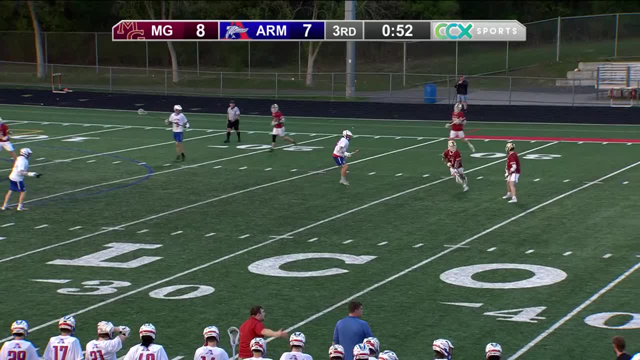 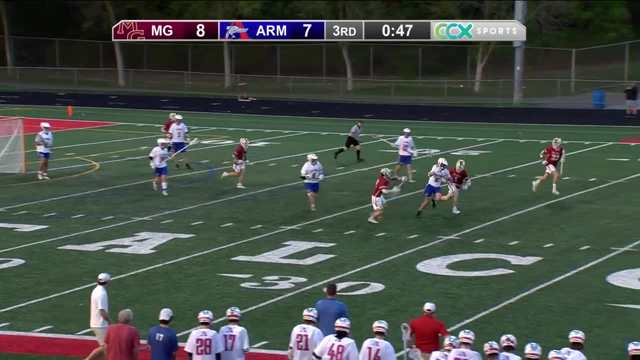 You've got to be jumping off that whistle, Oh man, If you want to take advantage. 50 seconds remaining And there's a shot, And it just hits Pappas out in front. Pardon, Aiden Robb Robb in transition. 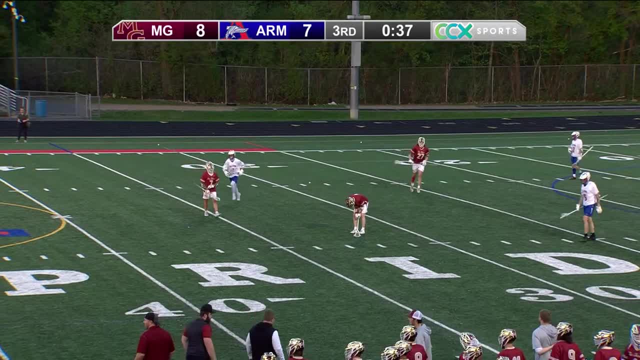 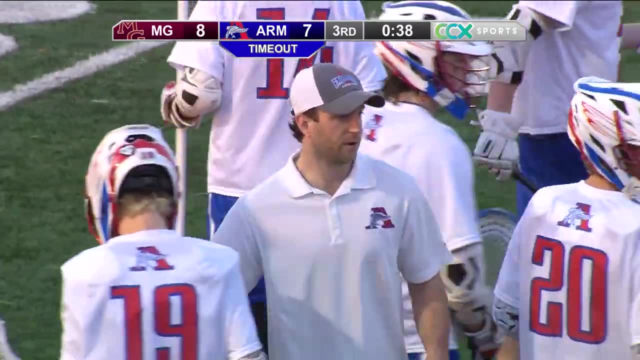 Now it's going to be a timeout by Ian Murphy with 37. Seven seconds left And I think a good timeout. Yes, Great call by Coach Murphy. Get him some of that. Yeah, Now how do we maybe get a goal or at least kill off the rest of this quarter? 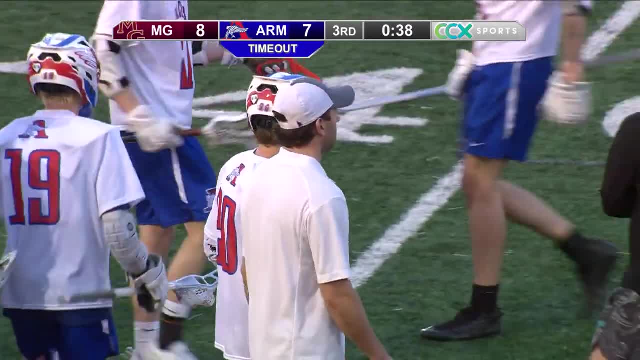 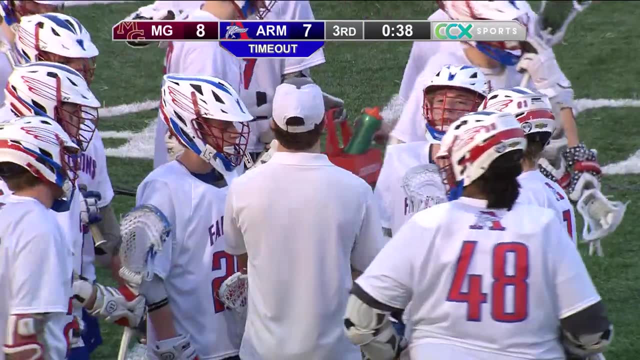 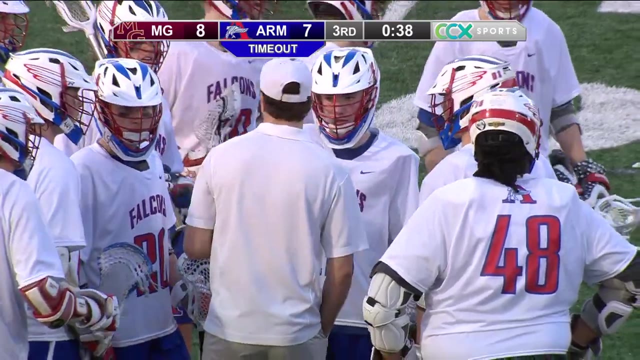 First of two second-half timeouts taken by Armstrong Stops the clock with 38 seconds remaining in the third quarter. Well, we'll look for the clipboard here and see if they do a set play. Certainly want to just get it in, maybe in the sticks of your best stick handlers. 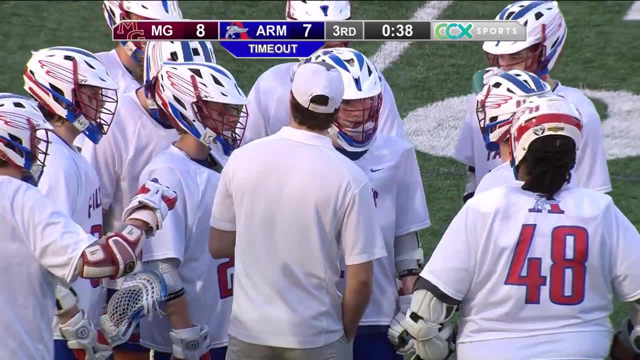 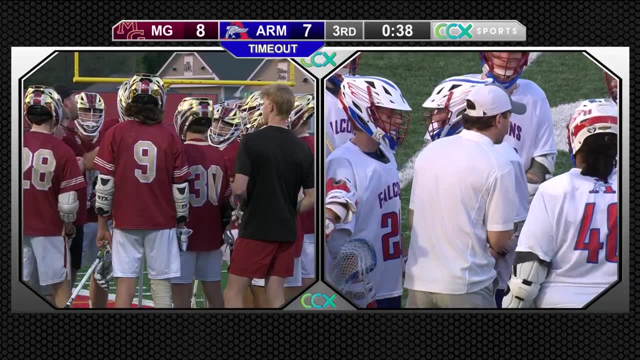 Well, they've been very good. They've been very good about getting Essendon into the box about 15, 20 feet out and letting him rip it, And he's been very effective there. But I would look for something like that from the Falcons. 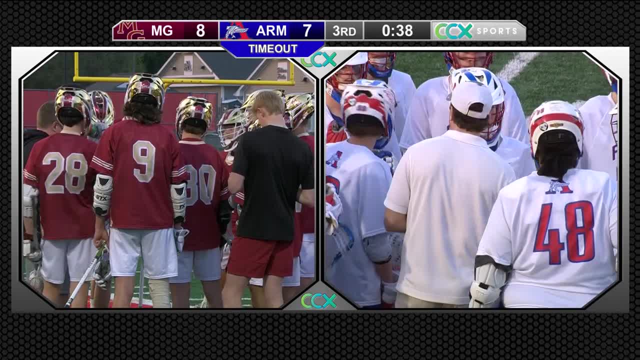 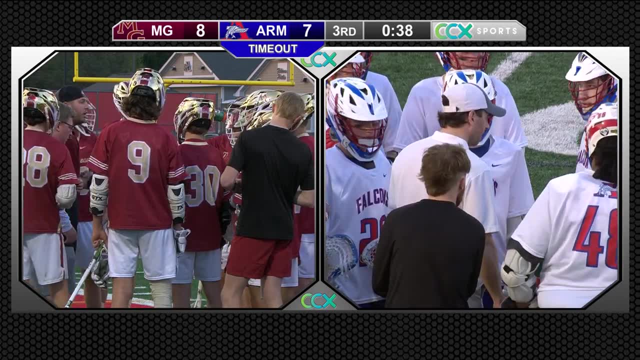 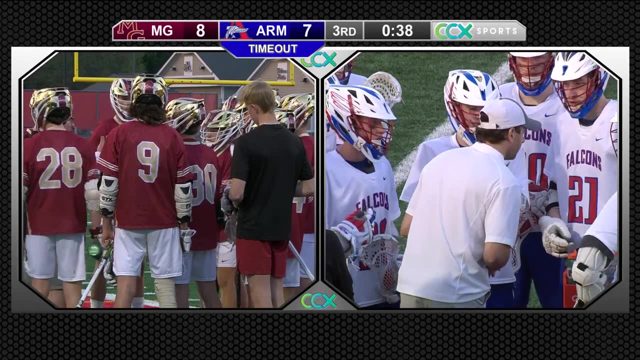 And try to get this game tied up before the half ends. Both coaches and obviously lacrosse- One of those unique sports where each coach sort of talks to the offense or the defense. There's two huddles on each sideline With an offensive and defensive coordinator and the head coach. 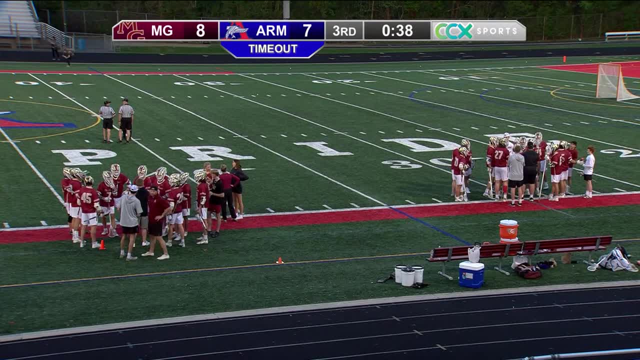 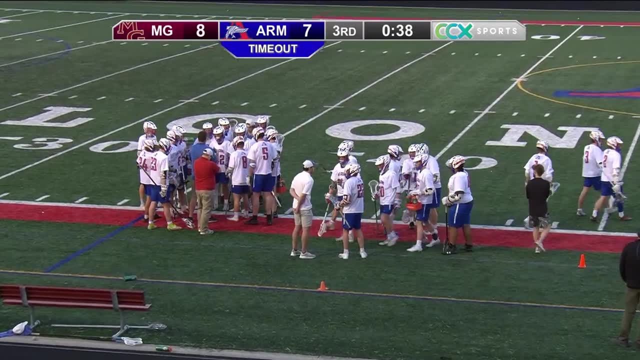 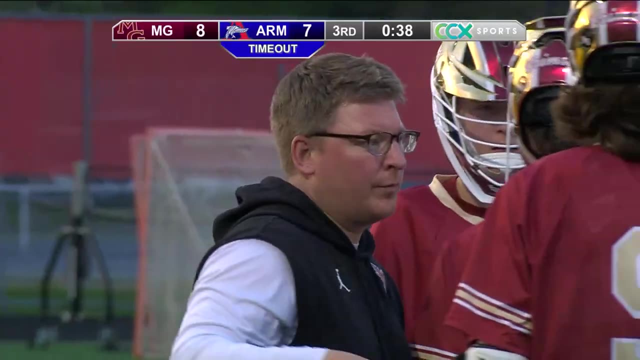 And you were saying before the game that your son Kyle knows Ian Murphy And they used to play together. Yeah, when Kyle came back from North Carolina, him and Ian played in the Minneapolis Lakers, the men's team in lacrosse here, And yeah, they know each other pretty well. 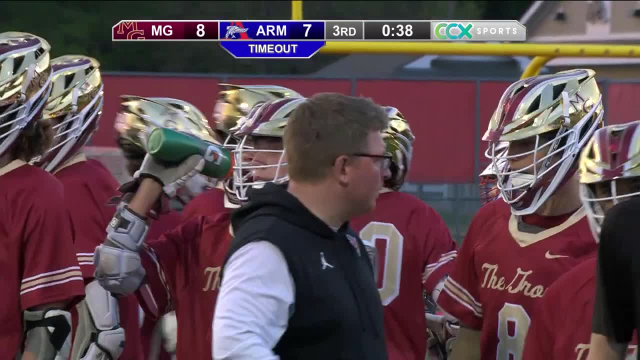 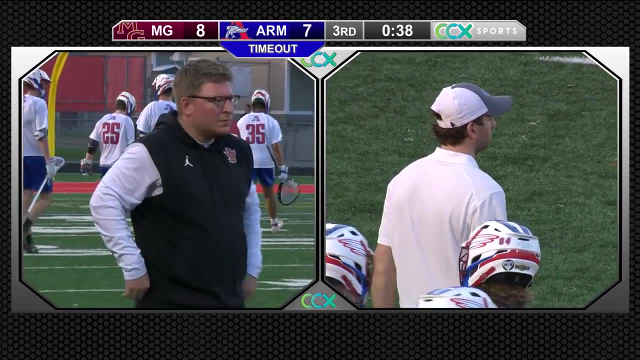 They always look forward to getting together because they aren't friends during the game, But afterwards they'll probably go out and have a Coke or two. Sounds good. And yeah, lacrosse is a small world right Between club and high school. 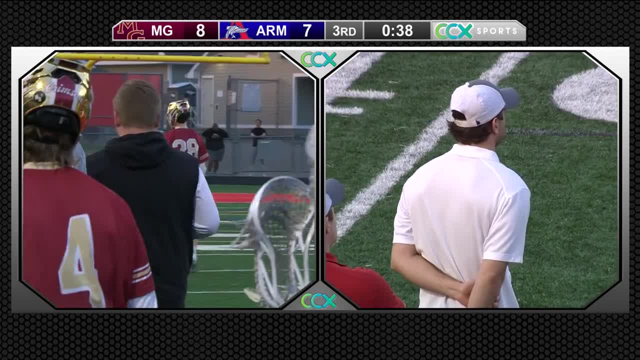 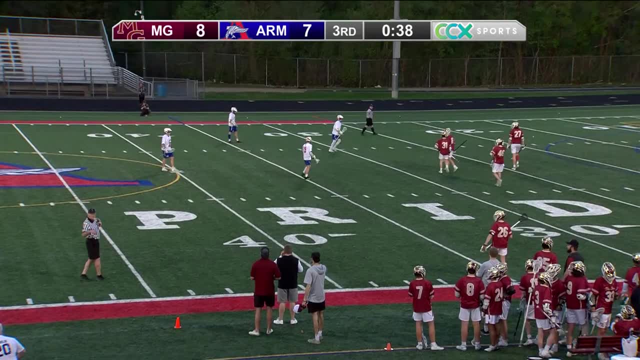 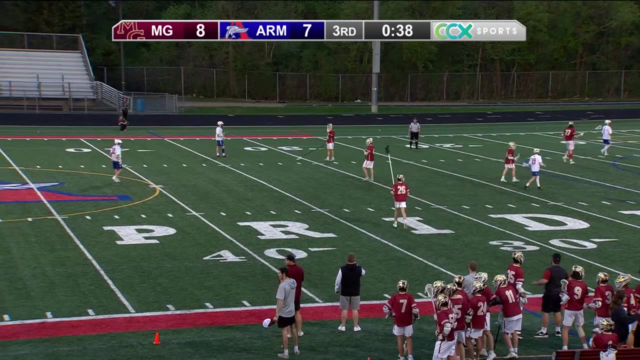 A lot of these coaches know each other, have coached a lot of the kids, So a lot of times you know from club and whatnot- whether it's Team Minnesota or any of the other clubs, which a lot of times you can take what you know from the club and apply to defending in the high school. 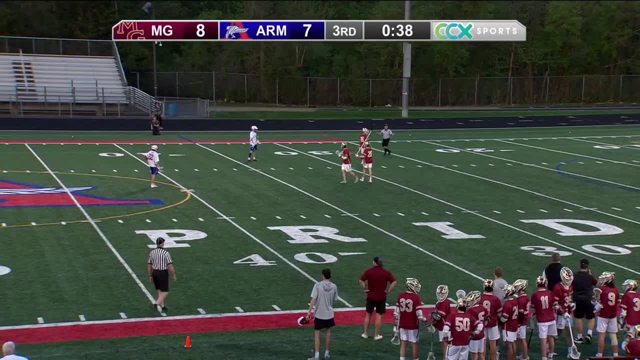 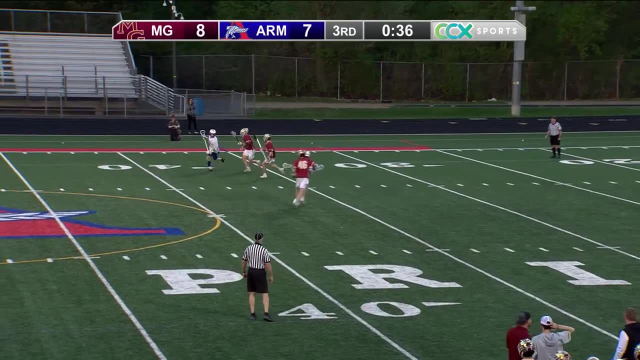 Yeah, and what's happening now is that a lot of these kids like Kyle back from college- NC2A lacrosse, where they're getting some coaching out east to really find out the game, And it's coming back here And our game in Minnesota has improved so much here. 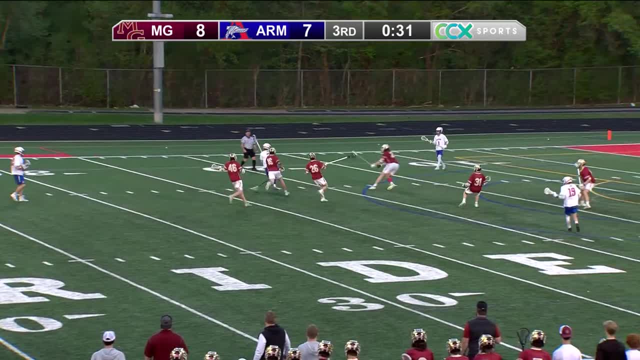 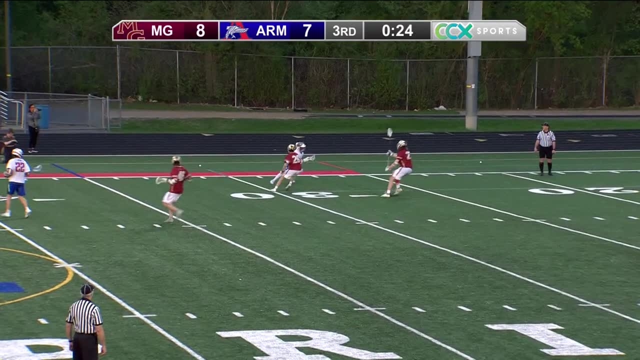 A lot of kids now are getting opportunities to play out east Albrecht spinning his way through multiple Crimson defenders and still possessing the ball Boy. Albrecht and Essendon are the real deal. They can play. Yeah, they really can. 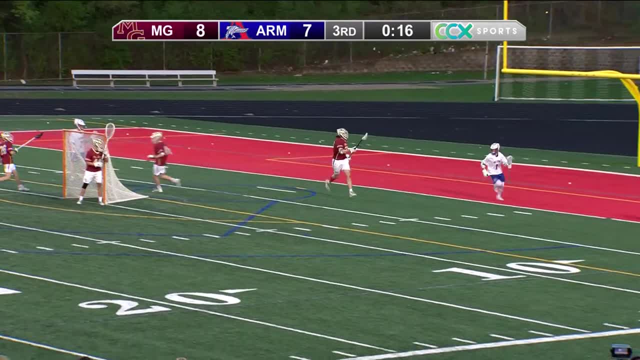 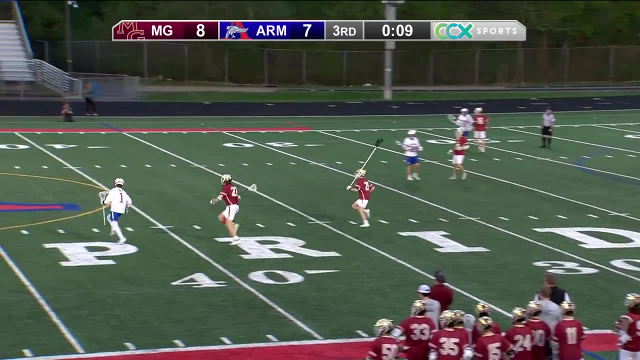 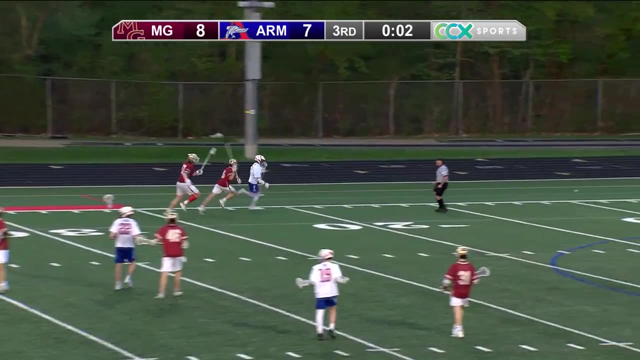 Now it's Frankie Annis. We'll dance around with it, probably content to just run this clock out Here as the third quarter is coming to a close. Annis just circling the field getting his steps in as time expires here in the third quarter. 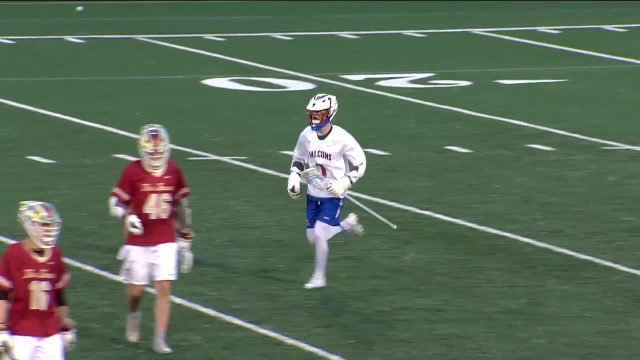 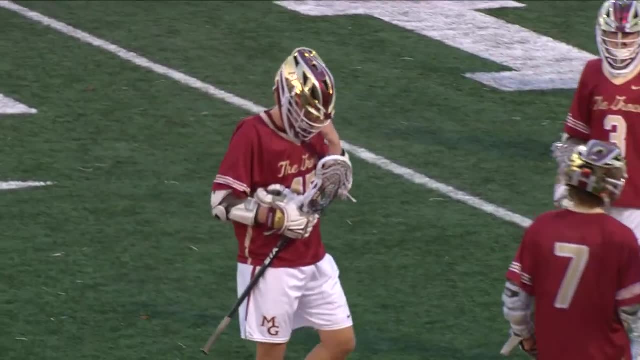 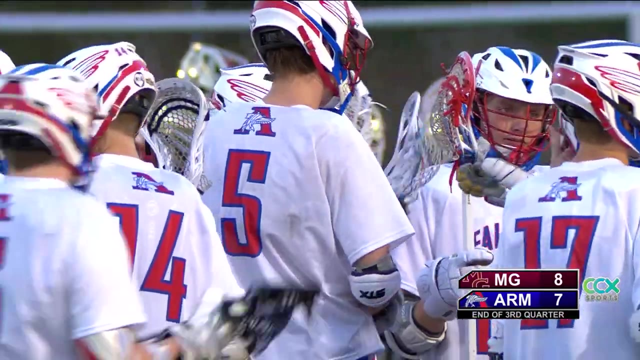 The Annis Marathon. Well, Maple Grove rattled off three goals after Armstrong had tied it at five. But Armstrong answers with two more And we head to the fourth quarter of play with a one goal game. As we expected here in Plymouth, 8-7 Crimson leading the Falcons. 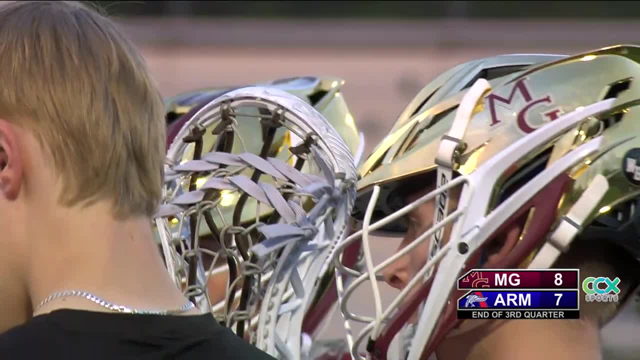 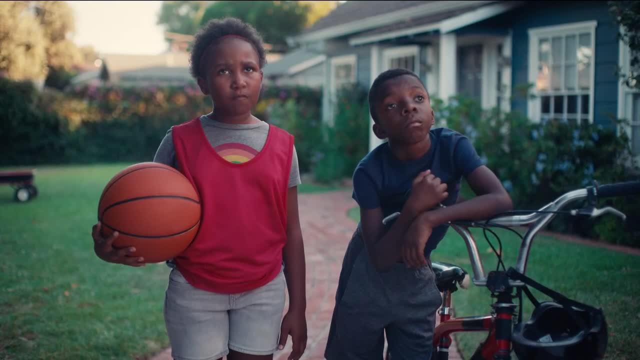 Don't go anywhere, folks. Back in a second here in Plymouth on CCX. Honey, what I think you need is a socket wrench. I play JV basketball. I'm sorry, I don't think it looks right. This is good. 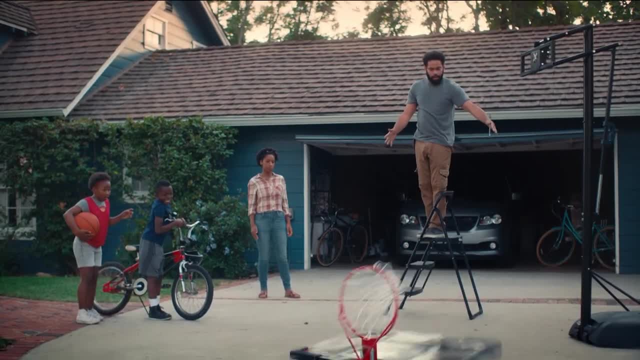 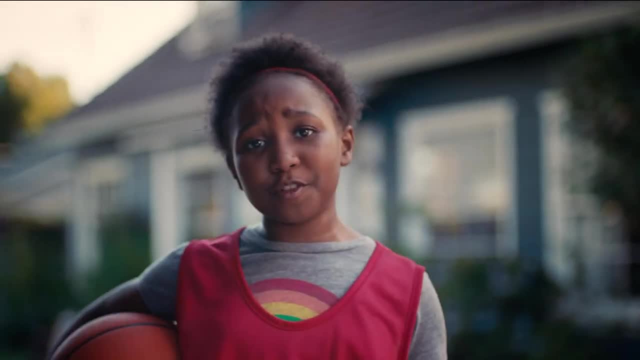 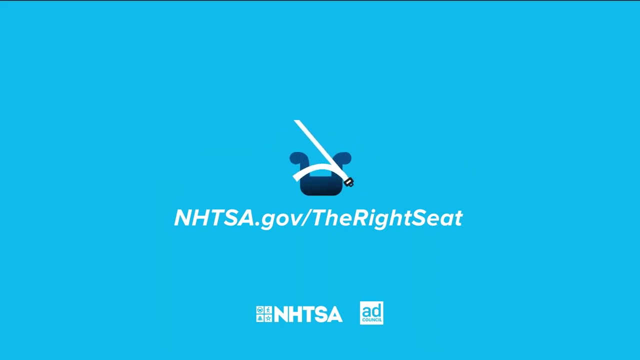 And it's all good, baby, Is it really all good? Ah, If you love me enough to routinely test your handyman skills, not to mention the strength of your marriage, then of course you'll visit NHTSAgov. slash the right seat to make sure I'm in the right car seat. 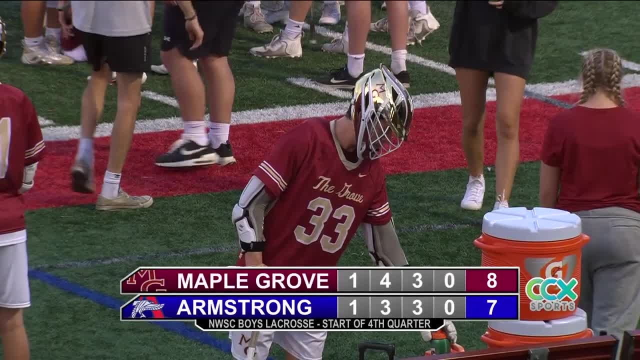 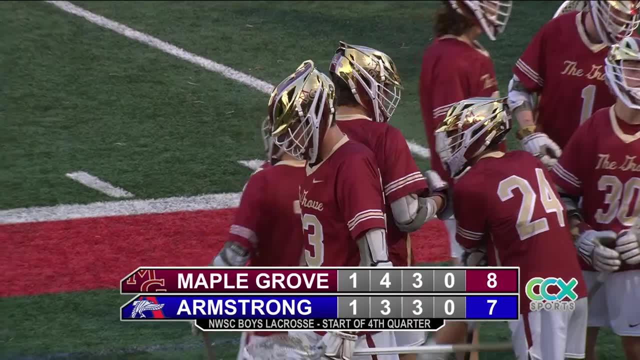 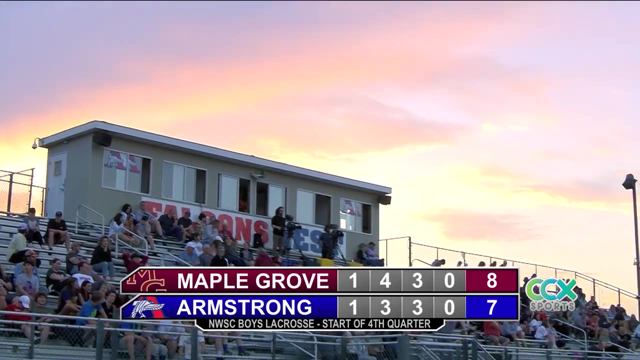 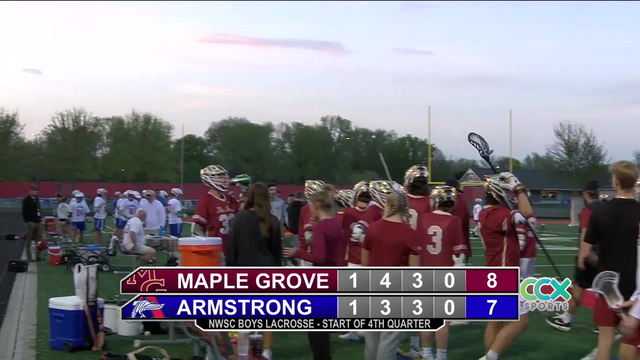 I'm going to call my dad, Tanner Brendan, with two goals in that third quarter, Each team scored three and we remain where we were at halftime Having this beautiful night for lacrosse in Plymouth here. And how we were at halftime was Maple Grove leading by a goal. 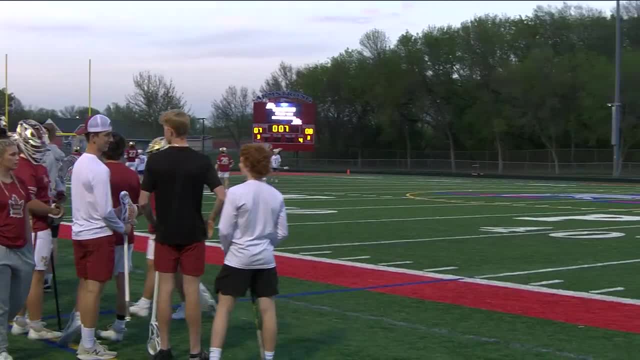 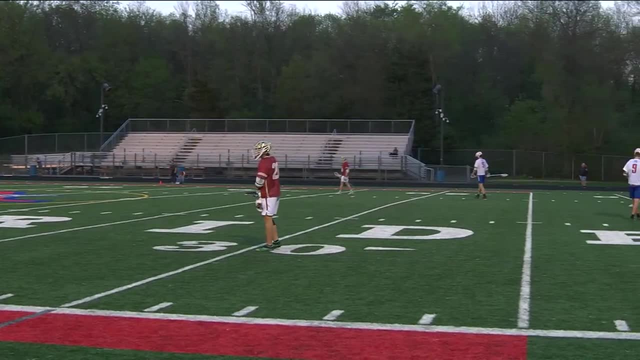 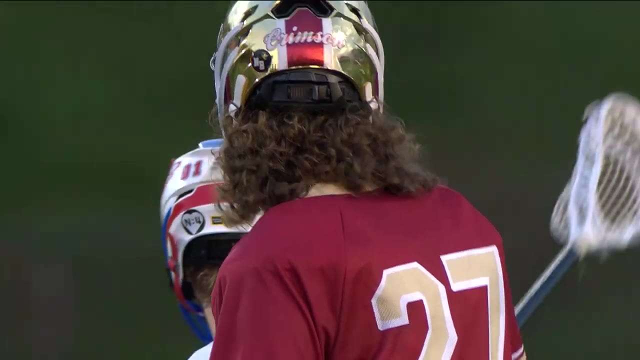 And they do so as well here. First quarter was really more defensive, and it's because of the saves the goalkeeper tenders did that we only had a goal apiece. But then things have started to open up a little bit more: Four goals for Maple Grove in the second, three for Armstrong and then in the third each team with three goals. 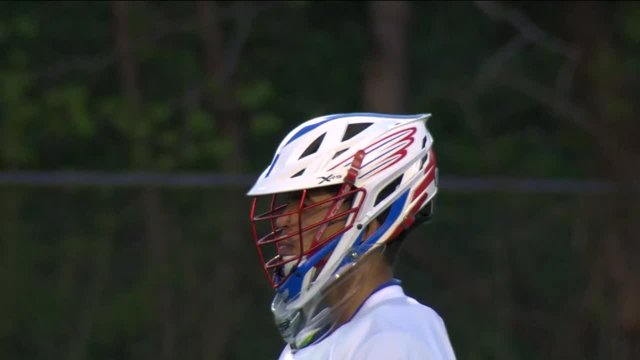 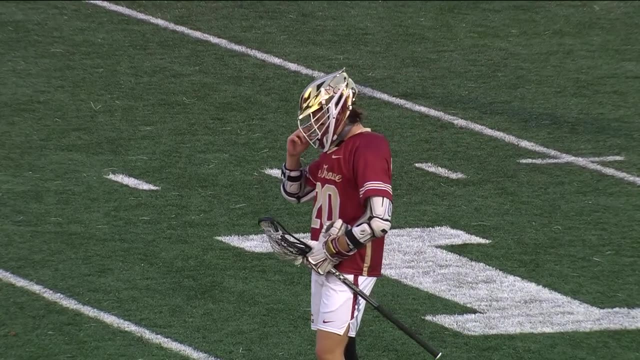 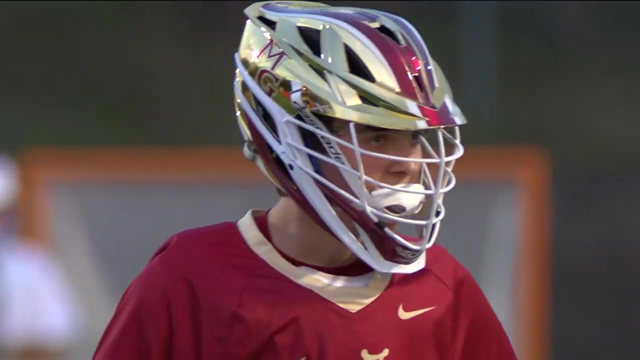 And what will we see Here in the fourth quarter? Dan Ficken- Only time will tell, but we're both looking forward to seeing it. as Xavier Wells and the company go to work, Peterson trying to beat him. He who done gets the best save, the right save at the right time- is going to win this game. 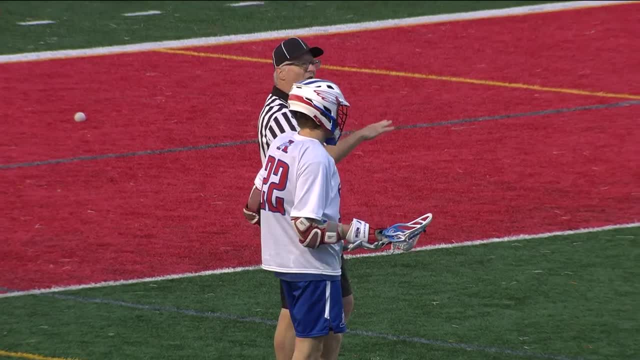 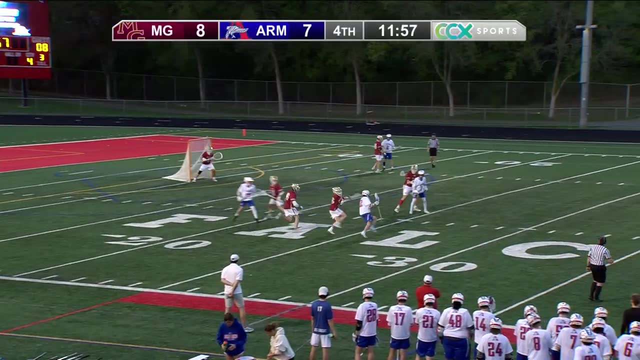 Because it has been offensive-oriented, But actually both goalies have been really impressive too. I mean, we've gotten a little bit of both defense and offense on both these teams- Yep, both teams scoring Ascension, just trying to run out this penalty. 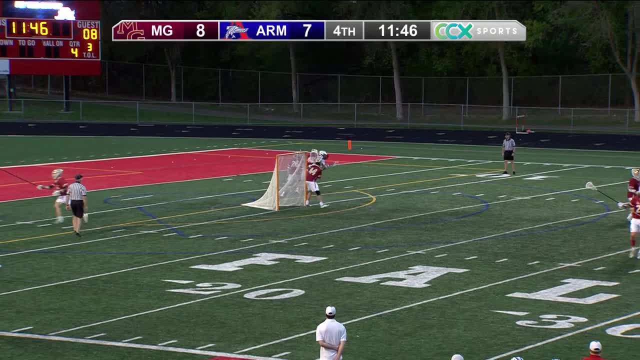 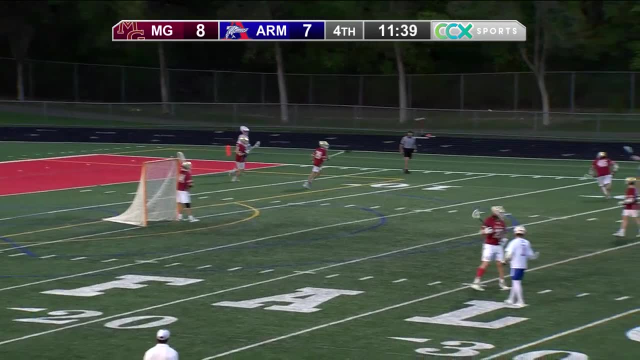 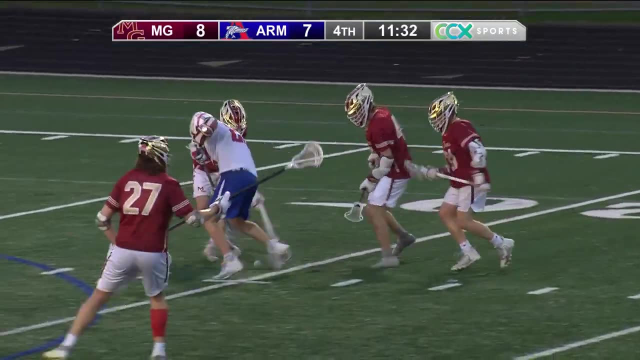 Fourth quarter starting the same way. the third quarter ended Robbinsdale-Armstrong content just to run around with it and kill off some time. That penalty's got to be over any second now. Still have Riley Hansen down in the box as a ground ball battled for in Armstrong's box. 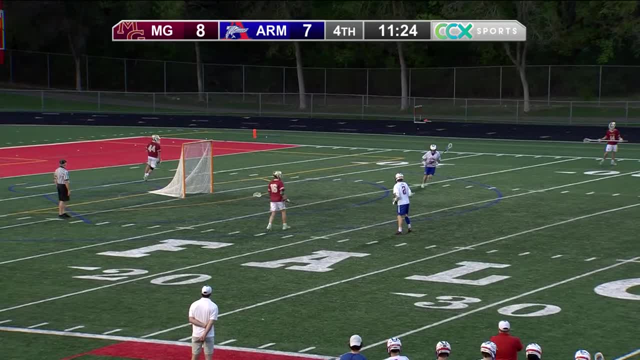 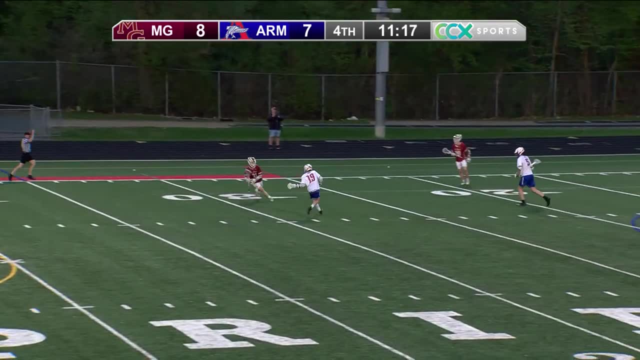 And it's won by the Crimson And they'll go back through their goaltender Farniak. Oh, Penalty has to be releasing soon. It feels like it's been at least a minute. Yep, There we go, Crimson with a chance here. 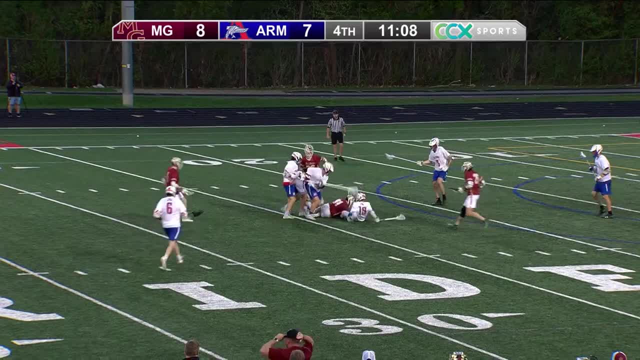 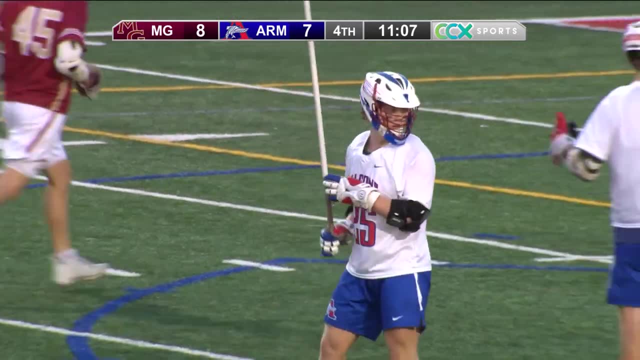 Tried to thread the needle but knocked down by Jack Neff. Now, every ground ball is critical in this kind of a game. Well, Maple Grove keeps trying to penetrate that middle. get it set up in front of the box And boy I tell you, Armstrong's done a great job of denying it. 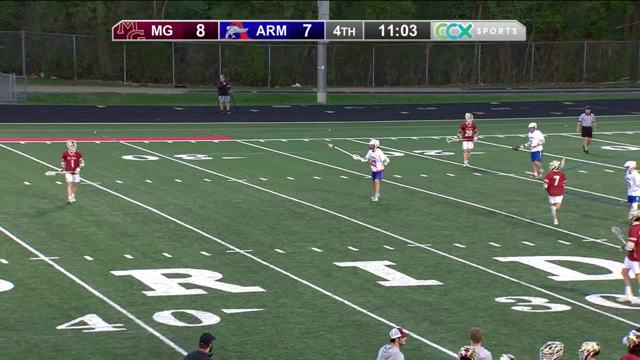 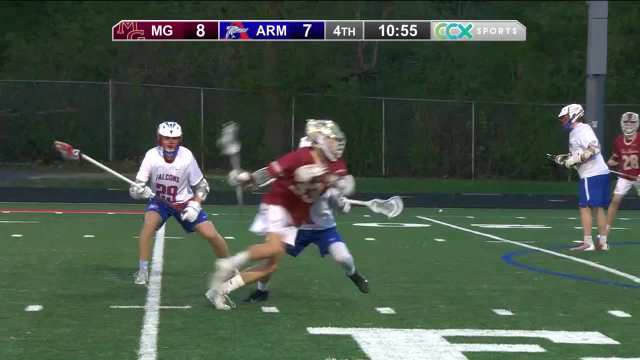 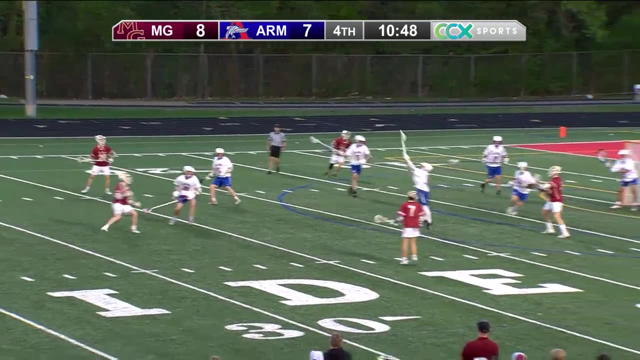 I mean They got a defender on the person right now. Steinkopf, who had a goal in that third quarter, gets it to Brendan, who had two Tanner Brendan spinning off the short stick. check for Peterson behind the net, Back out top Steinkopf. 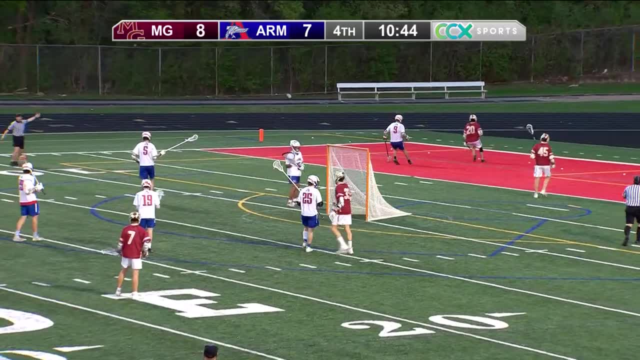 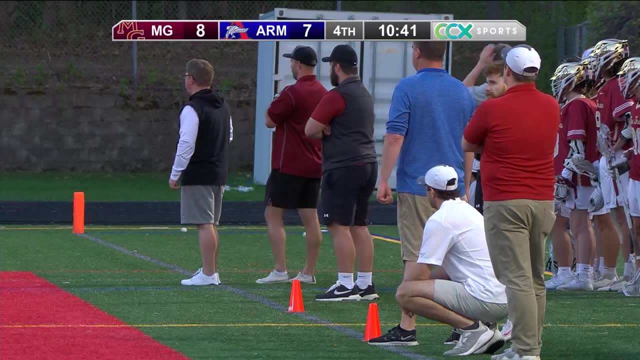 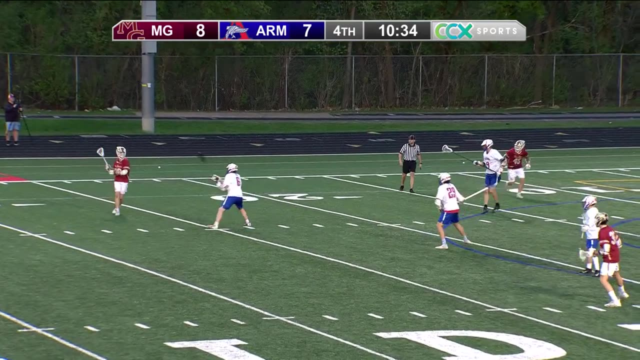 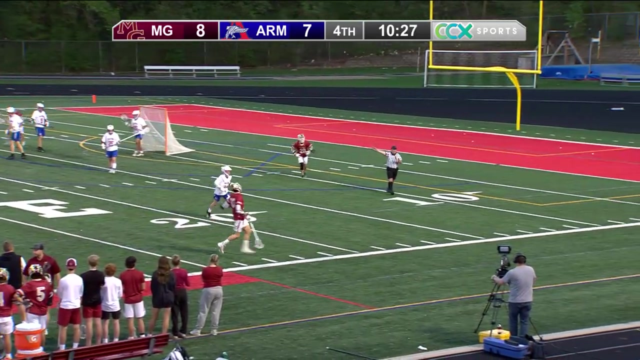 Got catch by Brendan and then he missed the net. Peterson hustling after it, He'll get there first. Bockey has got a hat trick tonight, Hounded by Pappas. A rare unforced error by Maple Grove. Both teams have popped it around pretty good. 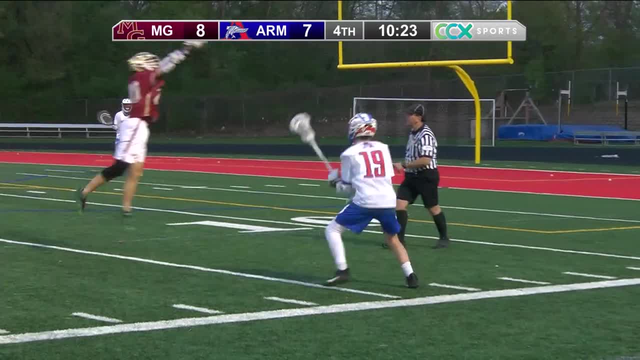 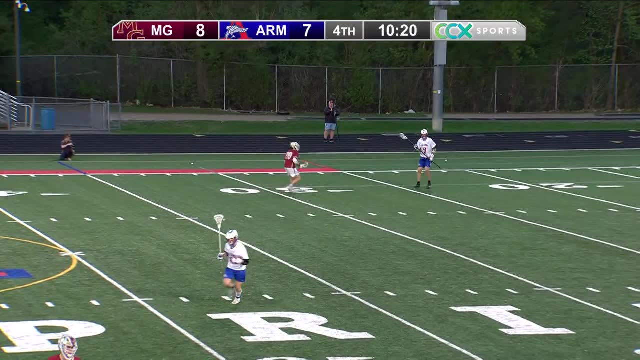 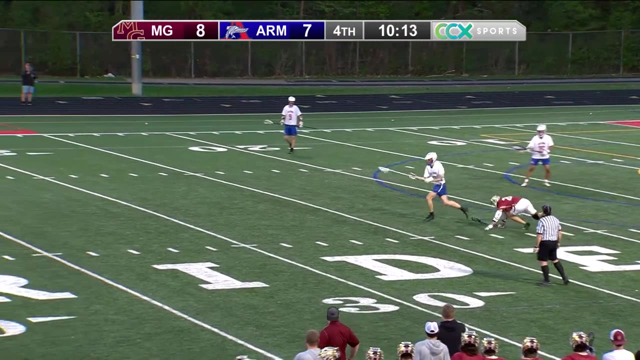 Yep And taken care of the rock tonight. But that errant pass turns it back over. And now Wells will track that one down and then lead the clearance. Pappas, Oh, a dangerous pass just over the stick of Peterson. They got some rangy defensemen to do Armstrong. 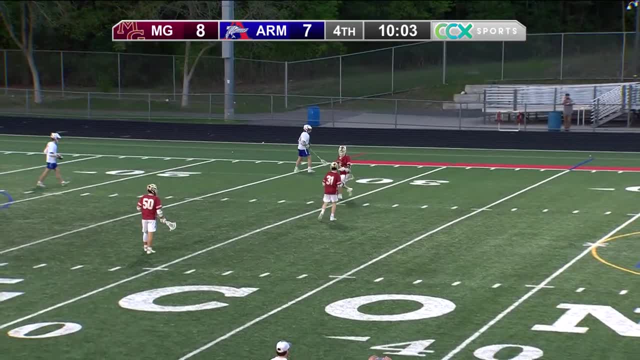 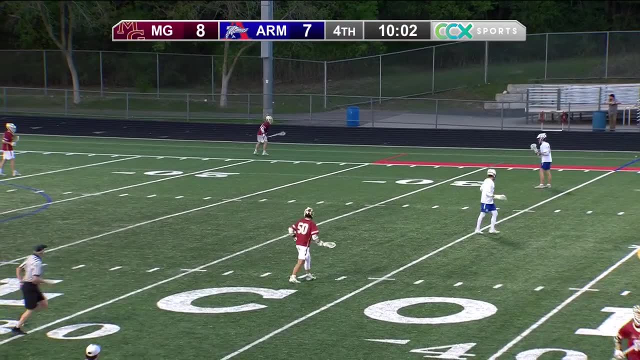 Ten seconds. That's got to be ten seconds and it is- Or maybe offside. Regardless, it's Crimson Ball. with ten minutes to go here in the fourth quarter, Still an 8-7 lead for the Crimson. Look at the D here. 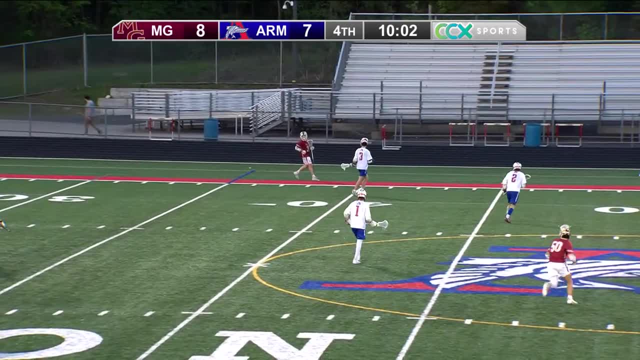 Now they're six-footers, plus, he had a six-foot stick to him. Boy, that's a big wingspan. Thank you very much. Yeah, they're at least six-footers and rangy. Yeah, Feed those guys some chili. 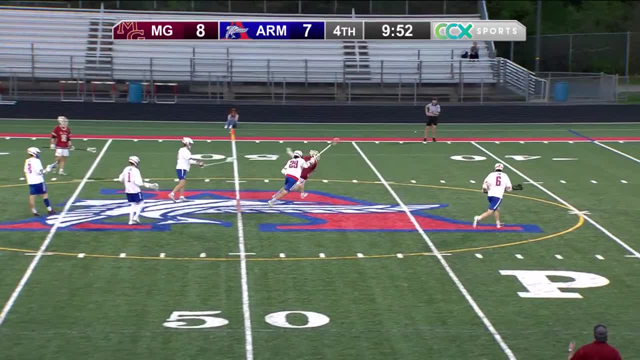 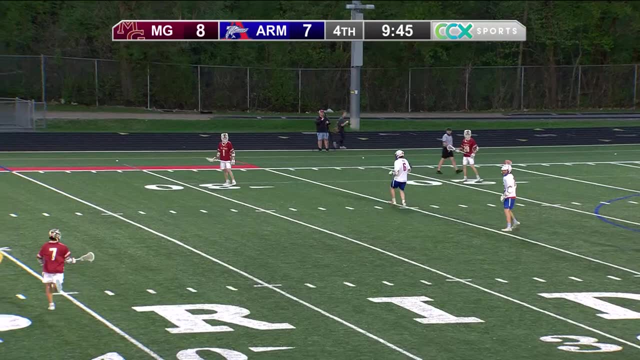 Steinkopf comes up to help out on the clearance. It can be so valuable to have a speedy, confident stick handler like Steinkopf And, as well as Connor Kasbaum, Seen him do that job tonight as well- Scanlon, no one stepping to him. 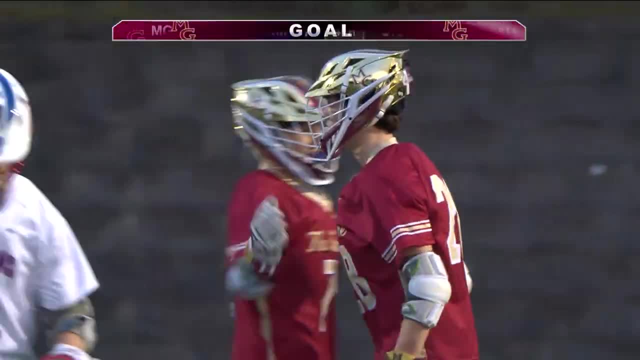 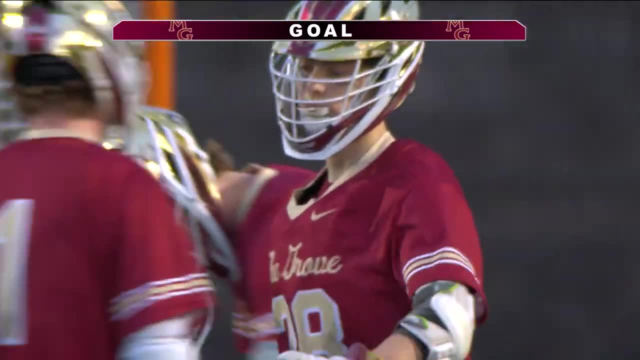 He'll get to the net Score. Score Rory Scanlon For the second time tonight. no one stepped to him, So he took advantage and found the back of the net Boy that was. you know. they've had him bottled up pretty good. 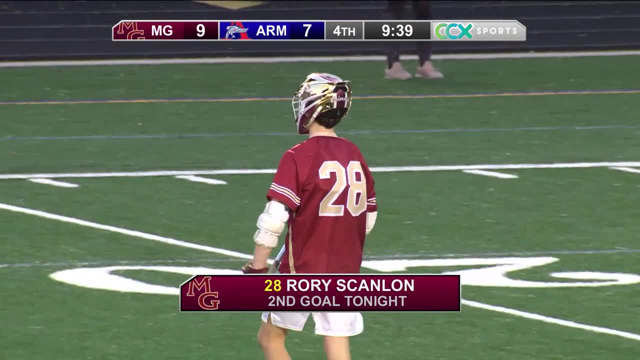 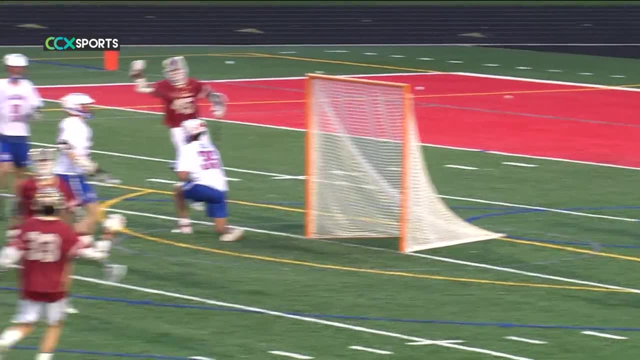 especially during the second quarter there in the first half, And he got away and came back through the middle And boy, don't let him get in the middle there. See the move right here, Covers it and just rips it quick. 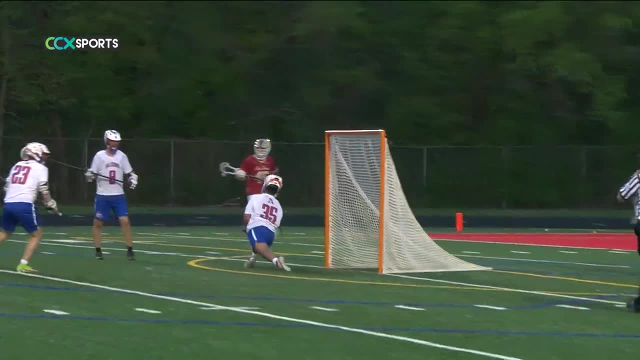 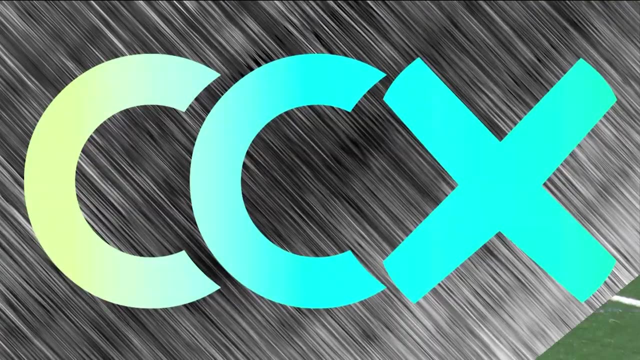 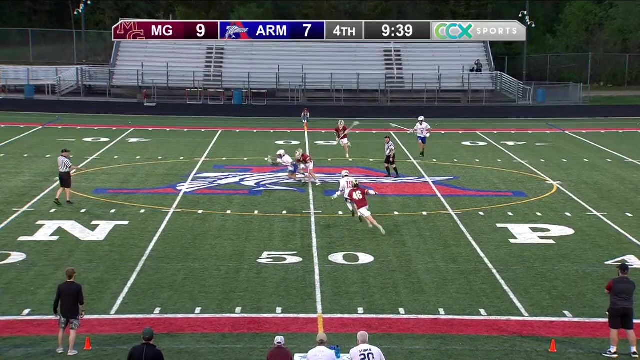 Nice goal, High-low bouncer into the short side of the net. Win here Would certainly put Maple Grove in the driver's seat. There's still some games left to play, But this would be a big step toward that conference title. And, like you said before the game, Kyle wants banners. 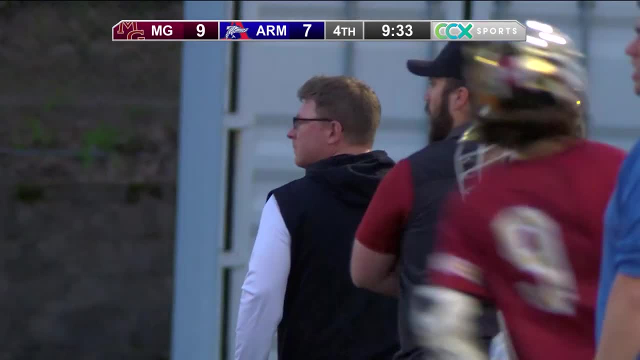 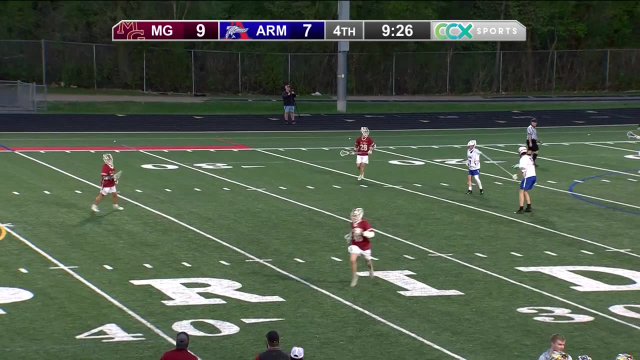 Yes, he does. He'll take conference banners, He'll take state titles, But you've got to win conference first and put yourself in position. Of course, the Crimson falling short in the section title game to Benilde St Margaret's last year 9-3.. 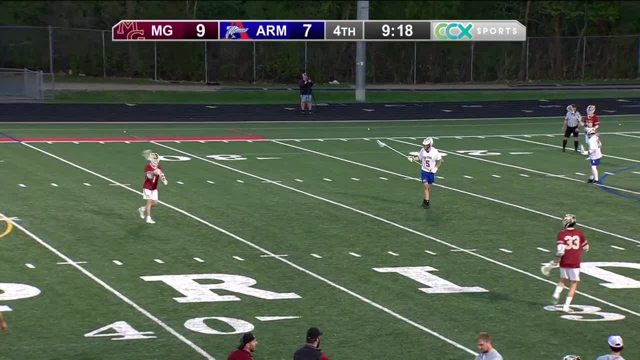 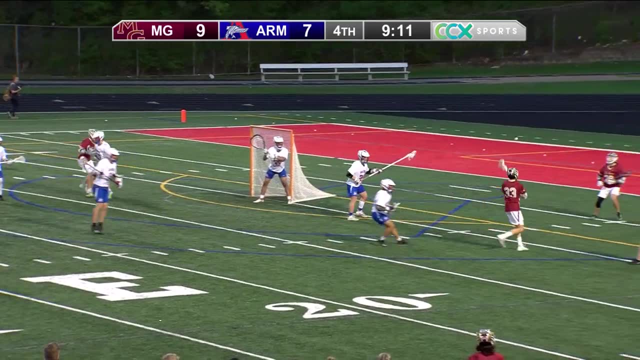 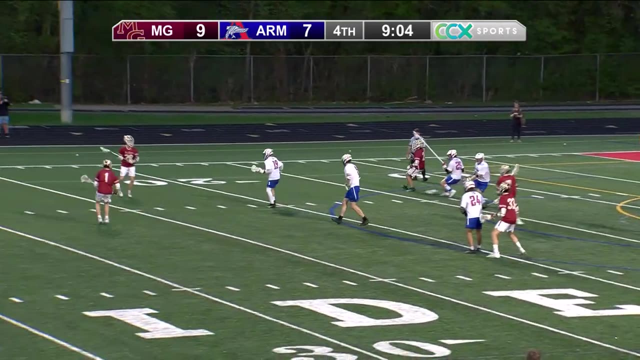 No shame in that. Benilde ended up winning state in overtime over Prior Lake. Brandon attacking downhill, A spin back, but well covered by the short stick. Peterson Using that quick step at X Back for Scanlon. Steinkopf feeds down low and they score again. 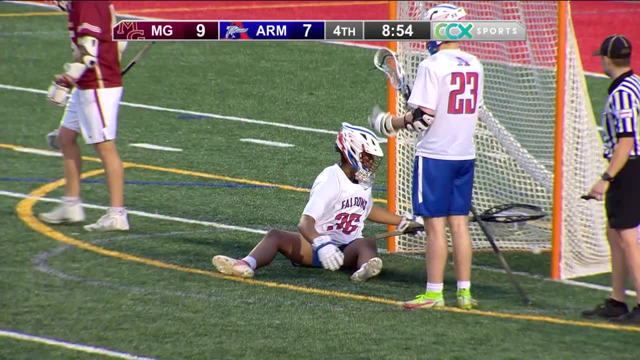 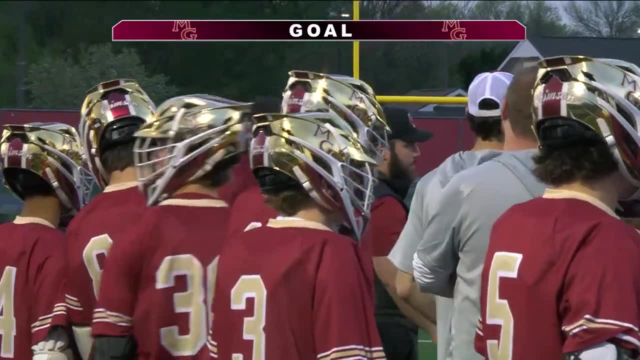 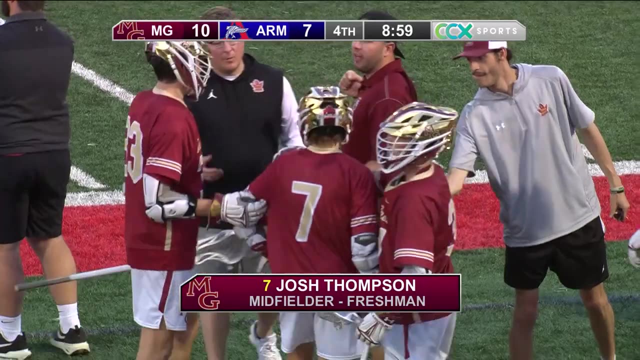 A well-placed bounce shot for Josh Thompson, Number seven, with his seventh goal of the season. Well, the Crimson are doing a great job getting it up top of them, bringing it down into the square area in front of the net. That was a little bit to the right or to the left of the net, but still got him in a beautiful position. 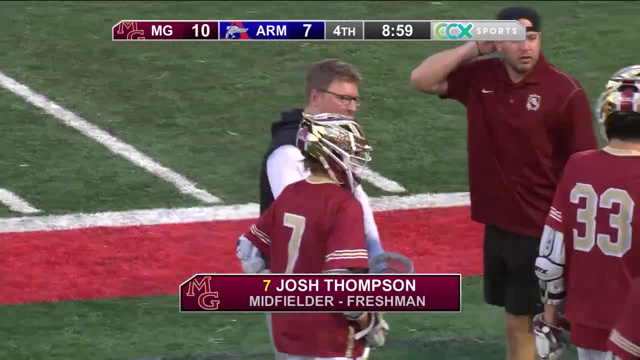 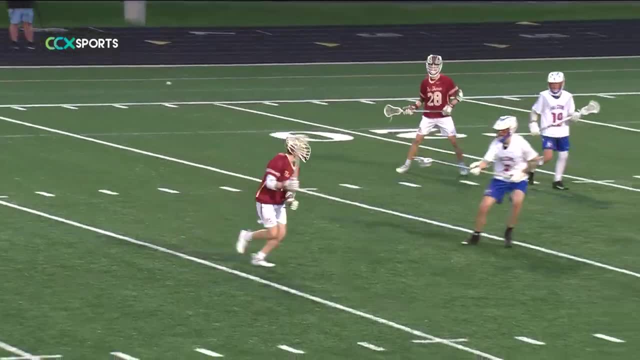 And that's a halftime adjustment, I think, because Steinkopf has three second-half assists from that top position feeding in the middle, And that's a freshman that just scored that. You see Steinkopf right here feeding in the middle, turning and shooting Dan Ficken. I'd say 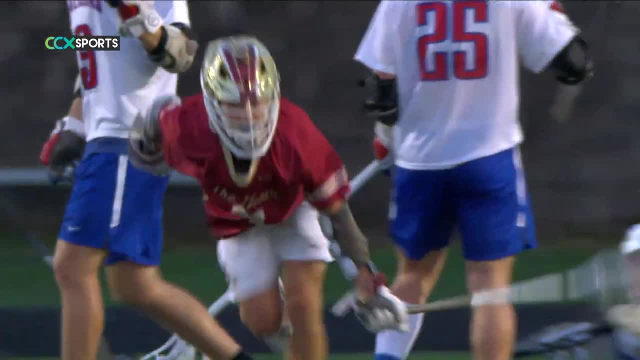 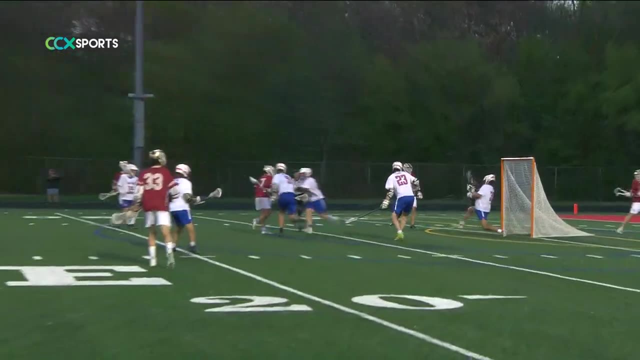 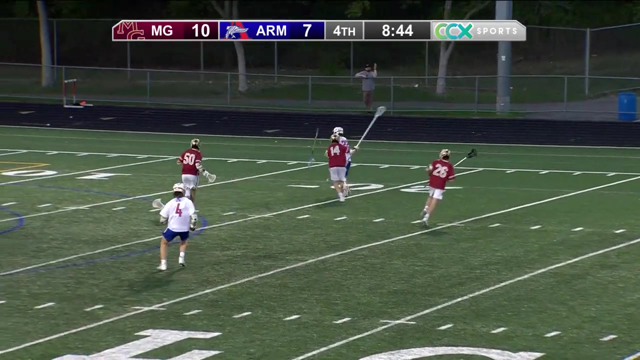 Whoever caught that, Kyle Ficken's father, must be a smart puppy, because they made some halftime adjustments and the freshman showing out Josh Thompson's seventh goal of his freshman campaign. That was a nice one Goal, coming in at 8.56.. 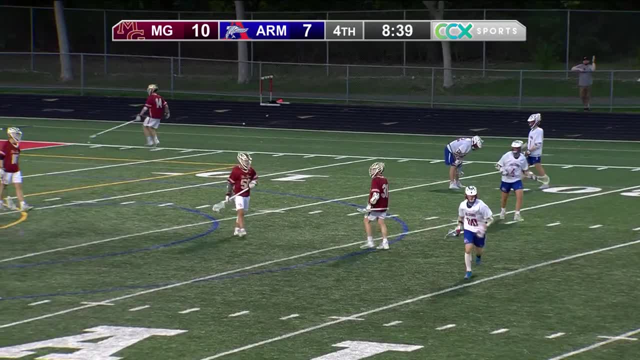 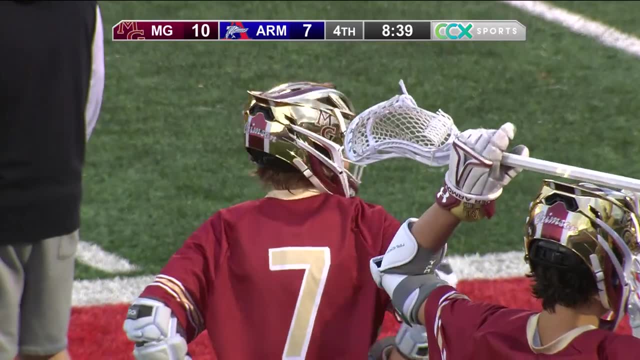 10-7. now Maple Grove, And once again they've rattled off and really they've scored five of the last six goals to have a three-goal And that's a three-goal lead, or well, that can't be right. 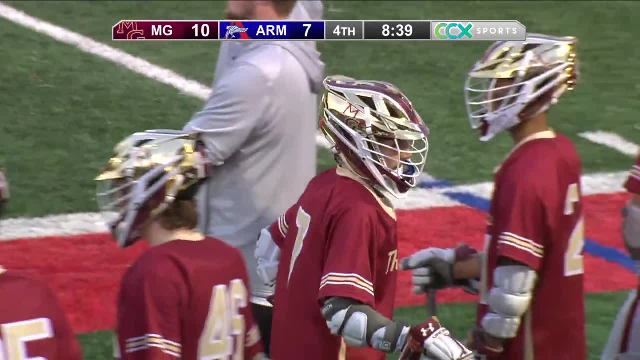 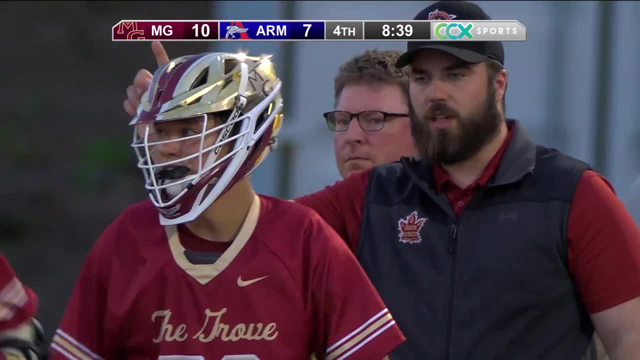 They've scored four of the last six goals, but back to a three-goal lead is the point. But how about Josh Thompson? And how about the freshman we've seen tonight: Olsen, Olsen's tall Olsen with a goal. Olsen's a player. 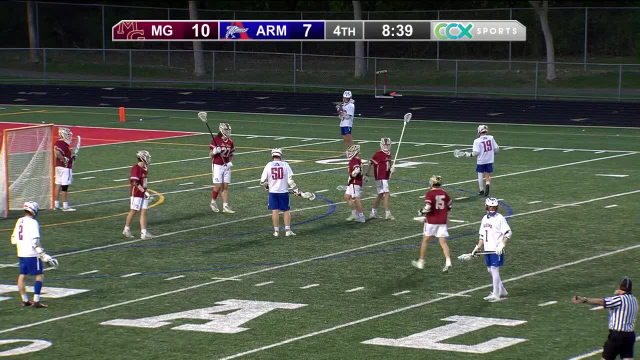 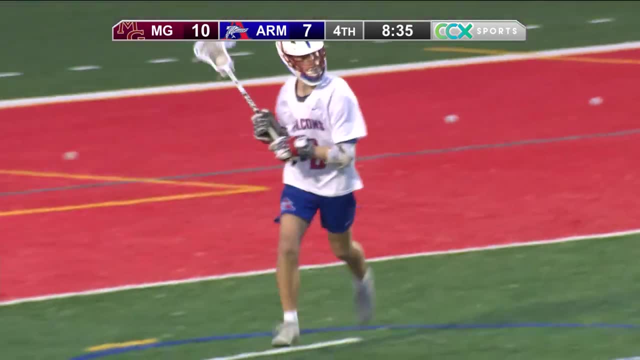 I'll tell you it's fun to watch these young freshmen coming in And you see the benefits now of the youth lacrosse programs that are starting to take hold here. They're starting to produce some players and the quality of the game's going way up. 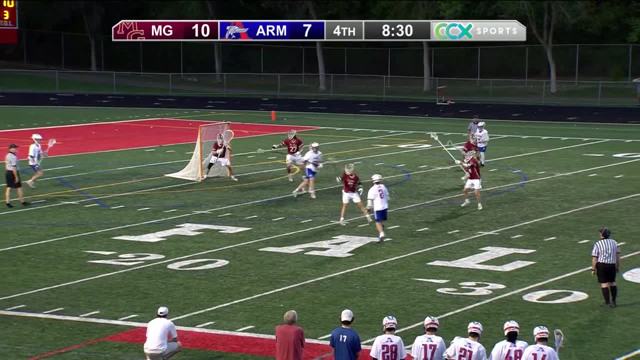 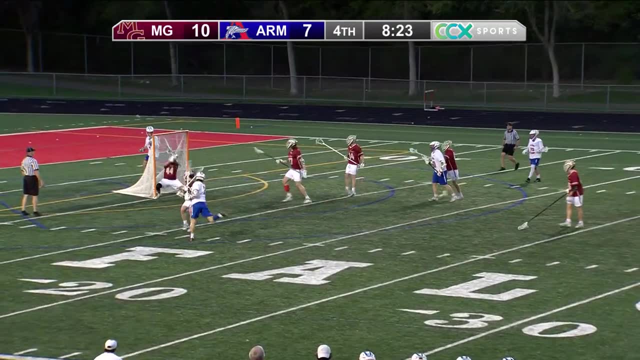 Corey Scanlon will take a knee as Maple Grove goes on the EMO. By my count, each team with five penalties apiece. tonight, Manis, There's a shot- Oh, that had some steam to it- from Nate Albrecht. 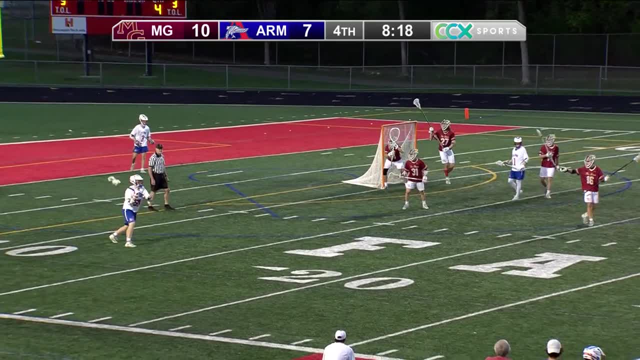 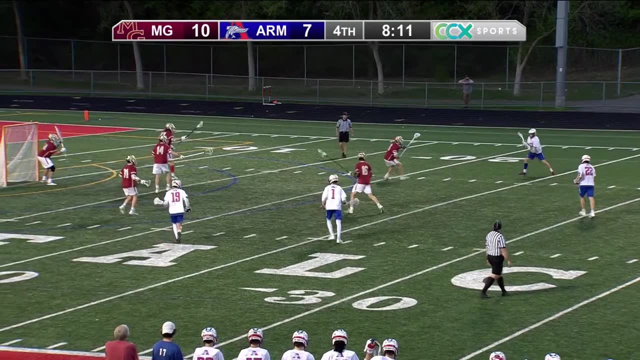 Mr Aldo showing off his cannon there. My gosh, that was a heck of a shot. Got a step to him faster. A little fake play, for Essin Does seem to be very right-handed, but it's worked well so far. 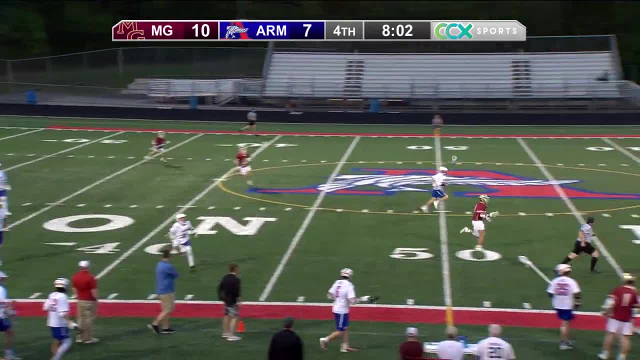 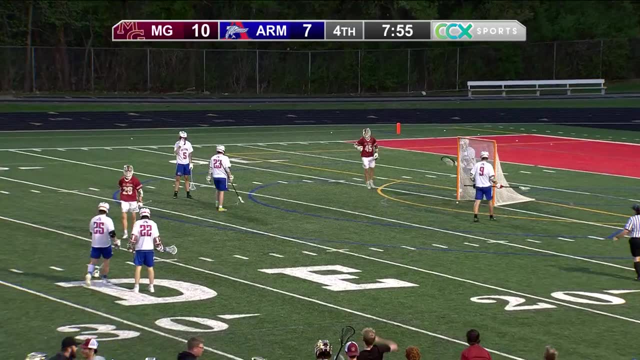 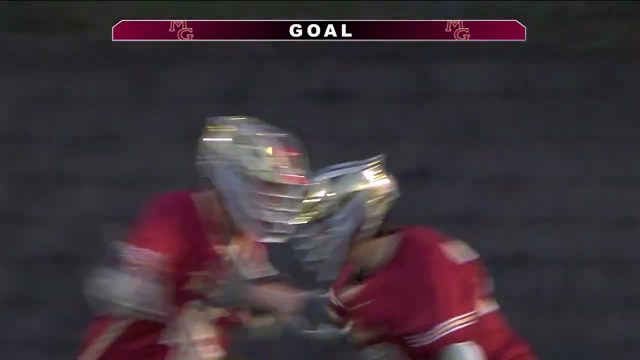 But Farniak makes a tremendous save And now outlets it quickly to big Briggs Leisner Transition. as Scanlon steps into one, It scores A hat trick for Rory Scanlon. They score shorthanded. It's four straight for Maple Grove. 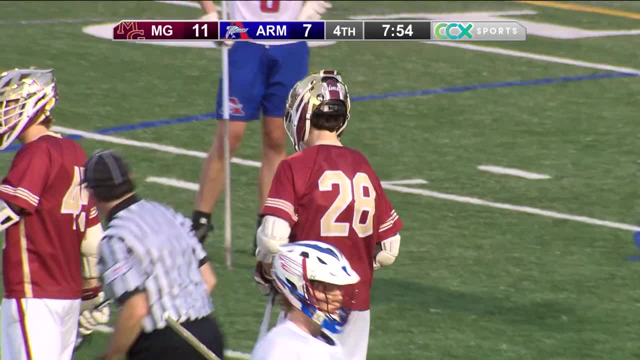 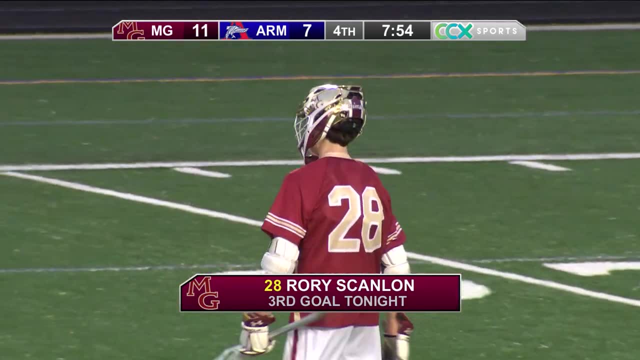 Well, as they say that dude be feeling it man, Wow, he didn't even hesitate, He's got it And he put it in the same exact spot. He's got that short side corner up top Just dialed in and just ripped it. 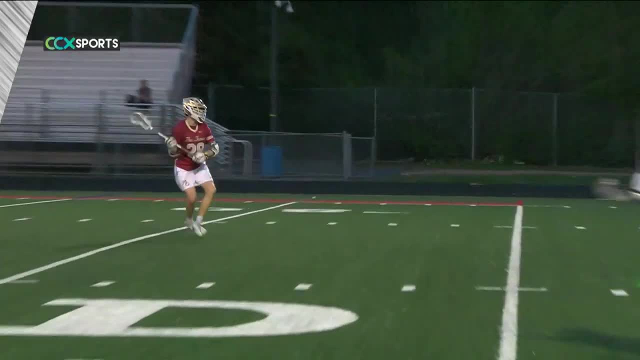 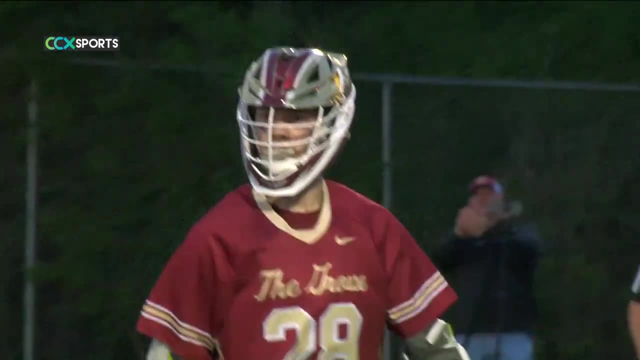 His second of the quarter, his third tonight. It's 11-7 Crimson. You didn't see that one until you saw the bulge in the back of the net. You can see the goalie now for Armstrong. Xavier Wall's kind of like okay. 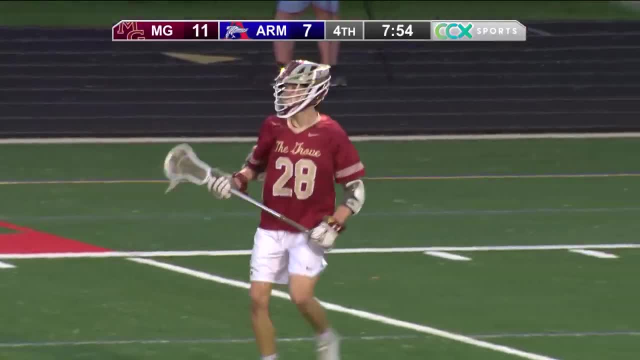 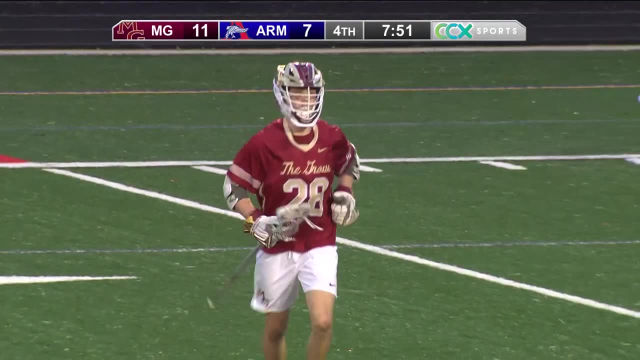 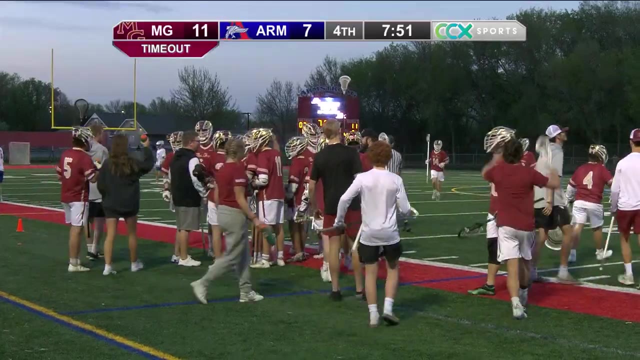 I got to think this one through as he stood behind the back of the net and kind of getting his Nerves calmed down a little bit. Timeout called by the Crimson to retain possession. Rory Scanlon, the Springfield-bound attackman, senior with his 27th goal. 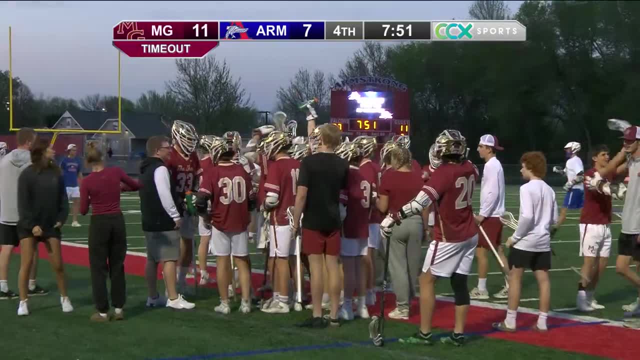 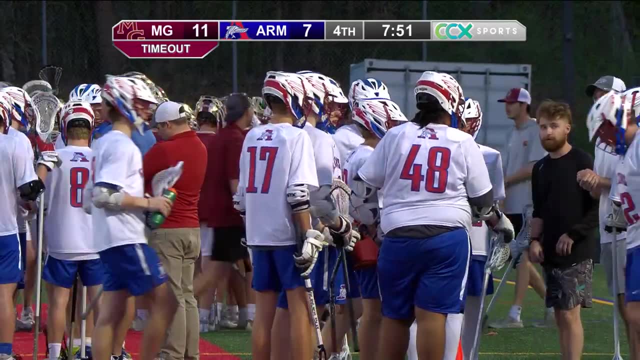 And he's really been the star of the show tonight because remember he had a goal in three first-half assists And now he's got two goals. so he's got three goals and three assists tonight. Scanlon does And he is really leading the line. 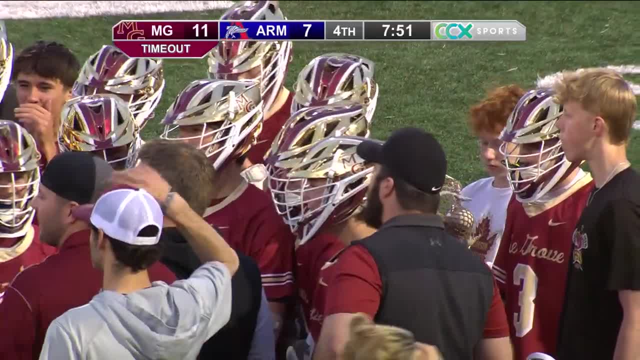 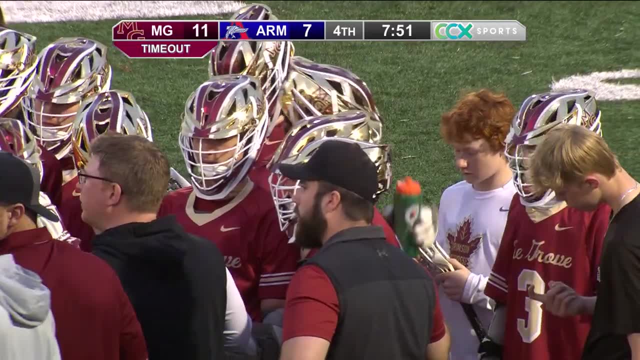 And for this Maple Grove offense, He's showing that he's the star that stirs the drink for the Crimson. right now He's got it all. The best thing he's doing, too, is he's got his head up and he sees. 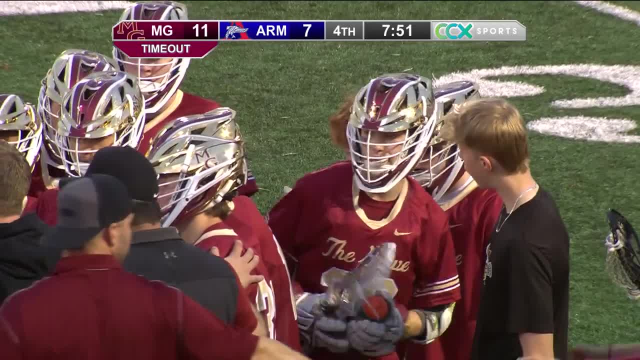 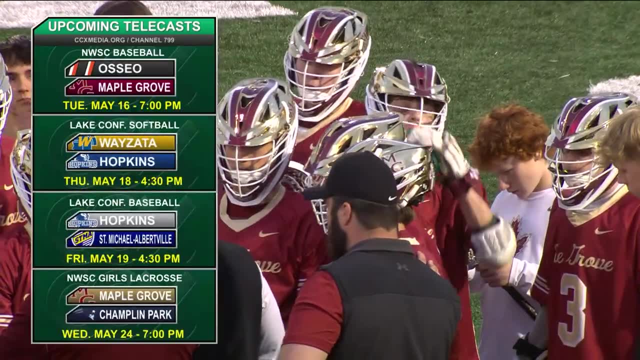 He sees where people are. That was a no-look pass on that last goal, but he knew exactly where his buddy was. Let's take a look at our upcoming broadcast here on CCX Sports. We have a couple baseball games for you and a girls lacrosse game. 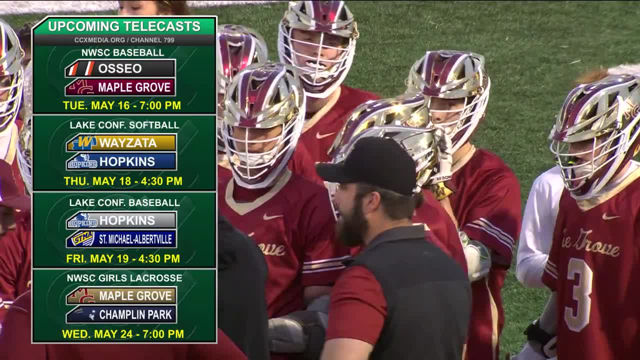 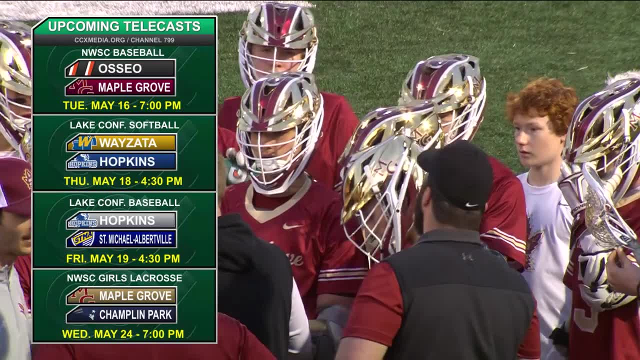 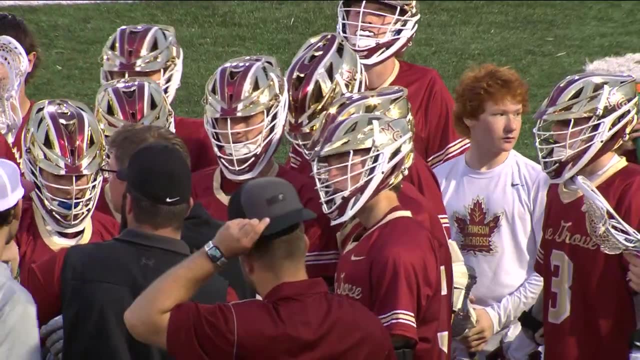 The Crimson girls lacrosse team will visit the Rebels of Champaign. They're going to be playing at the Brooklyn Park on Wednesday, May 24th. All those upcoming telecasts on Channel 799 CCX: Maple Grove boys trying to pick up their eighth win of the season. 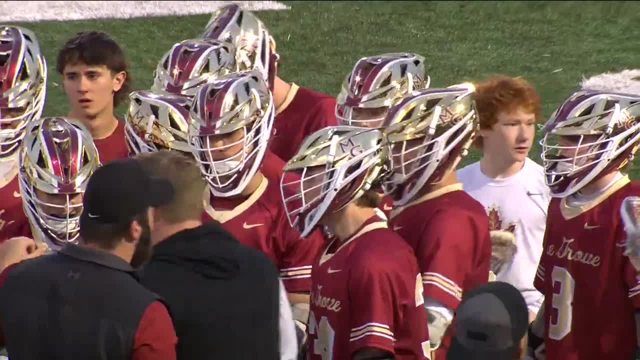 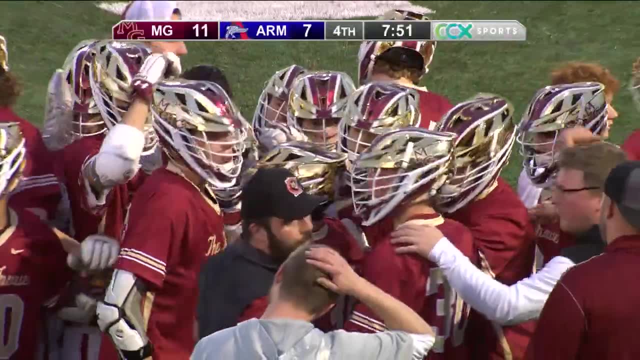 their eighth win in conference play, And certainly it's been, I think, undoubtedly a huge success for Kyle and his coaching staff here in their first season of charge. They're happy. They knew what they kind of had, though, when he walked in the door. 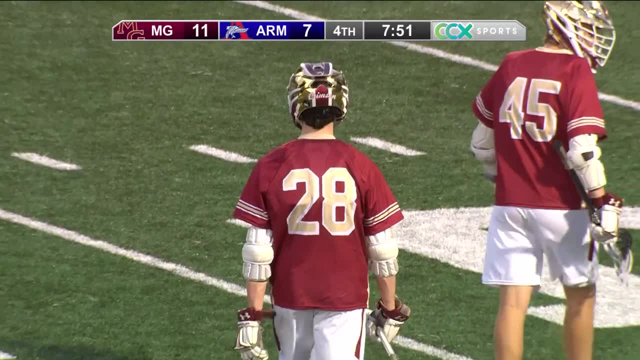 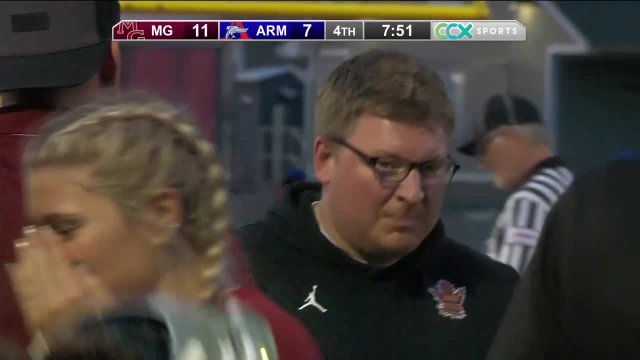 There's been some players on this team and he's real happy. He's just ecstatic to get the job here at Maple Grove and he loves it And you know I hope he does well. Yes, and I am biased. 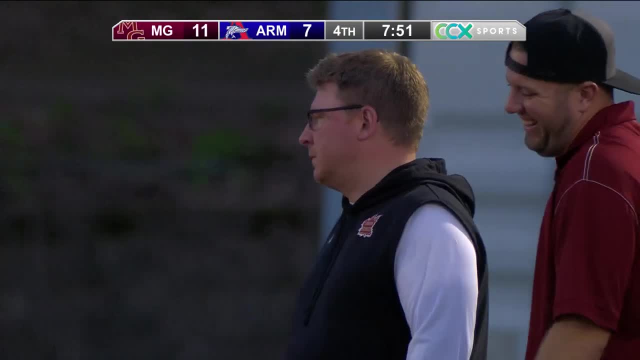 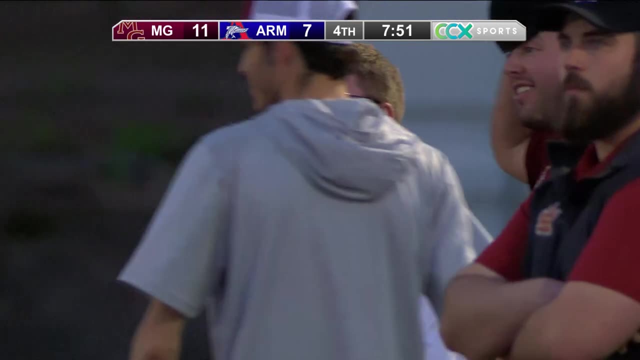 Sorry, folks Deal with it. Well, it is your son, so 7.51 to go in the game, 11 for the score. Crimson have rattled off all three goals here in this fourth quarter and taken what was an 8-7 game and made it 11-7. 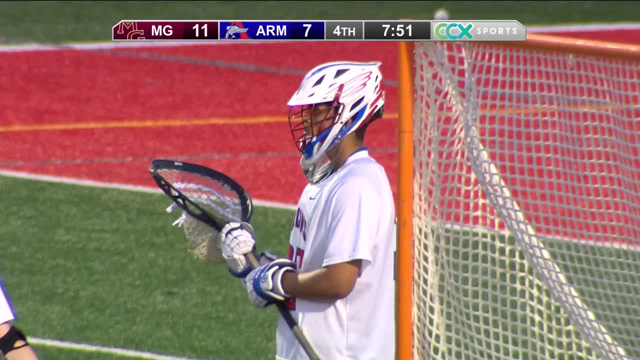 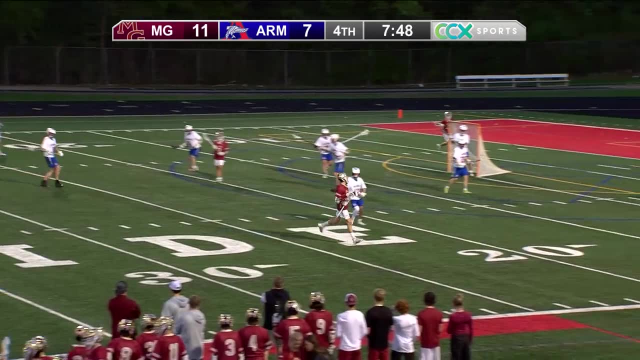 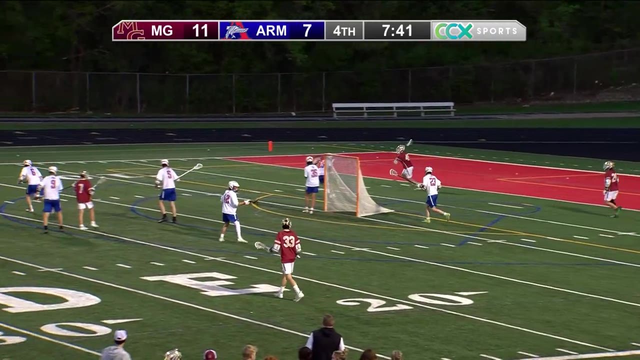 And Xavier Wells tries to stem the tide here, but Maple Grove goes to work offensively off the faceoff win. Throughout the season, Maple Grove- the fourth quarter's been their best. They've totaled 36 goals so far in the fourth quarter, not including tonight. 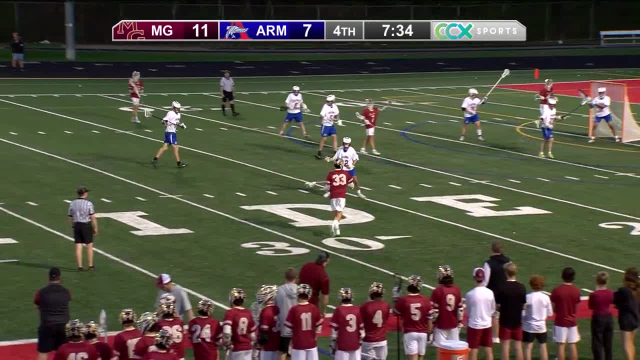 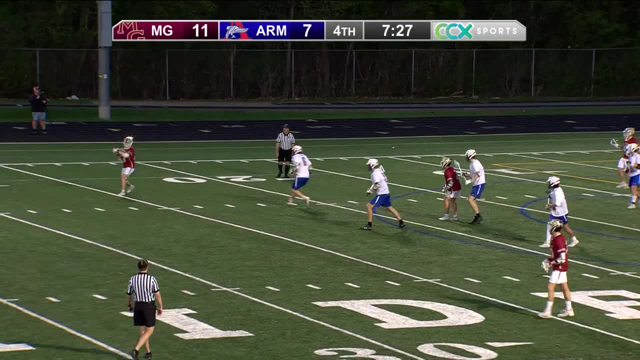 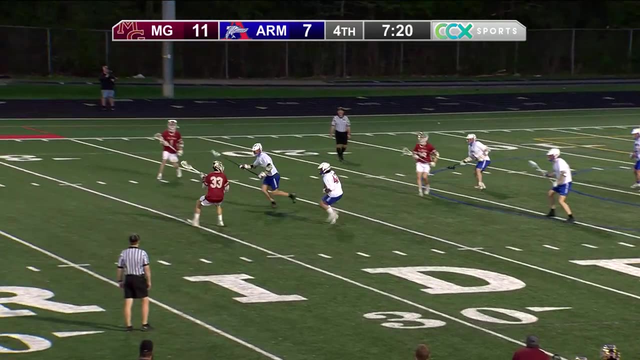 And their opponents have only scored 29 times on them. so they've got a plus-7 differential there, 39 plus 10, Matt, We've added three here in the fourth quarter. They're content to just pop that rock around as Brendan dodges down the alley. 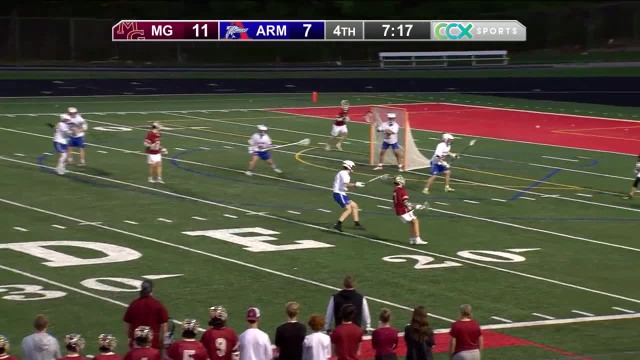 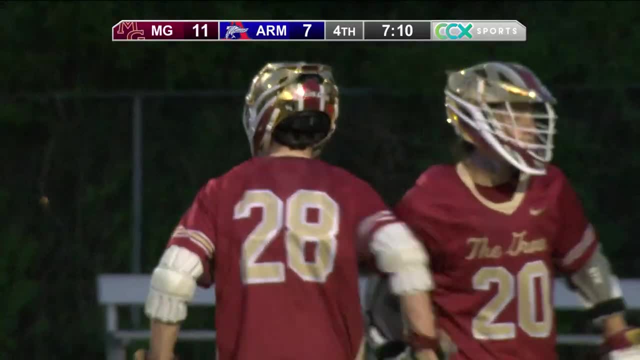 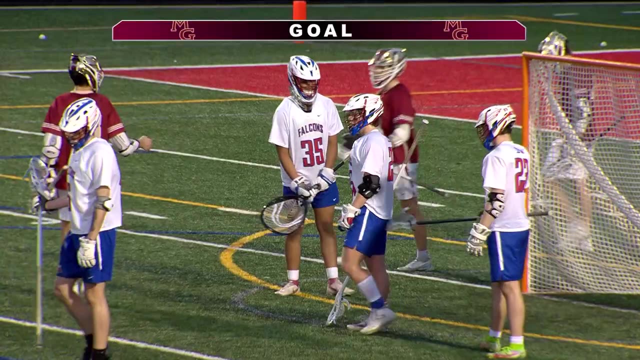 and then moves middle Low pass, dug out by Thompson. Just the poise of the freshman, Beautiful tic-tac-toe passing. It's Peterson to Scanlon for his third of the quarter. Can I say wow, Yeah, Holy buckets. 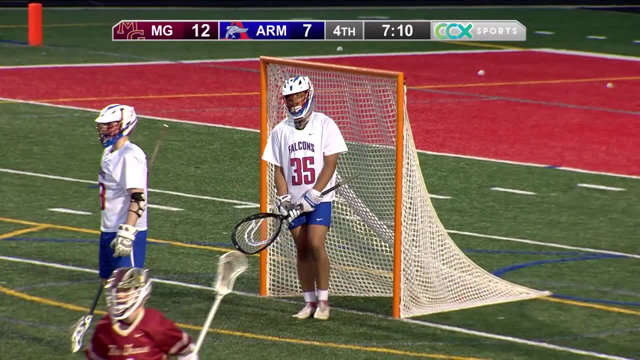 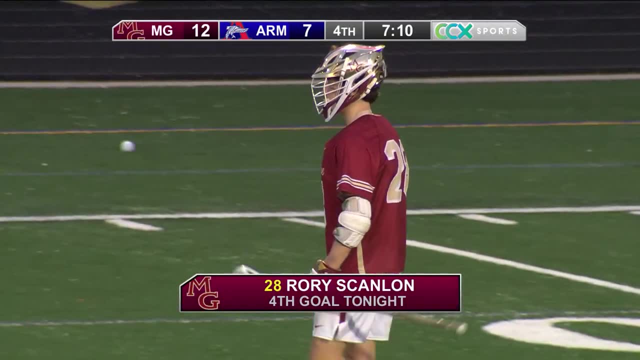 I'll say wow too. Wow, You got a feel for the goalie there. He didn't have a chance on that man Scanlon. they fed him up and boy, he don't miss. He does not miss. Great cut. 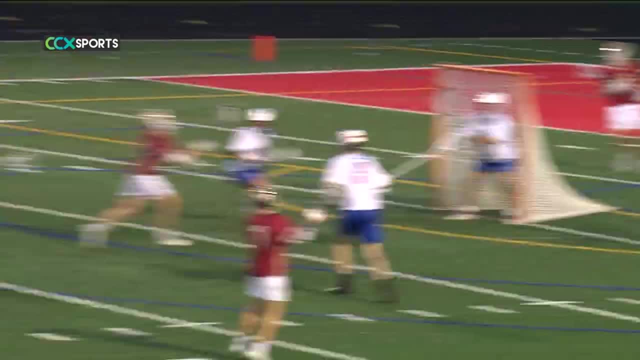 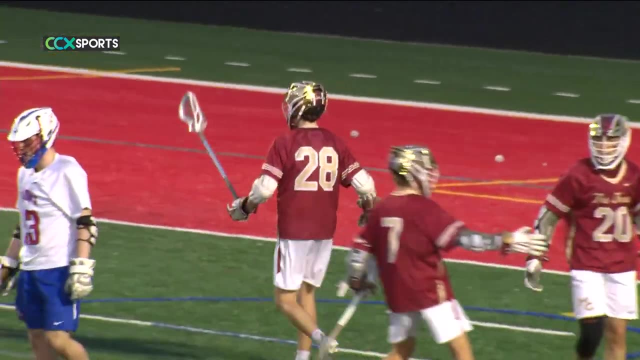 Scanlon now with four goals and three assists tonight. A seven-point game, 12-7 the score now. Well, the feed from Ricky Peterson was unbelievable. He knew right where he was. The cut was great. the whole thing Came right over the top. 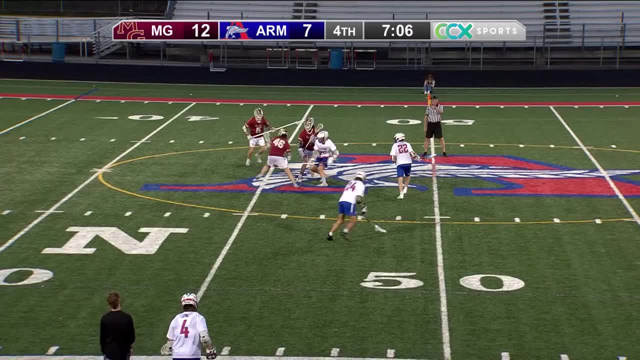 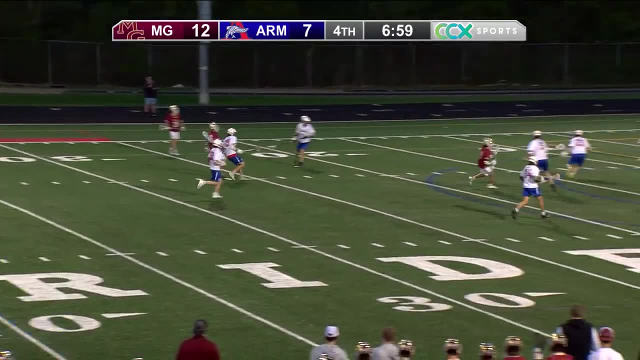 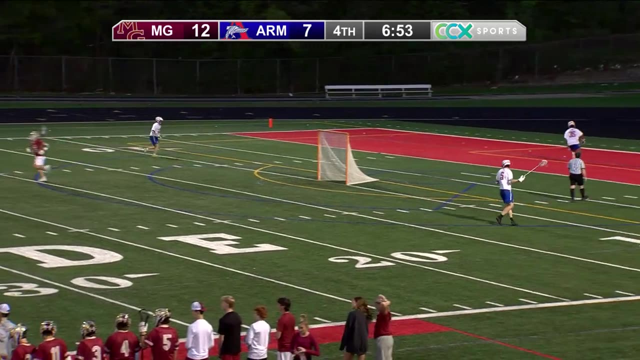 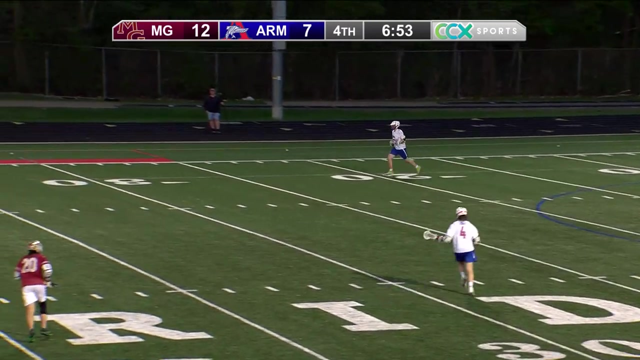 That was a special goal from the Crimson. Now they're starting to even win face-offs. They have scored four in this quarter And what was a one-goal lead is now five Wells will reenter play for the Falcons. Goal, Goal. 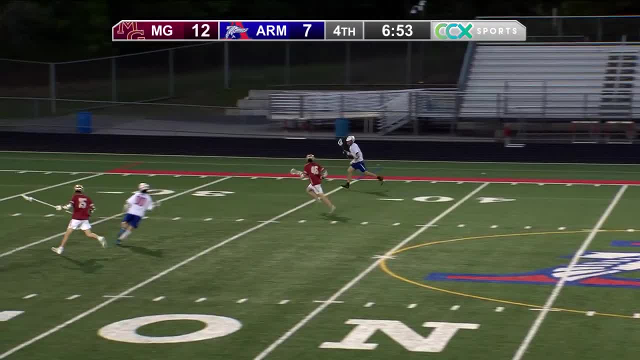 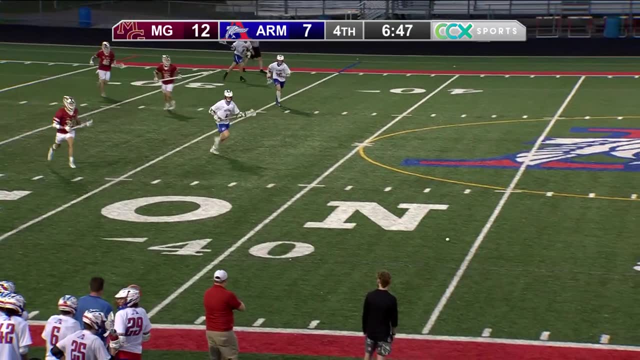 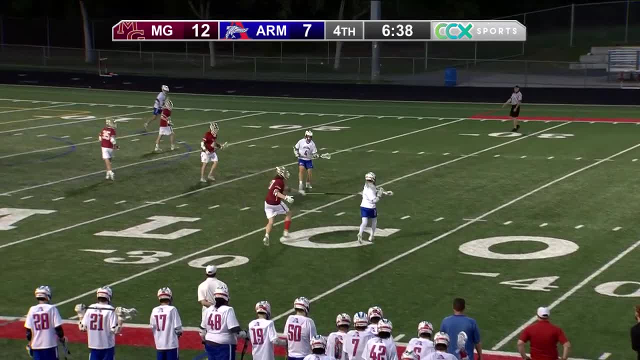 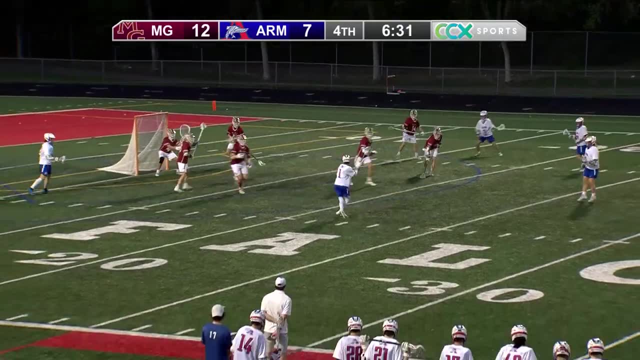 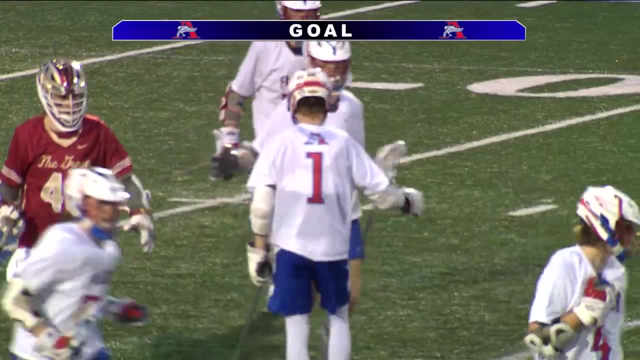 But now they got to make each of these possessions count. now, with about seven minutes left, There's a goal for Robbinsdale Armstrong. It's Annis, He's got a hat trick. Well, when you need a goal, go to your goal scorers. 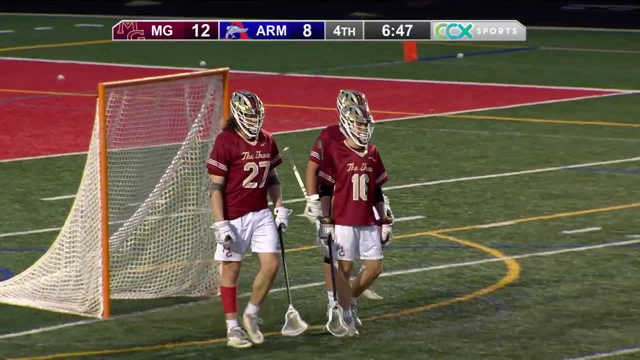 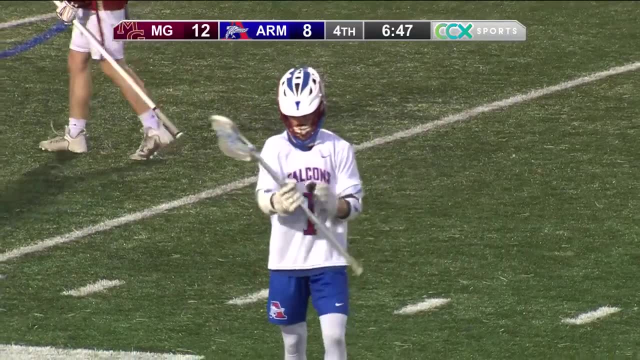 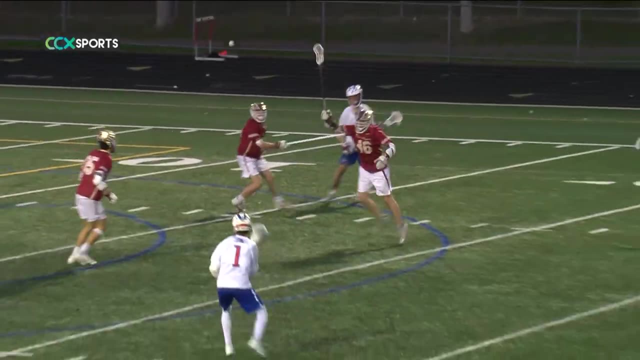 and they got the ball into the hands of Annis and he buried it and put it away: 12-8 the score as Annis finds the back of the net for Armstrong. That ends a four-goal run. Annis, and again he likes that low shot. 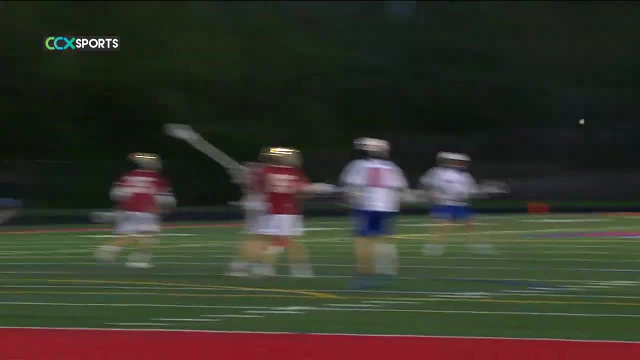 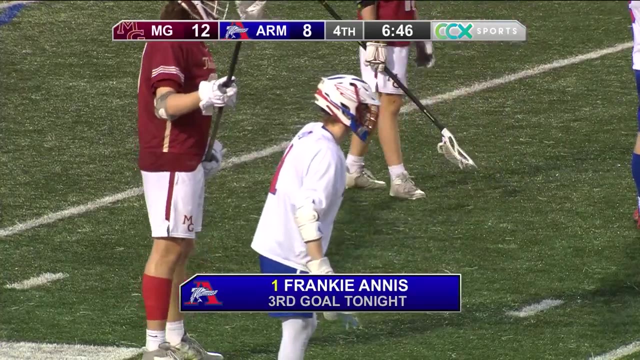 Varniak diving, but couldn't stop it. He's good at it too. You know a lot of the times you see that shot. they follow through too high and it goes over the net consistently and he's not. he's finding that spot every time with it. 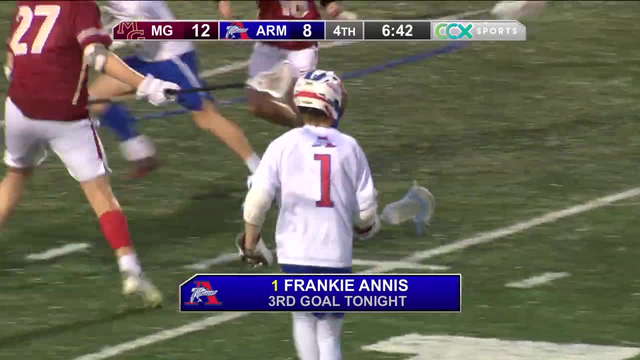 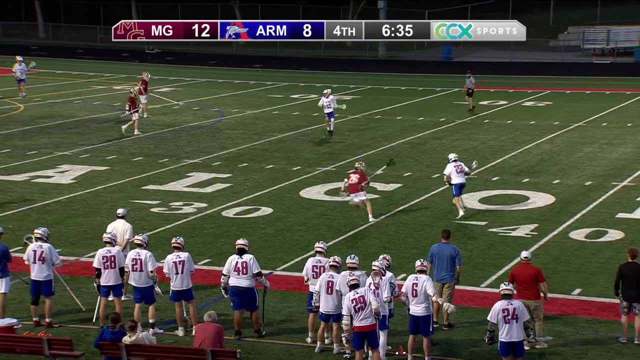 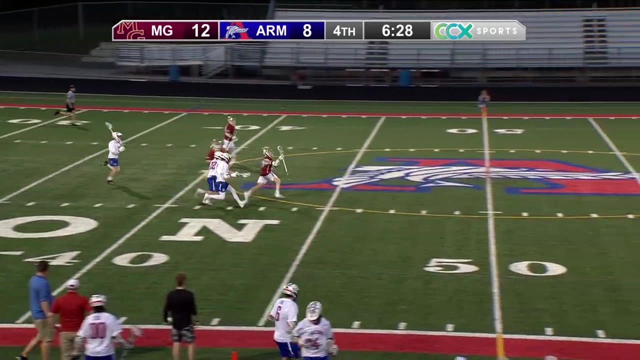 A hat trick for Annis Armstrong wins the draw. This is lacrosse, so still plenty of time left And a four-goal deficit not insurmountable. Essendon stripped from behind. What wonderful defense there. Maple Grove again in transition. 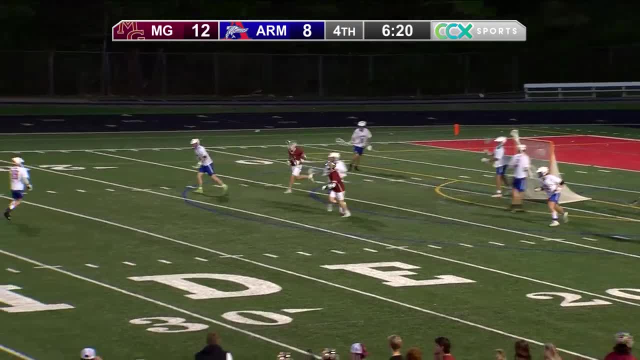 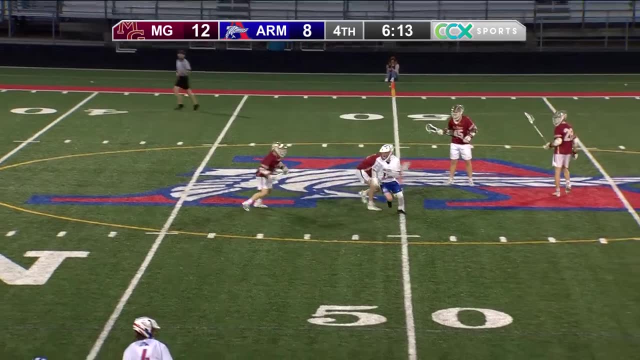 Scanlon Wines, fires and Wells makes the save Pretty safe. Pretty safe, Nice and controlled. Now they know what Scanlon's going to do. if you give him time and space, Nice, move by Northrop to spin free. 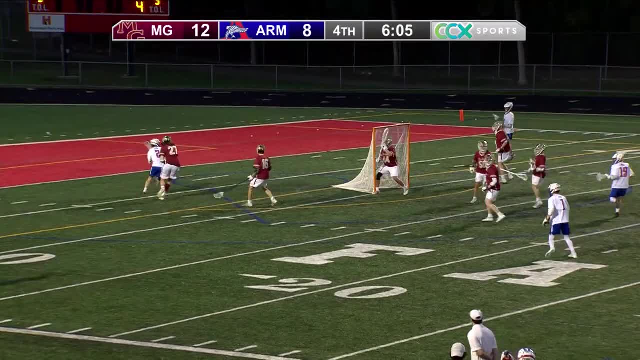 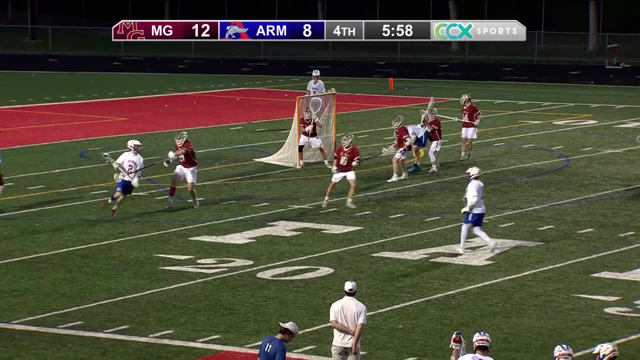 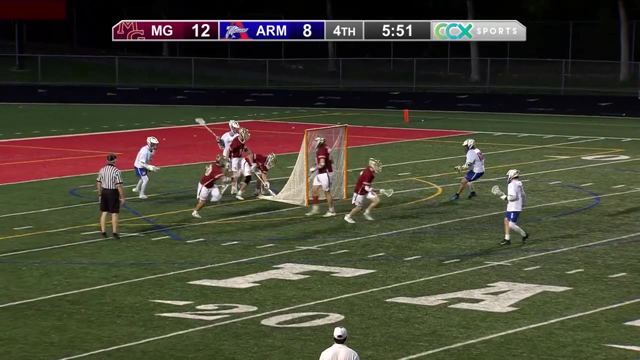 Gets it to Annis Albrechts. He has been held relatively in check tonight, Does have a goal and an assist, but the Maple Grove defense has been aware of him As Annis goes And Farniak makes a great save as he tries to go low and go five-hole on Farniak. 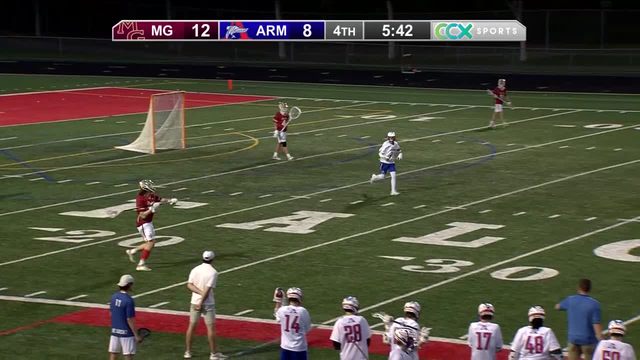 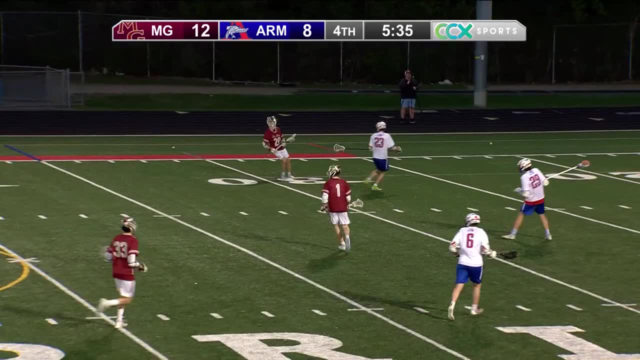 but he makes a tremendous stop. Well, he's good on those low shots because he just drops his body down and uses his body to block the shots and does a great job with it. Yeah, fearless in that respect. 5.36 says Scanlon gets a touch. 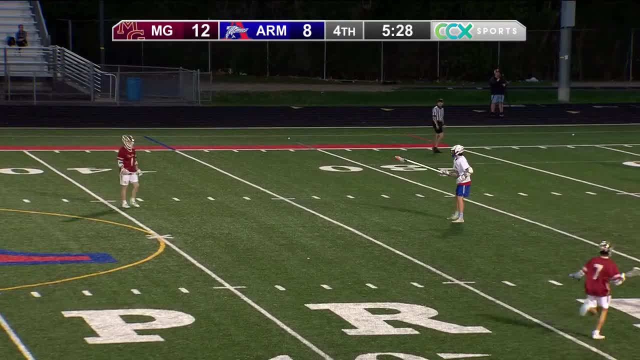 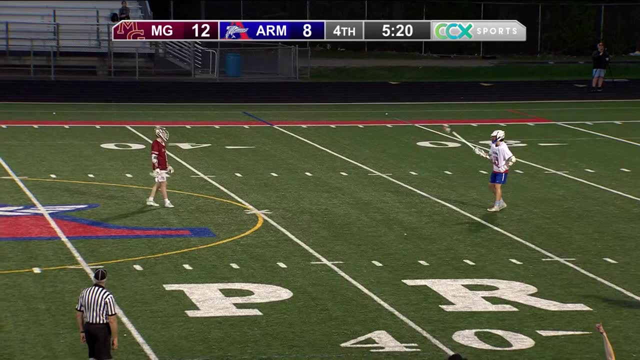 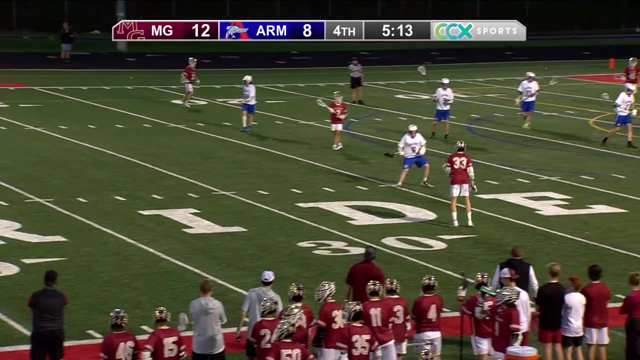 They'll continue to try to pour on the goals, but ultimately I think yeah, it may. if this score holds, or something like it, it's going to be the Crimson defense and Farniak in net. that is the difference, but you knew that once they started scoring. 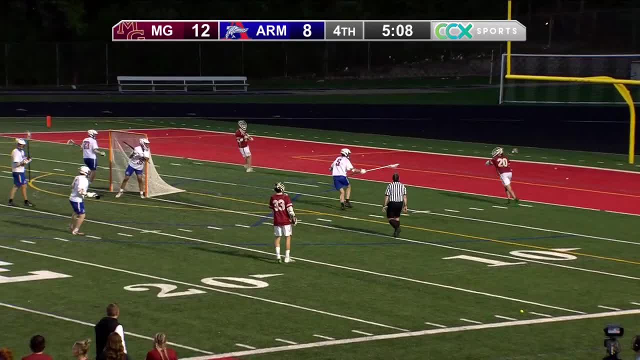 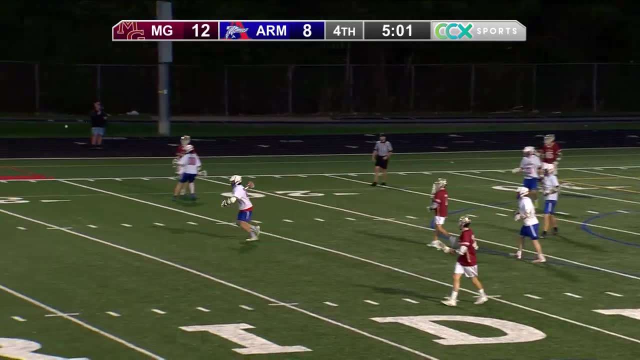 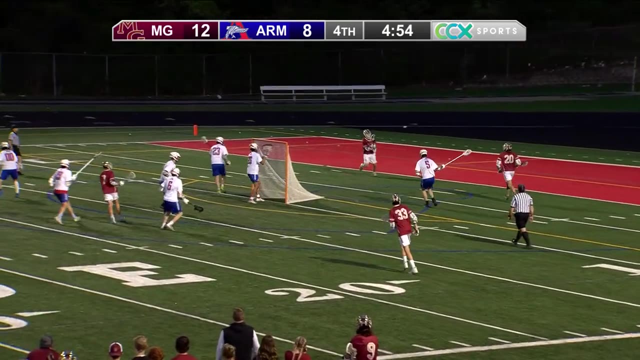 they've just gotten contributions up and down the line, Scanlon leading the way, but hat tricks from Bakke and Brandon as well. Both teams are good offensively. We knew the one that came up with a better defensive play, and Farniak has made the difference here for the Crimson totally. 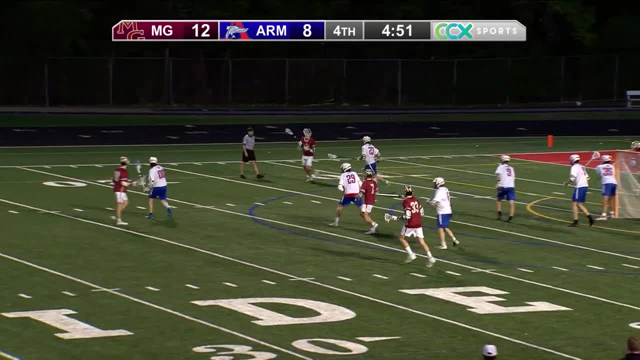 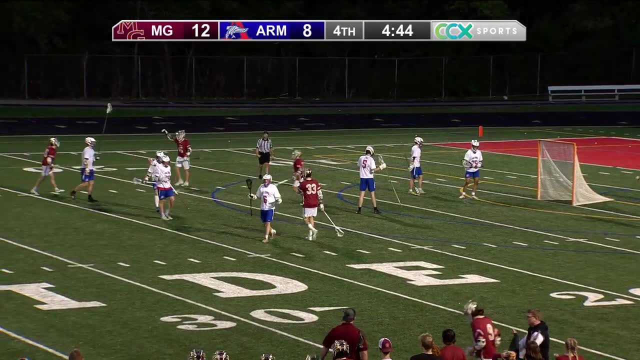 I mean, he's been spectacular. Xavier Wells hasn't been bad either, but Oh, he's been really good. There's a shot on shot and they score. Scanlon cannot stop scoring here in this fourth quarter, His fourth of the quarter. 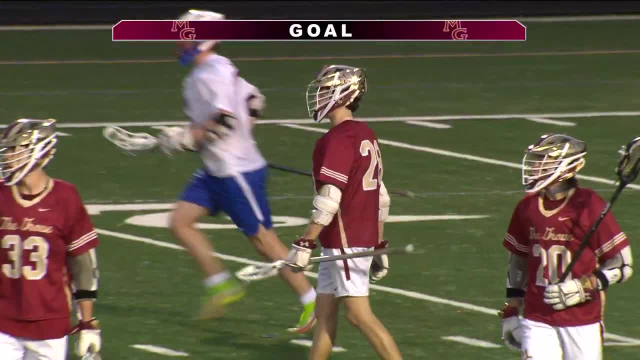 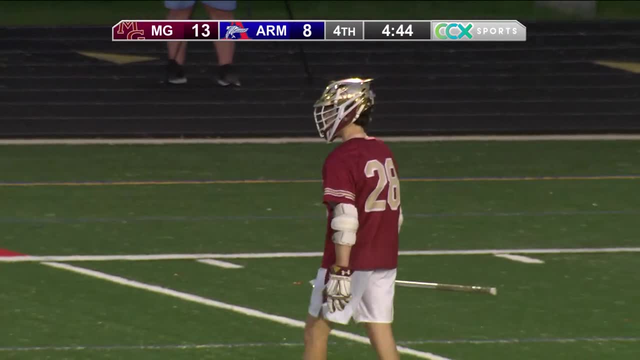 His ninth point of the game. I think he found his spot. It's kind of like a three-point shooter knows where his spot is. He gave it to consistently and he scored for it- Exactly pretty much the same spot he's been on the field. 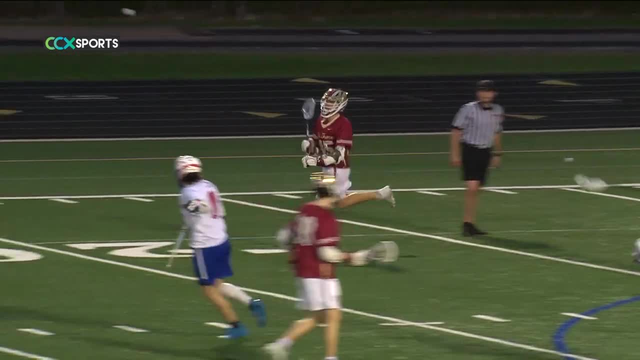 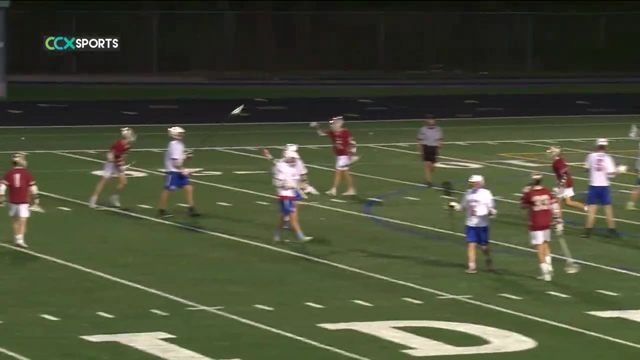 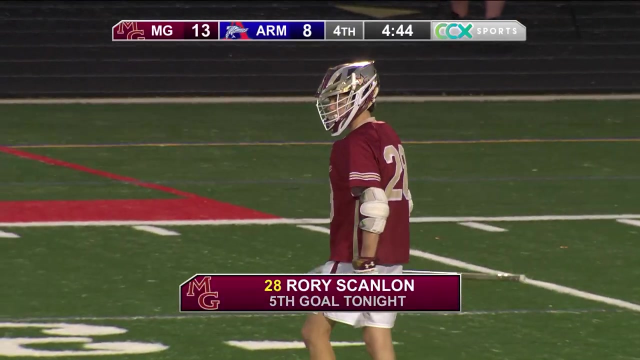 And the Crimson are smart enough to give him. and he's got the ball. Yeah, nothing fancy, It's Steinkopf. once again Steinkopf, with his fourth assist, But Rory Scanlon's fifth goal of the night. 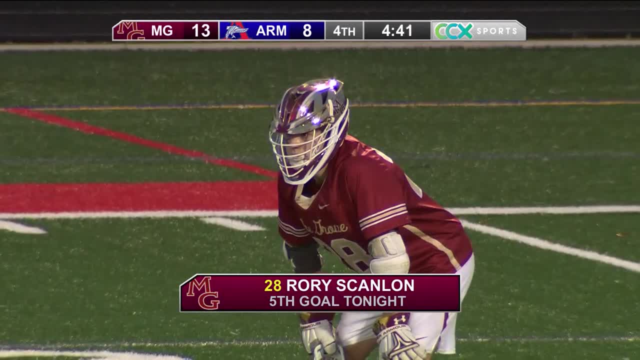 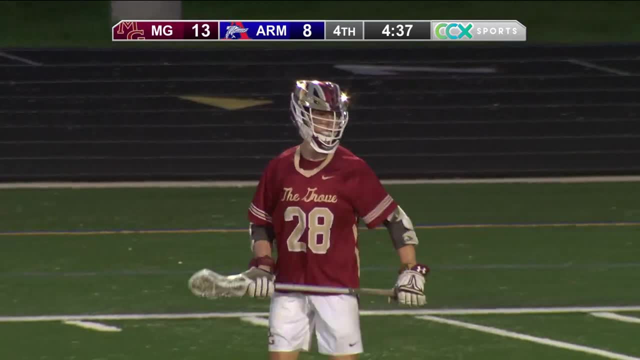 Well, you're seeing two: 44 to the fourth. Important it is to move the ball and stuff and especially move the ball to the guy that's scoring right now. It's got the hot hand And Correct myself, He's got. 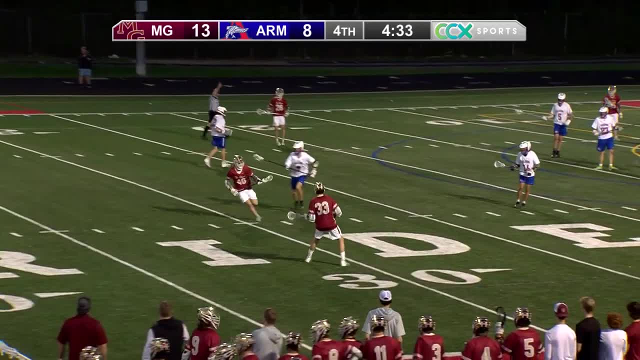 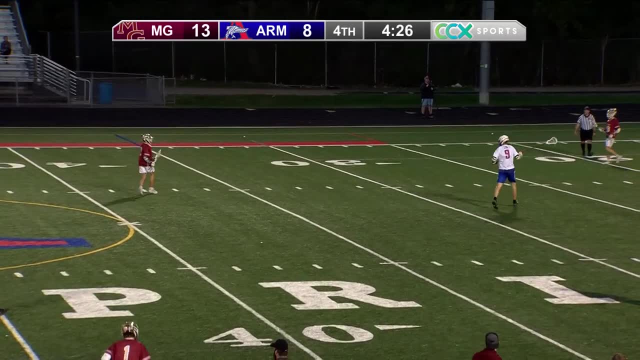 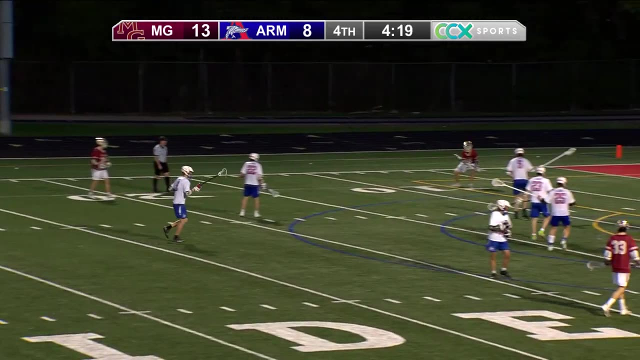 He's responsible for eight points tonight: Five goals and three assists. Rory Scanlon has really led the way. In case you're wondering what his season totals are now: 29 goals and 14 assists. So there's a chance he could leave here with 30 goals. 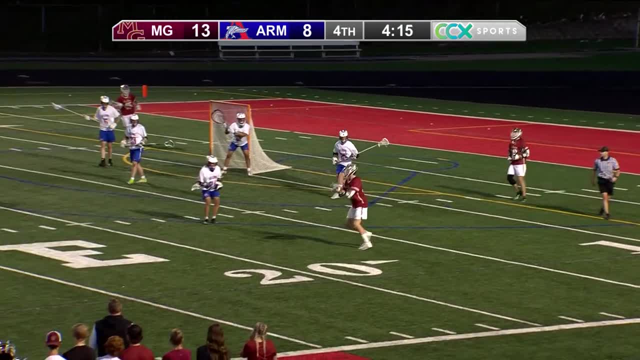 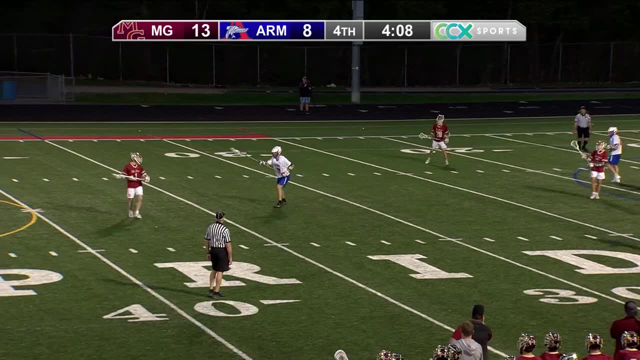 for his senior season. Peterson, Brendan, Up top for Steinkopf. Now we'll see if they've adjusted, or Scanlon, if they'll still find someone in the middle for him to feed it to. Armstrong has not made the adjustment. 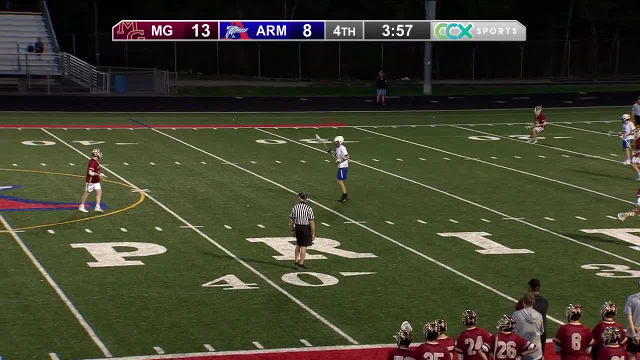 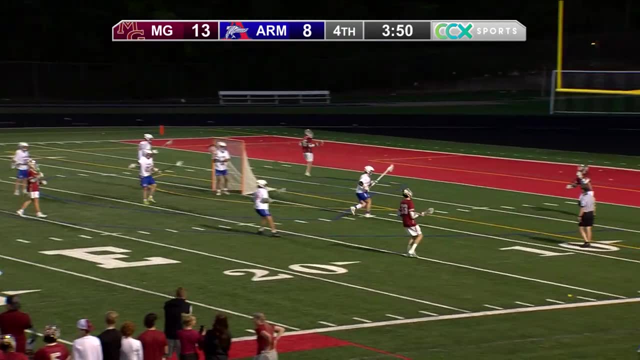 to that attacker in the middle. Well, there's the adjustment. They've got the long stick out high. now trying to prevent that pass from going in Might be too little too late, though. We've got under four minutes to go here in the game. 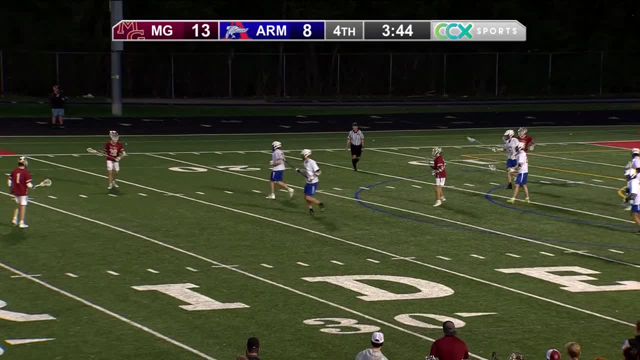 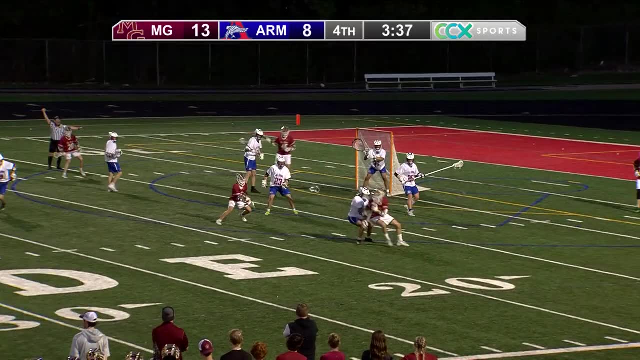 and a 13-8 deficit. Well, they're going to have to get aggressive here before too much longer and start double-teaming the ball. Yeah, and the ref will tell him to keep it in pretty soon. Brendan Spinning middle. 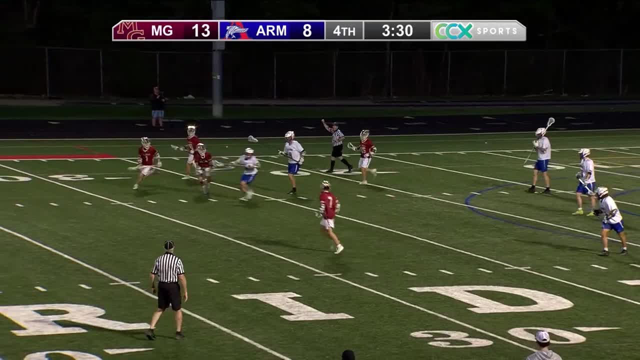 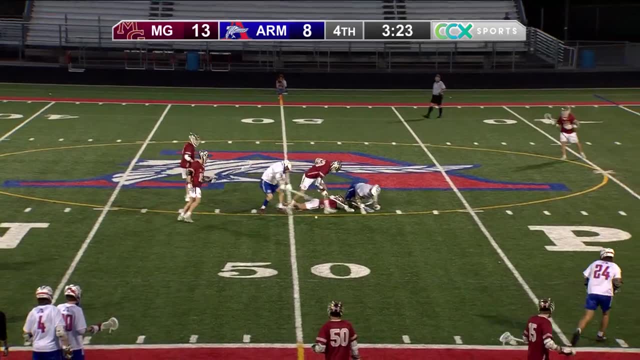 And there's the keep it in sign. It's knocked free off that errant pass. And now Armstrong tries to clear. Big check delivered by Thompson. I don't often see a freshman willing to throw his body around like that, But it's going to be Armstrong ball. 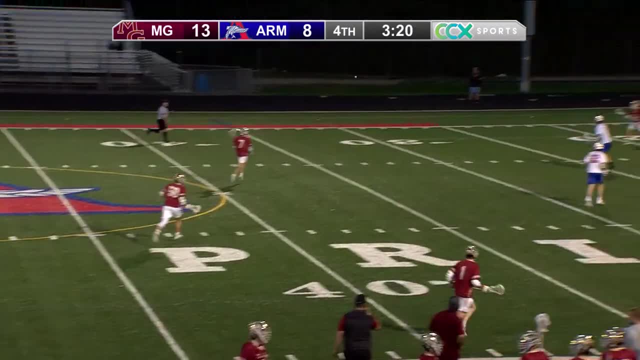 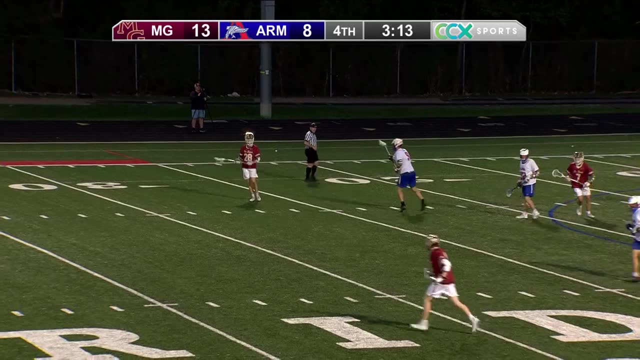 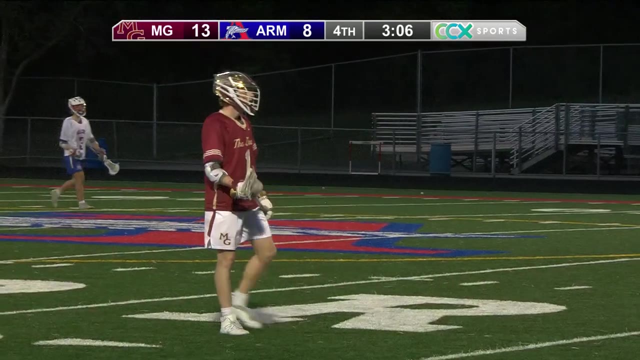 Oh, I think Maple Grove's getting it. Yeah, take your part. Thompson Re-enters, play And Scantlin will be in no hurry. Five goals and three assists- I don't remember off the top of my head. 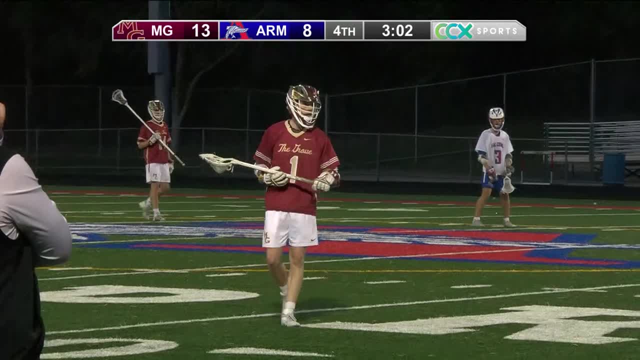 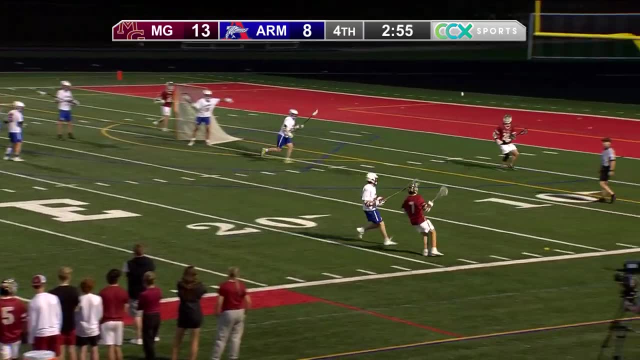 but he had good numbers last night too. So it's been a productive week for Rory Scantlin. Yes, it has Steinkopf. Well, Maple Grove really asserting themselves here in a big, big game. They've really stepped up. 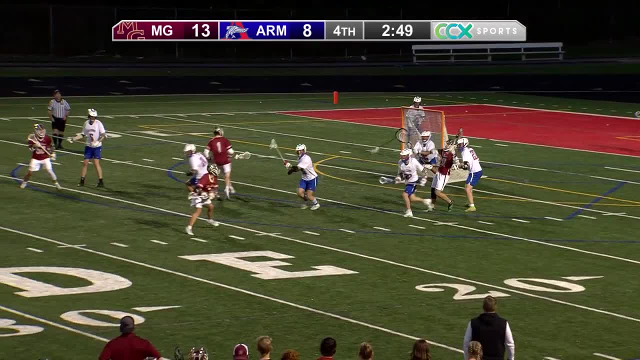 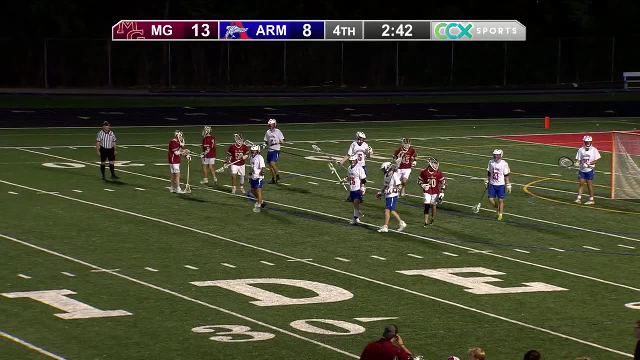 and they've met their game average of goals: Peterson for Steinkopf For Thompson. Rather Wells makes another tremendous save, punching it out Steinkopf. you talk about that adjustment, Dan. He's got four second-half assists. 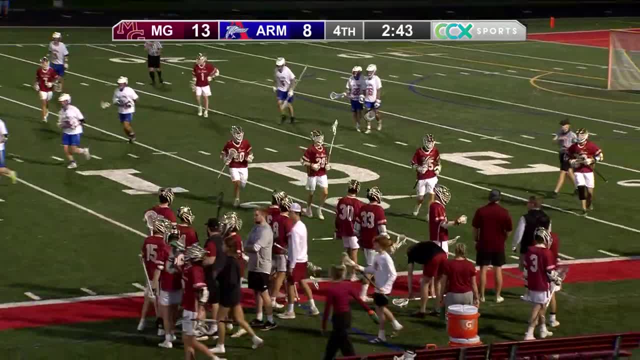 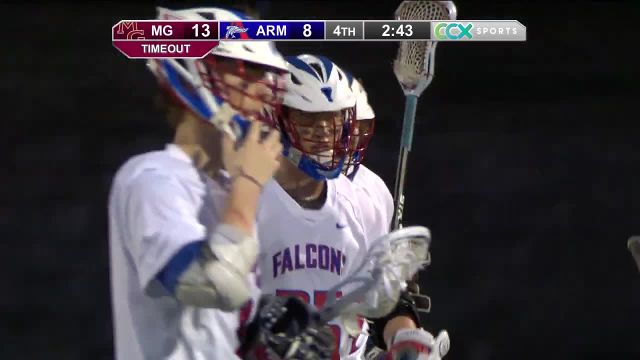 two in the third quarter and two in the fourth quarter, As a timeout is taken on the field by Maple Grove with 2.43 to go and a 13-8 lead for the Crimson. So unless something crazy happens, we'll set the scene here. 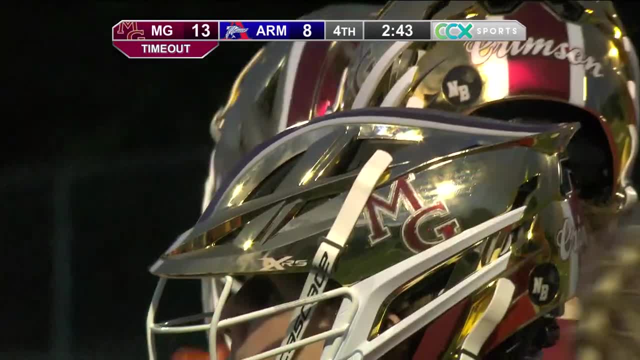 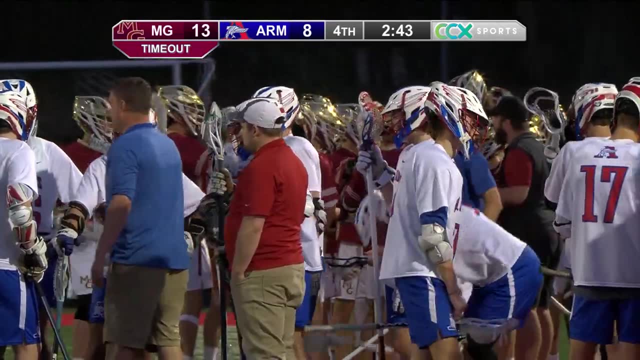 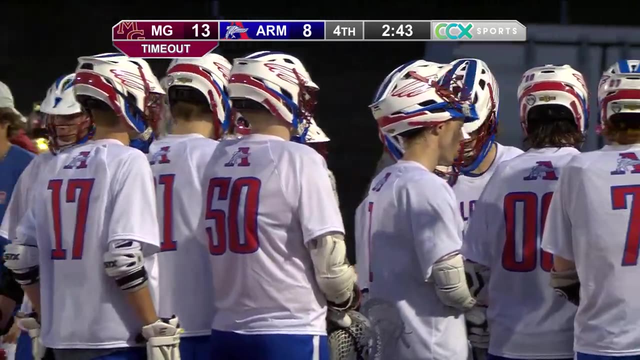 Crimson will improve to 8-1 on the season, 8-0 overall, And Robbinsville-Armstrong will suffer their second defeat of the season and their first conference loss, to fall to 6-1.. But the Crimson will have that lead. 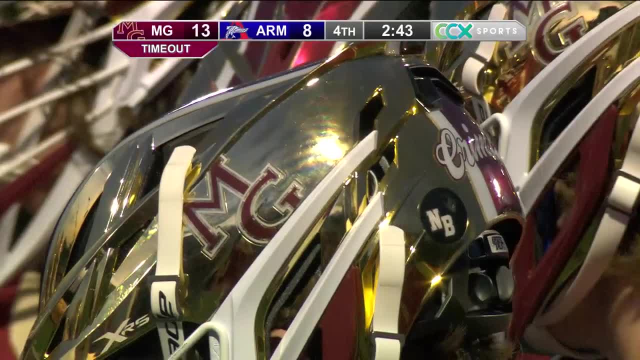 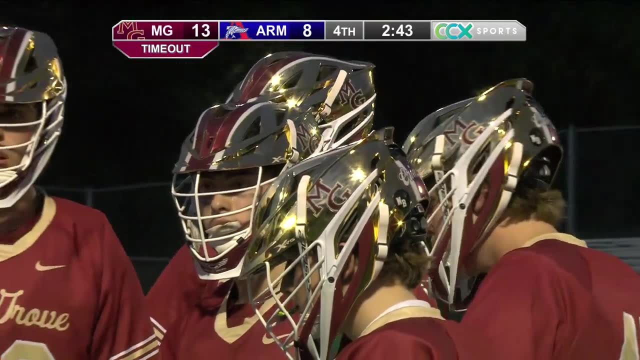 on the top of the Northwest Suburban Conference with just, I think, four or five games left to play, Got a lot of weight to hopefully putting up a conference banner, but again we've got the sections coming up here in these two teams. 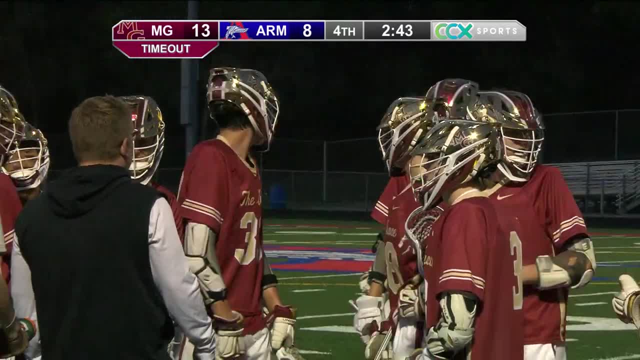 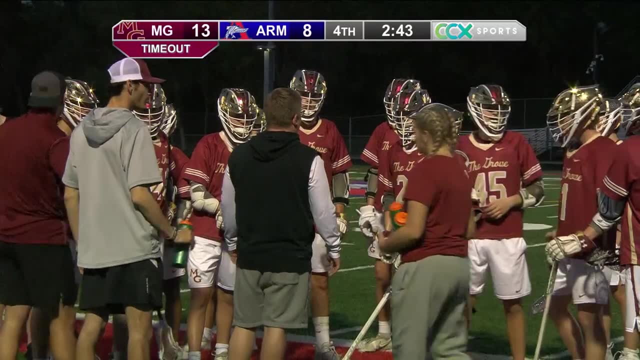 You're in the same section, Yeah, And so this would be nice, but it's going to be 0-0 the next time they meet. Well, and if you're just projecting ahead to section play, what'll be interesting is 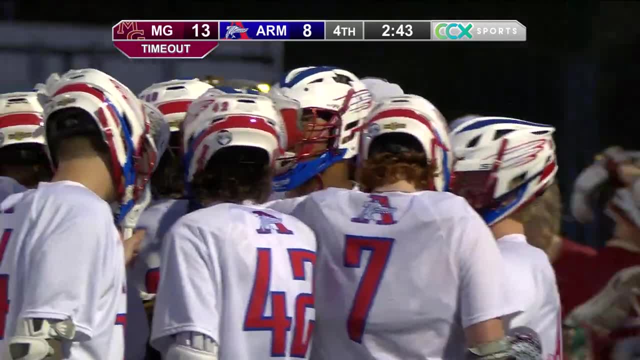 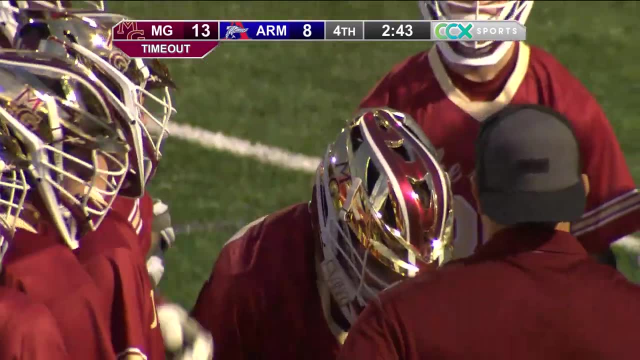 does Maple Grove get the two-seed or the three-seed? Benilde presumably gets the top seed, Robbinsville-Armstrong probably the four maybe, And then does you know, Wyzetta or Benilde or Maple Grove, rather get. 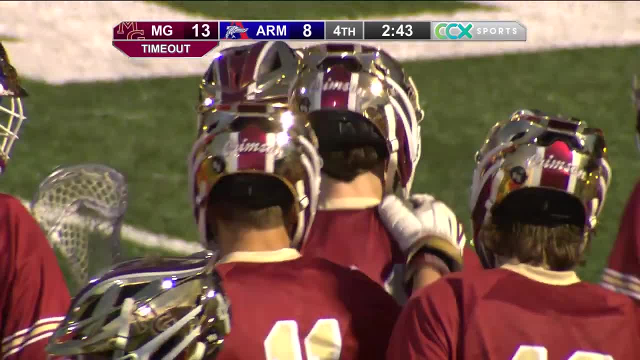 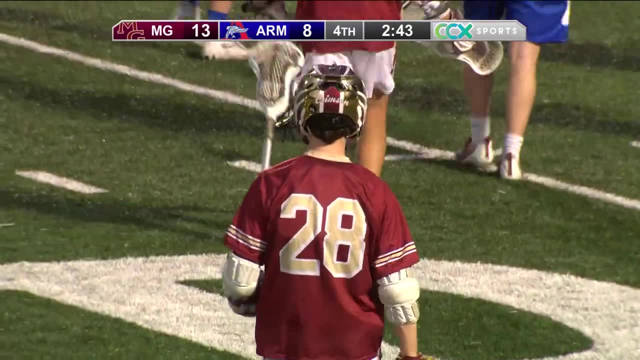 what seed do they get? And you know, we'll just have to see how things play out. The two teams don't play each other, That's it. They don't play each other, They don't meet head-to-head, so it's going to be up to the placement. 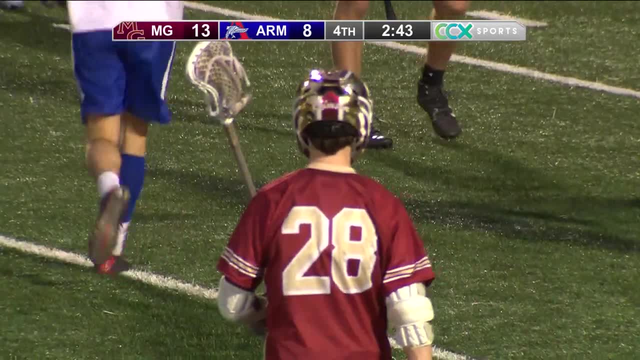 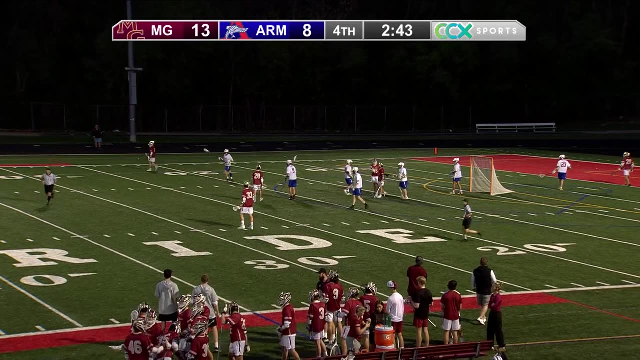 in the section committee at the MSHSL, but we'll see what happens. Either way, you know you're going to have to go through them. Got to beat the best to be the best, That's right. You got to beat the defending state champ. 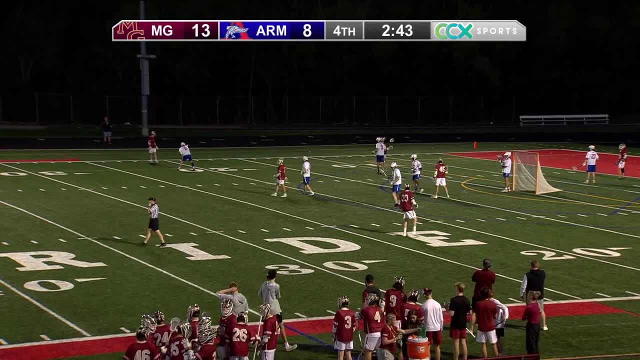 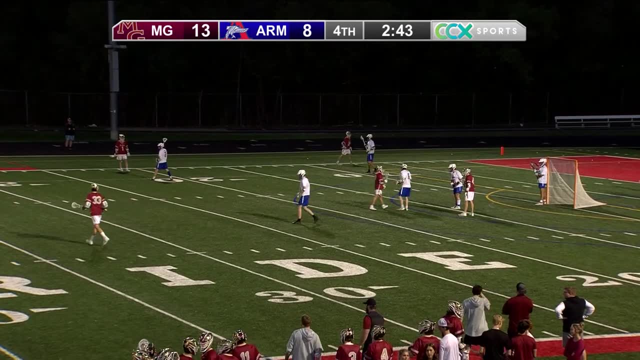 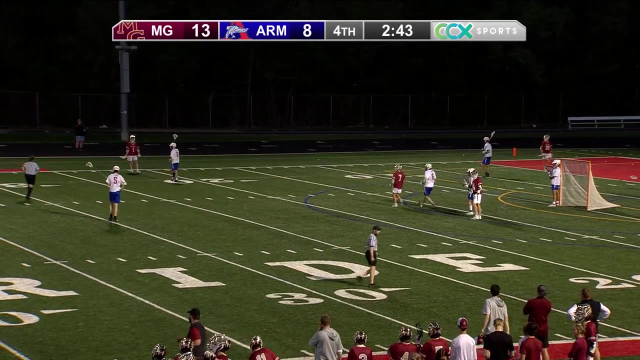 and they look like. well, we'll see. Yeah, they've been perennial powerhouse for a reason, even with a new coaching staff. Now the refs talking to the Armstrong coaching staff a little bit about something, But we're back to action here. 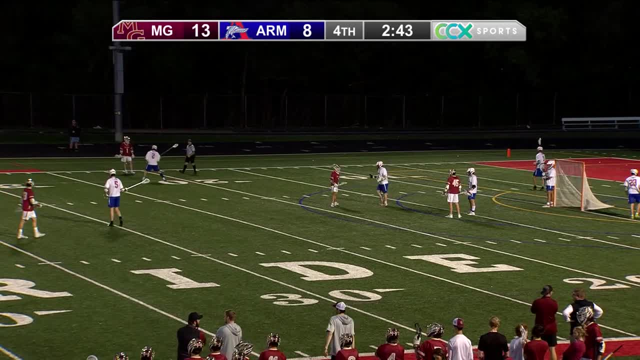 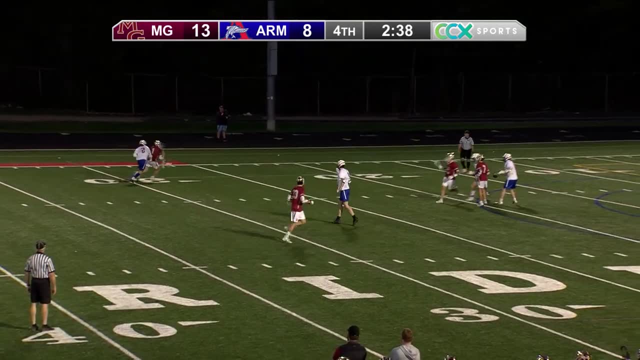 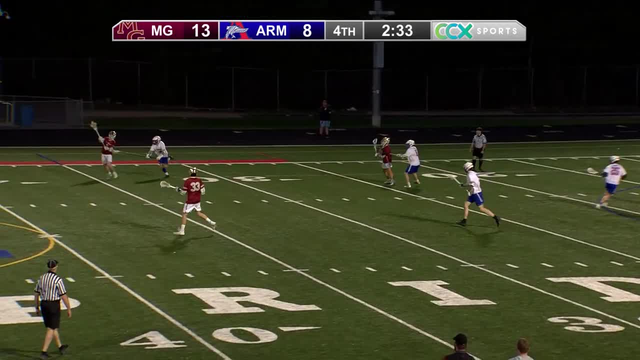 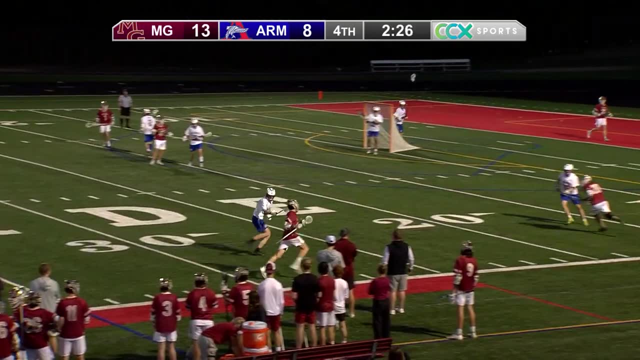 Oh, and actually you know who's out there with a long pole is Nate Albrecht. Oh, really, Yeah, Oh good, pickup Number two, because you just hear the parents saying: come on, Nate, and Albrecht is hounding. 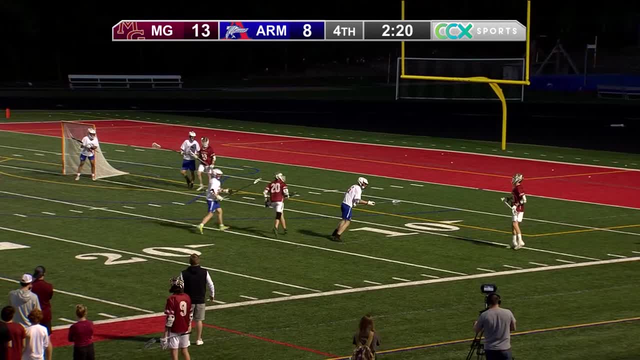 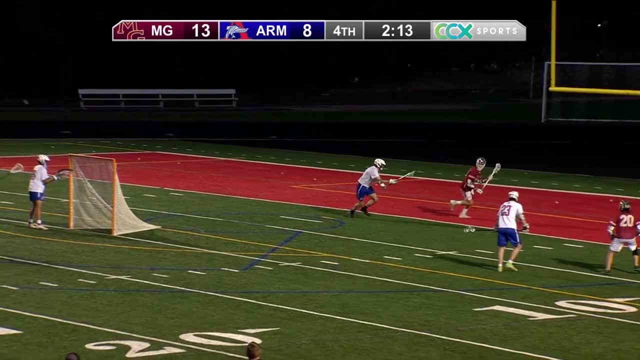 trying to get the ball back, So they got Albrecht out there with a long pole. Oh, I like the creativity as they try to get the ball back. Didn't work, So Brendan jogs back behind X. Why not innovate? 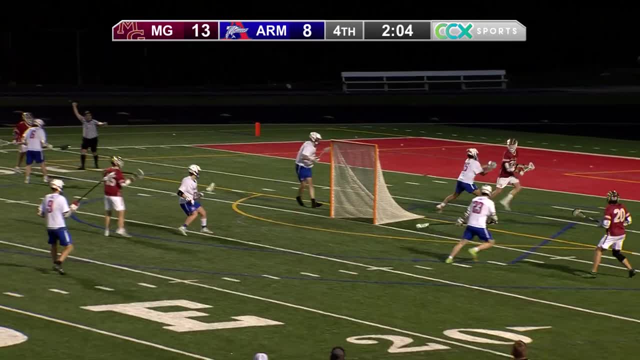 Why not innovate? Why not? Why not, right You bet? Try something new man, Something to throw at the other team to kind of make them look like what Five-goal deficit. with two minutes left, You got to do something. 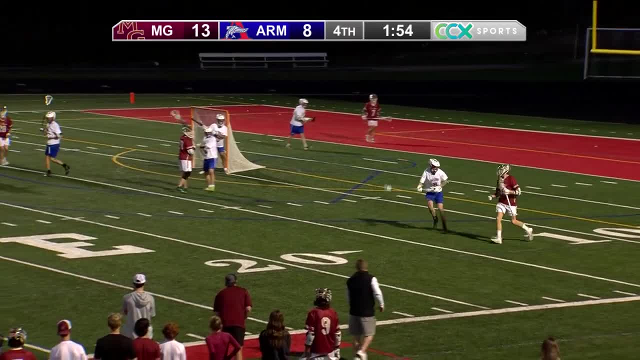 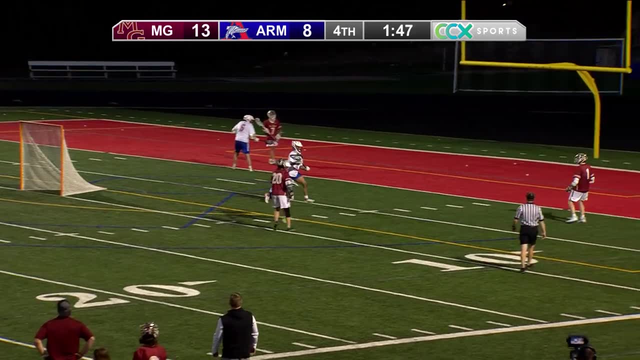 Is Brendan Scanlon cutting to the goal, but they didn't find him, So Brendan will jog it up top. Casual catch for Steinkopf. It's amazing how much more skilled the lacrosse is here than it was even a decade ago. 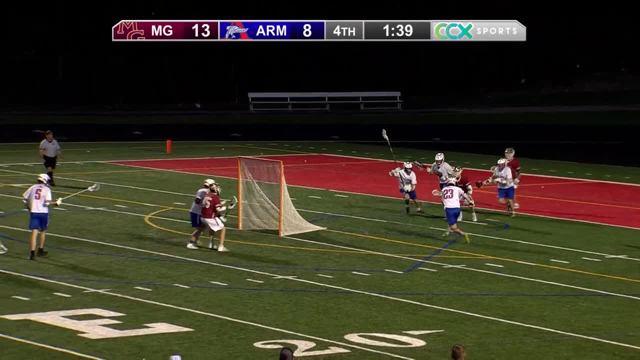 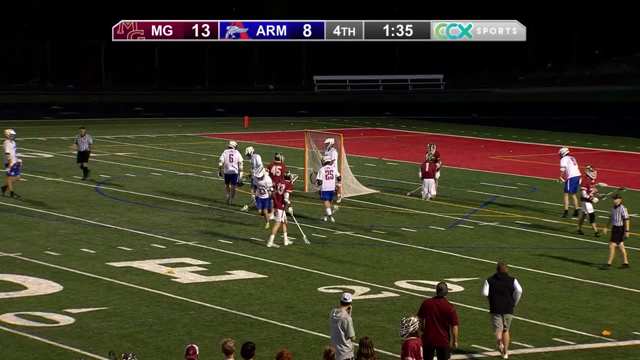 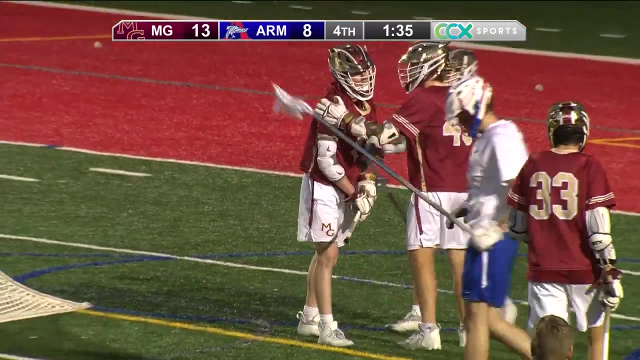 Oh my gosh, Not even close Steinkopf, Nice to feed. in front A flag flies. Someone is down Steinkopf, I think may have gotten hit as Coach Ficken on the field. Let's check on his player. 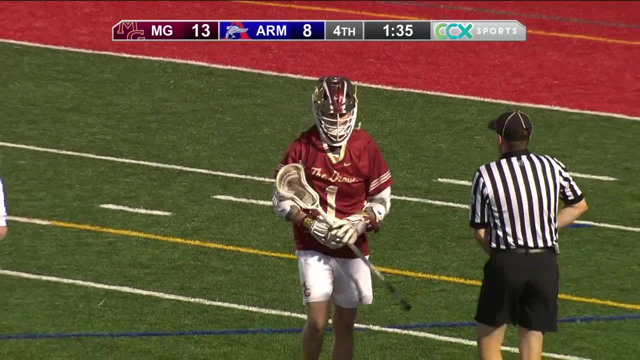 Steinkopf's day will be done. Yeah, you don't want to lose Mr Steinkopf. He's had an amazing game today. Yeah, he really has. Steinkopf came in with five assists. He's nearly got five. 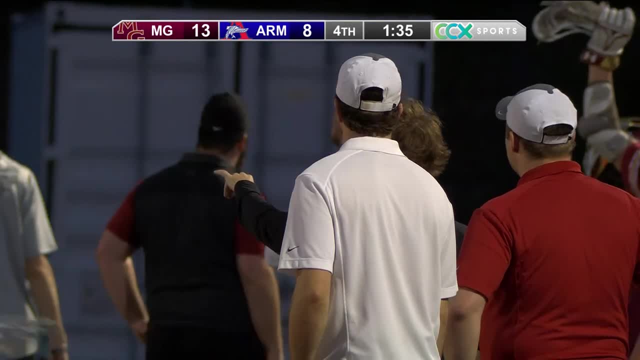 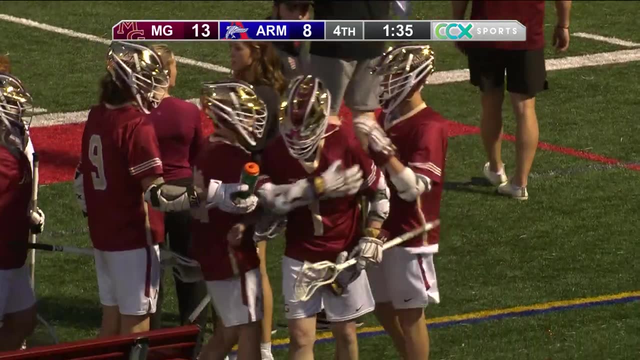 Five assists here in the second half. Yeah, he's been the feeder, so to speak, for the big dogs to eat, So his day will presumably be done after he took a big hit. Get the ice bags out, son, You'll get through it. 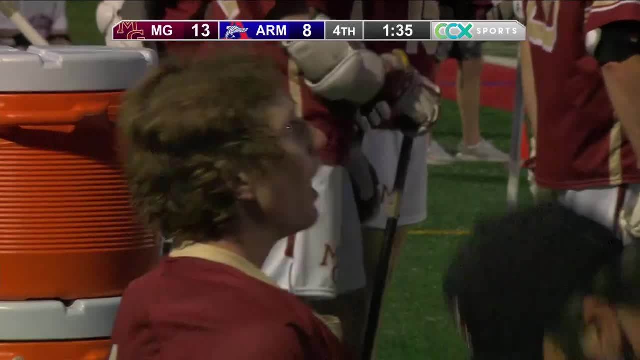 I always used to get a kick out of him too. I remember when Cal came home from hockey he complained about his bruises. He came home from lacrosse with more bruises. He wouldn't say a word about it. It's just part of the game. 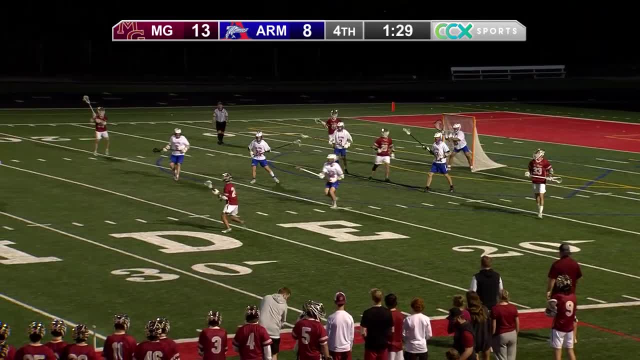 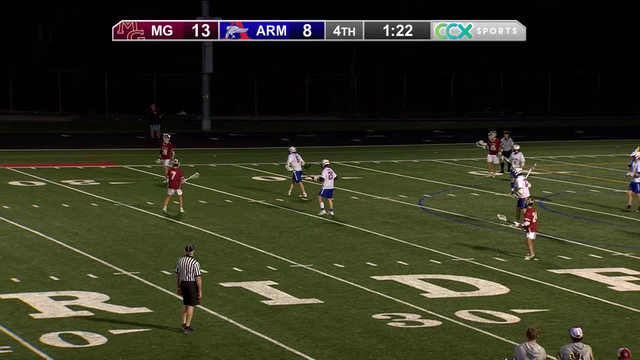 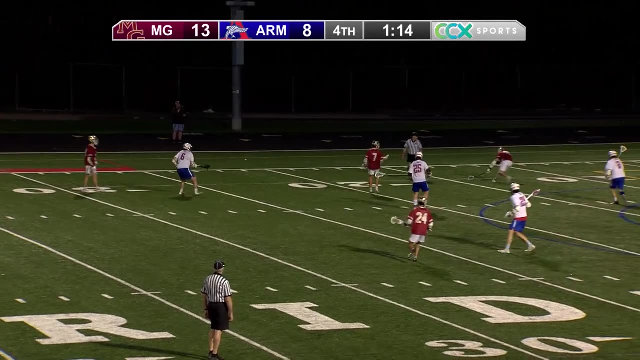 Yep And then with a minute 30 to go, Well, a big win for the Crimson here and then puts them solidly in control of the conference and the section right now where they want to be comparatively Yep- I mean undefeated in section play at 4-0, so nothing. 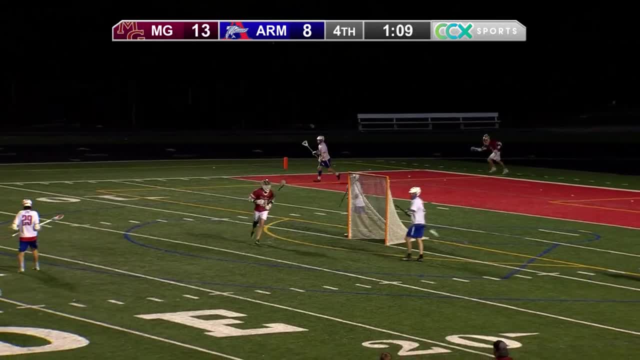 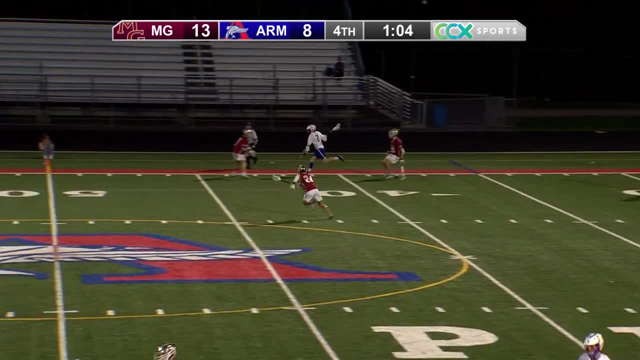 Can't complain about that. And really, you know, like your son said, the first real test they've had this season other than the non-conference game against Chan Mm-hmm, And for them to, you know, For them to score at their season average right 13 goals. 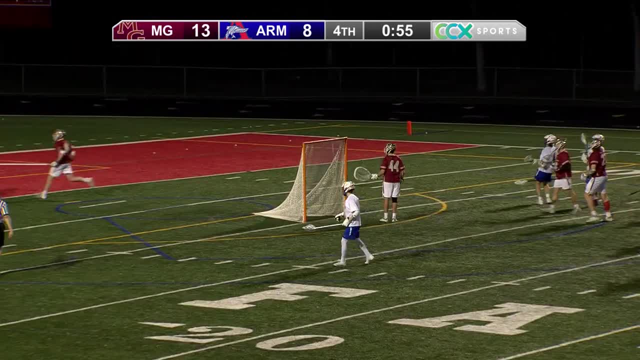 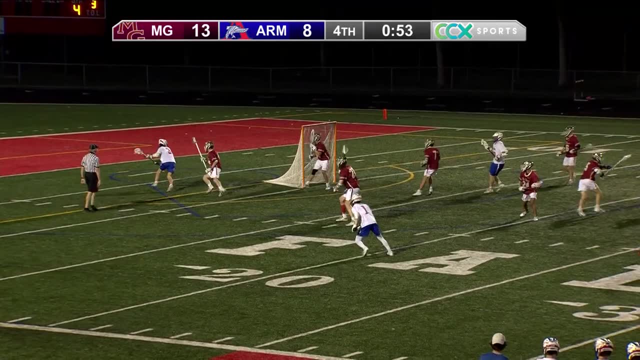 Yep, So the offense humming along. Coe missed the net on that shot, as we're under a minute to play, So I think the Crimson you know can safely say: hey, we passed our first real test of the season Olsen. 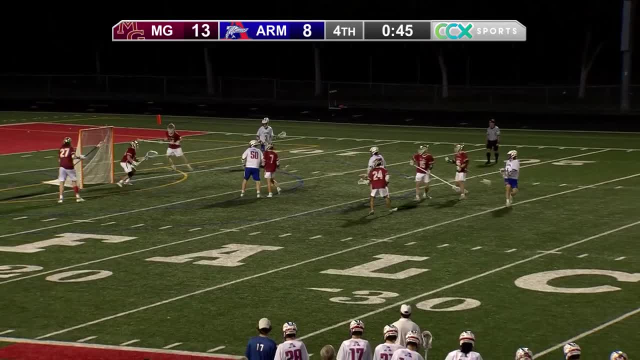 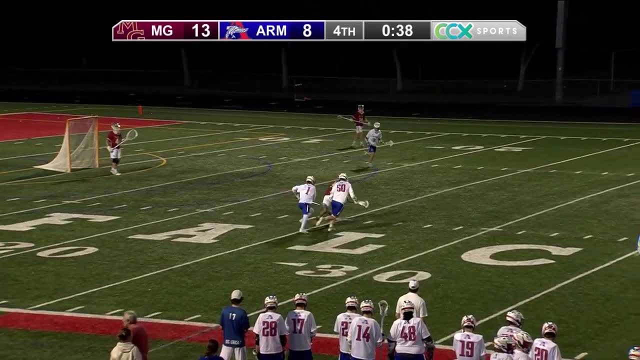 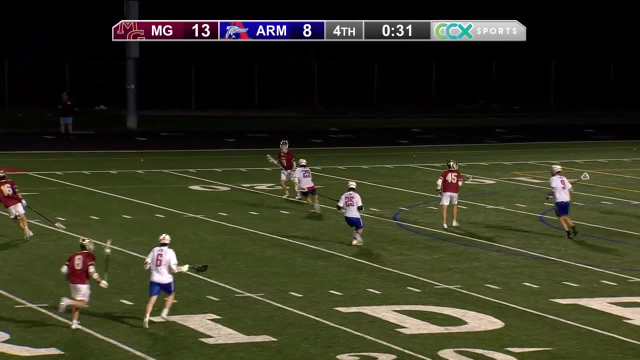 Olsen Feeds for Coe. His bounce shot harmlessly into the big butterfly net of Farniak. Good outlet here by the Crimson And they'll pull it back with 30 seconds left on a five-goal lead. Nice, smart play. 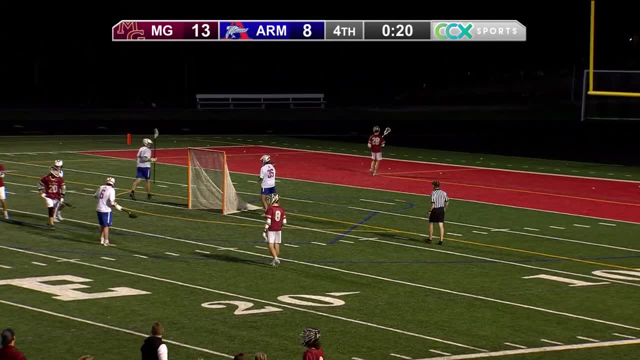 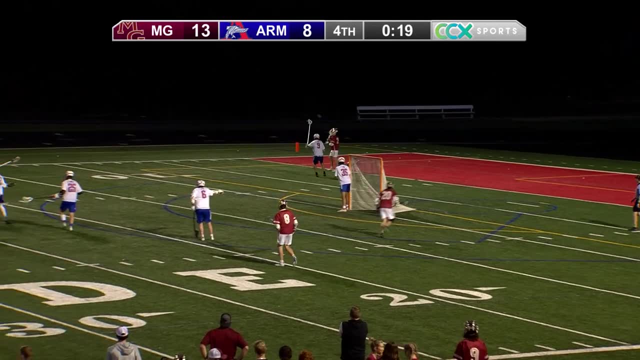 Peterson goes high, low and Wells stones him 20 seconds left. It would have been academic, but still a beautiful stop by Xavier Wells, his seventh save of the night. He's done a tremendous job. Some of those saves have been just spectacular. 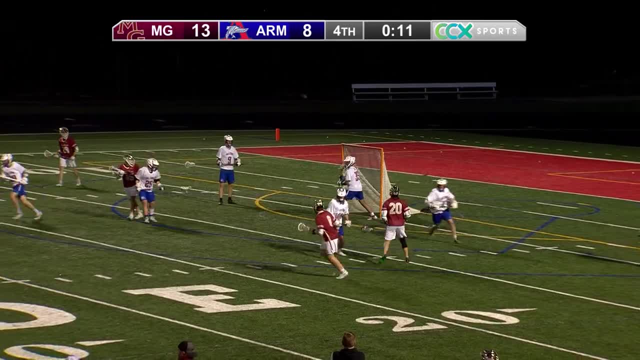 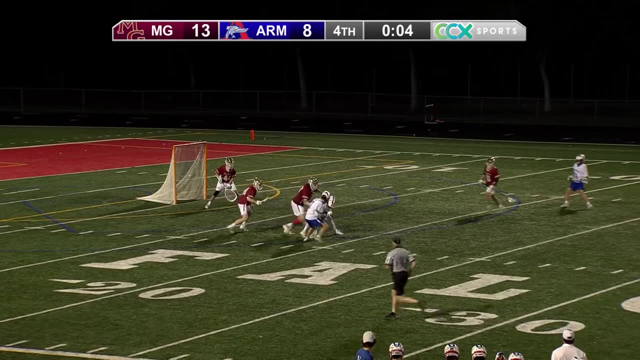 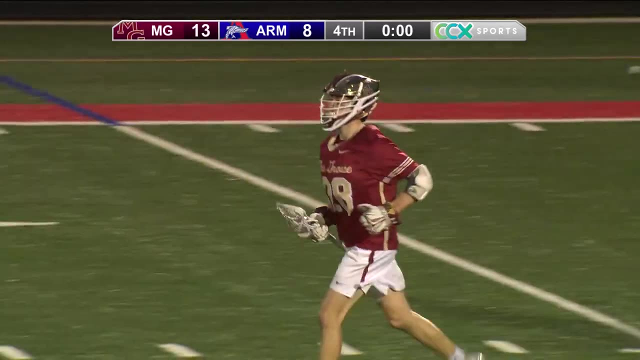 Oh my gosh. Peterson wants one more and Wells makes yet another save. He'll chuck it down to the other end. As time runs out here in the Plymouth, Take a look at the new, updated standings in the Northwest Suburban Conference. 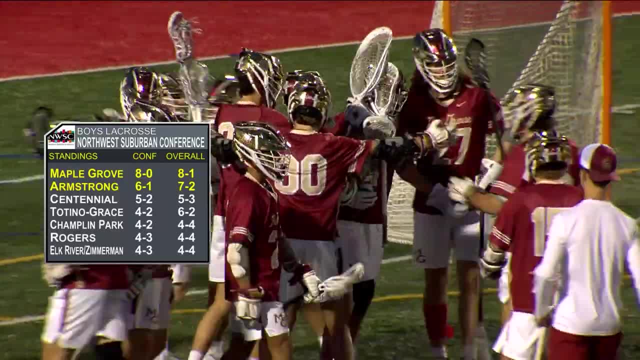 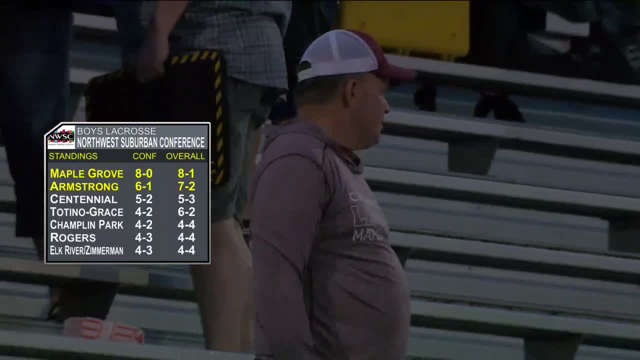 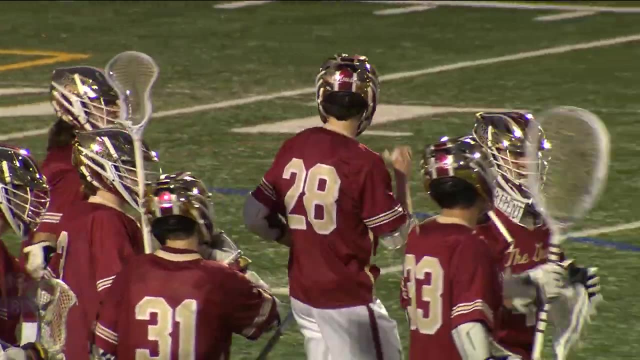 Maple Grove now with a game-and-a-half lead over Armstrong, with it 13-8 victory here on the road to improve to 8-0 in the conference, 8-1 overall Armstrong with the loss Falls to 6-1 in conference play and 7-2 overall. 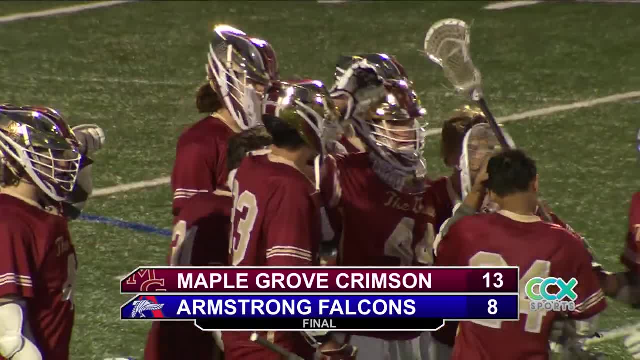 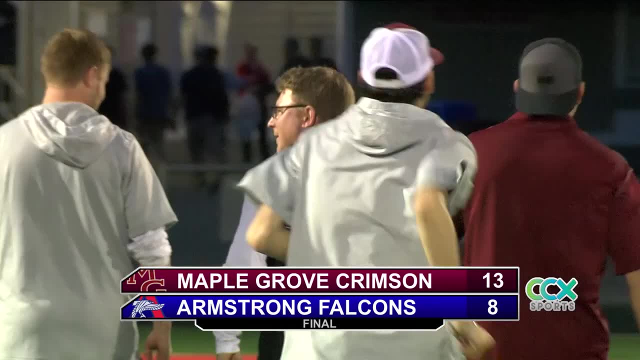 But just a massive win for Kyle Ficken, Dan, your son and his Crimson. Yeah, just the fourth quarter did it. They played like they do the regular season. Their best quarter has been their fourth quarter and they've learned how to finish this year. 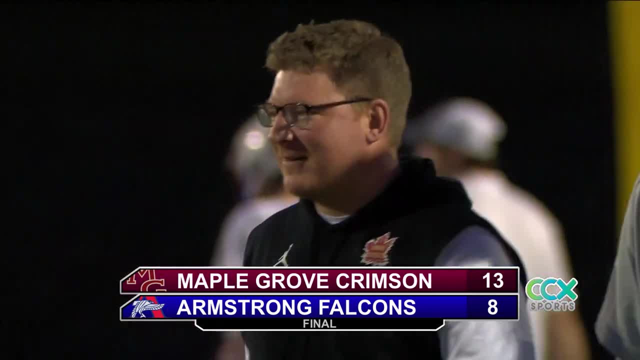 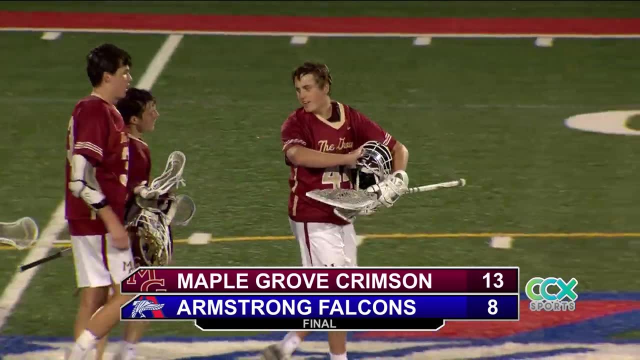 And you can see he's got a satisfied smile on his face that they did it again. So it could be a nice year for the Crimson, And with good reason. absolutely. Rory Scanlon's five goals and three assists lead the way for the Crimson. 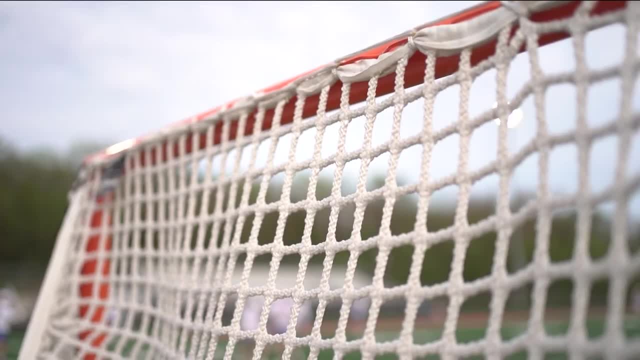 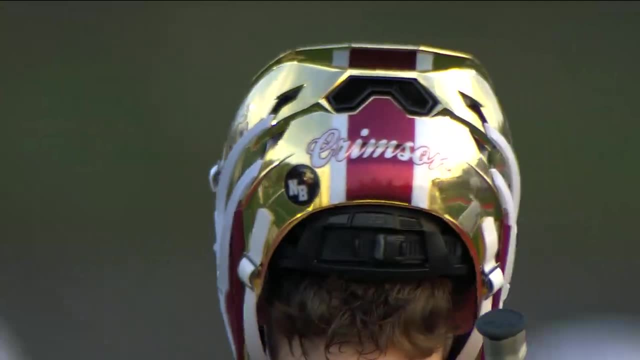 who pull away in the fourth quarter and earn a hard-fought victory on the road here in Plymouth. So that'll do it for us here from the Falcons' nest, For my broadcast partner Dan Ficken, Director Isaac Rice and our entire CCX crew. 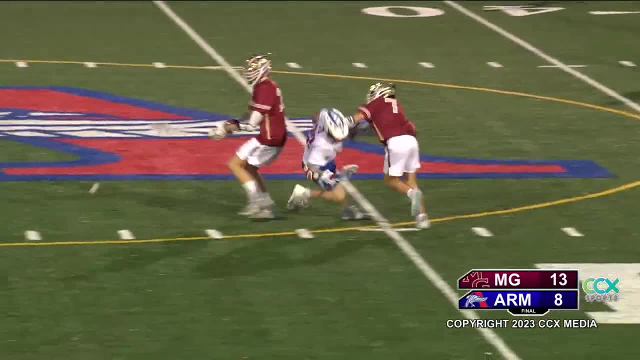 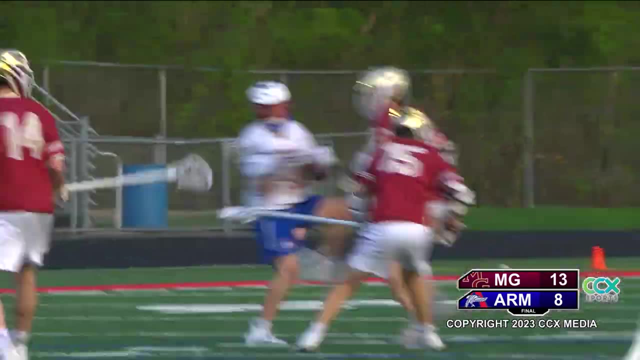 I'm Bill Hupp saying good evening From Plymouth, the final Maple Grove 13,, Armstrong 8.. Thanks for watching this presentation of high school boys lacrosse on CCX, CCX, CCX, CCX, CCX. 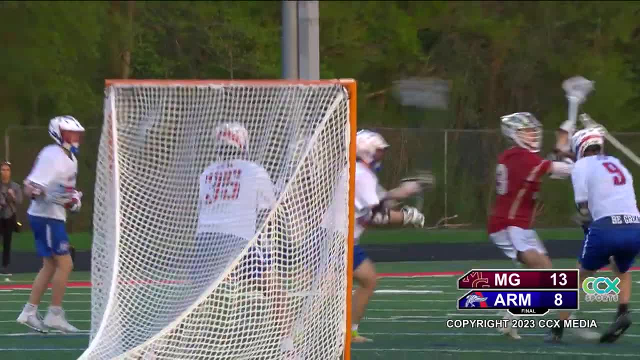 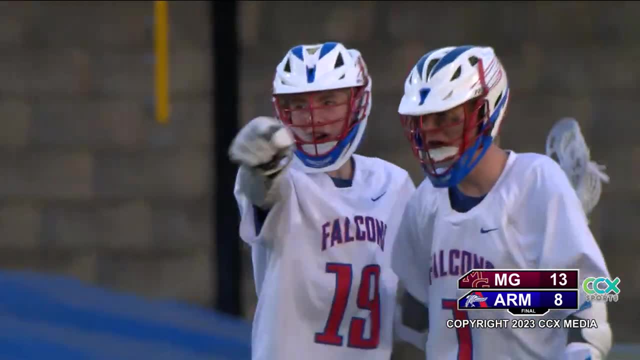 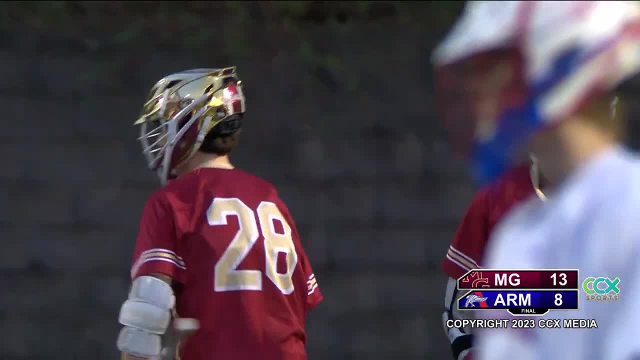 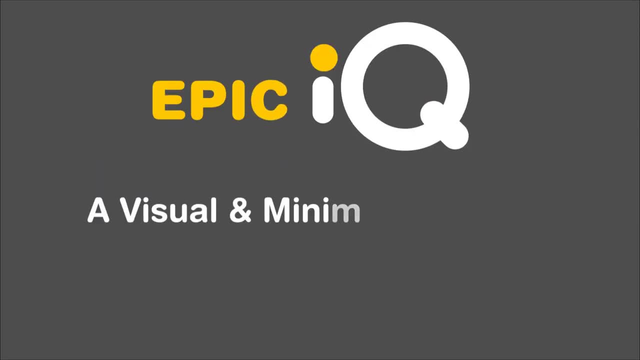 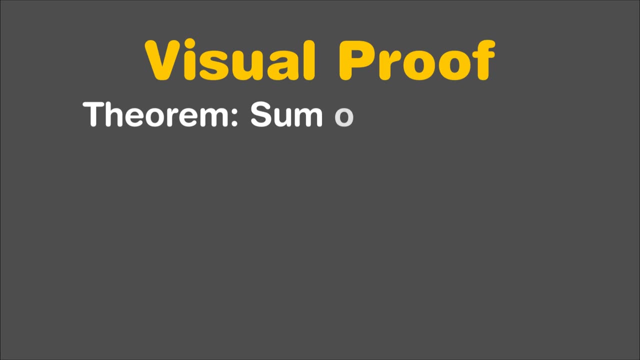 Epic IQ: A Visual and Minimal Approach to Learning and Education. The theorem states that the sum of the first n odd natural numbers is always a perfect square and is equal to n square. This can be proved in a number of ways, but there is also a proof without words.